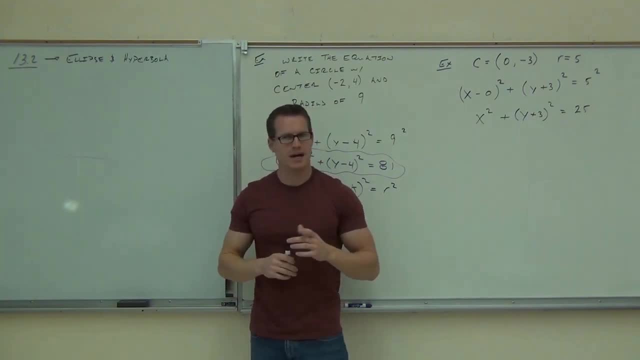 Now there are a couple other shapes, one of which you might have seen before. The other one I guarantee you haven't- We're going to talk about in section 13.2, ellipses and a hyperbola. 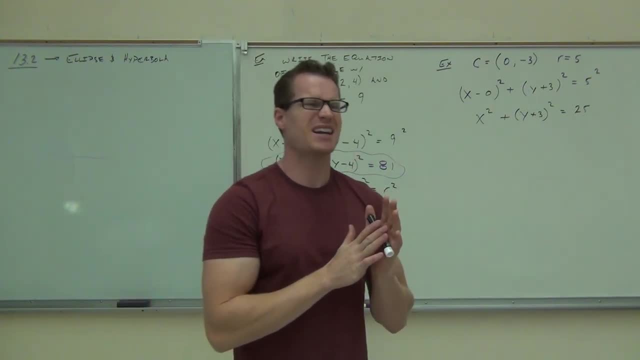 Now, an ellipse is kind of like a circle, but it's not exactly a circle. You ever go to the gym and you see those big round like they're usually blue or gray, those exercise balls, And they're pretty much. it's a sphere actually, but if you look at it from the profile it's a circle, right. 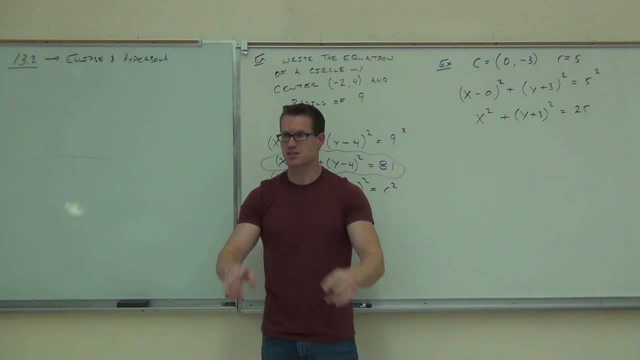 Now, I'm a pretty big guy. If I sit on one of those circles, is it still going to be a circle? No, it's going to go right And it's going to kind of smush out the sides. Well, it's going to have like a shape in the middle, but ignore that. 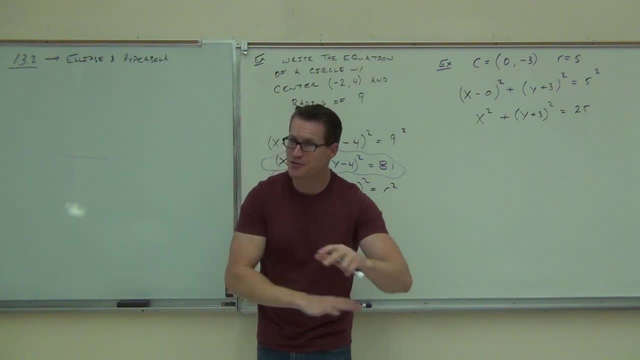 So and it's going to be completely flat on the bottom, But if you ignore the completely flat part, it looks kind of like an ellipse. An ellipse looks very much like a squished circle. It's what would happen if you took your cone. remember those cones we had. 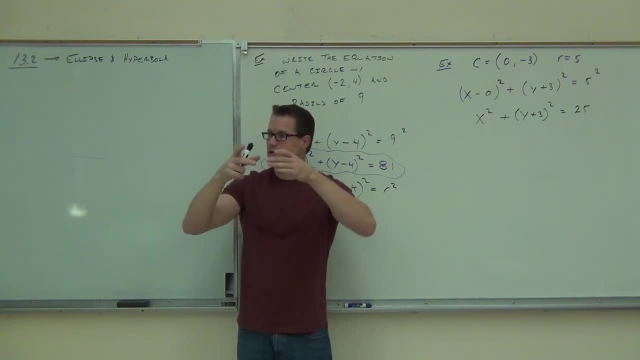 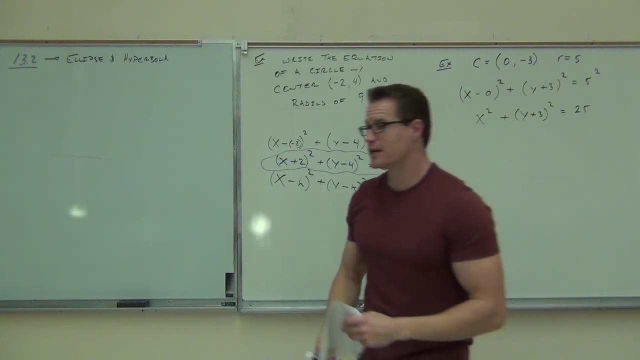 And you didn't slice it straight across, you sliced it diagonal. You're not going to get a circle, you're going to get an ellipse. It's an elongated circle. That's where we get this ellipse from, So an ellipse looks a lot like an elongated circle. 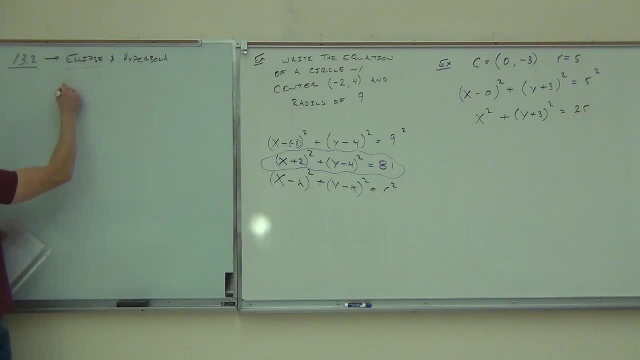 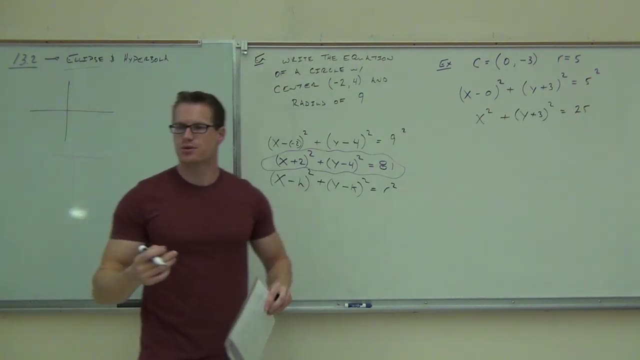 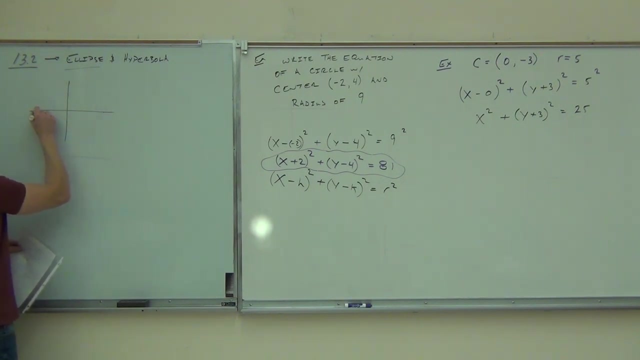 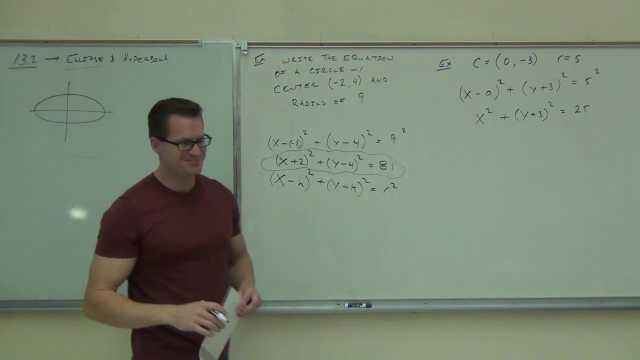 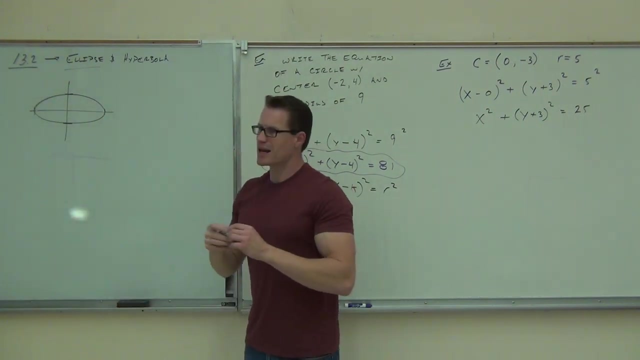 So we'll talk about that one first. So here's an ellipse that's centered around. These are my stewy heads and I've missed my marks. There we go. That's an ellipse, or very similar to an ellipse. It looks kind of like an oval. 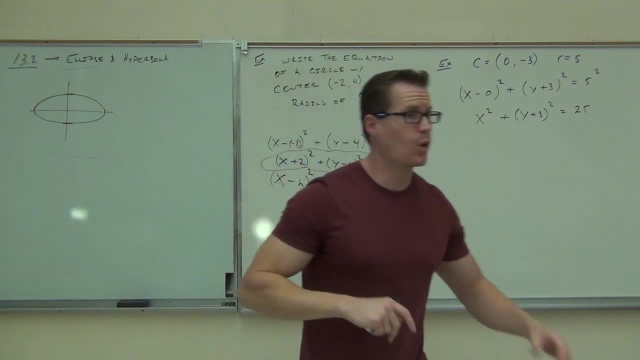 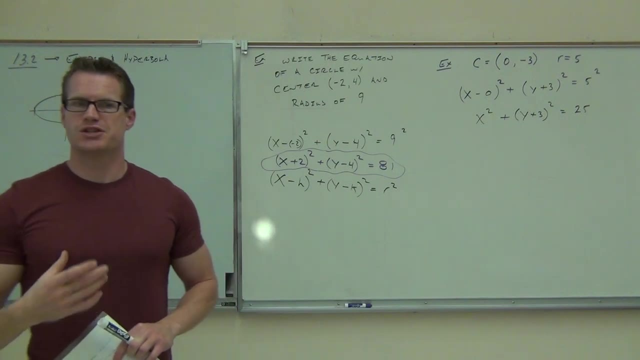 It's a smashed circle. It's a circle that's elongated in one direction. It's either elongated lengthwise or heightwise. Now we have a couple of letters to signify where this is going. Let's cross the x and the y. 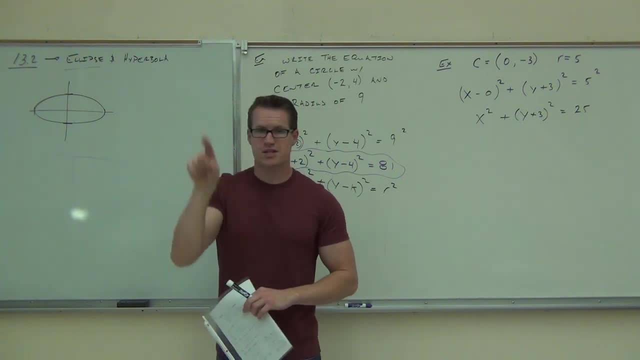 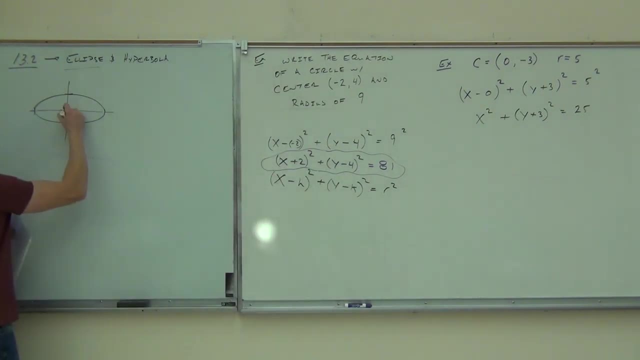 You see, with circles we cross at the center of the same number at all four points right, Because it's a circle, it goes out the same distance in every direction. Ellipses don't, If our ellipse is centered at. 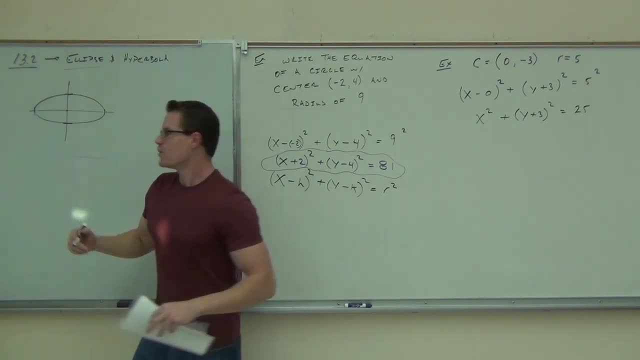 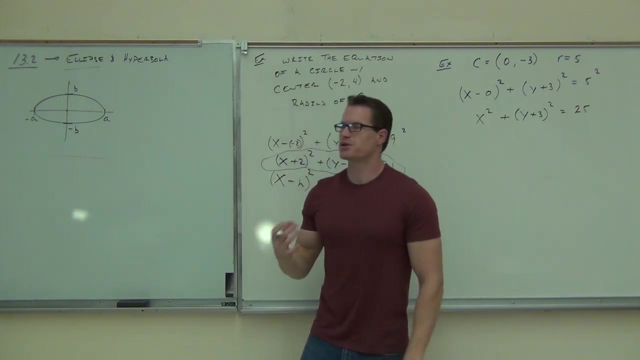 we go out, sure, a certain direction in y and a certain direction in x. We call these points, according to the x coordinates, a and negative, a, b and negative b. Now here's how we associate this with an equation. 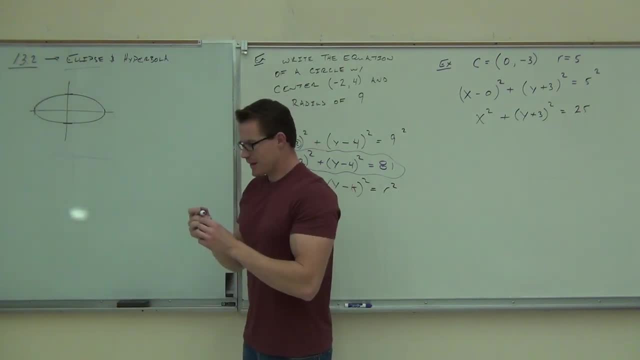 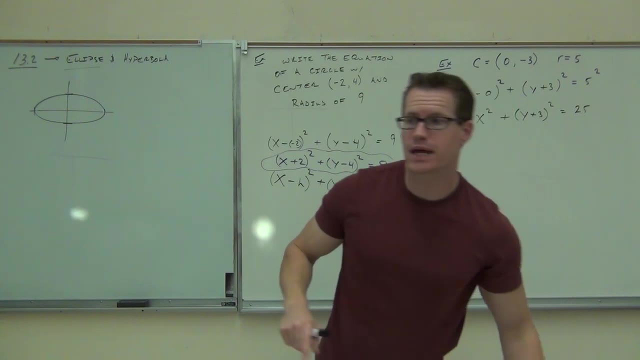 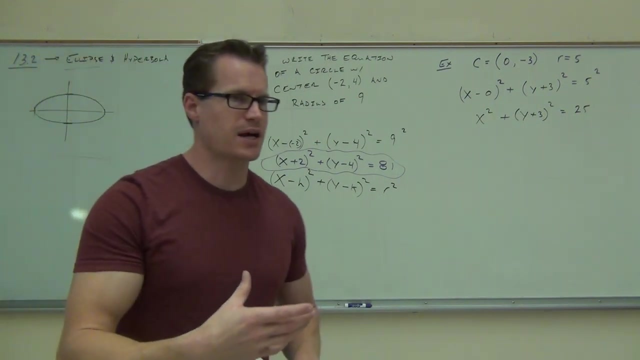 That's an ellipse, or very similar to an ellipse. It looks kind of like an oval. It's a smashed circle. It's a circle that's elongated in one direction. It's either elongated lengthwise or heightwise. Now, we have a couple of letters to signify where this is going. Let's cross the x and the y. 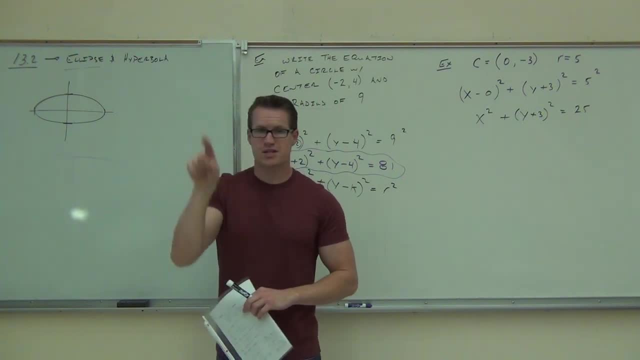 You see, with circles, we cross at the center of , the same number at all four points, right? Because it's a circle, it goes out the same distance in every direction. Ellipses don't. 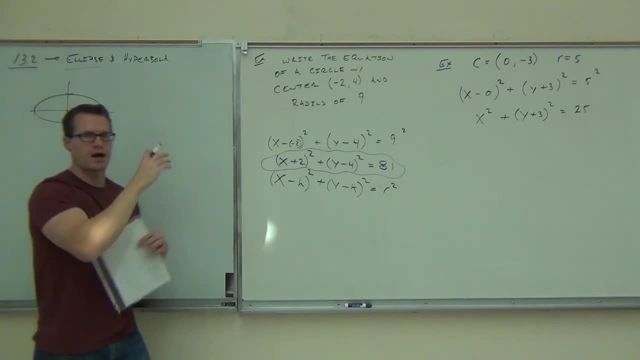 If our ellipse is centered at , we go out, sure, a certain direction in y and a certain direction in x. 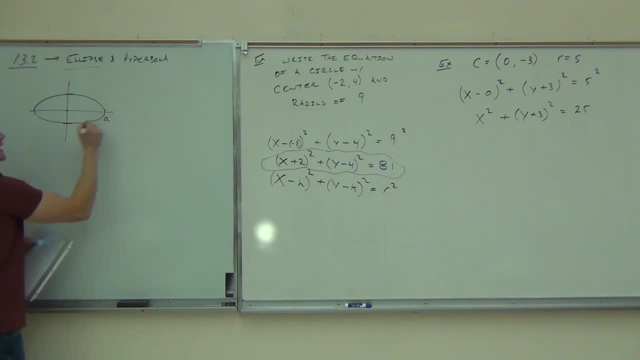 We call these points, according to the x coordinates, a and negative a, b and negative b. Now, here's how we associate this with an equation. Here's the equation for ellipses. 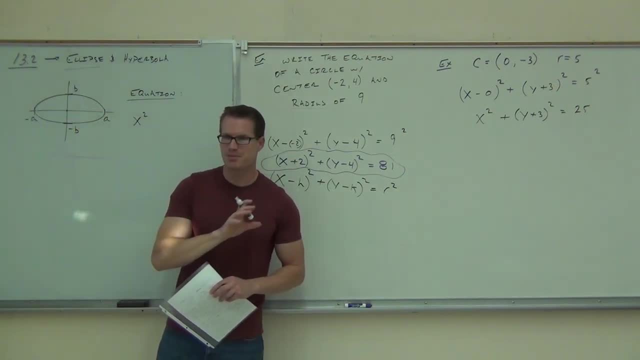 Does that look familiar? x squared is in every shape that we have, parabolas, circles, hyperbolas, ellipses. Does that look familiar? 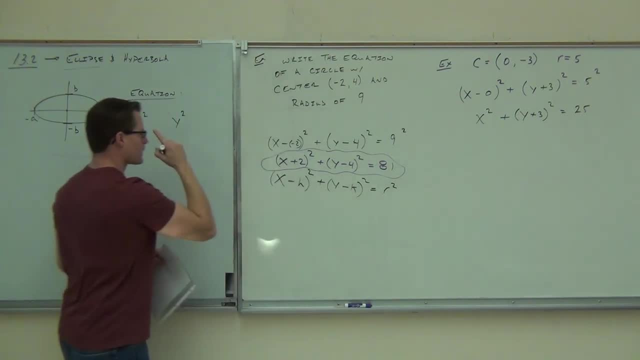 That's not in parabolas, but it sure is in circles. Does that look familiar? Right there, that is a circle so far. Are you with me? That's a circle. Here's what makes this different than a circle. 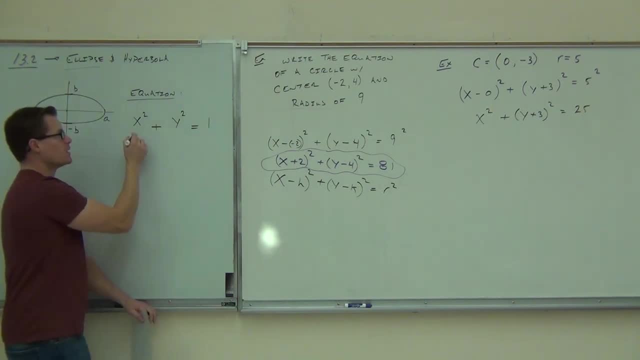 You still have an x squared, you still have a y squared, you still have a plus in the middle of it. 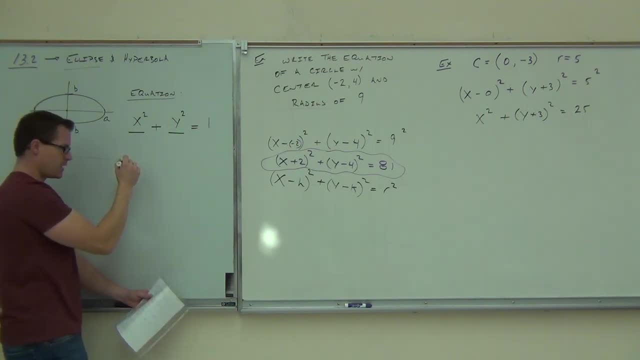 What's different is that these two things are being divided by a squared and b squared, respectively. 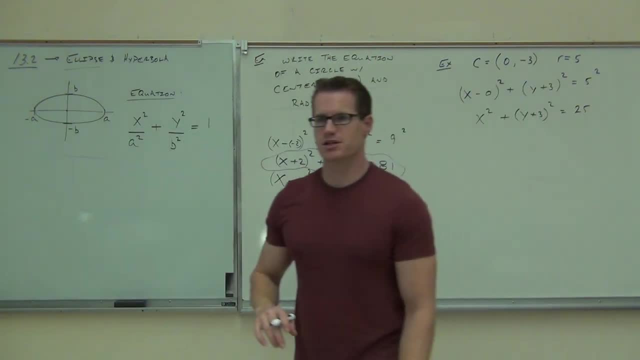 Now, you're going to find this out in just a minute, so I'll give you a hint first. 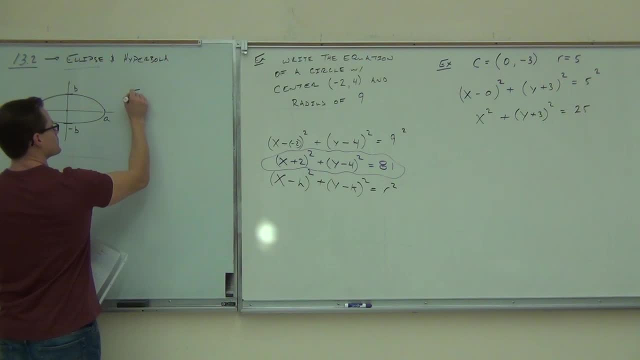 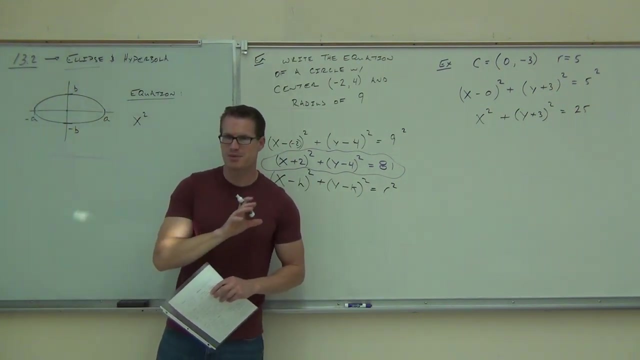 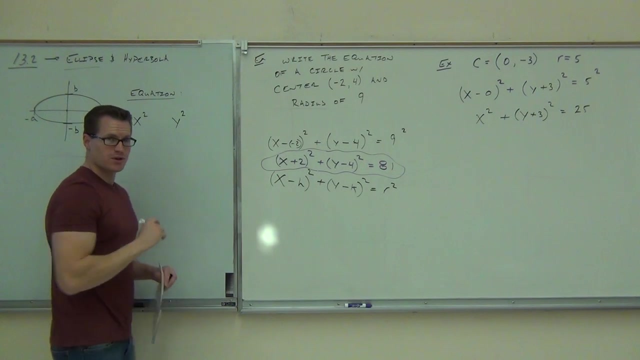 Here's the equation for ellipses. Does that look familiar? x squared is in every shape that we have: parabolas, circles, hyperbolas, ellipses. Does that look familiar? That's not in parabolas, but it sure is in circles. 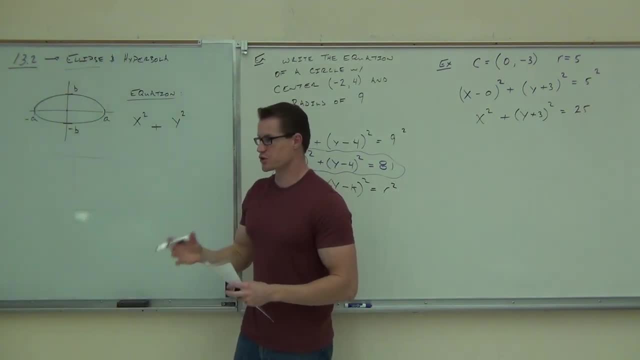 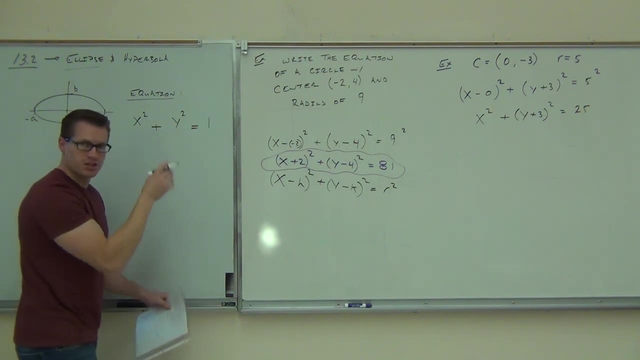 Does that look familiar? Right there, that is a circle. so far, Are you with me? That's a circle. Here's what makes this different than a circle: You still have an x squared. you still have a y squared. you still have a plus in the middle of it. 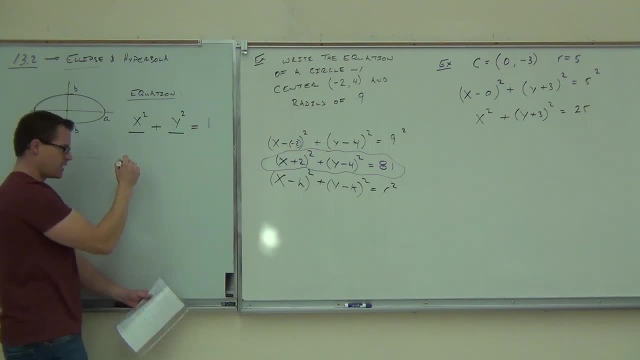 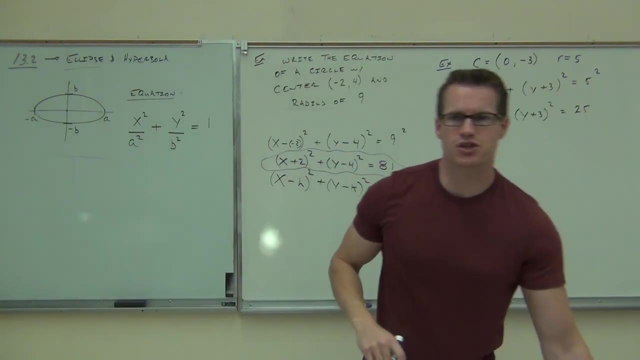 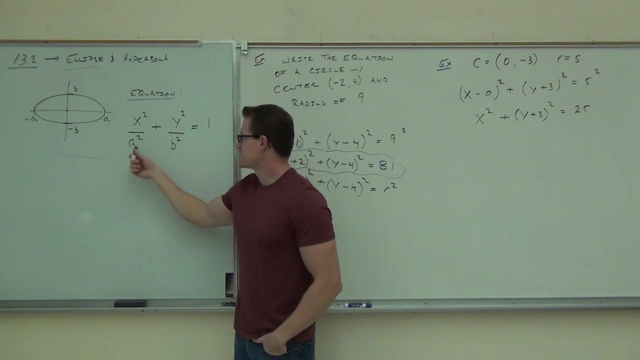 What's different is that these two things are being divided by a? squared and b? squared respectively. Now, you're going to find this out in just a minute, so I'll give you a hint first. In order to be an ellipse, these things have to be different. 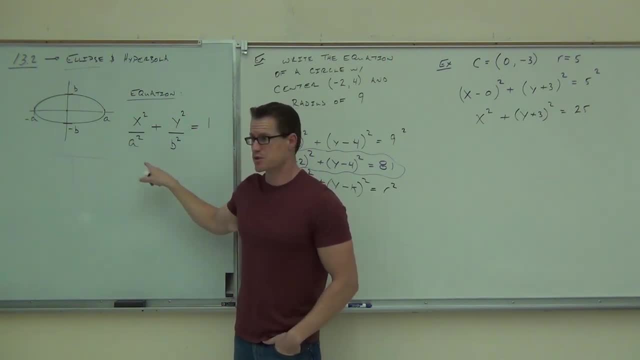 I'm going to prove this to you on the formula right now. Okay, look at the numbers a and the numbers b. Notice how a is given by the number that's associated with x- Are you with me on that? And b is given by the number that's associated with y. 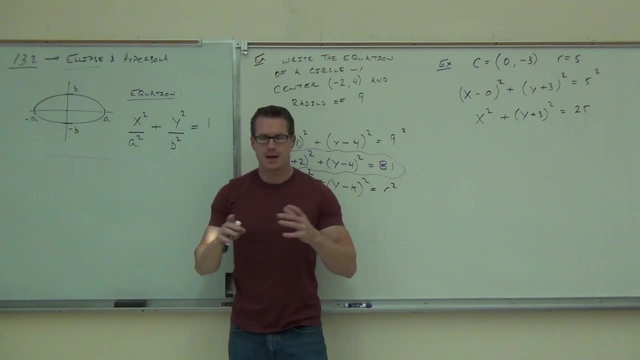 Okay, we got that. What would happen if these were the? Look at the board. you've got to get this. What would happen if these are the same number? If these were the same number, this would go out the same and this would go out the same. 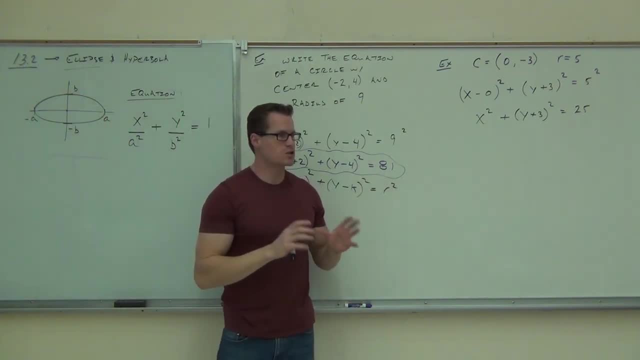 What shape would you have? A circle? Yeah, a circle. So ellipses and circles are different. only by having these different numbers here. Okay, if these were the same numbers there, you'd have a circle. Do you get me? 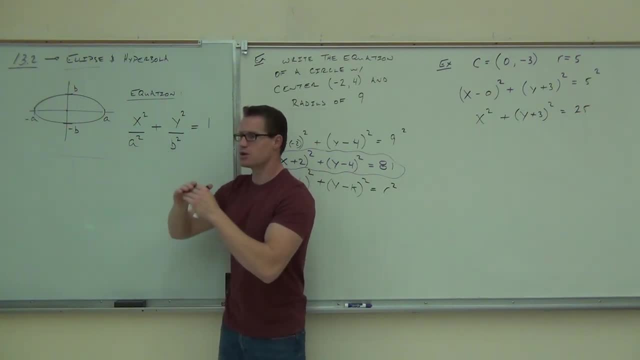 This is the elongation along x. this is the elongation along y. Those things are different than you have an ellipse. If they're the same, then you have a circle. So are ellipses and circles really different Formatically? no, not really. 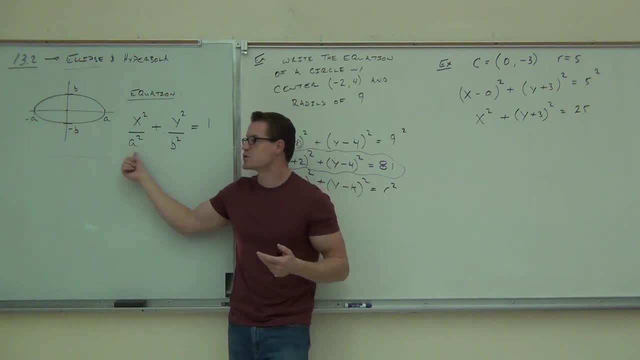 They're the same exact equation, except that these numbers are different for ellipses. Alright, so it's a very similar idea. We typically have this equal to 1 because we want to make sure that we can identify these things. That's why they look a little bit different than the circle equations do. 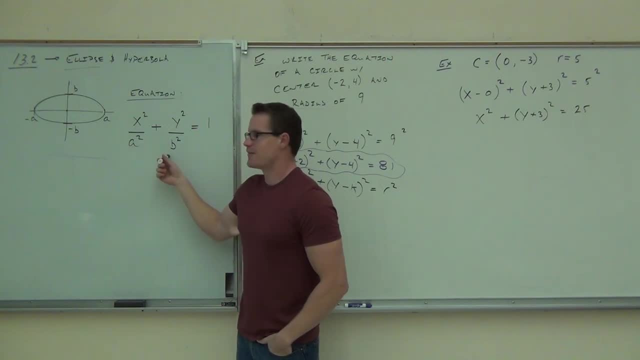 In order to be an ellipse, these things have to be different. I'm going to prove this to you on the formula right now. Okay, look at the numbers a and the numbers b. Notice how a is given by the number that's associated with x. Are you with me on that? And b is given by the number that's associated with y. Okay, we got that. 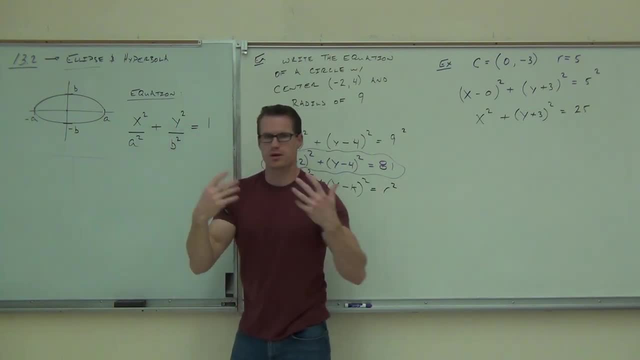 What would happen if these were the... Look at the board, you've got to get this. What would happen if these are the same number? 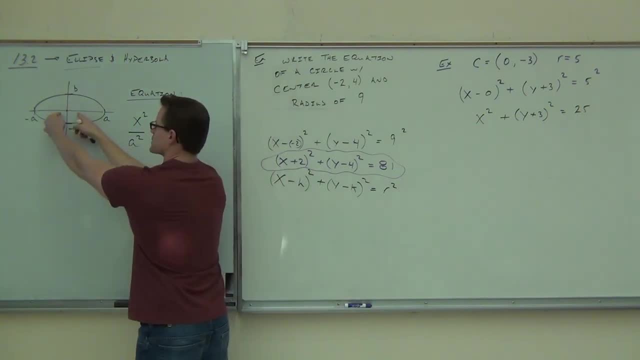 If these were the same number, this would go out the same, and this would go out the same. What shape would you have? A circle. 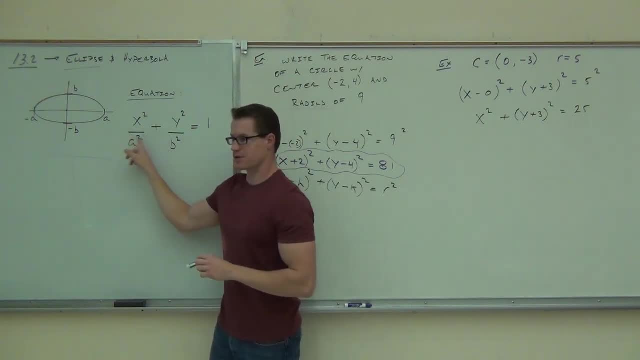 So, ellipses and circles are different only by having these different numbers here. Okay, if these were the same numbers there, you'd have a circle. Do you get me? 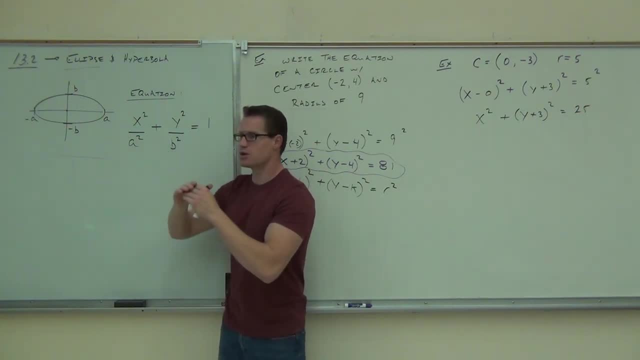 This is the elongation along x, this is the elongation along y. Those things are different than you have an ellipse. If they're the same, then you have a circle. 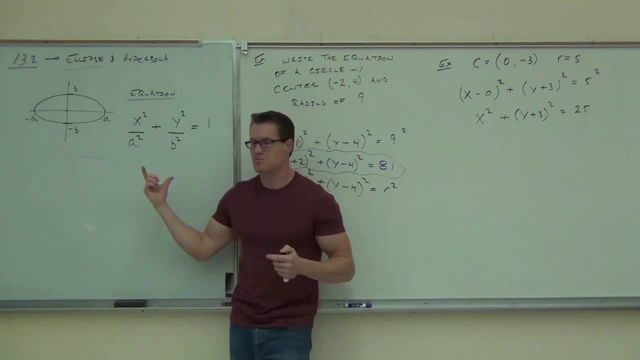 So, are ellipses and circles really different? Formatically, no, not really. They're the same exact equation, except that these numbers are different for ellipses. 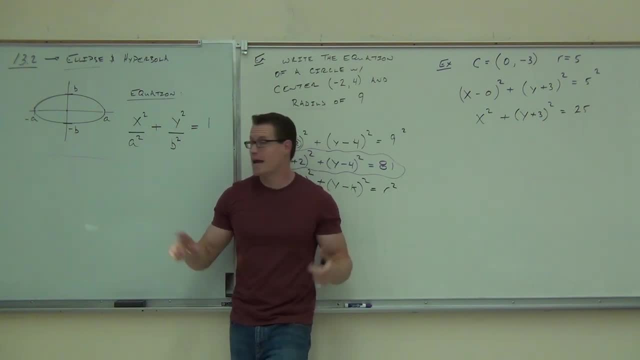 Alright, so it's a very similar idea. We typically have this equal to 1 because we want to make sure that we can identify these things. That's why they look a little bit different than the circle equations do. Other than that, they're very similar. 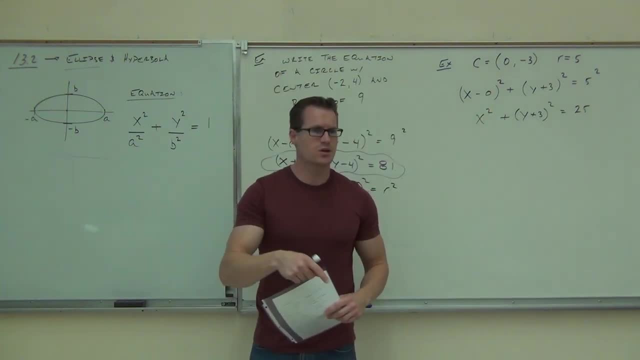 Would you like to give a couple of these a try? Okay, before we do, let me make a couple notes so you're going to be able to refer back to this. 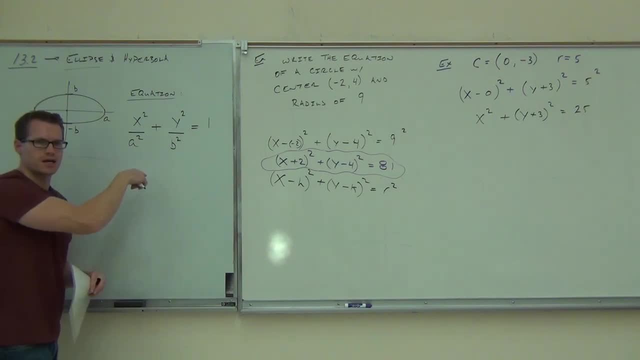 The x-intercepts are given by plus or minus a. How do we know that? Well, it's the number right under x. 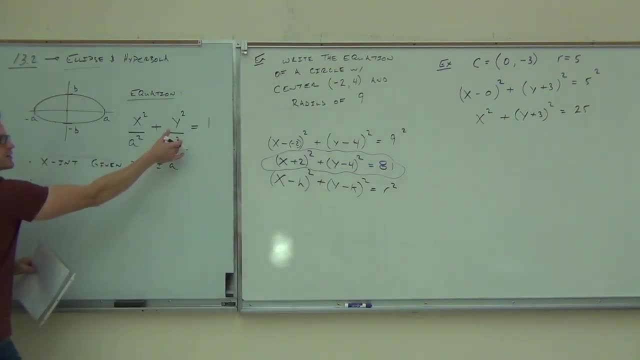 That number under x is associated with our x-intercepts. The number underneath y is associated with our y-intercepts. So, y-intercepts are given by plus or minus a. 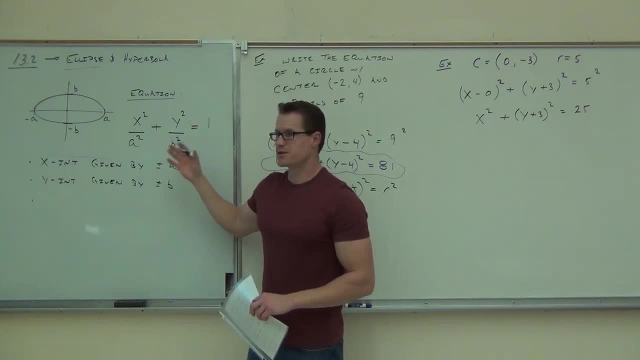 And lastly, this one right here is centered at . You know how I can tell? Is anything being added or subtracted to x? Anything being added or subtracted to y? It's going to have the same exact situation as a circle. 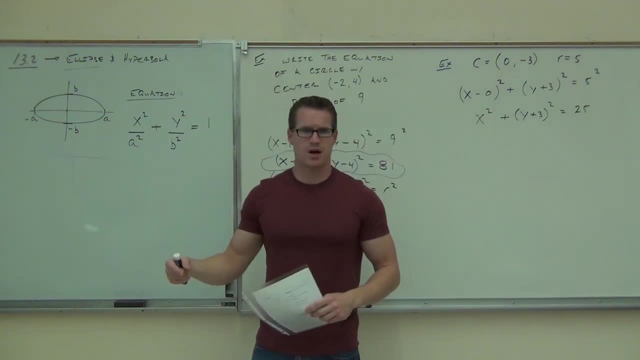 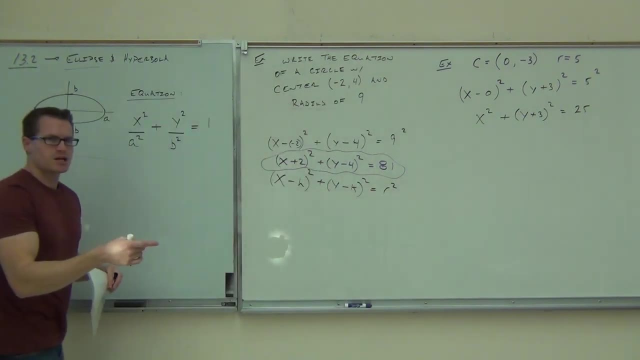 Other than that, they're very similar. Would you like to give a couple of these a try? Okay, before we do, let me make a couple notes so you're going to be able to refer back to this. The x-intercepts are given by plus or minus a. 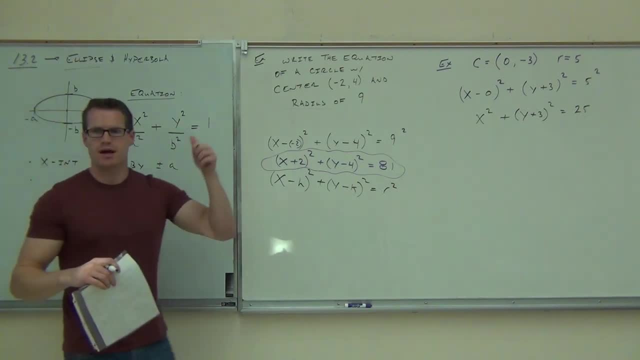 How do we know that? Well, it's the number right under x. That number under x is associated with our x-intercepts. The number underneath y is associated with our y-intercepts. So y-intercepts are given by plus or minus a. 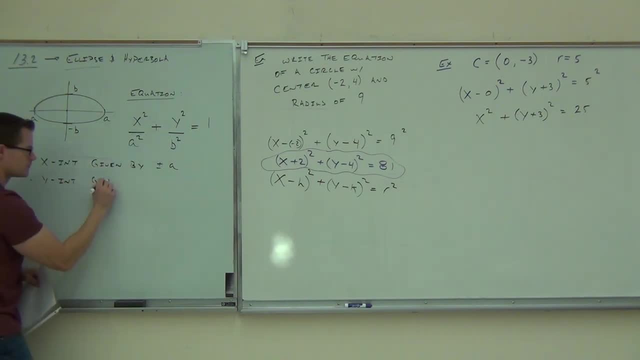 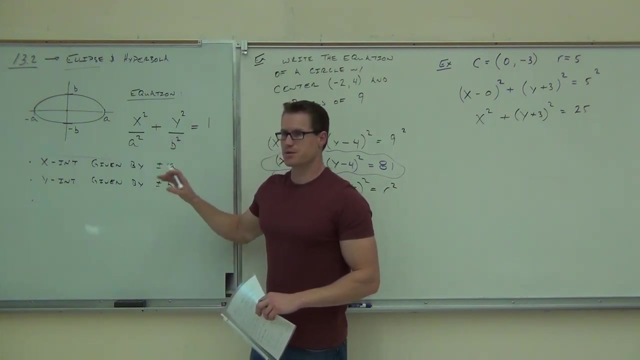 Plus or minus b And lastly, this one right here is centered at- You know how I can tell- Is anything being added or subtracted to x? Anything being added or subtracted to y. It's going to have the same exact situation as a circle. 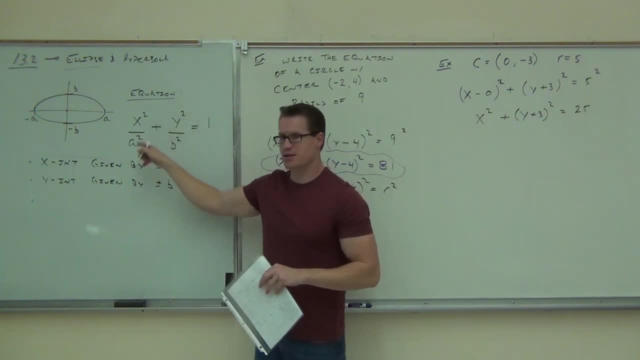 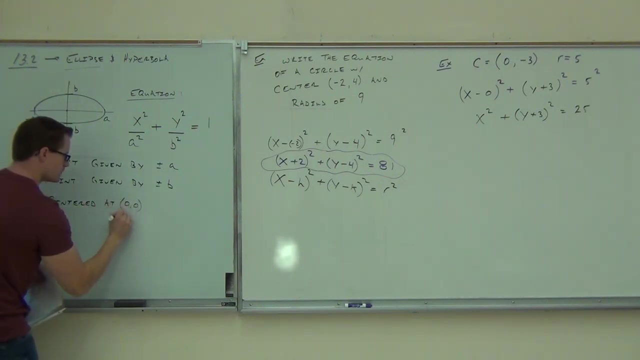 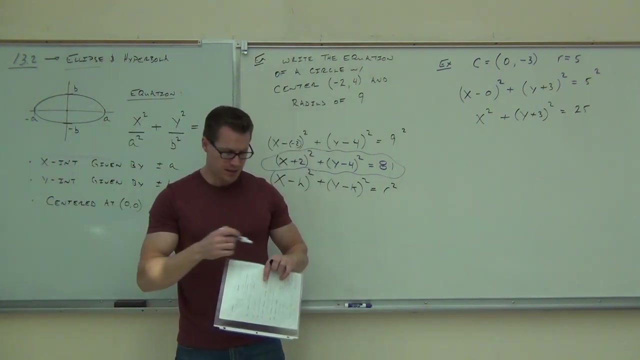 It pretty much is a circle. it's just elongated in one direction. So this thing is centered at: Could we move it around? Could we shift it Exactly the same way as we did before? We're going to try two examples and we'll start here next time with some shifts. 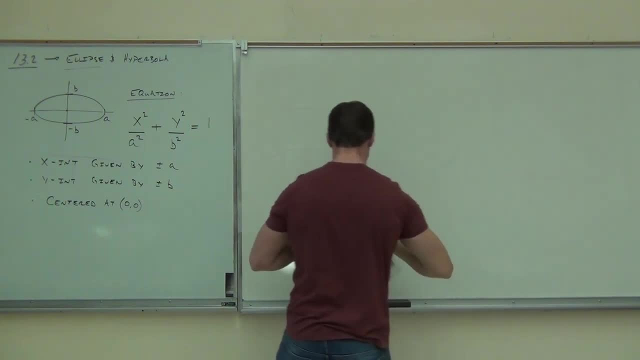 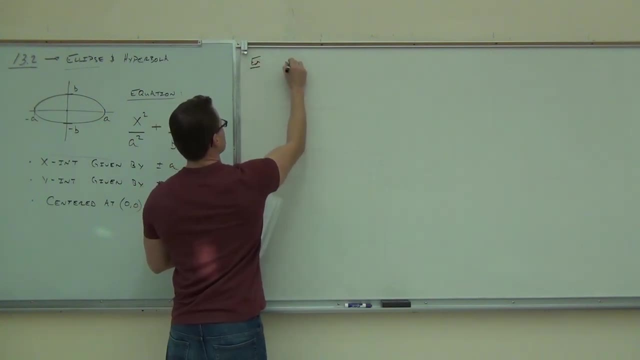 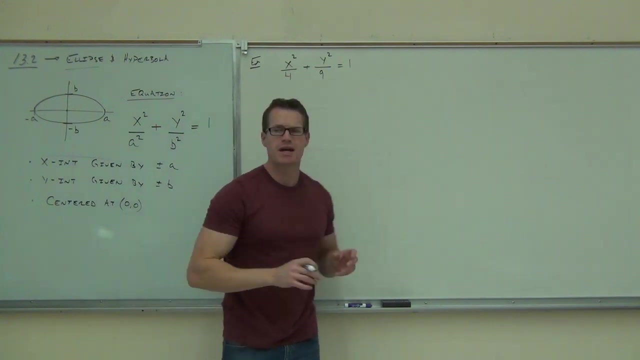 Okay, the first thing you have to be able to do with these formulas of these equations, is be able to determine whether they're parabolas, whether they're parabolas, whether they're circles, whether they're ellipses or hyperbolas. 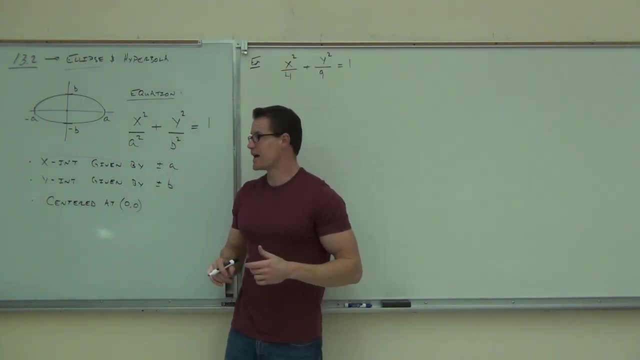 First thing: is this thing a parabola? No, Parabolas won't have a y squared. Is this thing a circle? No, It looks really similar, though right, Look at it. I mean, it's got an x squared, it's got a y squared. 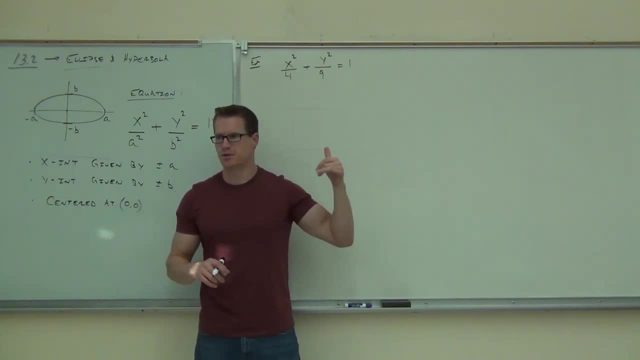 it's got a plus. What makes this thing not a circle? The bottom, The bottom. Why the bottom two? Because they're different. They are different If they had been the same number, look it If they'd been the same. that's a circle, right there. 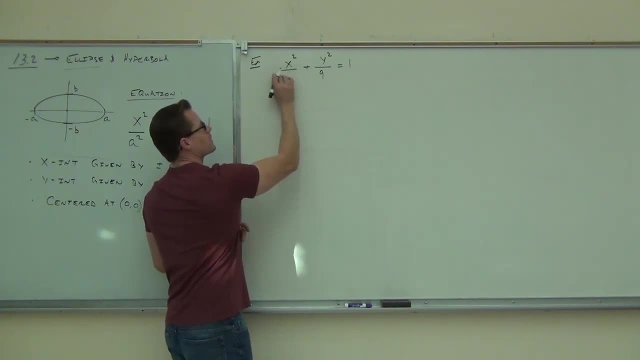 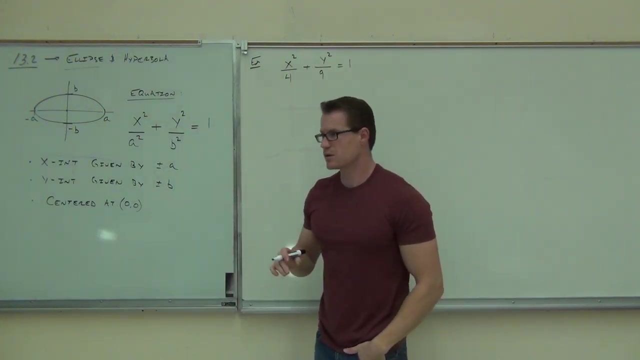 That's definitely a circle. Why can we see this? Well, let's go ahead. let's look at our x and our y intercepts. This is definitely an ellipse. Can you tell me where the center is gonna be on this? Zero, zero. 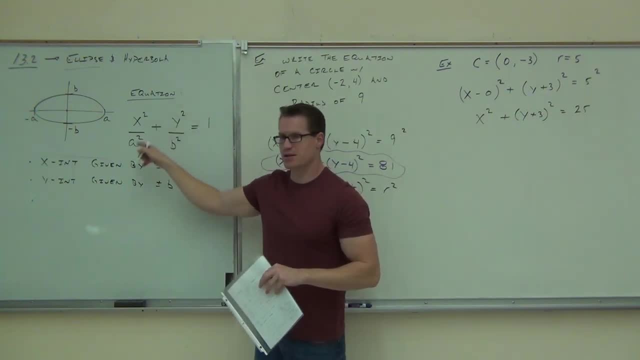 It pretty much is a circle, it's just elongated in one direction. So, this thing is centered at . Could we move it around? Could we shift it? Exactly the same way as we did before. 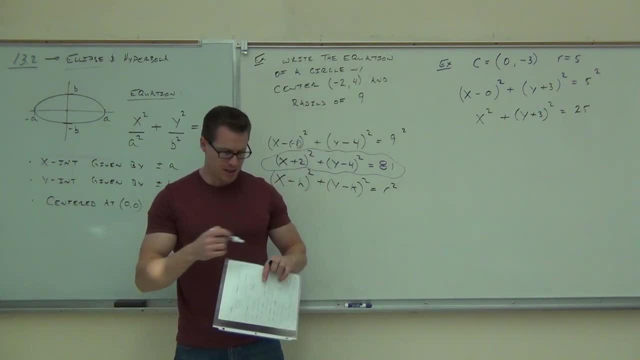 We're going to try two examples and we'll start here next time with some shifts. 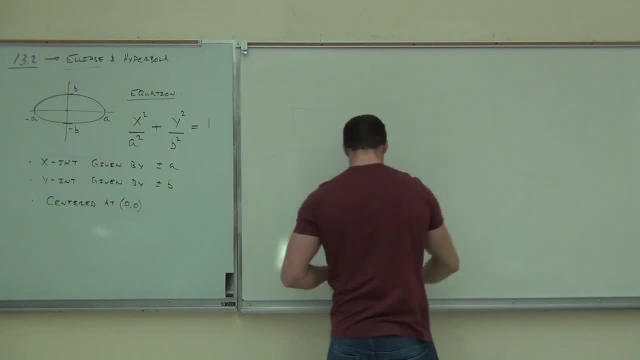 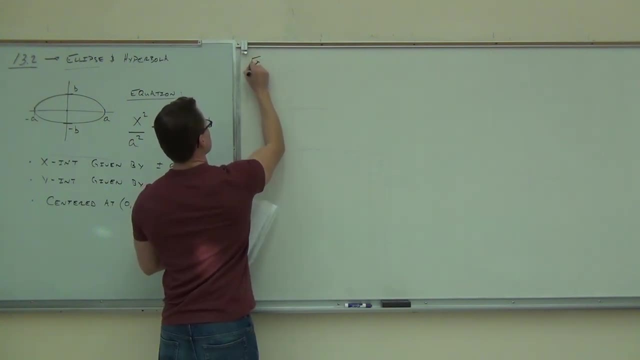 Okay, the first thing you have to be able to do with these formulas, with these equations, is be able to determine whether they're parabolas, whether they're circles, whether they're ellipses, or hyperbolas. First thing, is this thing a parabola? No. Parabolas won't have a y-squared. Is this thing a circle? No. It looks really similar though, right? Look at it. I mean, it's got an x-squared, it's got a y-squared, it's got a plus. 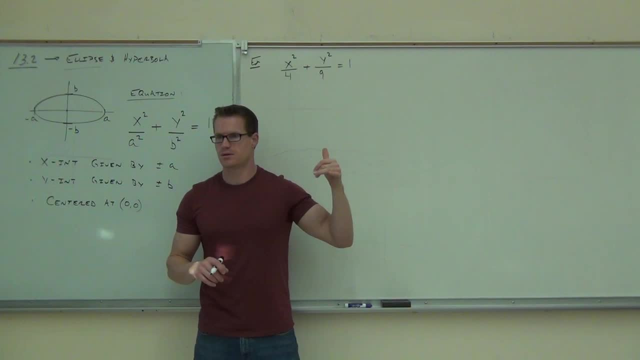 What makes this thing not a circle? The bottom. The bottom. Why the bottom two? Because they're different. They are different. 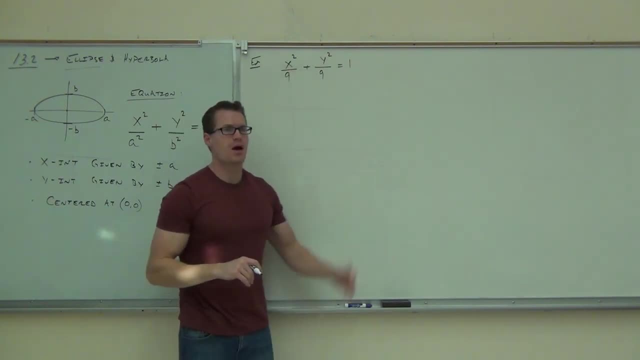 If they had been the same number, look at it. If they had been the same, that's a circle right there. That's definitely a circle. Why can we see this? 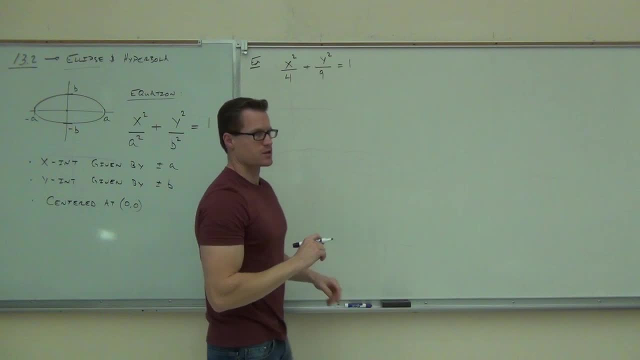 Well, let's go ahead and let's look at our x and our y-intercepts. 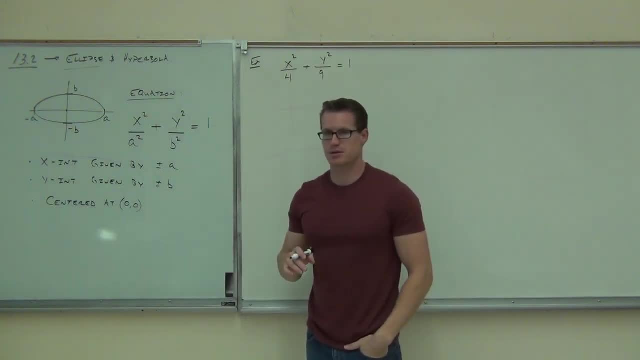 This is definitely an ellipse. Can you tell me where the center is going to be on this? Zero, zero. Good. Zero, zero is not being shifted at all. There's nothing being added or subtracted to the x and the y. There's no parentheses there. 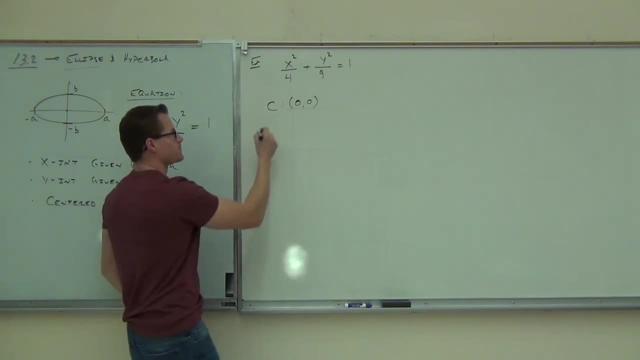 We're going to find our x-coordinates, our x-intercepts, and our y-intercepts. What are they? 4, 16, or 2? What do you think? 4, 16. It's very much like the radians, isn't it? Look at that. That's a squared, right? 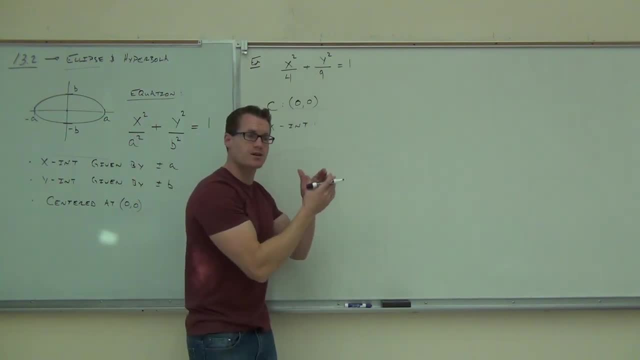 That's a squared. So if we're treating this as a squared, then our x-intercepts are a, or the square root of whatever number you have here. 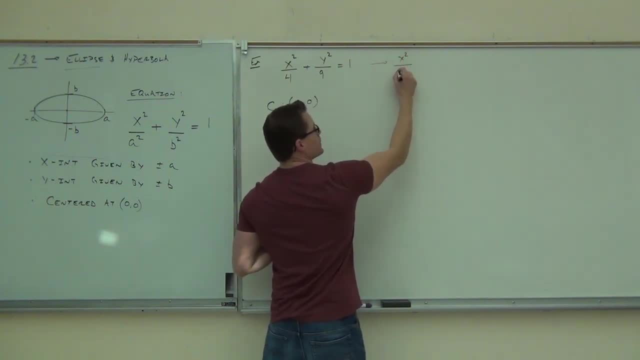 Notice that you could write this x squared over 2 squared. True? Yeah. So y squared over 3 squared equals 1. 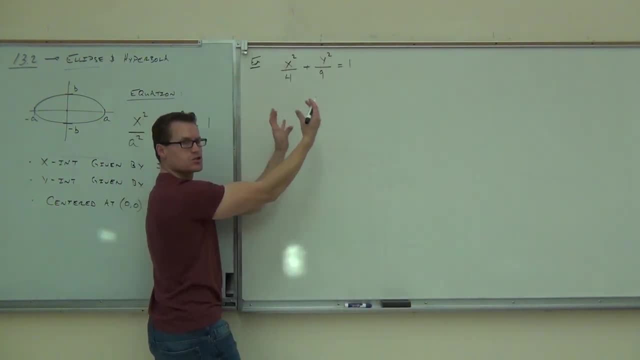 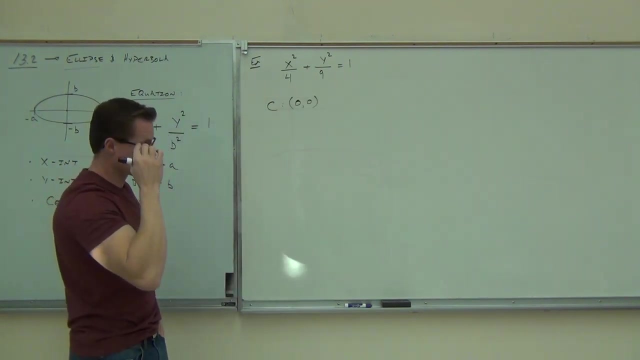 Good, zero, zero's not being shifted at all. There's nothing being added or subtracted to the x and the y. There's no parentheses there, So our center is at zero, zero. We're gonna find our x coordinates, our x intercepts. 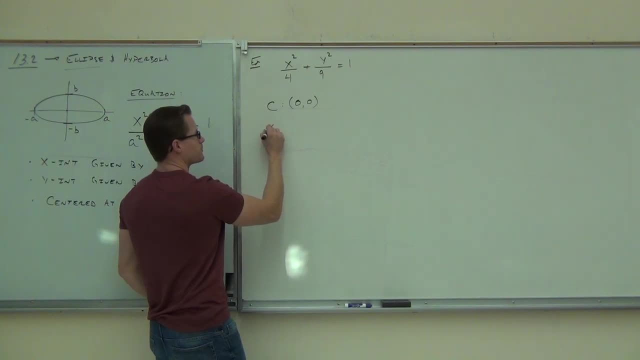 and our y intercepts. What are they? four of 16 or two? what do you think? Four of 16, it's very much like the radians, isn't it? Look at that, that's a squared right. That's a squared. 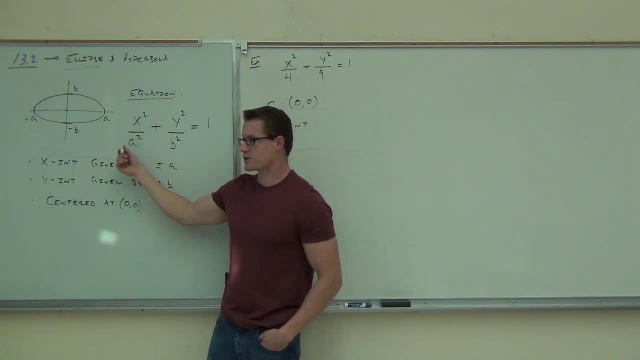 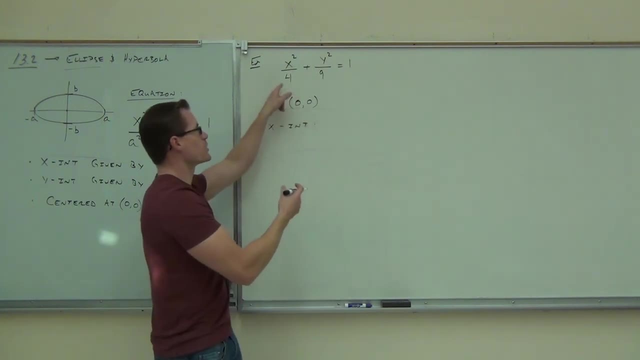 So if we're treating this as a squared, then our x intercepts are a or the square root of whatever number you have here. Notice that you could write this: x squared over two squared, True, Mm-hmm Yeah. 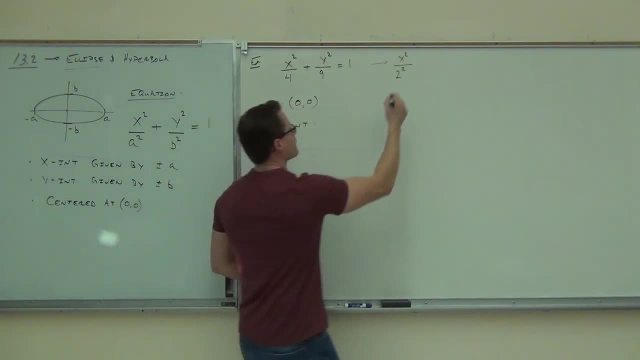 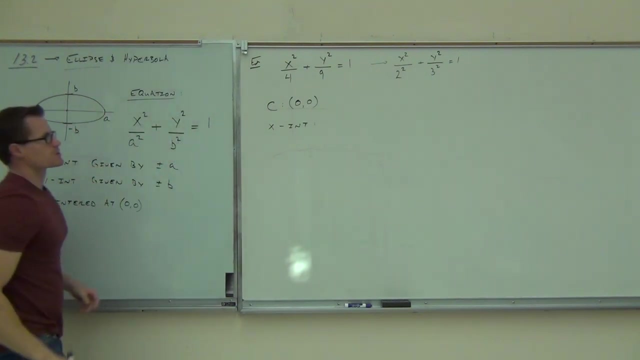 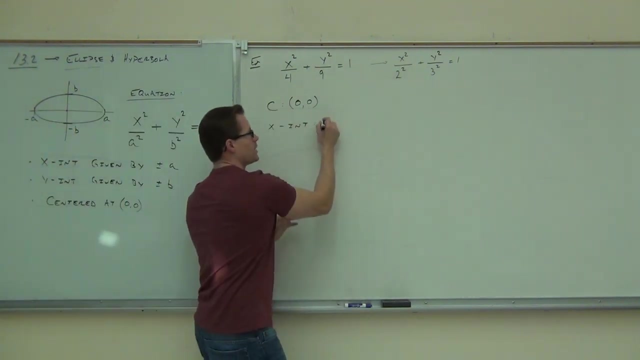 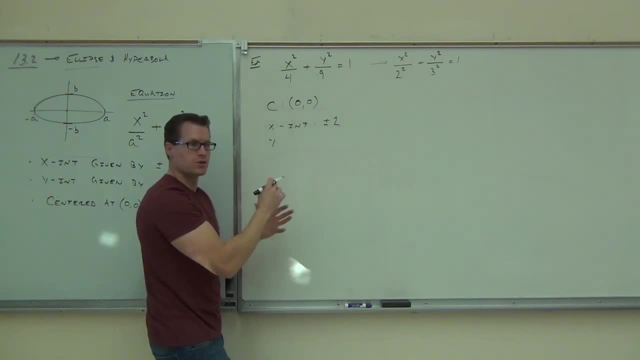 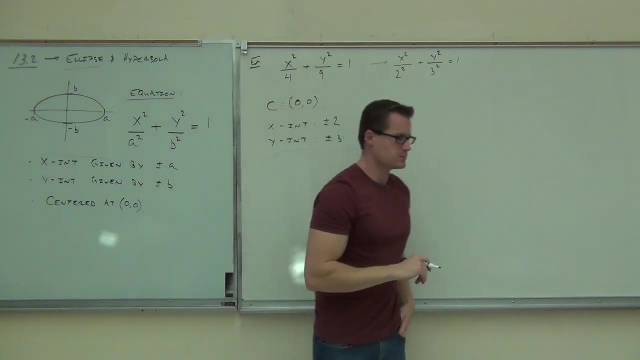 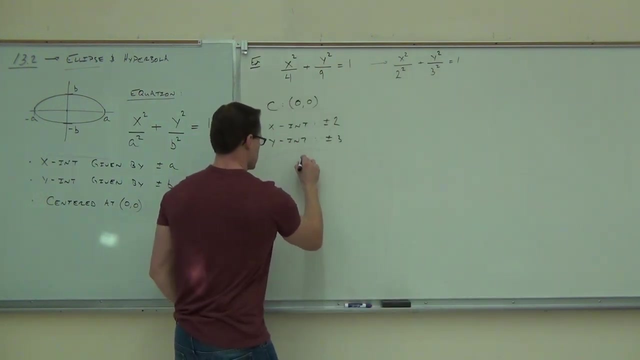 And the three squared says: well, three is your plus or minus, three is your y. intercepts You still so far, so good on this? Yeah, Can you graph it? Yeah, Yeah, let's try it, Just like a circle. you're going to start with the center. 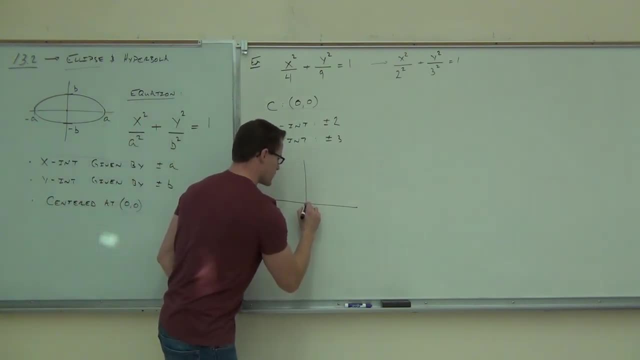 Where's the center? at Zero zero, zero one. So we're right there at the center. Now I know I used the words x intercepts and y intercepts, so please watch it for a second. If your center is not at zero zero, then what this means. 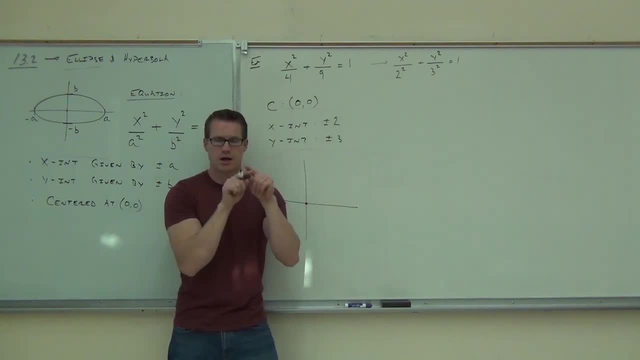 is you go two on the x direction and three on the y direction. no matter where you're at, Where are your centers at? In this particular case, since we're centered at zero, zero, it's going to be our x intercepts and our y intercepts. 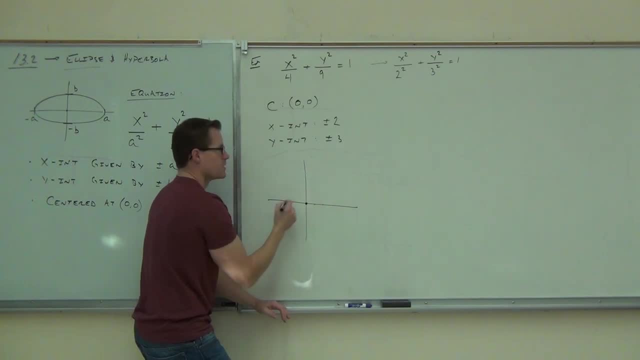 Because it says: you're going to go to the right two spots, You're going to go to the left two spots. You OK with the left and the right. there It's the number that's associated with the x. You take the square root of that. 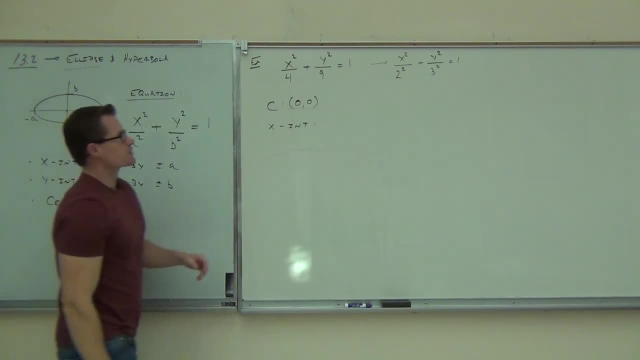 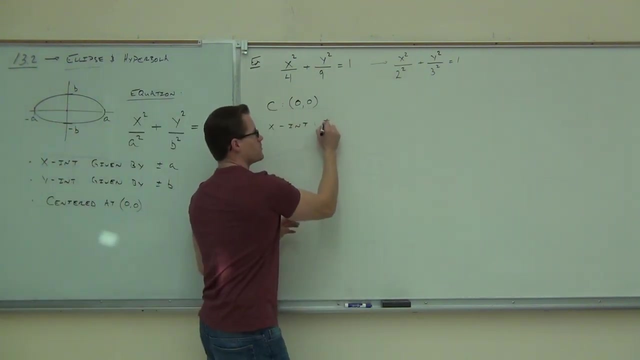 That fits the formula of our ellipse. So if a squared says that a is our x-intercepts, 2 squared says that plus or minus 2 is our x-intercepts. And the 3 squared says, well, plus or minus 3 is your y-intercepts. Are you still so far so good on this? Can you graph it? Yeah. 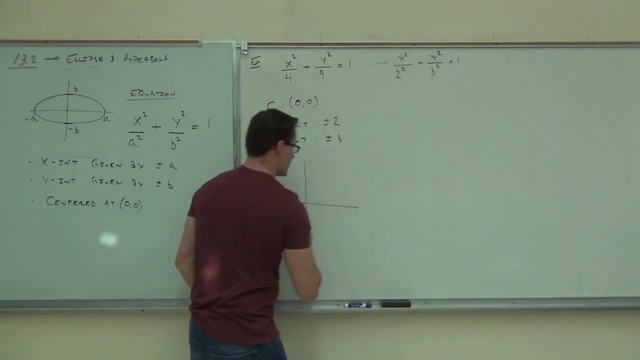 Yeah, let's try it. Just like a circle, you're going to start with the center. Where's the center at? 0, 0, 0, 1. So we're right there at the center. 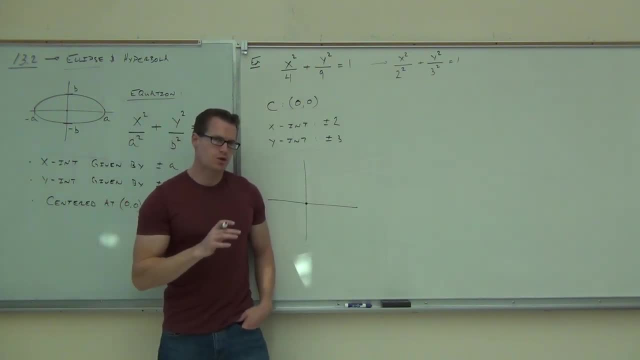 Now, I know I used the words x-intercepts and y-intercepts, so please watch it for a second. 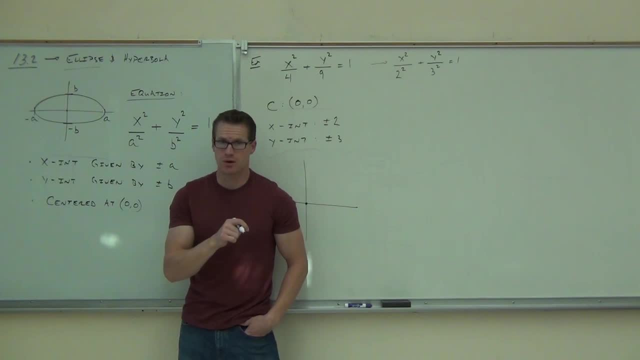 If your center is not at 0, 0, then what this means is you go 2 on the x-direction and 3 on the y-direction, no matter where your center's at. Okay? 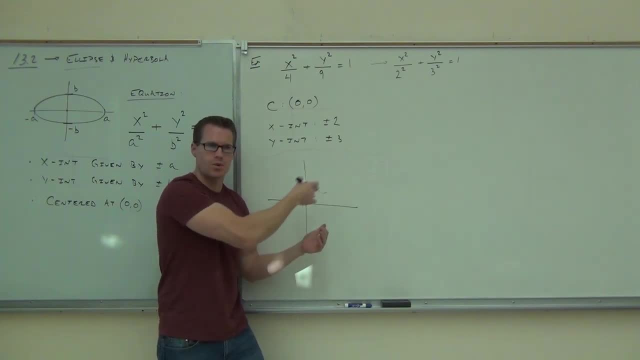 So in this particular case, since we're centered at 0, 0, yeah, it's going to be our x-intercepts and our y-intercepts. Because it says you're going to go to the right 2 spots. You're going to go to the left 2 spots. You okay with the left and the right there? It's the number that's associated with the x. 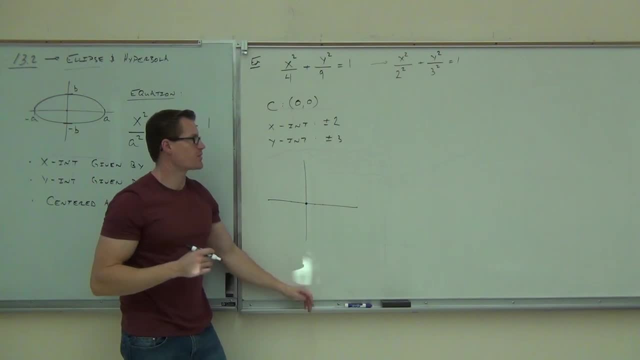 You take the square root of that. It's telling you how far to go along the x. How about the y? How far are we going to go? 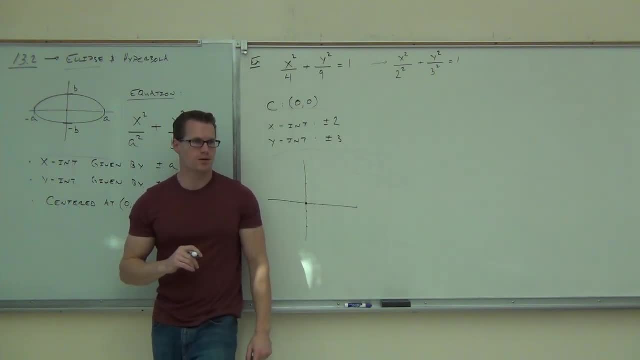 By the way, let me ask you this question right now. Could you immediately tell, just by looking at the equation, which direction the ellipse is going to be stretched out on? 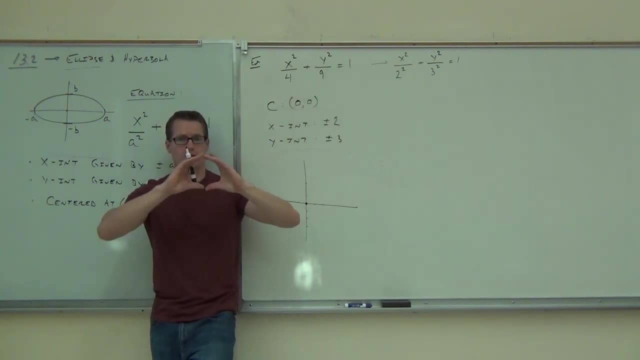 What's that tell you? Which direction is it going to be stretched out more? Is it going to be along the x or along the y? That number's bigger. 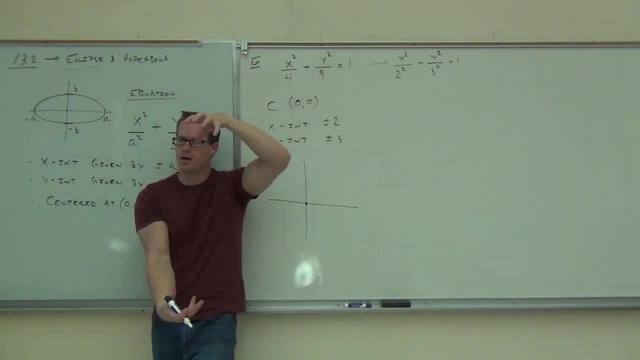 That means you're stretching out along that particular axis more and more. So that's another way to say if those numbers were the same, you'd be stretching out the same exact way, right? It'd be a circle. So here we're saying, oh, we're stretching out more along the y-axis. It's going to be one of these tall ellipses. Not one of those long ellipses. So since we have our spots here, here, here, and here, we can make our ellipse. 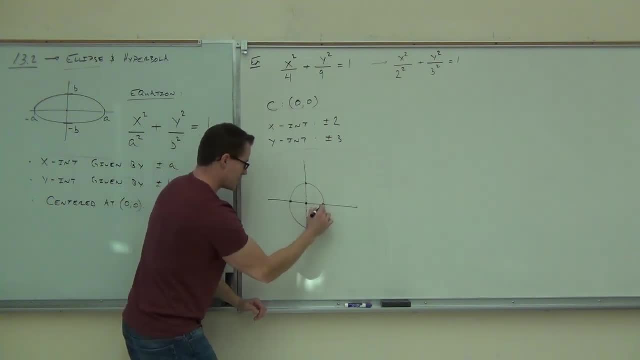 We can try to make our ellipse. That looks horrible. 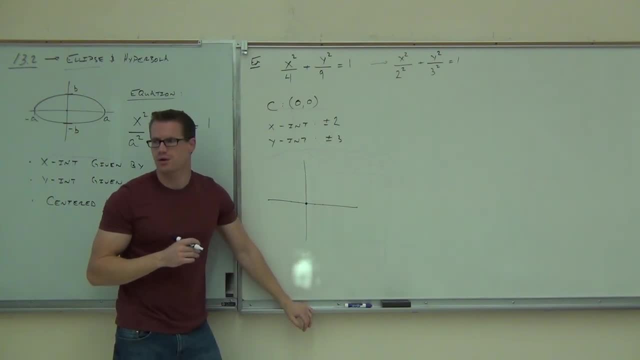 It's telling you how far to go along the x. How about the y? How far are we going to go? By the way, Let me ask you this question right now: Could you immediately tell, just by looking at the equation, which direction the ellipse is going to be stretched out on? 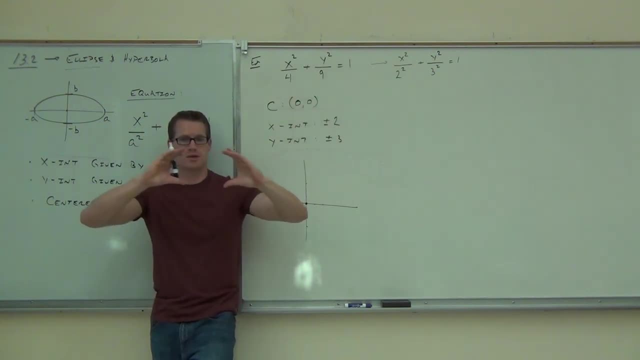 What's that? tell you Which direction is it going to be stretched out more? Is it going to be along the x or along the y? That number's bigger. That means you're stretching out along that particular axis more and more. So that's another way to say if those numbers were the same. 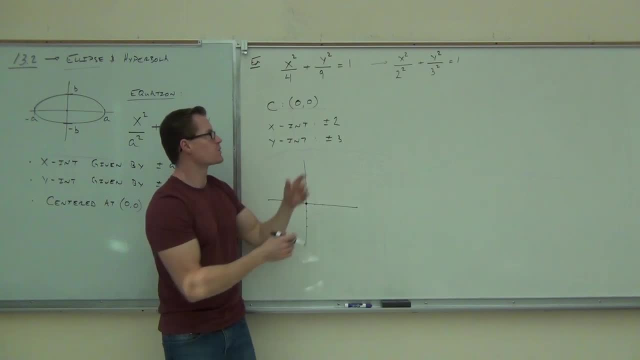 you'd be stretching out the same exact way, right, It'd be a circle. So here we're saying, oh, we're stretching out more along the y or along the y axis to find where the y axis is going to be. I would have to say: just imagine all this is going to be. 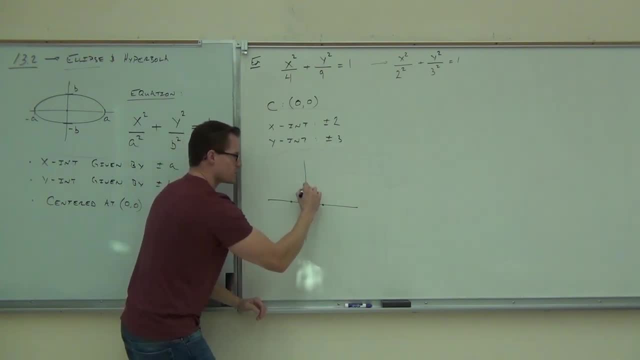 in one of these longer ellipses, and that's going to be in one of these tall ellipses, not one of those long ellipses. So, since we have our spots here, here, here and here, we can make our ellipse. 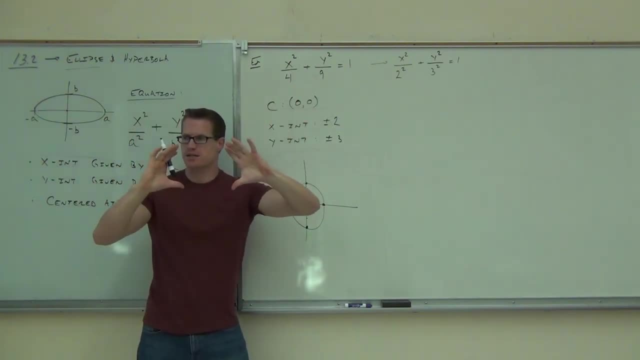 We can try to make our ellipse. That looks horrible, But that's the idea. We're taking our equation, we're finding the spread on the x axis or in the x direction. if we're not centered at the origin, the spread along the y axis. 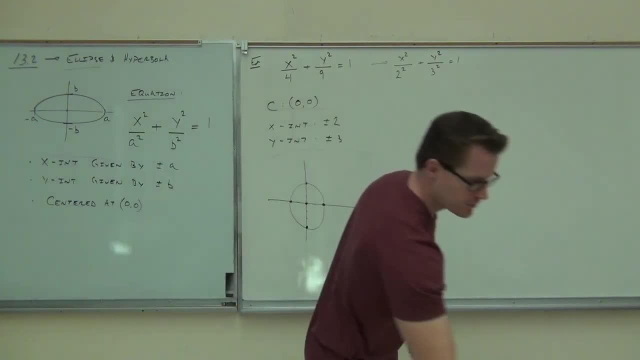 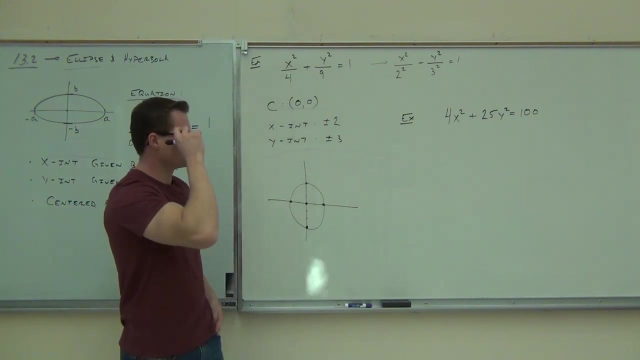 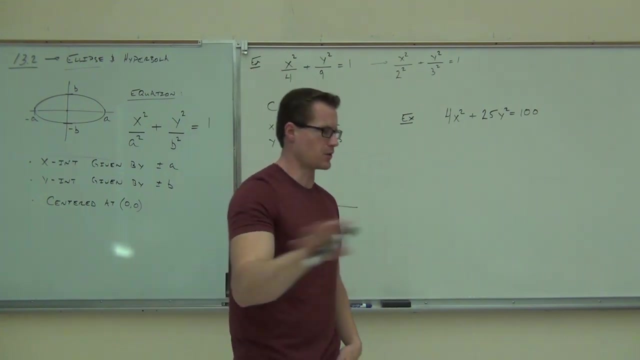 And whatever our center is All, right, center is Okay. our last example for today: Now, that looks a little weird. That looks a little weird. Let's go through the process. Let's identify what type of shape this is. Firstly, is it a parabola? That looks nothing like a parabola. Is it a circle? Is it a circle? 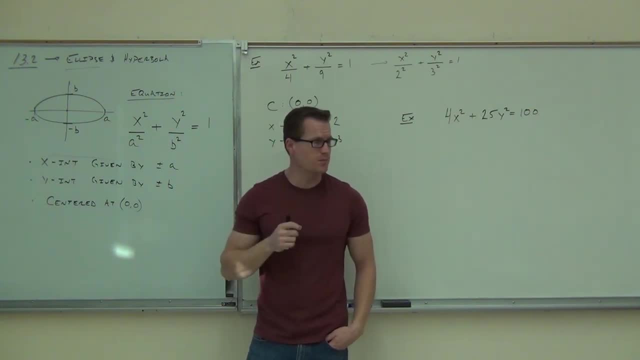 It's got a square, doesn't it? In both the x and the y. it's got a plus in the middle. However, are the numbers the same? If the numbers were the same, you'd have a circle, But I want you to see this. What defines an ellipse for us, what makes things easy, is: 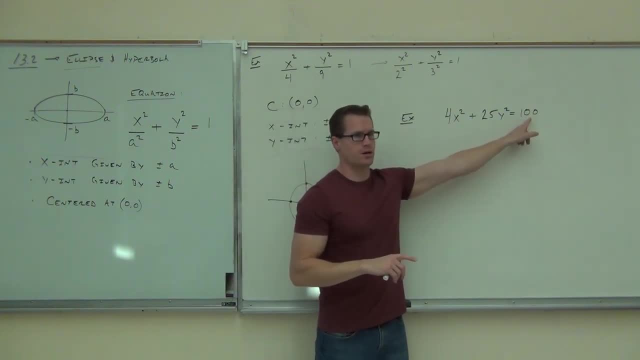 that we have a 1 over here. Can you make that into a 1?? Yes, And I don't mean subtract 99.. We don't want to do that. How do you make that into a 1?? If you do that, divide by what? 100. 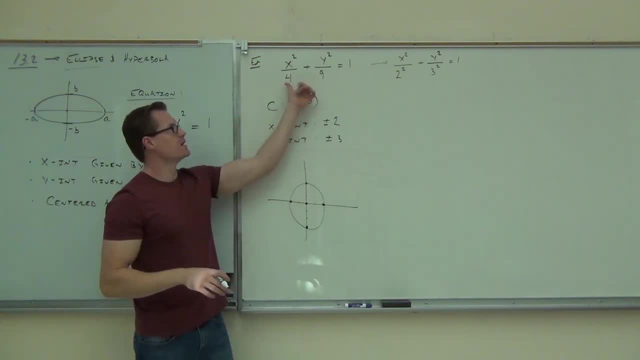 But that's the idea. We're taking our equation. We're finding the spread on the x-axis or in the x-direction if we're not centered at the origin. 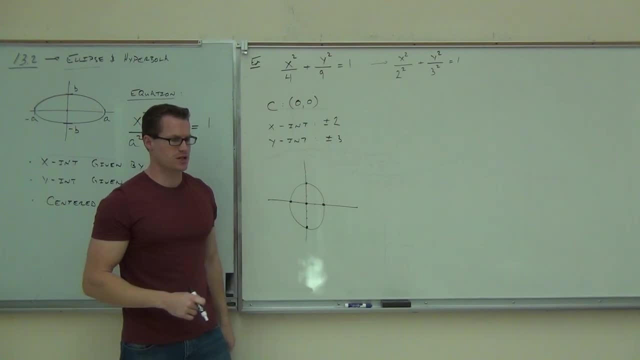 The spread along the y-axis. And whatever our center is. Okay, our last example for today. 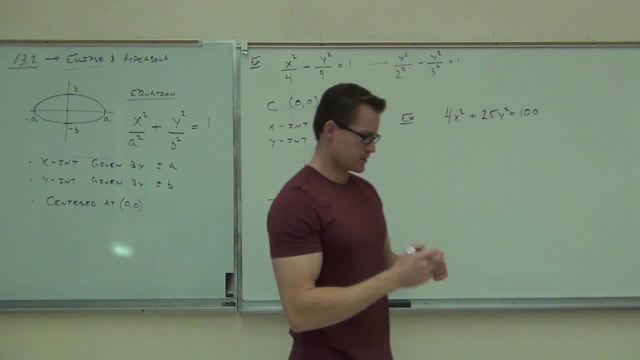 Now that looks a little weird. That looks a little weird. Well, let's go through the process. Let's identify what type of shape this is. 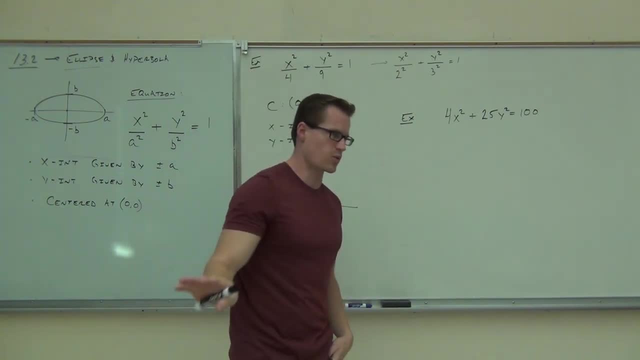 Firstly, is it a parabola? No. That looks nothing like a parabola. Is it a circle? Yes. Is it a circle? No. It's got a square, doesn't it? In both the x and the y. It's got a plus in the middle. However, are the numbers the same? No. If the numbers were the same, you'd have a circle. 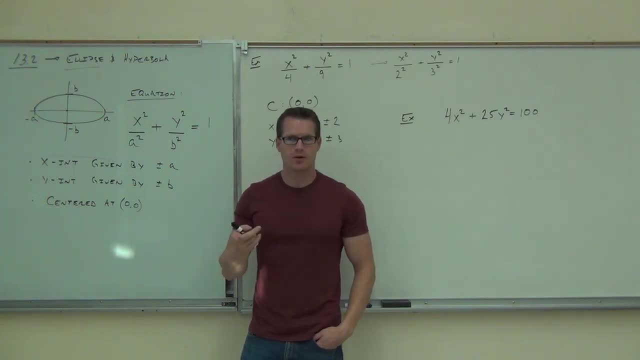 But I want you to see this. What defines an ellipse for us, what makes things easy is that we have a one over here. Can you make that into a one? Yes. And I don't mean subtract 99. 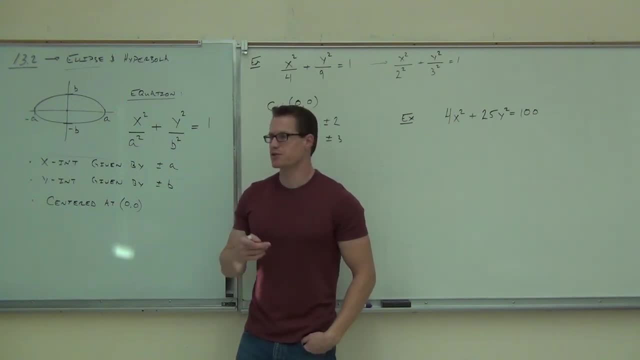 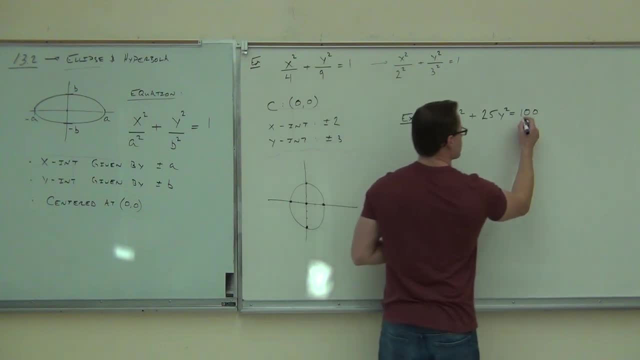 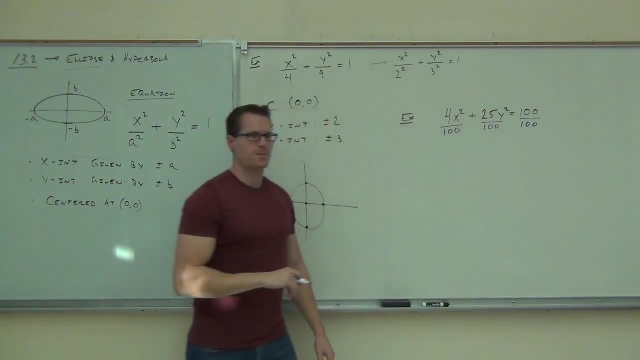 How do you make 100 into 1?? You divide by 100. So we're going to divide by 100. But that means I've got to do it here and I've got to do it there. Can you simplify those fractions? 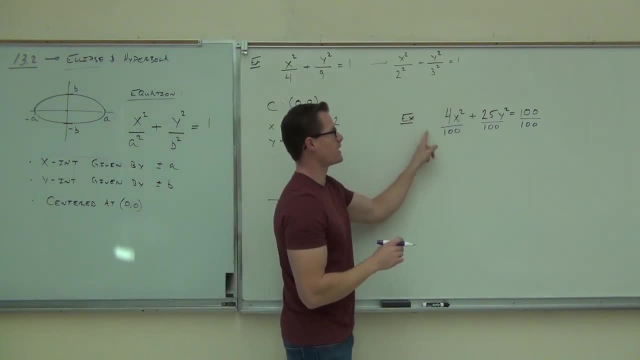 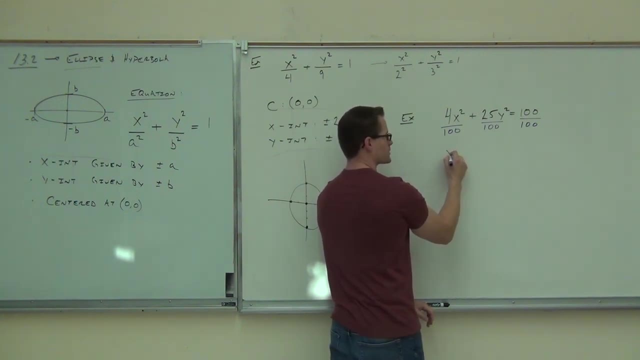 Uh-huh. Okay, tell me everybody what does this fraction simplify, as please? 250.. How much 250.. 1 over 25.. Okay, so I'm sitting on x squared, That's going to be 25.. Remember, 4 over 100, that's. 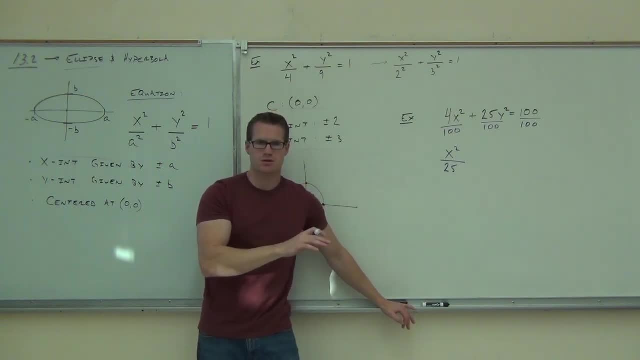 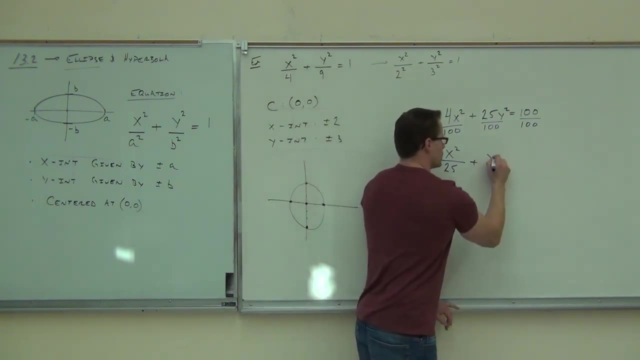 1 over 25.. Are you okay on simplifying that fraction? Okay, plus what's 25y squared over 100? Tell me what that is, please. 1 fourth Good, Of course you mean y squared over 4.. Equals how much? 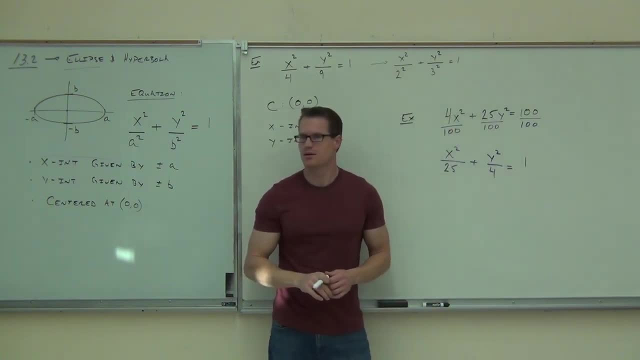 1. Does that look a little bit better? Yeah, Can you identify? look at the board. can you identify that if those numbers were exactly the same when I divided by 100, I'd get exactly the same numbers here and I would have. 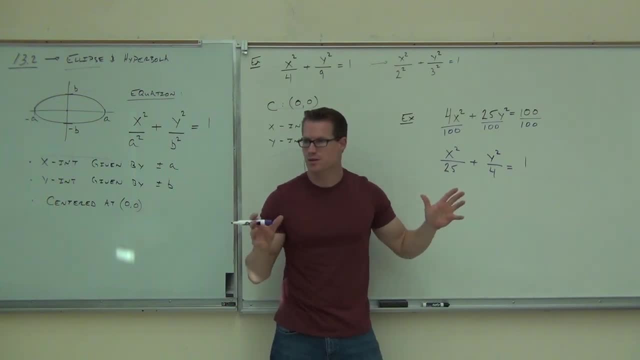 a circle. So how can you immediately tell whether something's an ellipse or a circle? They both have squares, they both have pluses, but the numbers are the same for circles and they're different for ellipses. How many people feel okay with that idea? All right, 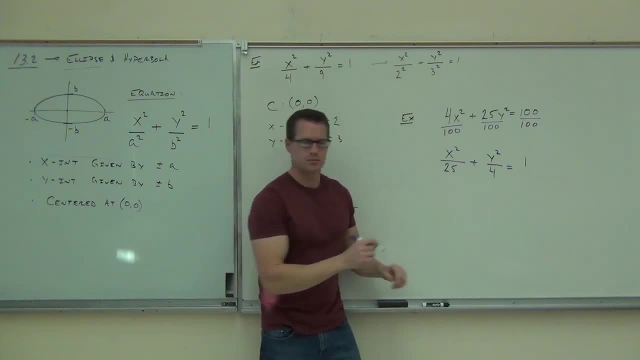 Would you be able to tell me the center Zero? Yeah, there's nothing being added or subtracted. we have to shift it. Would you be able to tell me the distance we're going along, the x direction? how much Plus or minus 5.. 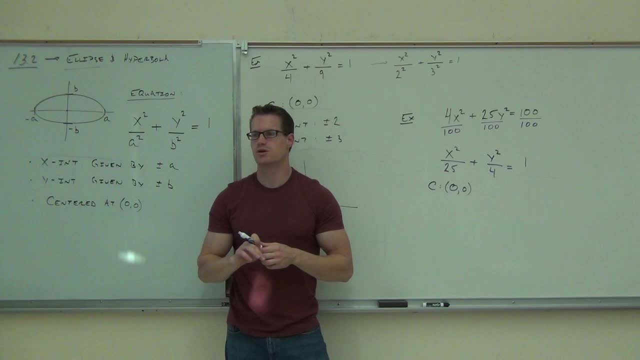 Not 25?? No, because you're doing squares. Ah, so along the x direction we're going plus or minus 5.. How much someone on the right hand side along the y direction? 2. 2, good, plus or minus 2.. Now is this going to be an ellipse spread this way along the 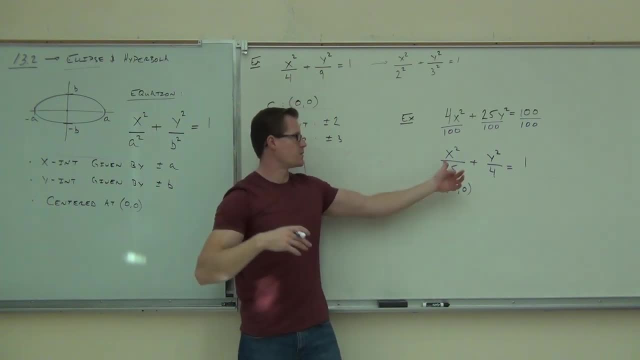 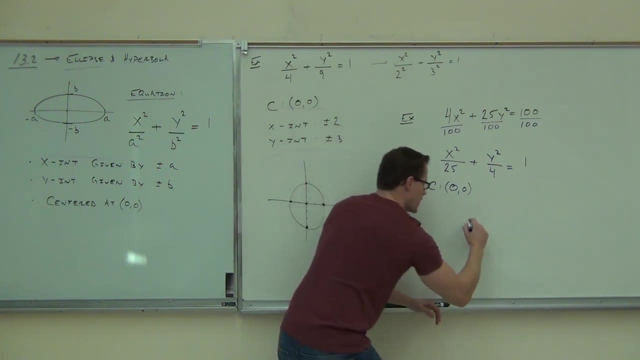 x or this way: along the y, Along the x, That number's bigger. that means we're spreading out more along the x and along the y, So the x direction. I'm not even going to draw the x intercepts, I'm just going to put 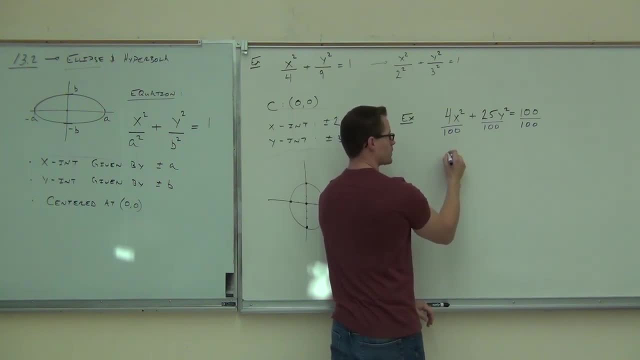 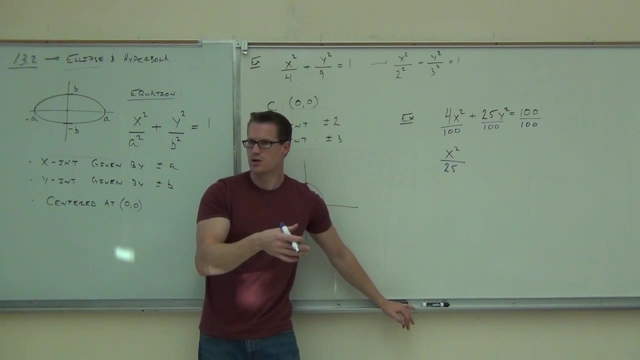 Okay, so I'm sitting on x squared, that's going to be 25. Number 4 over 100, that's 1 over 25. Are you okay on simplifying that fraction? Okay, plus, what's 25y squared over 100? Tell me what that is, please. One-fourth. 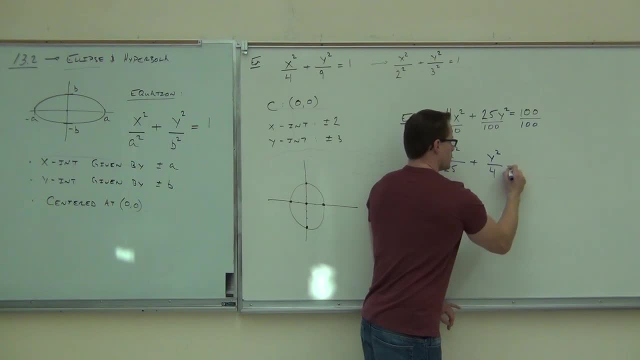 Good. Of course, you mean y squared over 4 equals how much? One-fourth. Does that look a little bit better? Yeah. 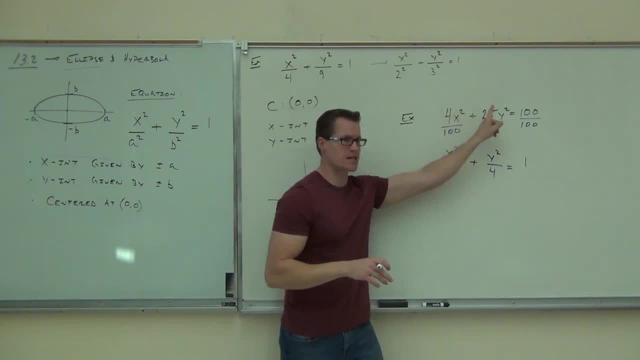 Can you identify, look at the board. Can you identify that if those numbers were exactly the same, when I divide it by 100, I'd get exactly the same numbers here, and I would have a circle? So how can you immediately tell whether something's an ellipse or a circle? They both have squares. 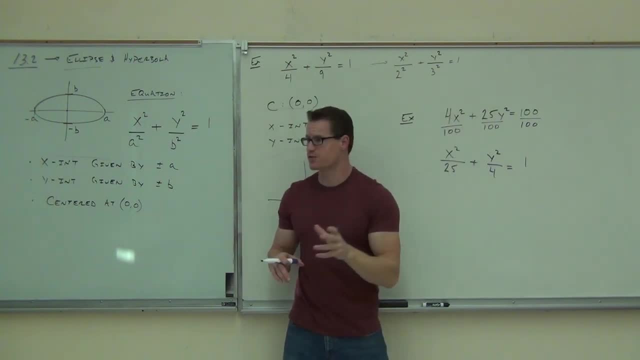 They both have pluses, but the numbers are the same for circles, and they're different for ellipses. I mean, we'll be okay with that idea. All right. 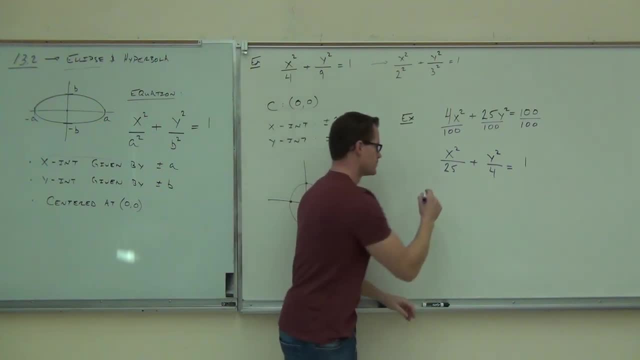 Would you be able to tell me the center? Zero. Yeah, there's nothing being added or subtracted. We haven't shifted this. 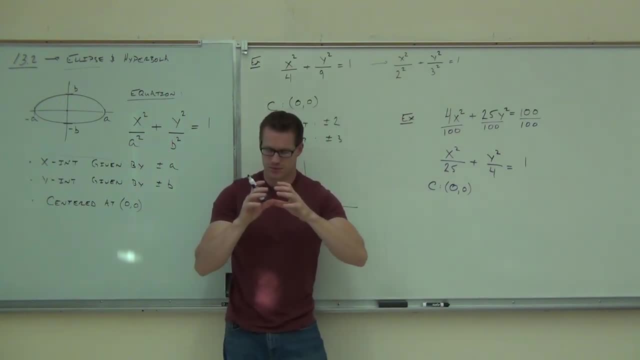 Would you be able to tell me the distance we're going along the x direction? How much? Plus or minus 5. Not 25? No, because you're doing square. Ah, so along the x direction, we're going plus or minus 5. How much, someone on the right-hand side, along the y direction? Two. Two. Good. Plus or minus 2. 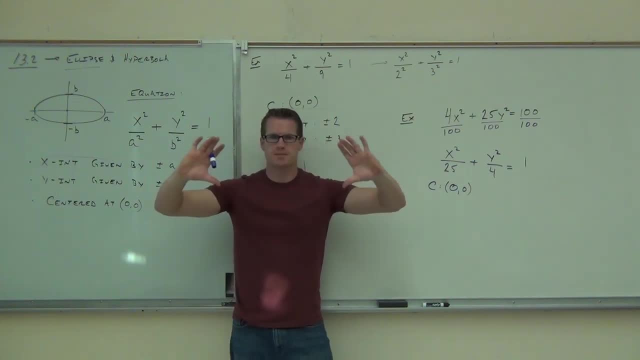 Now, is this going to be an ellipse spread this way, along the x, or this way, along the y? Along the x. That number's bigger. That means we're spreading out more along the x. Along the x and along the y. 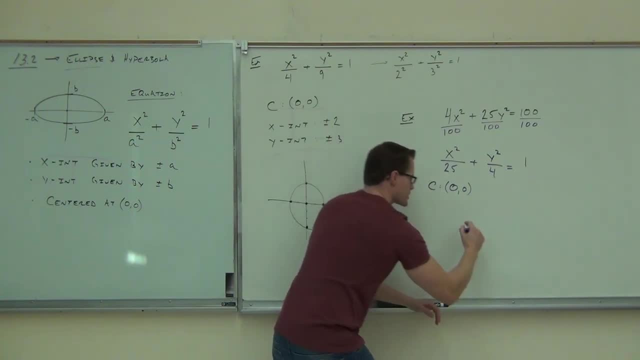 So the x direction, I'm not even going to draw this, the x intercepts. I'm just going to put this on my graph. 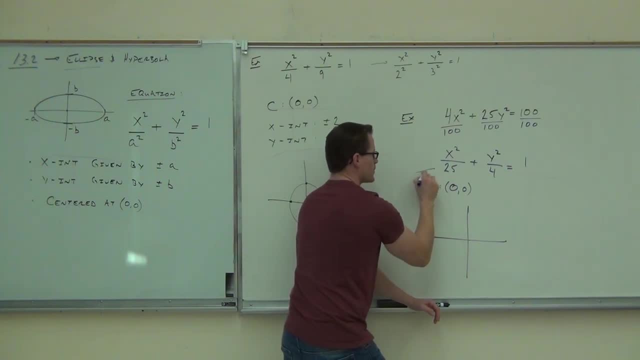 this on my graph. I know that this right here can be written as 5 squared. This right here can be written as 2 squared, Since this is associated with our x. it says: from 0, 0, I'm going to be going plus or minus 5.. That's 5 to the right. that's 5 to the left. That. 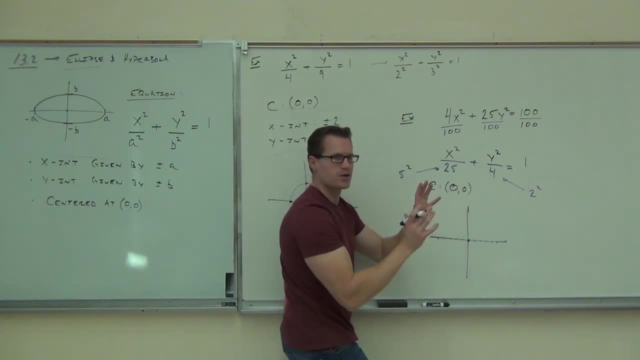 gives us our spread along the x. Since this was a 4, I know that I can write that as 2 squared. That means that we're going to be going plus or minus 2 from the center of our ellipse. That's up 2 and down 2.. 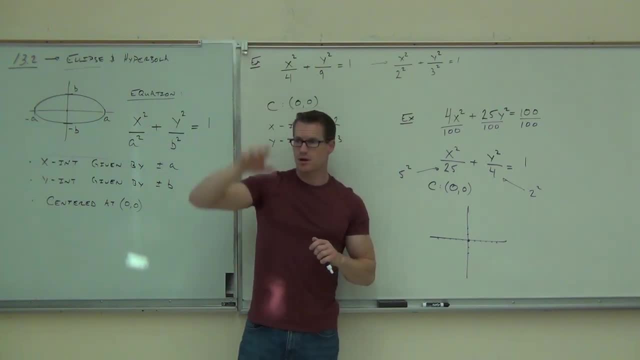 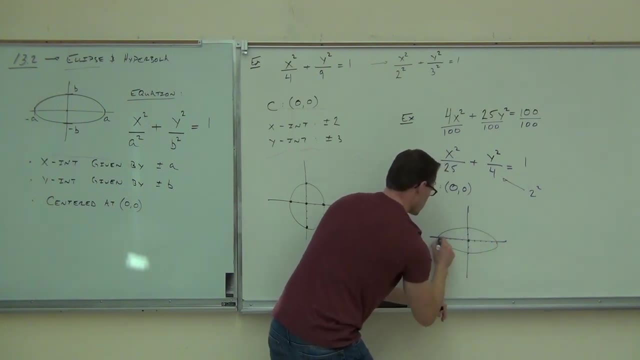 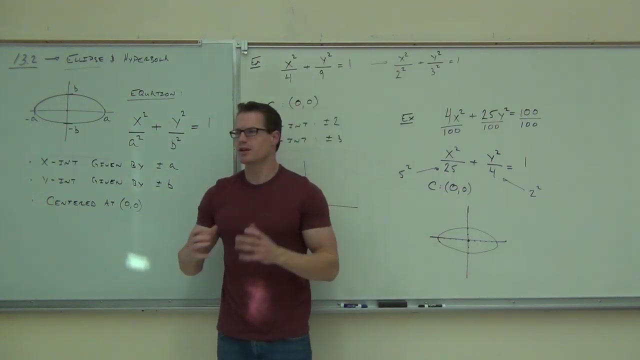 Quick show of hands. how many people feel okay getting that far on these? Now draw your ellipse. Ooh, that's pretty good. So with just a little bit of work, we can actually be very accurate on these shapes. That's all we're going to be able to do on that thing is draw the ellipse along the 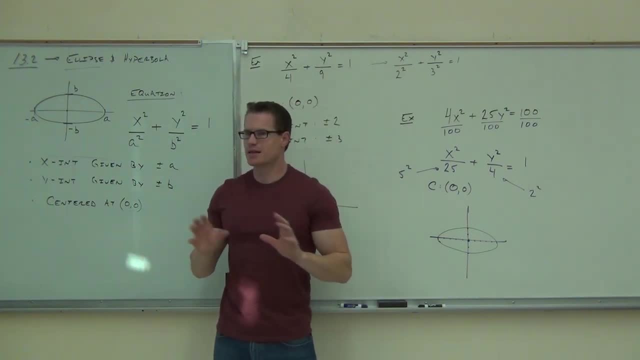 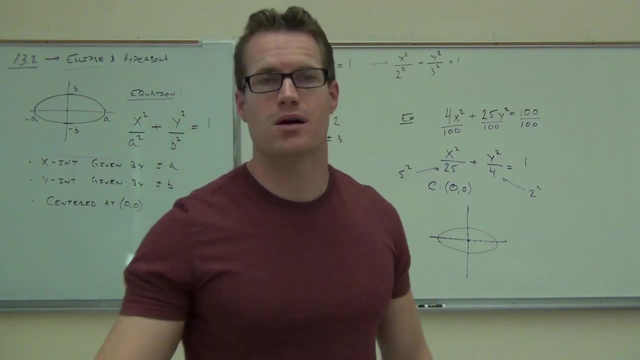 graph like that. Do you feel okay with circles and ellipses? We'll start on one of these examples next time. I'll show you how we can shift it around. talk about hyperbolas. make those things up and that will be our class. 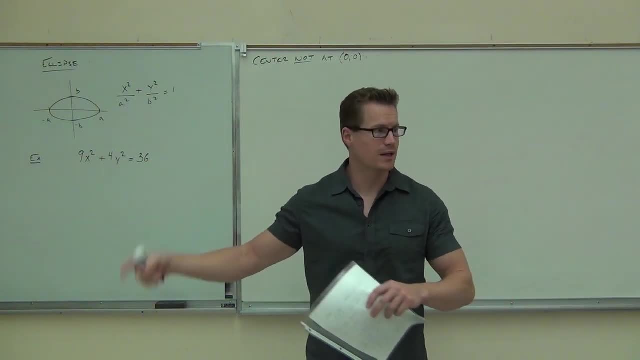 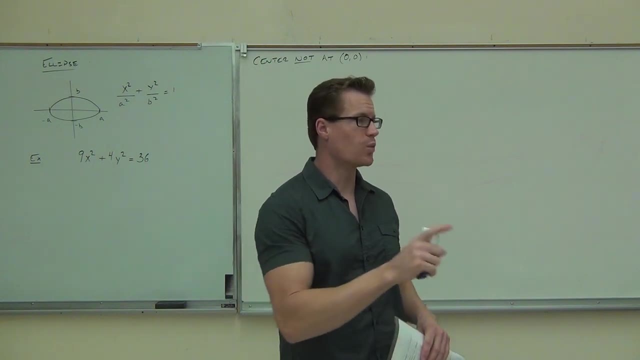 Alright, so we're talking about conic sections again and we have this thing called an ellipse. Yesterday we went over the formula for an ellipse- how to kind of determine whether something is a circle or an ellipse. So we're going to do one more example, talking about 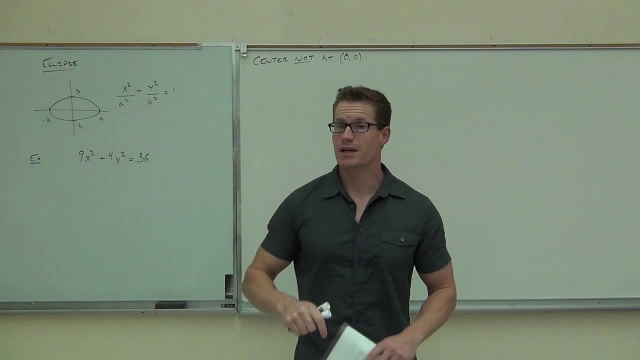 this. Let's look back at this example. Firstly, you need to be able to determine whether or not it's a parabola. You need to be able to determine what type of figure it is. just by looking at the equation, So automatically we can rule out a parabola. We can rule out. 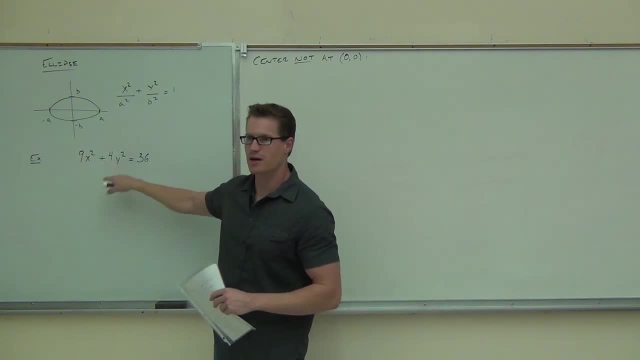 a parabola because that's a y squared. Y squareds are not associated with parabolas, So this thing is either a circle or an ellipse. I can say it's a circle or an ellipse because it's got a plus right here. We're going to find out in a minute if that thing changes. 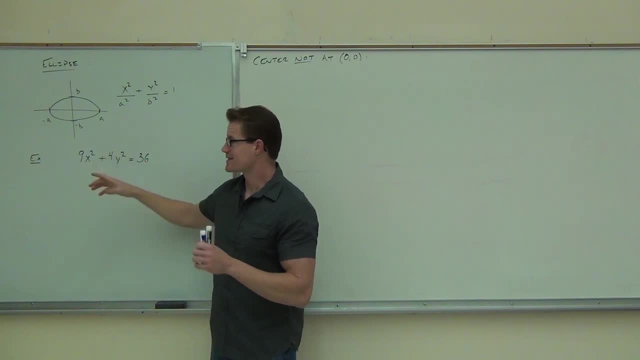 to a minus, we're going to have a different shape altogether. Alright, so it's not a parabola, because parabolas don't have y squared. It's either a circle or an ellipse, because circles and ellipses both have an x squared and a y squared, and 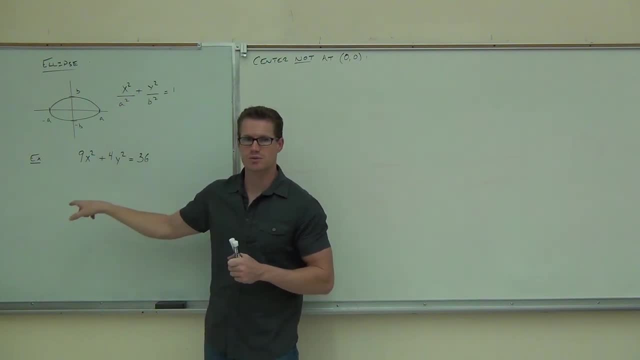 a plus. Is this thing a circle or an ellipse? What do you think? Why is it not a circle? Because circles have x squared and y squared. Why is it not a circle? Okay, if this had been a 9,, what shape would it be? 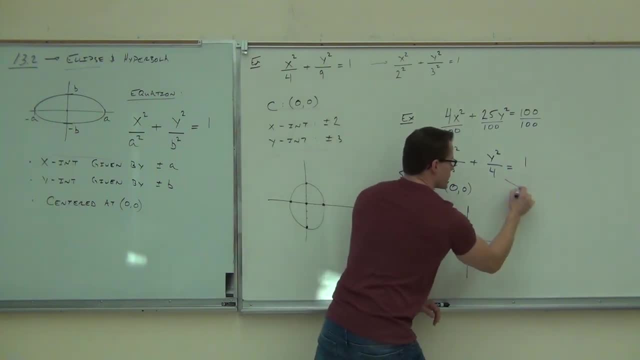 I know that this right here can be written as 5 squared. This right here can be written as 2 squared. 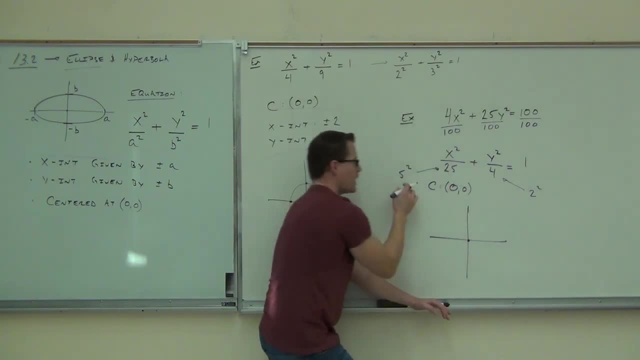 Since this is associated with our x, it says from 0, 0, I'm going to be going plus or minus 5. That's 5 to the right. 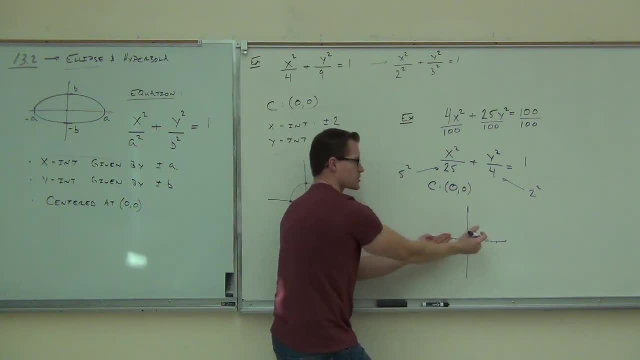 That's 5 to the left. That gives us our spread along the x. Since this was a 4, I know that I can write that as 2 squared. That means that we're going to be going plus or minus 2 from the center of our ellipse. That's up 2 and down 2. 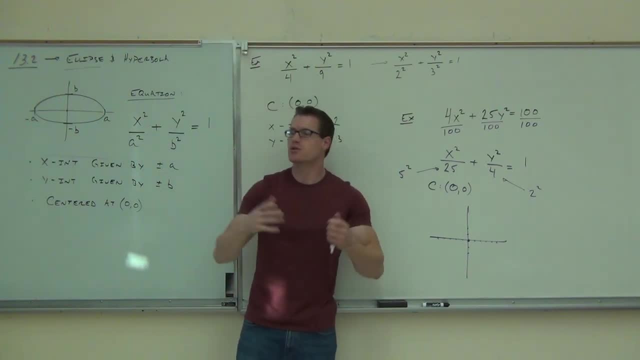 Quick show of hands, how many people feel okay getting that far on these? Now draw your ellipse. Oh, that's pretty good. 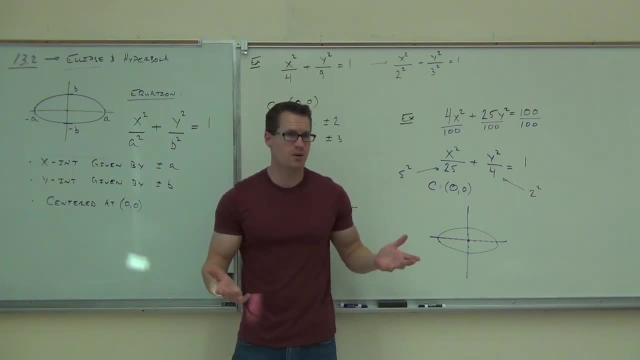 So with just a little bit of work, we can actually be very accurate on these shapes. 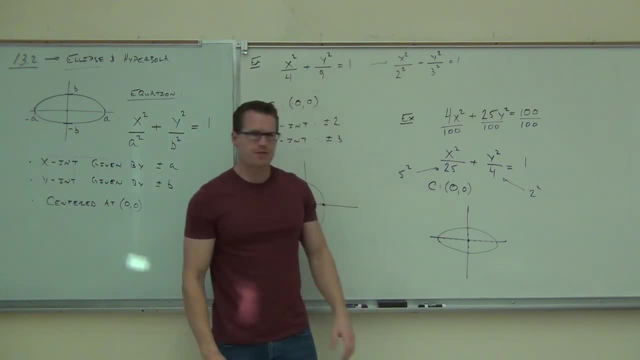 That's all we're going to be able to do on that. The thing is drawing the ellipse about like that. Do you feel okay with circles and ellipses? 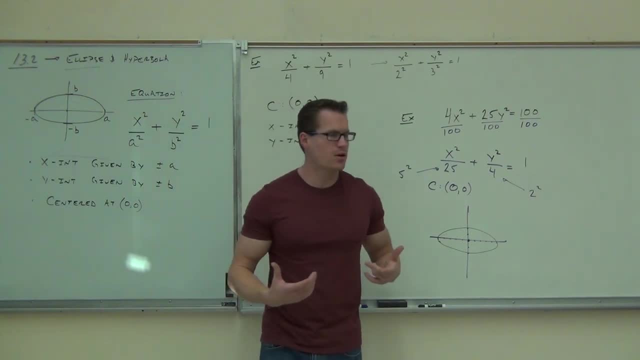 We'll start on one of these examples next time. I'll show you how we can shift it around, talk about hyperbolas, make those things up, and that will be our class. 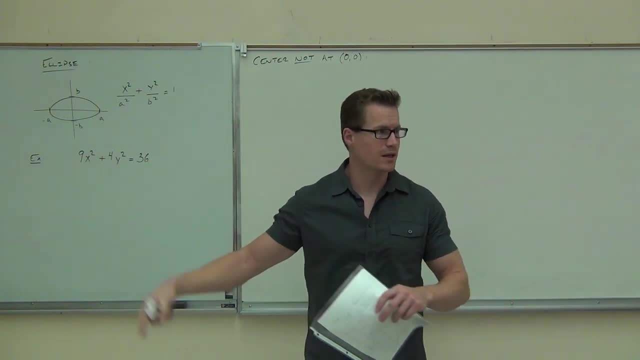 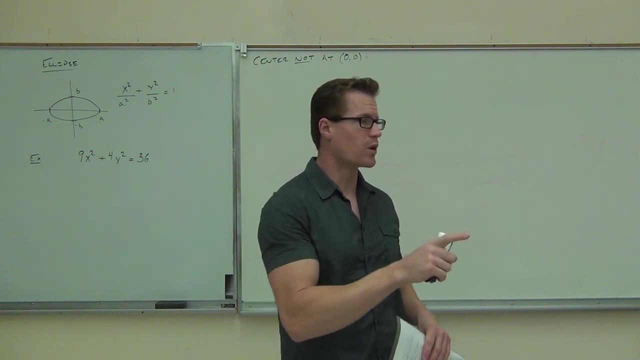 Alright, so we're talking about conic sections again, and we have this thing called an ellipse. Yesterday we went over the formula for an ellipse, how to kind of determine whether something is a circle or an ellipse. So we're going to do one more example talking about this. Let's look back at this example. 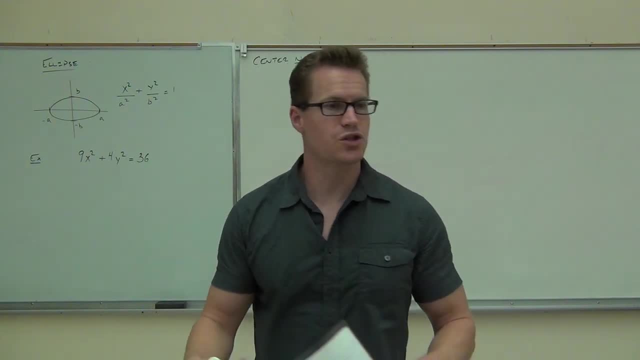 Firstly, you need to be able to determine what? Type of figure it is just by looking at the equation. 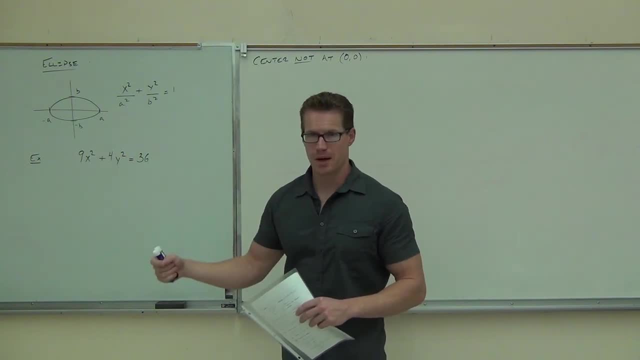 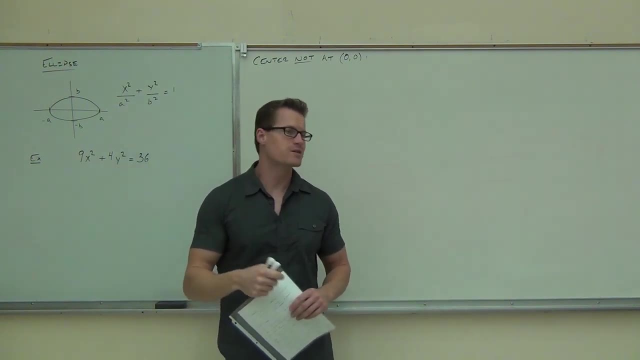 So automatically we can rule out a parabola. We can rule out a parabola because that's a Y squared. Y squareds are not associated with parabolas. So this thing is either a circle or an ellipse. I can say a circle or an ellipse because it's got a plus right here. We're going to find out in a minute if that thing changes to a minus, we're going to have a different shape altogether. 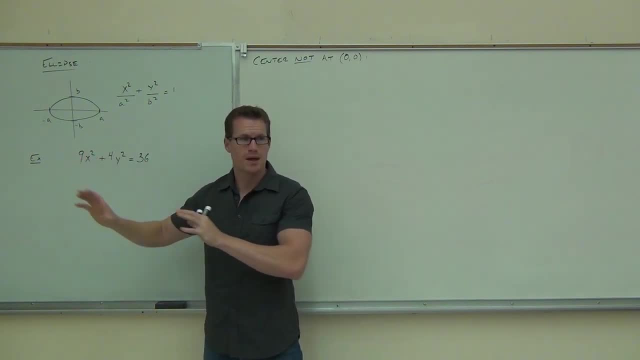 Alright, so it's not a parabola because parabolas don't have Y squared. 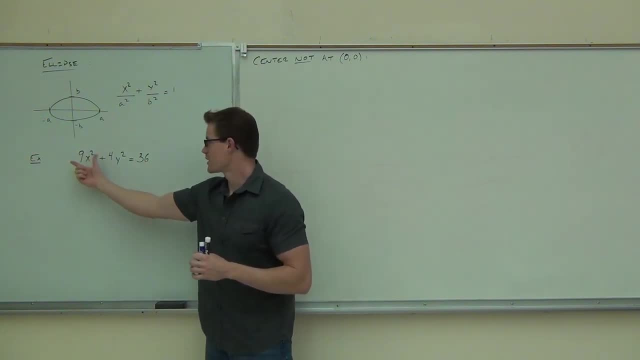 It's either a circle or an ellipse. Because circles and ellipses both have an X squared and a Y squared and a plus. Is this thing a circle or an ellipse? What do you think? It's an ellipse. Why is it not a circle? Because circles have X squared and Y squared. Why is it not a circle? Different. 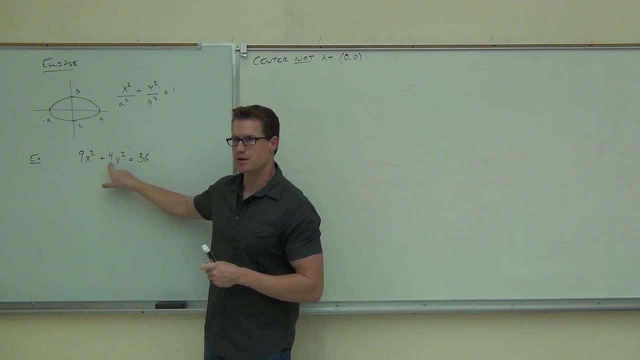 Okay, if this had been a 9, what shape would it be? Circle. 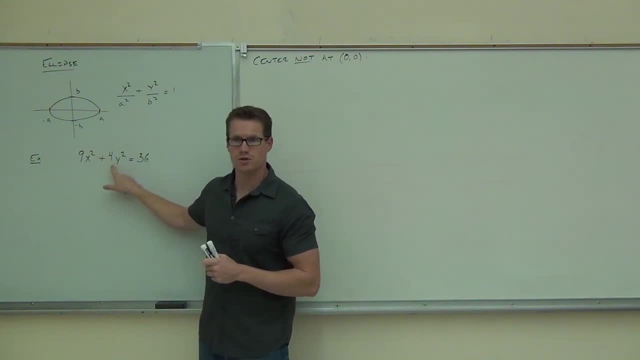 If that had been a 4 and that had been a 4, that would also be a circle. If the numbers are the same, it's a circle, Now with ellipses. we don't really like to have this number over here. that's not a 1.. 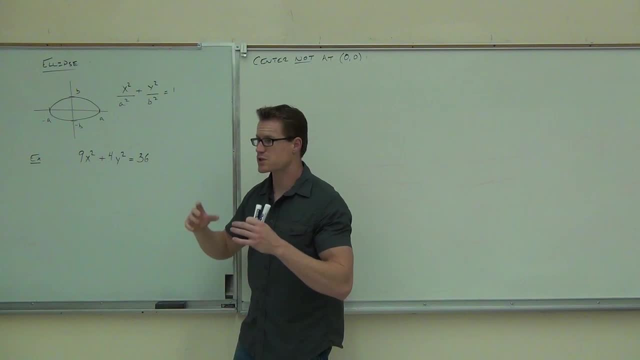 So how do we get rid of that number? Okay? so first thing we're going to do: make sure we get a 1 over here. That means we're going to not subtract 35, but we're going to divide by 36, making sure we get it into. 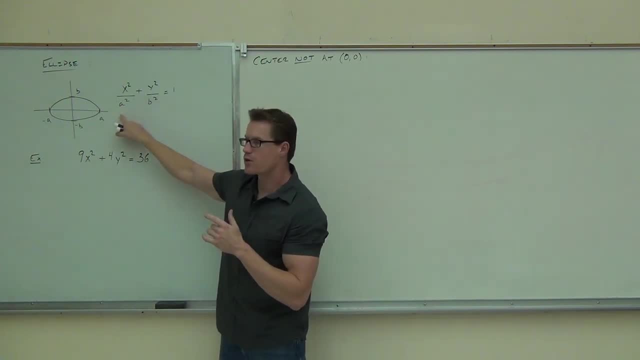 this format because this is going to tell us how far we go on the x and how far we go on the y axis, just by looking under those respective coordinates. So we'll look underneath the x. that'll tell us how far we're going x direction plus and minus. We'll look underneath. 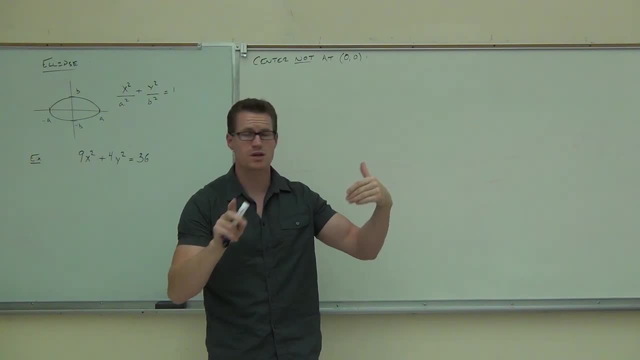 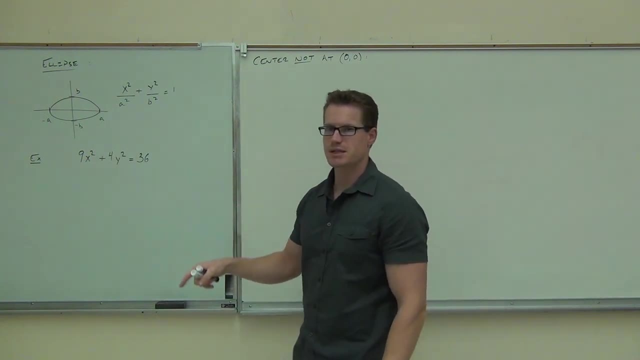 the y. that'll tell us how far we're going. y direction plus and minus. Go ahead and complete that problem for me. So I want you to divide everything by 36.. I want you to find out where the center is. Hopefully it's obvious at this part where the center is for this ellipse. We haven't. 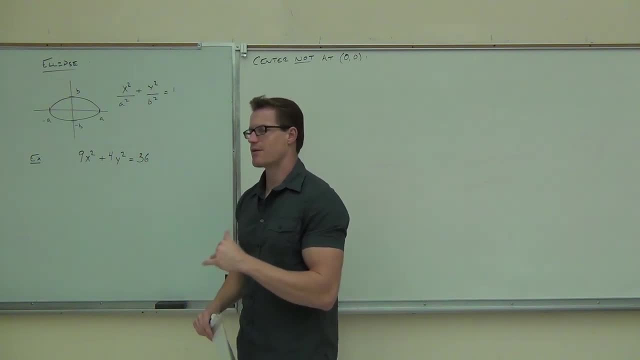 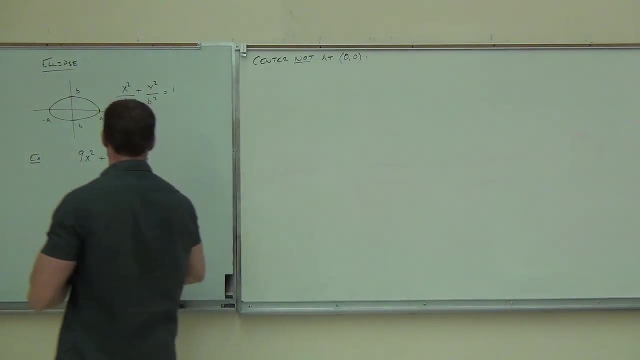 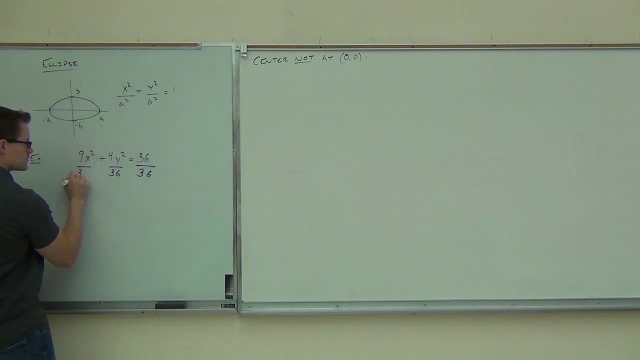 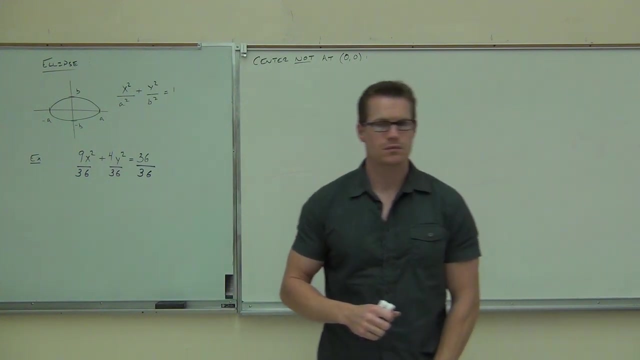 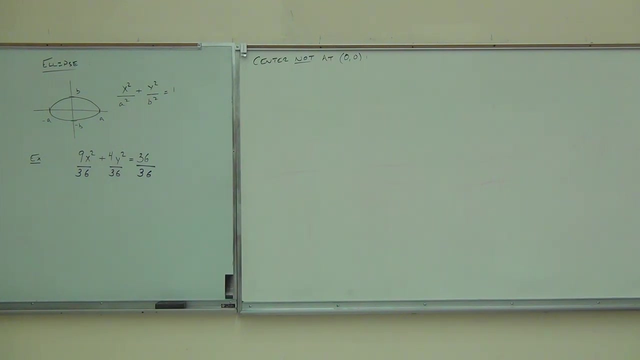 started shifting these around. We're going to talk about that in a minute- And then grab that on your table. Why don't you grab it? So divide it by 36.. Hopefully you were able to get down and simplify these fractions too. What's this fraction become? 9x squared over 36.. How much do we get out of that? 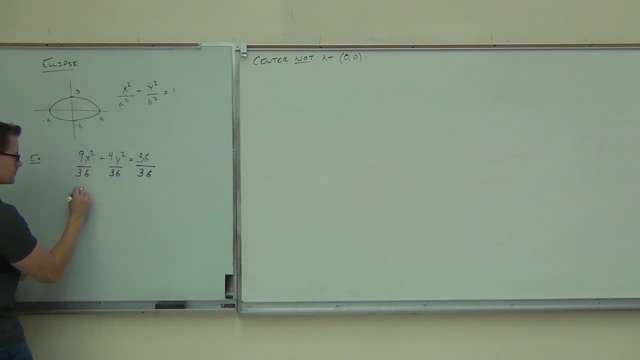 x squared over 4.. Well, somebody else. what do we get out of the next fraction? 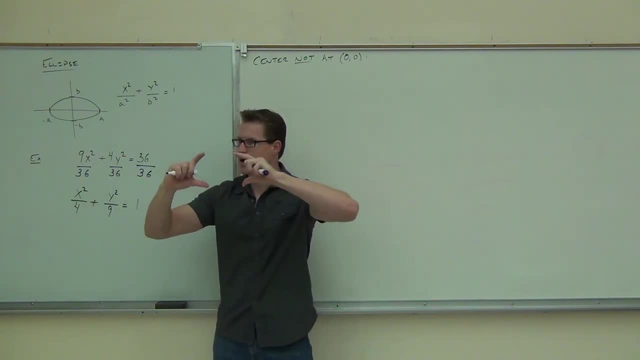 an ellipse If we have different numbers here. what it's saying is it's spreading out, it's squishing out that circle in one direction. If those numbers were the same, it'd say I was squishing that out the same amount in both directions. that would give me a circle. 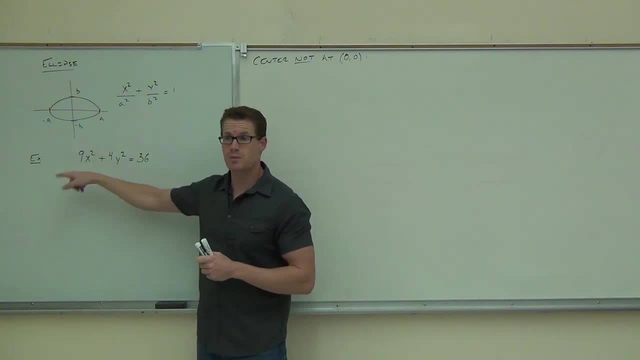 If that had been a 4 and that had been a 4, that would also be a circle. If the numbers are the same, it's a circle. 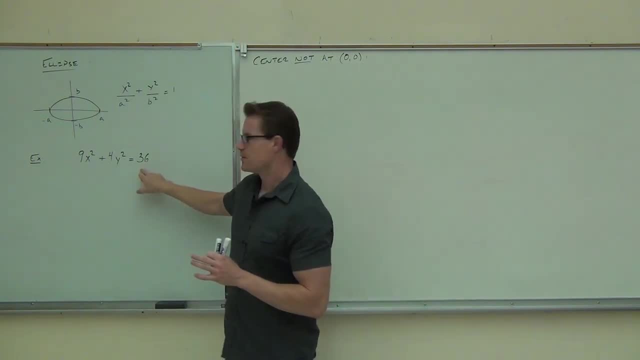 Now, with ellipses, we don't really like to have this number over here that's not a 1. So how do we get rid of that number? 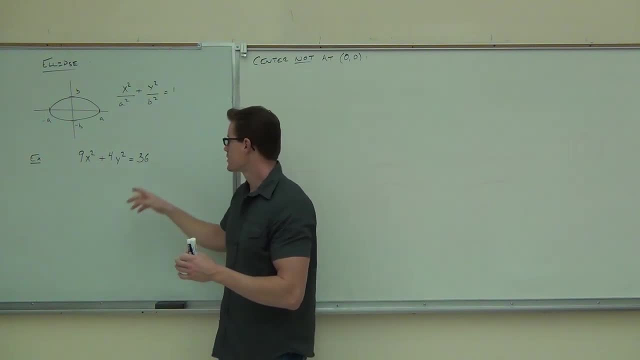 Okay, so first thing we're going to do, make sure we get a 1 over here. That means we're going to not subtract 35, but we're going to divide by 36. Making sure we get it into this format because this is going to tell us how far we go on the X and how far we go on the Y axis just by looking under those respective coordinates. 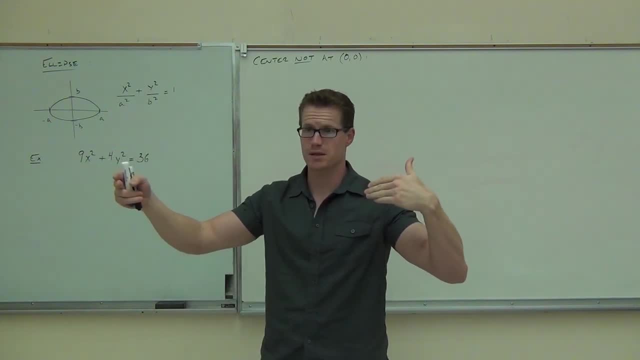 So we'll look underneath the X, that'll tell us how far we go in X direction, plus and minus. Look underneath the Y, that'll tell us how far we go in Y direction, plus and minus. Go ahead and complete that problem for me. 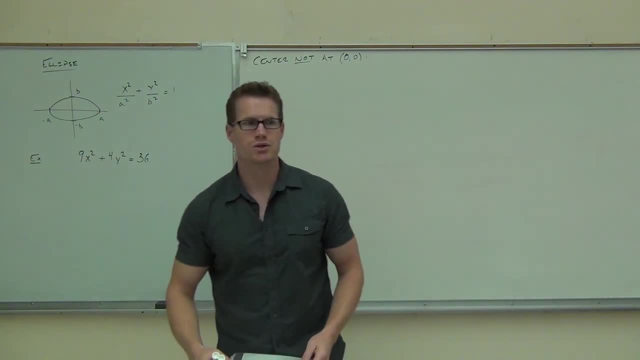 So I want you to divide. I want you to divide everything by 36. I want you to find out where the center is. 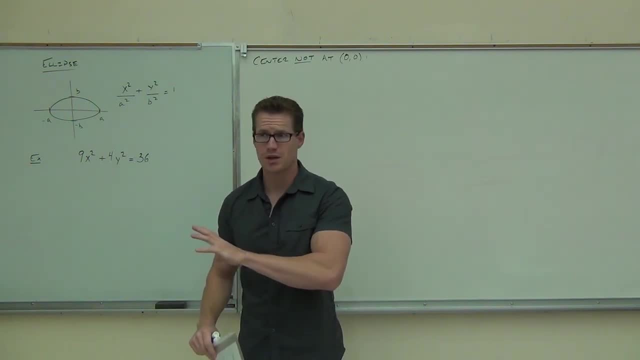 Hopefully it's obvious at this part where the center is for this ellipse. We haven't started shifting these around. We're going to talk about that in a minute. And then grab that on your table. Why don't you grab it? 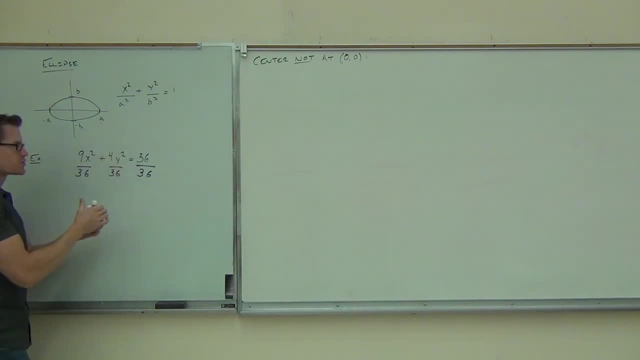 So divided by 36. Hopefully you'll be able to get down and simplify these fractions too. Once this fraction becomes 9 X squared over 36, how much do we get out of that? X squared over 4. . . Somebody else, what do we get out of the next fraction? Y squared over n. Good. Equals to? One. 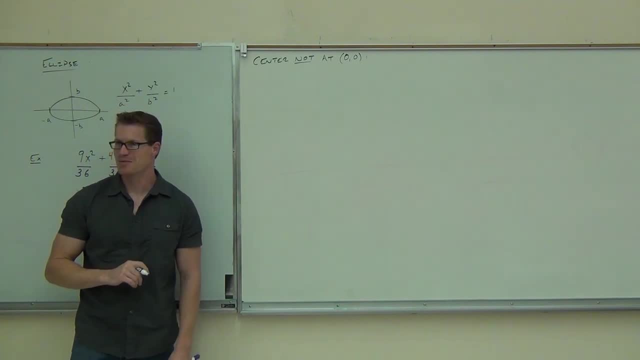 Why, are you guys awake today? Oh, my gosh. I got three people talking. Usually, we're pretty good at this stuff. Did you make it down this far? Yes. 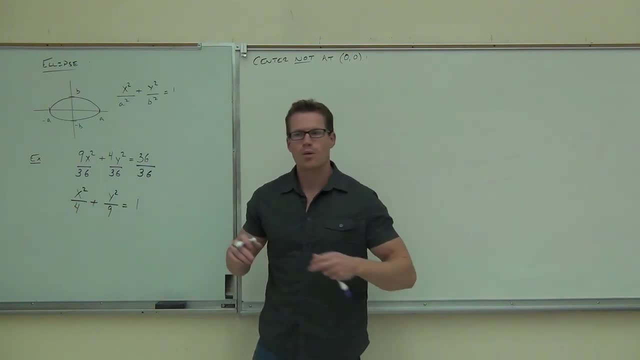 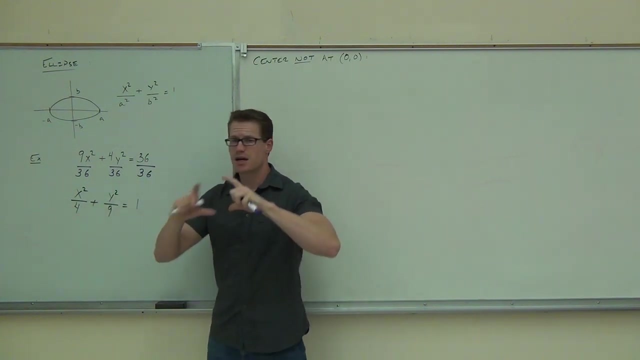 Okay, now, that's clearly an ellipse. Again, what we're looking at here is x squared plus y squared. That tells us we're some sort of circular figure, all right? We're either a circle or an ellipse. If we have different numbers here, what it's saying is it's spreading out, it's squishing out that circle in one direction. If those numbers were the same, it'd say I was squishing that out the same amount in both directions. That would give me a circle. 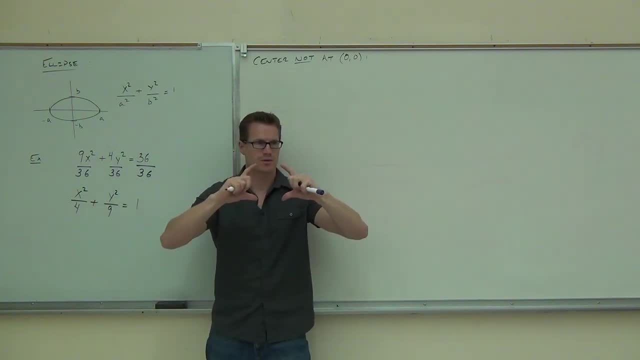 So here we have well along the x direction. we're having well, not four. we're going to find out- we're going to look at it in a minute- how far out we go from any direction on the x, But here we're going at nine. that means we're going to be spreading out which 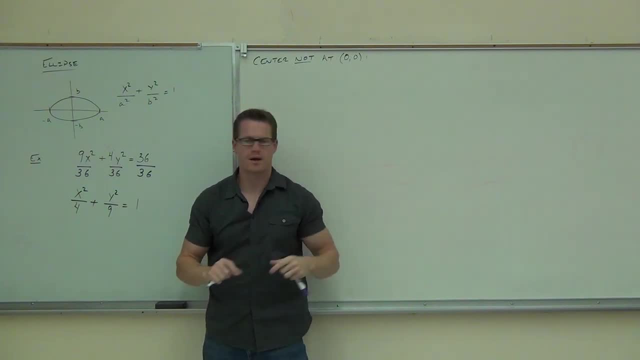 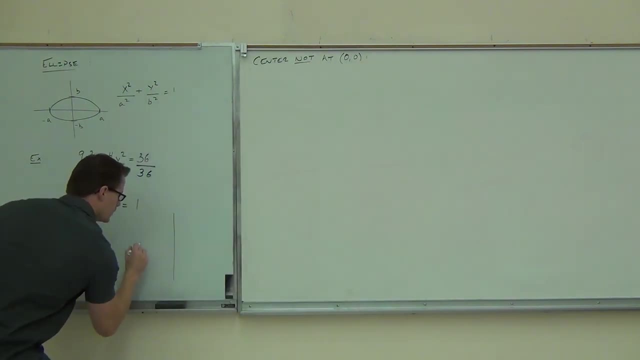 way. More along the x or more along the y. What do you think? More along the y, More along the y? I said that number's bigger. that means we're in that direction that much more. Also, where is the center of this ellipse? 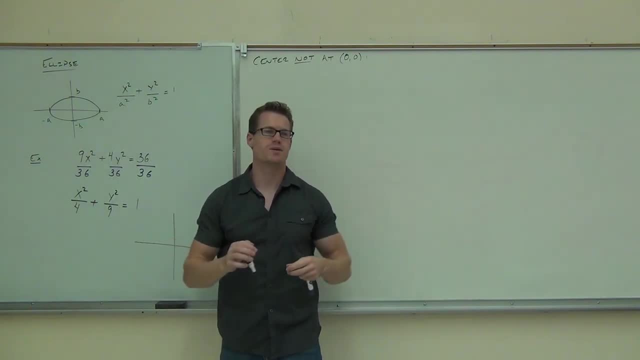 The origin, Yeah, the origin. good, Someone said zero, zero. Why is it around the origin? Or why is it right at the origin? Not just because it's an ellipse, but if we look at the top of our function here we've. 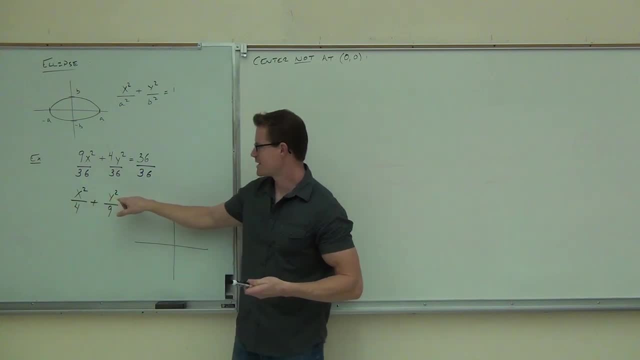 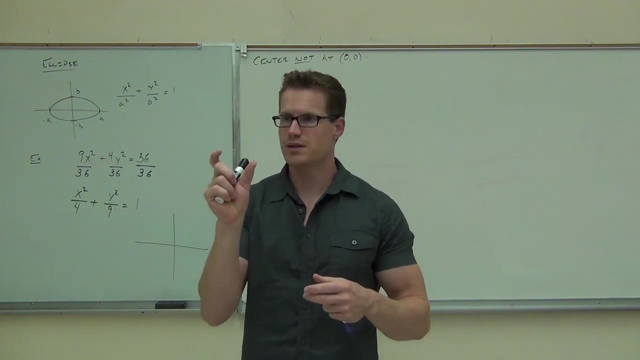 got. is there anything being added to x? No, And we've got. is there anything being added or subtracted from y? No, That means it's not shifting it around, Just like on our circles. before, if we had a plus x or minus x, that meant left or right. 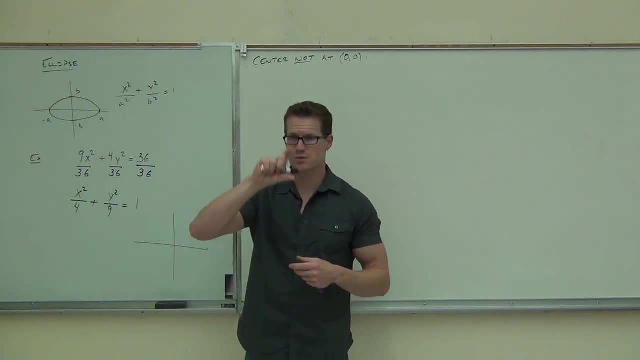 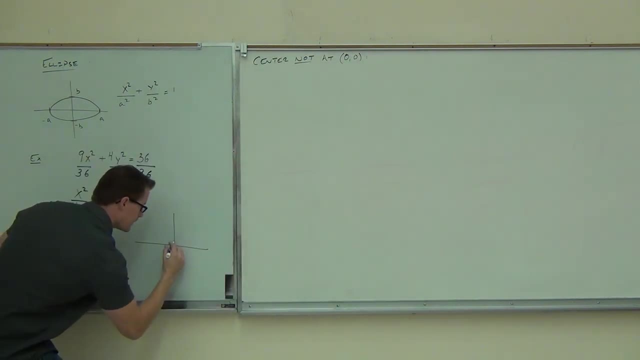 shift. And if we had a plus or minus y, that means we're even going up and down from the origin. So right here we're not shifting this at all. that means our center is right at the origin, Center's right at the origin, so center's zero, zero. 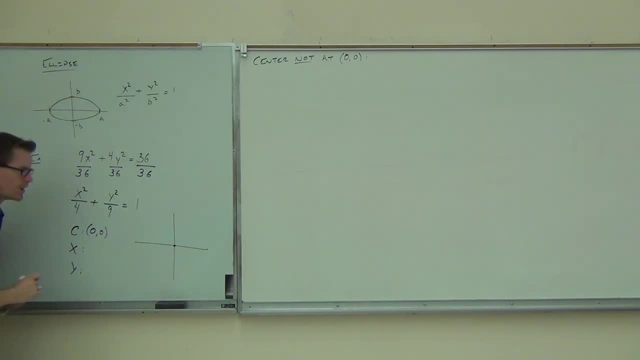 Okay, Okay, Okay, Okay. Also talk about the x direction and the y direction. Along the x direction, how much are we going left and right? Are we going 4, are we going 16, or are we going 2?? 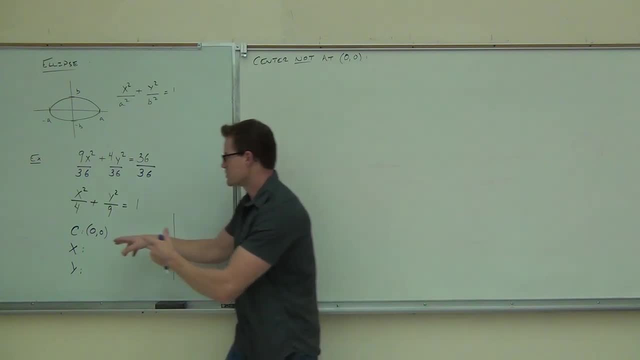 Those are the three most common answers, because people get confused as to what you do with that number. Do you take it just like it is, Do you square it, or do you square root it? Which one Square it? So we're not going to square it, right? 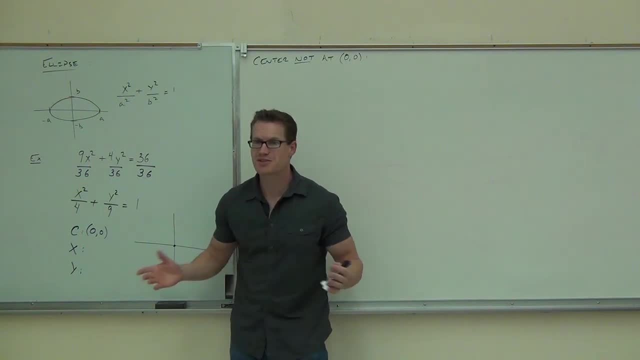 If we square it, we're going to get 16.. I'm going to square it, We're going to unsquare it. What's the opposite of what's unsquaring? it mean Square root, It's square root. A square root and a square are inverse operations. 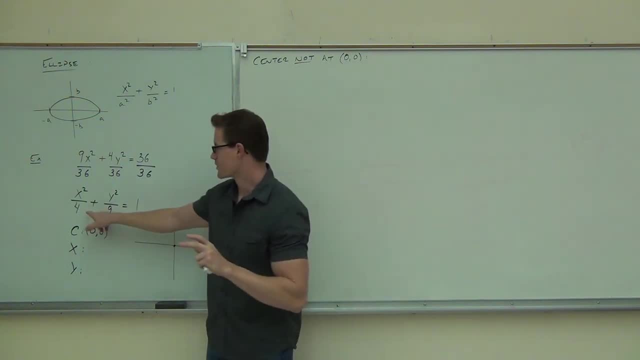 That's how we identify the square root to begin with. So if you're going to look at this thing right here and you go, OK, I know I'm not going left 4 and right 4.. I'm definitely not going left 16 and right 16.. 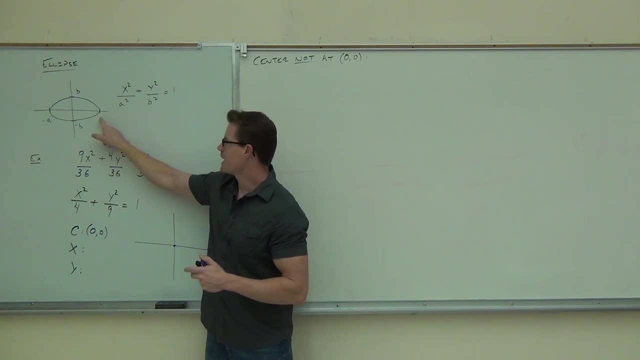 We look here and this says that this number is our a after it's been squared. So we need to undo that. We're going to take a square root of that. So if this is a squared, we want to find just a. 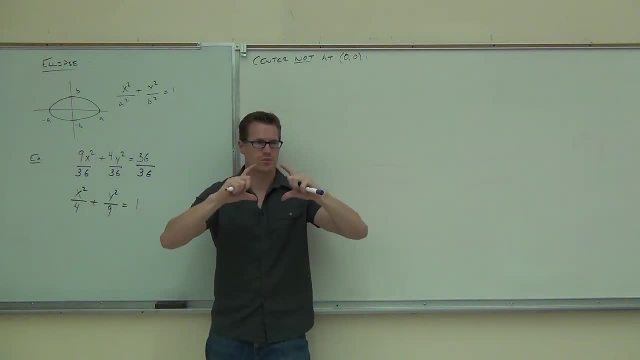 So, here we have, well, along the x direction, we're having, well, not four. We're going to find out, we're going to look at it in a minute, how far out we go from any direction on the x. But here, we're going at nine. That means we're going to be spreading out which way? More along the x or more along the y? What do you think? Along the y. The y, that number's bigger. That means we're in that direction. That much more. 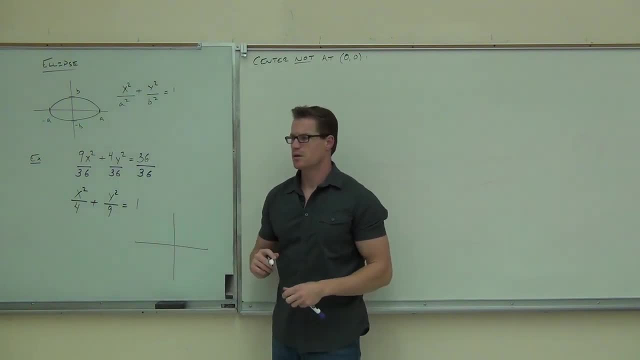 Also, where is the center of this ellipse? The origin. Yeah, the origin. 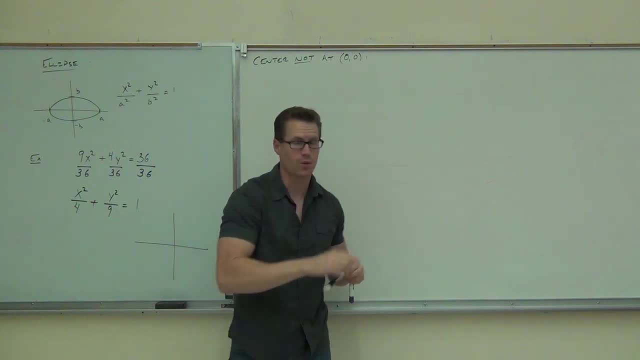 Good. Someone said zero, zero. Why is it around the origin? Or why is it right at the origin? 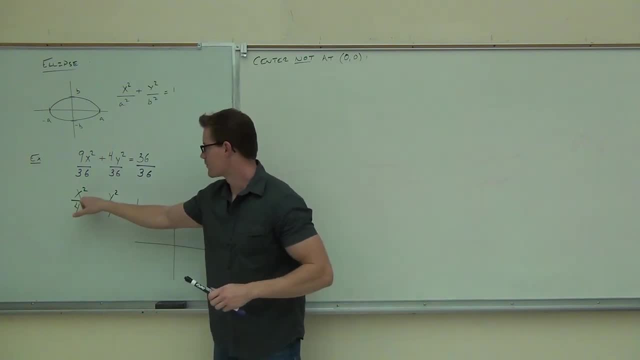 Not just because it's an ellipse, but if we look at the top of our function here, we've got, is there anything being added to x? No. And we've got, is there anything being added or subtracted from y? No. 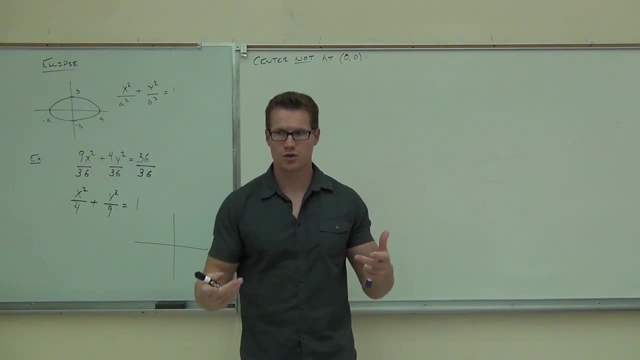 That means it's not shifting it around. Just like on our circles before. 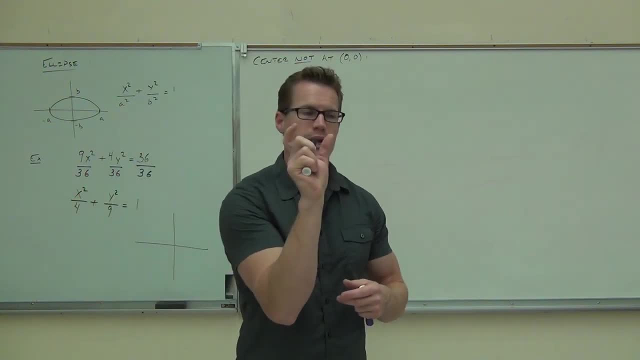 If we had a plus x or minus x, that meant left or right shift. And if we had a plus or minus y, that means we're going up and down from the origin. So, right here, we're not shifting this at all. That means our center is right at the origin. 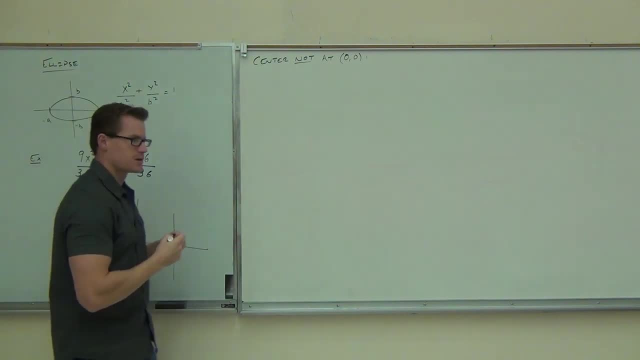 Center's right at the origin. 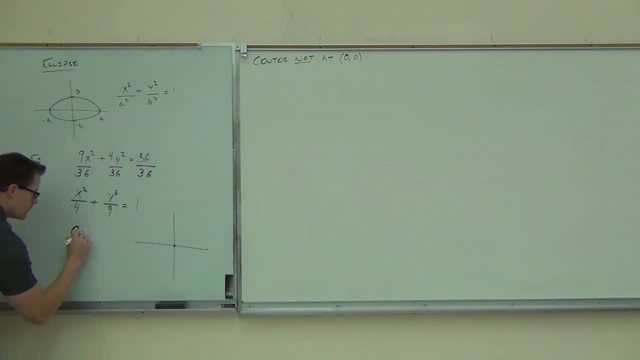 So, center's zero, zero. We'll also talk about the x direction and the y direction. 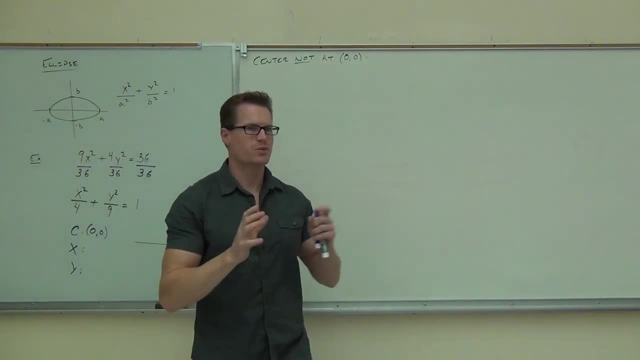 Along the x direction, how much are we going left and right? Are we going four, are we going 16, or are we going two? Those are the three most common answers because people get confused as to what to do with that number. Do you take it just like it is? No. Do you square it or do you square root it? Which one? Square root. 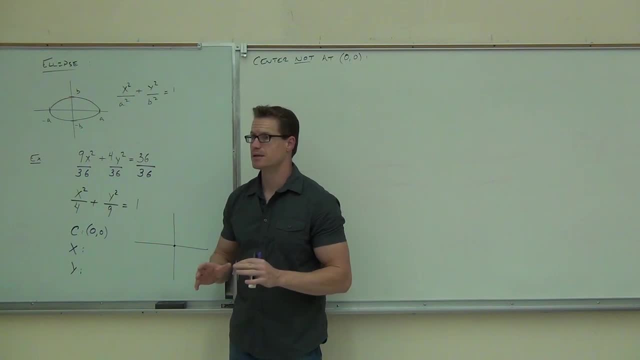 So, we're not going to square it, right? If we square it, we're going to get 16. Am I going to square it? Two square. 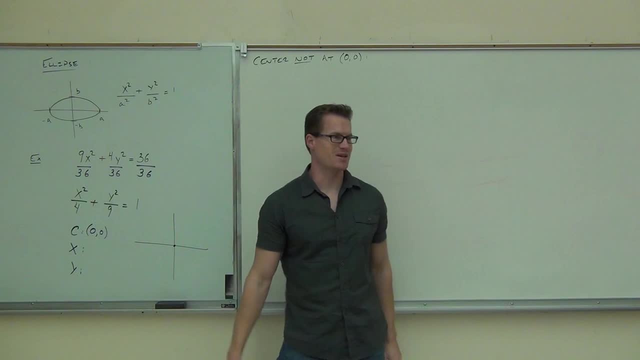 We're going to unsquare it. What's the opposite of, what's unsquaring it mean? Square root. It's square root. A square root and a square are inverse operations. 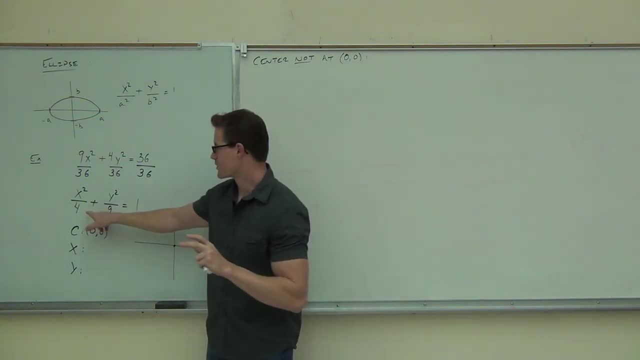 That's how we identify the square root to begin with. So, if you're going to look at this thing right here and go, okay, I know I'm not going left four and right four. 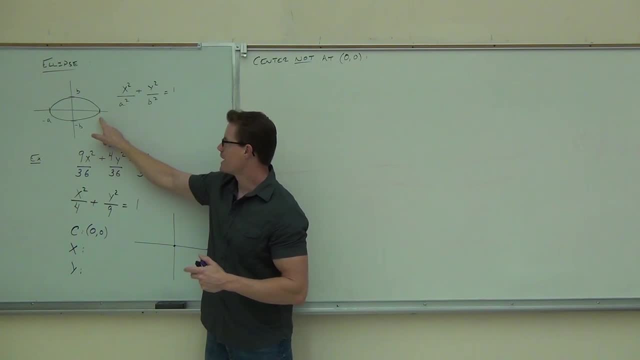 We look here and this says that this number is our a after it's been squared. So, we need to undo that. 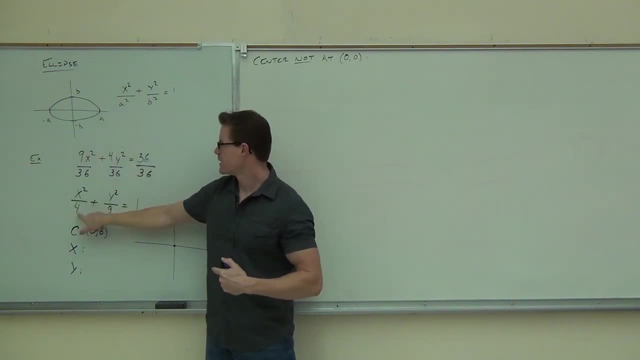 We're going to take a square root of that. So, if this is a squared, we want to find just a. That's the square root of four. We're going to get two. Why? 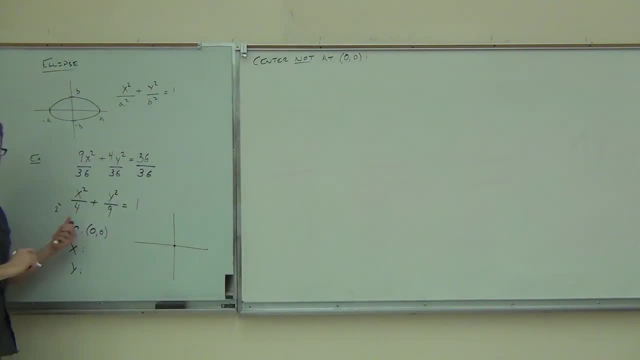 Well, you could write this as two squared. True? That fits that format. 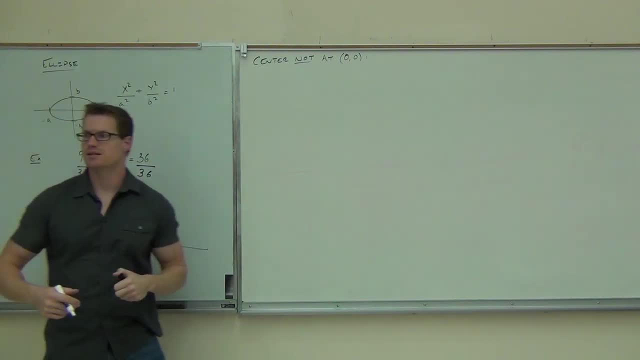 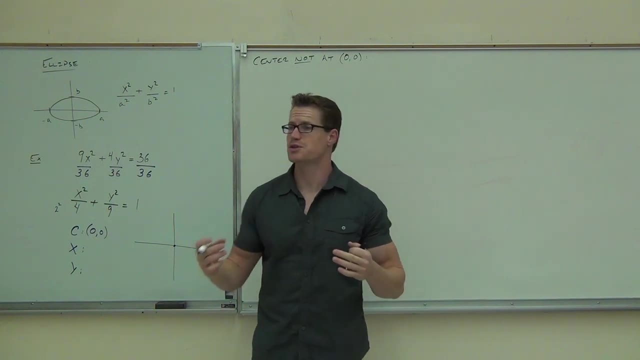 So, if that's two squared, our a in this case is two. To get rid of the square, we've got the two. That means we're going left two and we're going right two from wherever our center happens to be. Now, in the past few examples, our center's been at zero, zero. 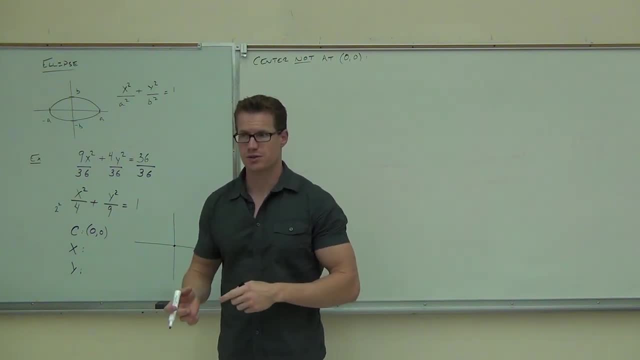 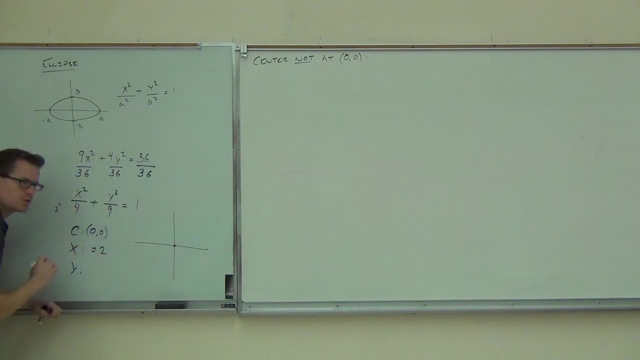 In just a moment, we're going to look at where our center's not at zero, zero. That's why I've kind of omitted the word x-intercept. I'm just talking about x now and the y-intercept. I'm just talking about y now. Because in the moment, we're not going to have a center there. These distances won't exactly be x and y-intercepts. They'll just be movement along the x-direction, negative and positive. Movement along the y-direction, negative and positive. So, in our case right here, yeah, we're going plus and minus two units from wherever our center is. 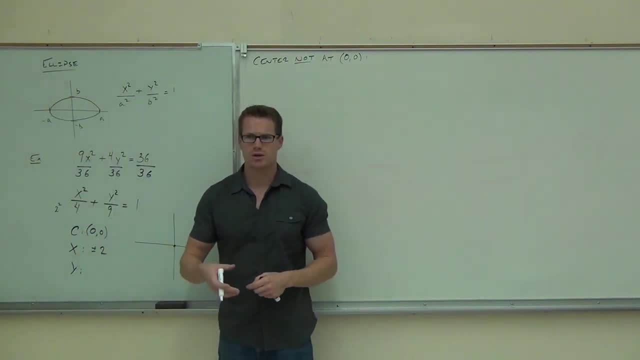 How about along the y? How much are we going? Up and down, how much? Three. 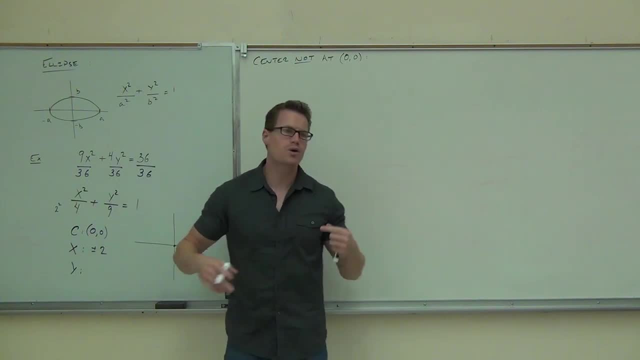 Good, because we're looking at nine. That can be written as three squared. Or you think about it, the square root of nine, that gives us three. 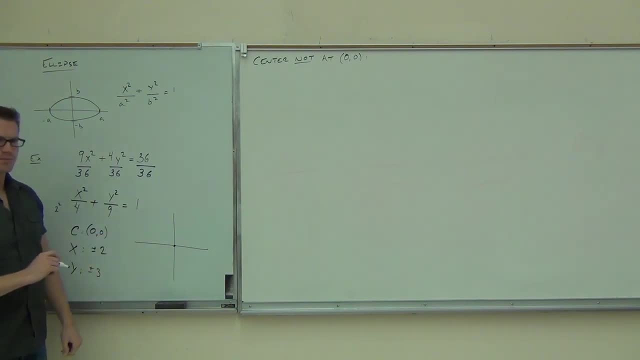 So, from our center, hopefully you went right two, left two, up three, down three. And it shows you, if you look at that, we are spreading out more along the y just like we thought. 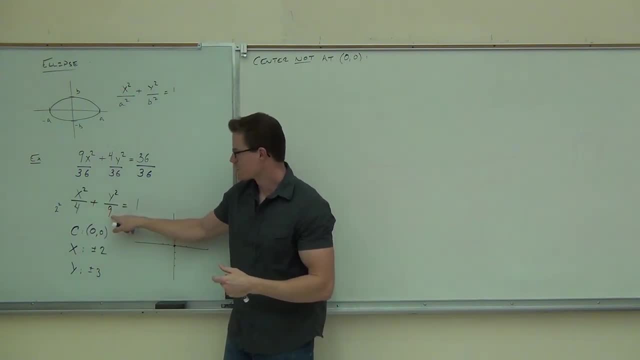 It's certainly an ellipse because these numbers are different. And this number was bigger underneath the y. It's associated with our y, so we're going to spread out more along the y. It's going to make a taller ellipse rather than a wider ellipse. 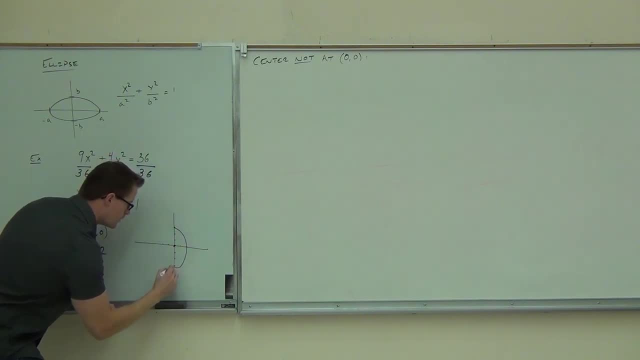 There we go, that's our picture. How many people were able to make that picture? 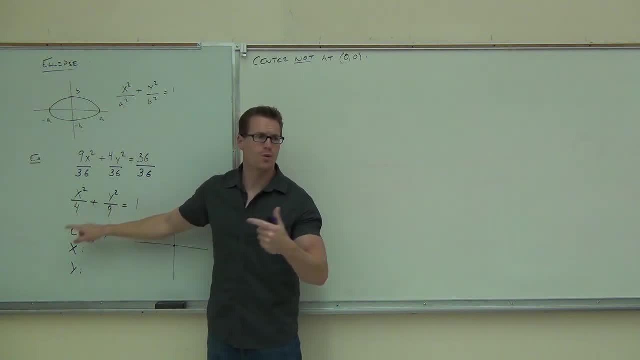 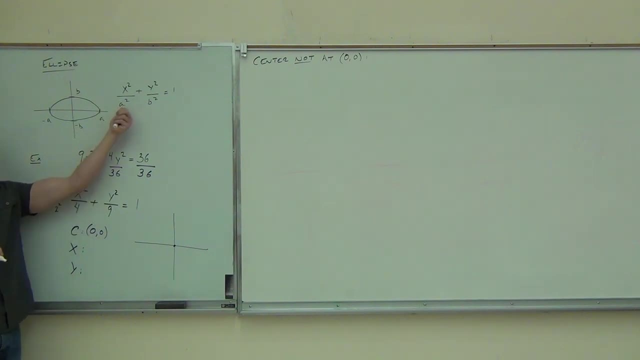 We're going to undo that, The square root of 4, we're going to get 2.. Why, Well, you could write this as 2 squared True, That fits that format. So if that's 2 squared, our a in this case is 2.. 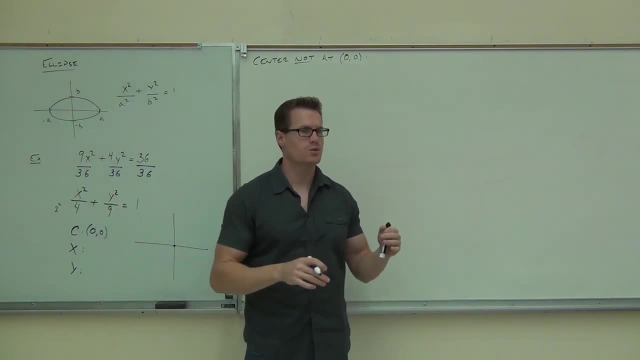 If you get rid of the square, we've got the 2.. That means we're going left 2 and we're going right 2 from wherever our center happens to be. Now, in the past few examples, our center's been at 0, 0.. 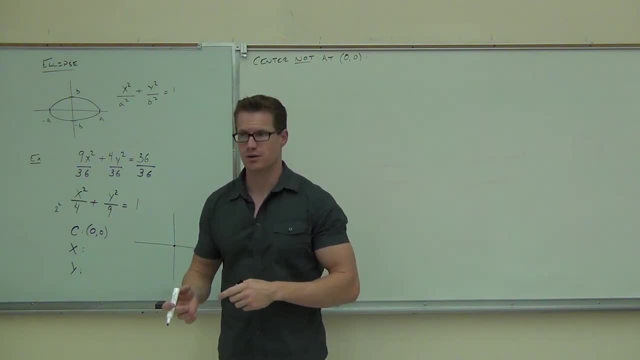 In just a moment we're going to look at where our center's not at 0, 0.. That's why I've kind of omitted the way that we use the word x-intercept. I'm just talking about x now And the y-intercept. I'm just talking about y now. 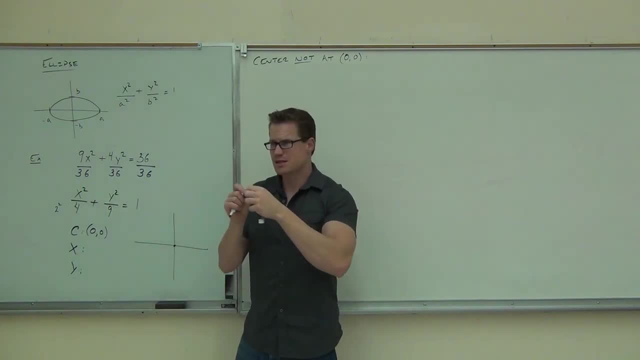 Because in the moment we're not going to have a center there. These distances won't exactly be x and y-intercepts, They'll just be movement along the x-direction- negative and positive, moving along the y-direction- negative and positive. 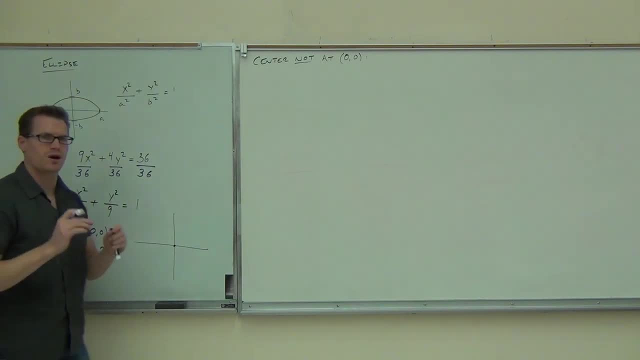 So in our case, right here, yeah, we're going plus and minus 2 units from wherever our center is. How about along the y? How much are we going Up and down? how much? 3. Good, because we're looking at 9.. 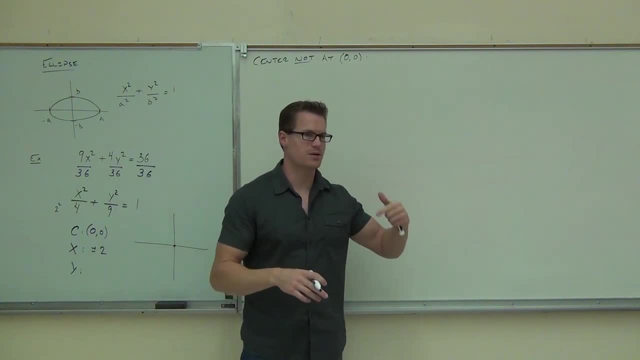 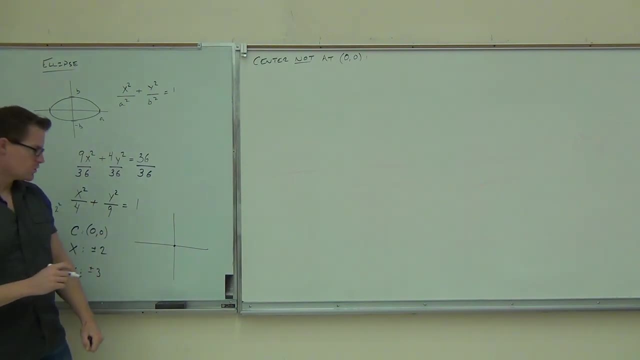 That can be written as 3 squared. What would you think of it? How about the square root of 9? that gives us 3?. So from our center, hopefully, you went right: 2, left 2, up 3, down 3.. 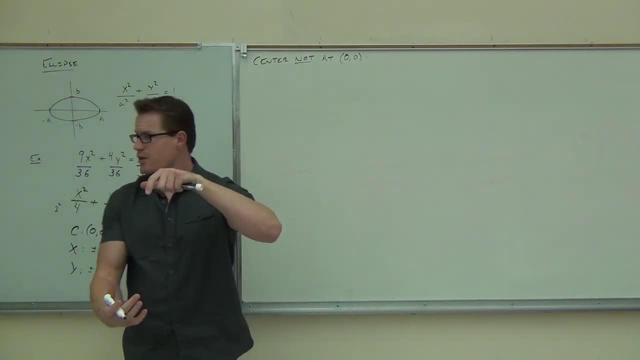 And it shows you, if you look at that we are spreading out more along the y, just like we thought. It's certainly an ellipse, because these numbers are different And this number was bigger underneath the y. It's associated with our y. 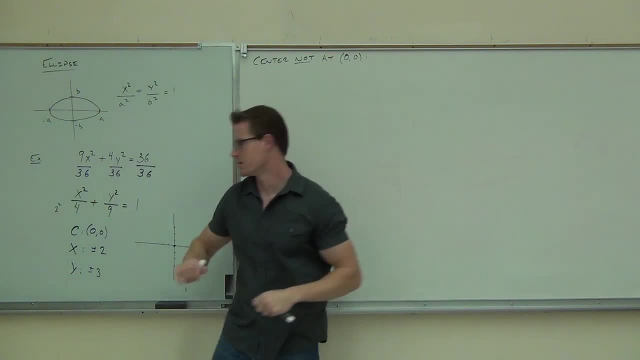 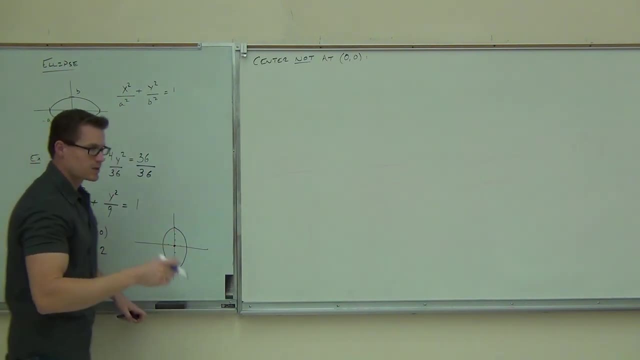 So we're going to spread it out. We're going to spread out more along the y. It's going to make a taller ellipse rather than a wider ellipse. There we go. That's our picture. How many people were able to make that picture? 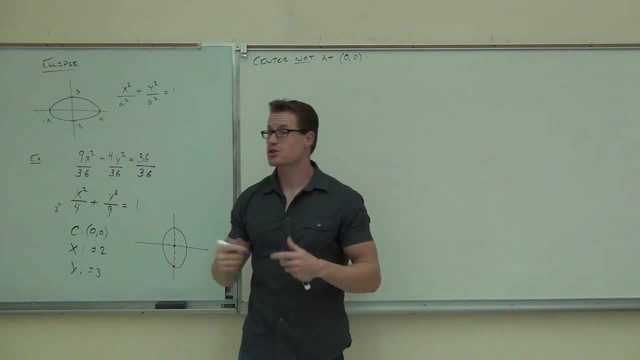 Good for you. That's fantastic. Now, are there cases, just like circles, where we don't have to have our ellipses centered around 0?? Well, I hope so, because I've been talking about it for the last five minutes, right? 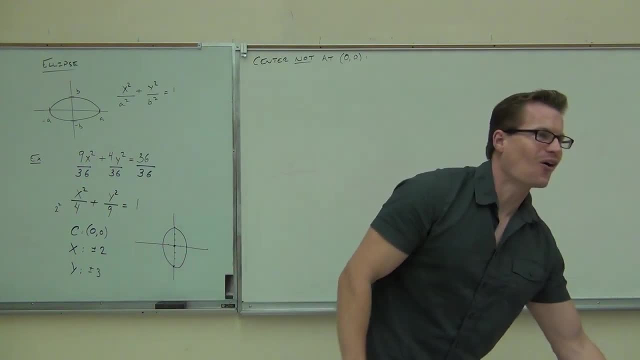 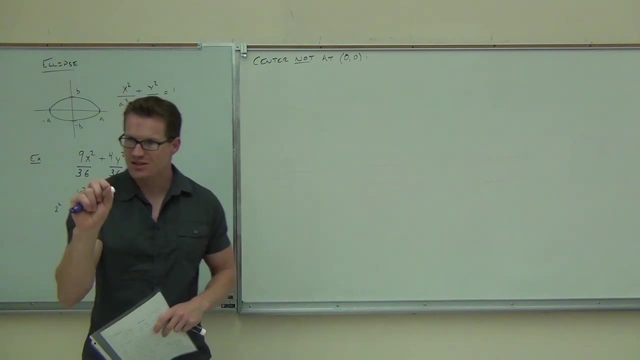 I hope that's the case, Otherwise that was a wasted five minutes. Yeah, there are. We're going to look at the equation for making ellipses that aren't at the center of our graph, So aren't centered at the origin, in other words. 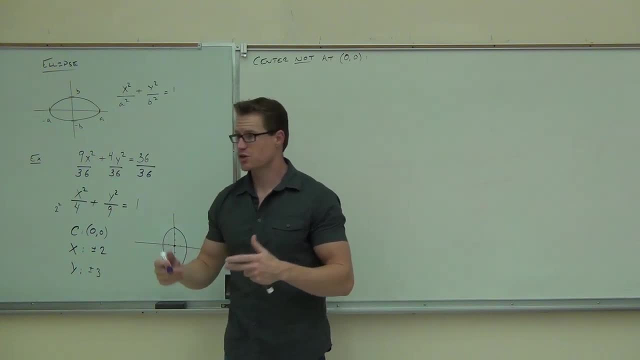 Good for you, that's fantastic. Now, are there cases, just like circles, where we don't want to have our ellipses centered around zero? Well, I hope so because I've been talking about it for the last five minutes, right? I hope that's the case, otherwise that was a wasted five minutes. Yeah, there are. 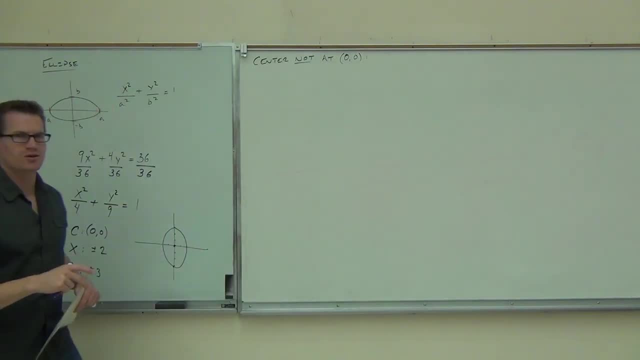 We're going to look at the equation for making ellipses that aren't at the center of our graph. So, aren't centered at the center of our graph. 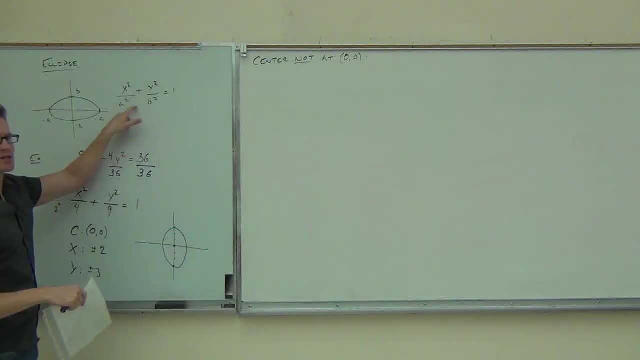 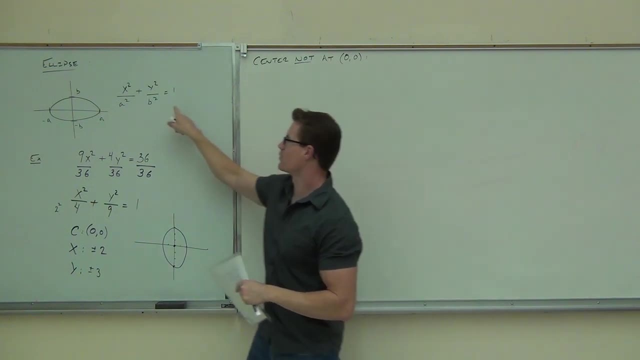 They're centered at the origin, in other words. Now, it's going to look very similar to this, but what can you expect to happen from this formula to a formula that's not centered at zero, zero? What do you think is going to change? Is the a going to change? What do you think? Is the b going to change? Is the one going to change? What is going to change? The top. 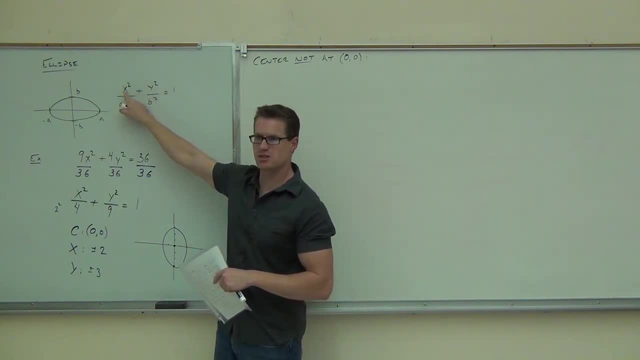 The top, yeah. What's going to happen with this? How's it going to look? Instead of just x squared, what might I expect to have up there? Is that going to be x squared minus two or plus two? Is that going to be x squared minus two or plus two? 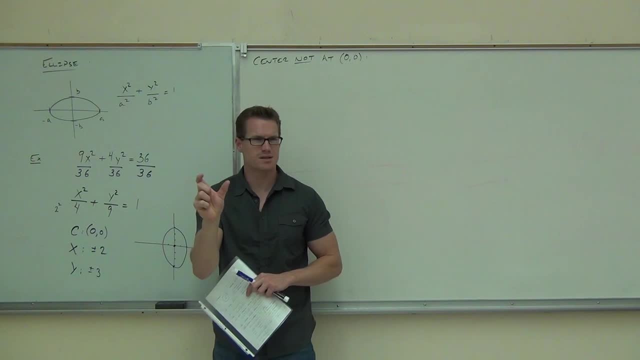 We're probably going to have a number in there. In what? Inside of what? Some parenthesis. 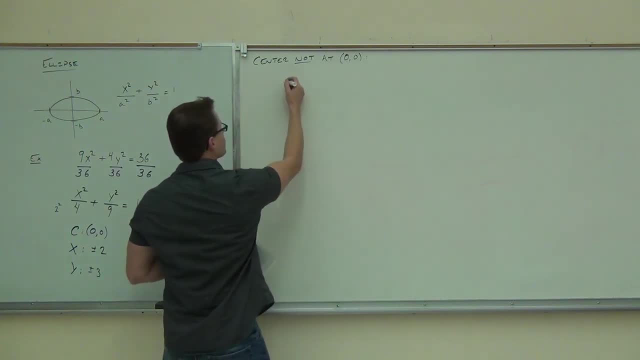 Some parenthesis. We're going to have some parenthesis. Just like we had with the circles. 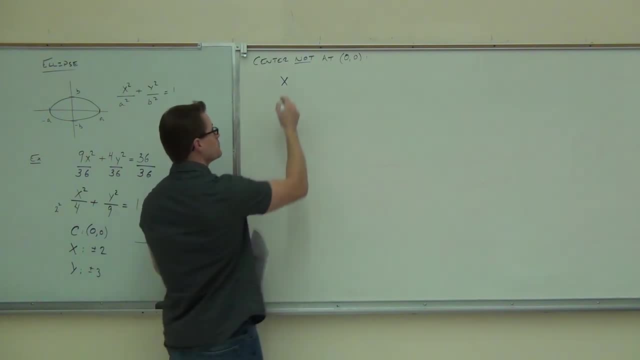 What letter was normally associated with the x? H. And with the y? 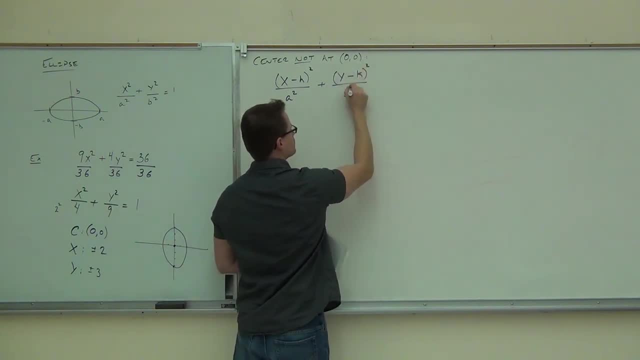 Yeah. Hey, does that look familiar? Yeah. 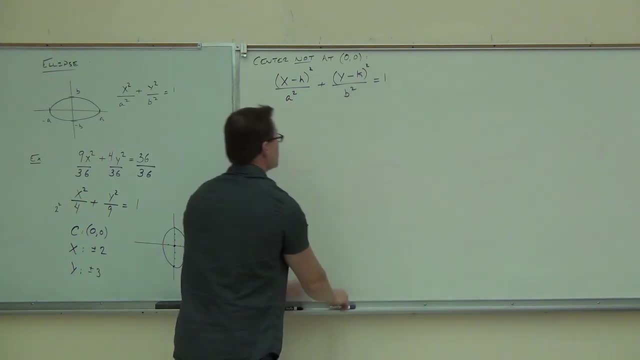 I hope it looks familiar. If you do this to it, that looks just like a circle, doesn't it? Yeah. With a radius of, well, one. 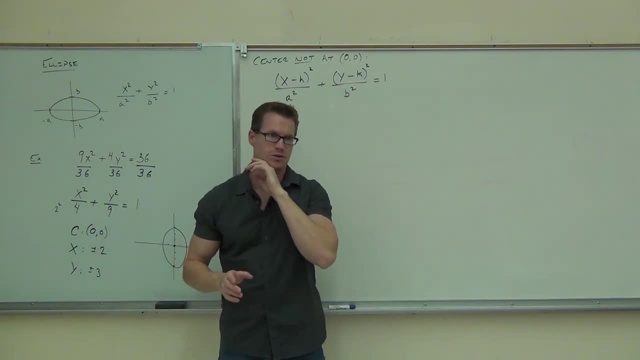 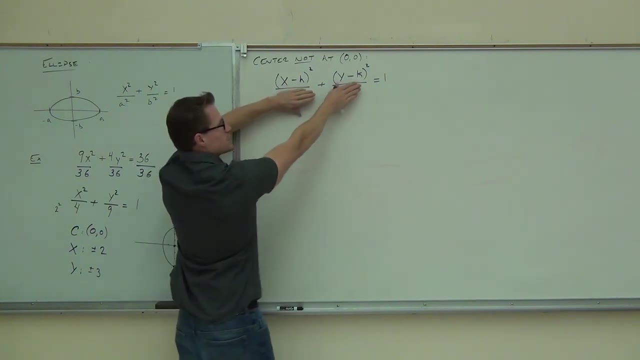 And that's called the unit circle. You'll talk about unit circle when you get to Math 2 or your trigonometry class, or whatever you have. But that would be a unit circle, saying the radius is one. But that thing looks exactly like a circle. 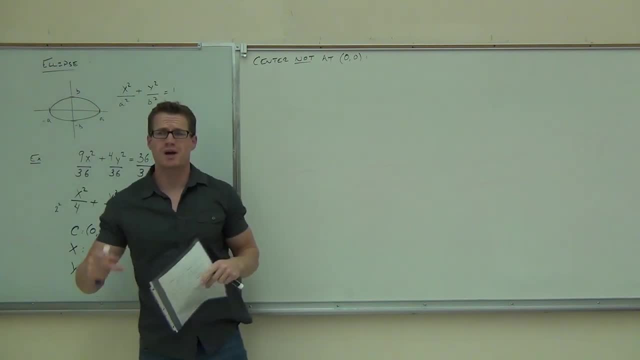 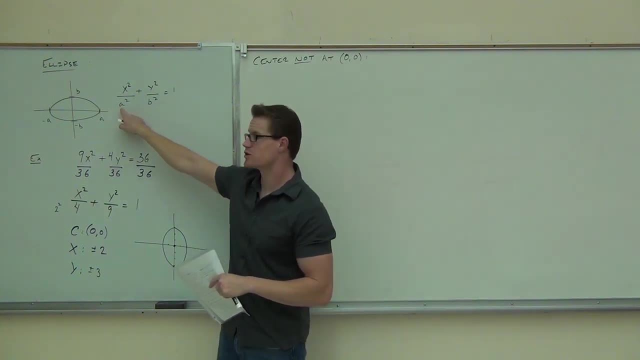 Now it's going to look very similar to this, But what can you expect to happen from this formula to a formula that's not centered at 0, 0?? What do you think is going to change? Is the a going to change? 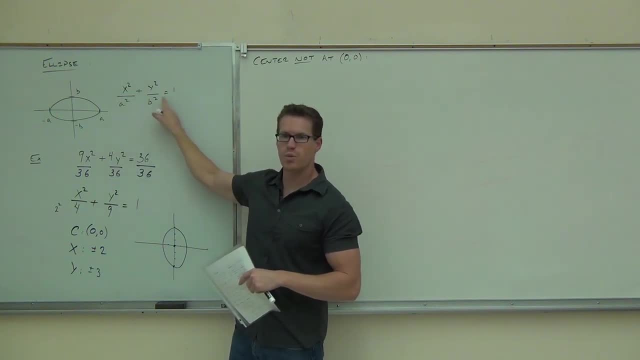 What do you think? Is the b going to change? Is the 1 going to change? What is going to change? The top, The top, yeah. What's going to happen with this? How's it going to look, instead of just x squared? 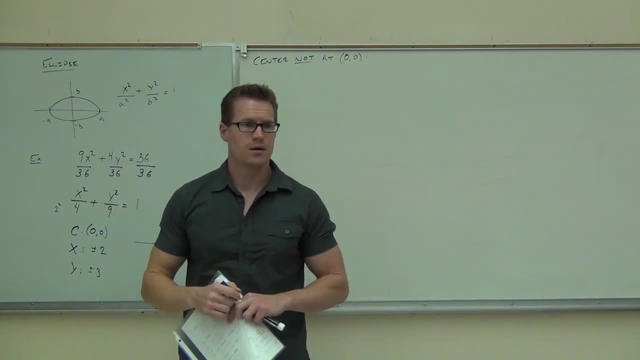 What might it look like? How do I expect to have up there X squared minus 2 plus 2.. Is that going to be x squared minus 2 or plus 2? We're probably going to have a number in there. in what? 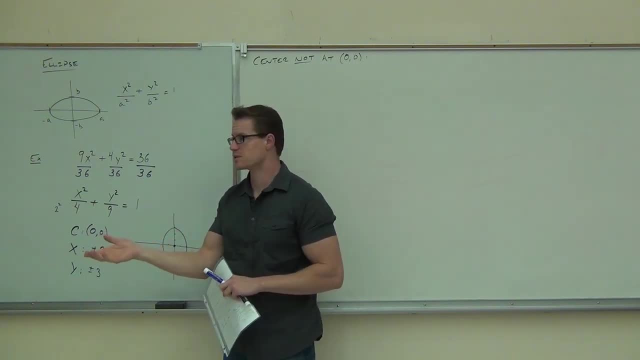 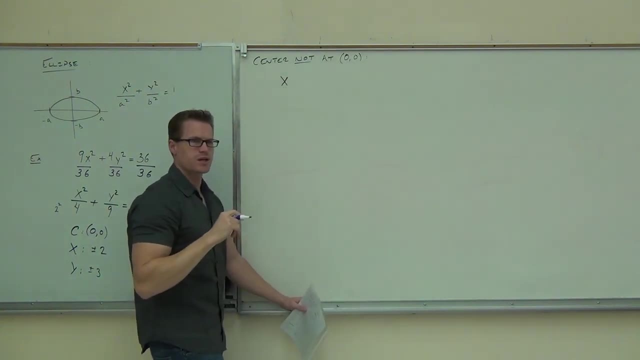 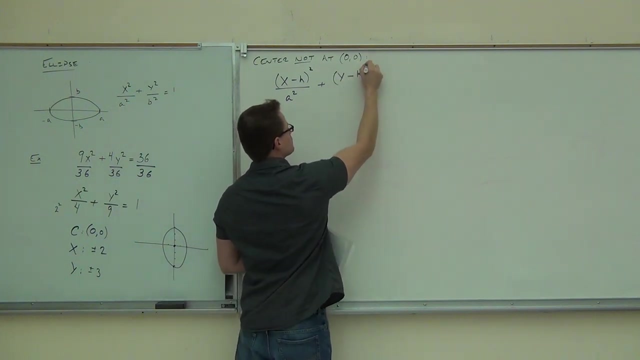 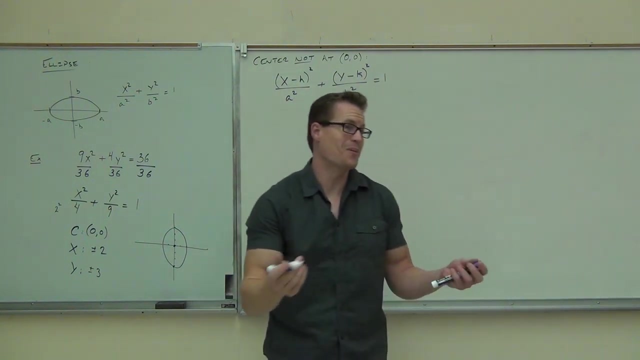 Inside of what The letter x, Some parentheses. We're going to have some parentheses, just like we had with the circles. What letter was normally associated with the x, H, H, was, And with the y, K? Hey, does that look familiar? 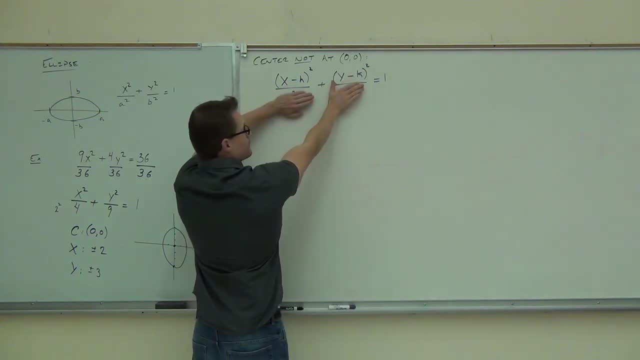 Yeah, I hope it looks familiar If you do this to it. that looks just like a circle, doesn't it? Yeah, With a radius of 1. That's called the unit circle. You'll talk about unit circle when you get to Math 2. 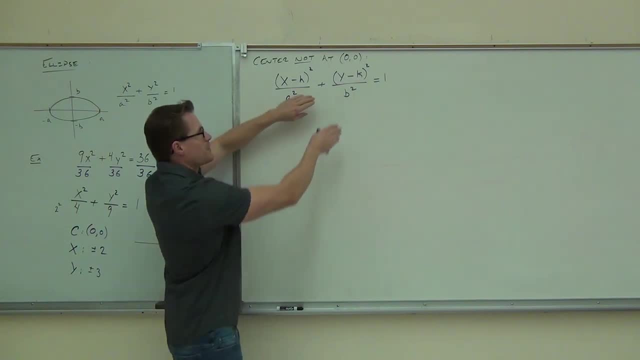 or your trigonometry class or whatever you have, But that would be a unit circle, say, and the radius is 1. But that thing looks exactly like a circle. Now, if I divide it by numbers that are different, I don't have a circle anymore, I have an ellipse. 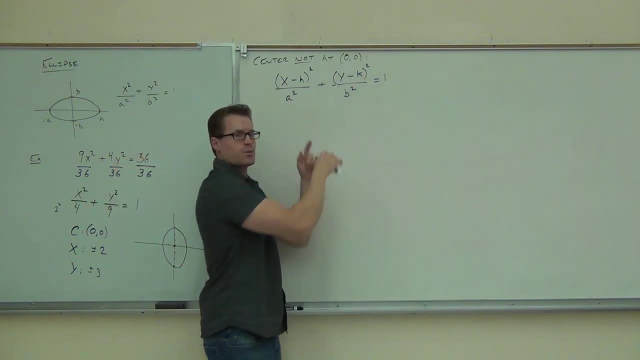 That's what we talked about this whole time. right, If these numbers are the same, we still get a circle. Even like that, it's still a circle, So our ellipses are just spread out circles. of course, but now that we have this x minus h, y minus k idea, 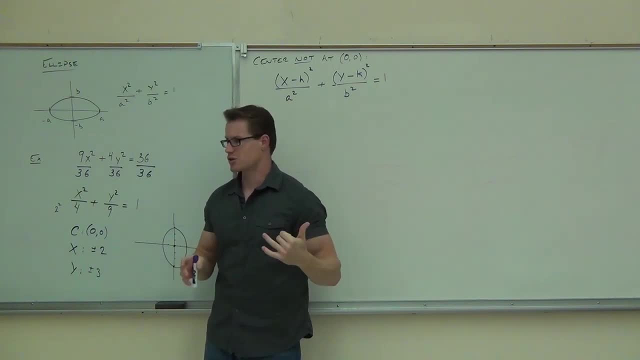 that's the shifting, just like we had with the circles in the last section. You guys seeing the similarity between those two things? All right, Let's see if we can shift that around, Since this is pretty much very similar to a circle. 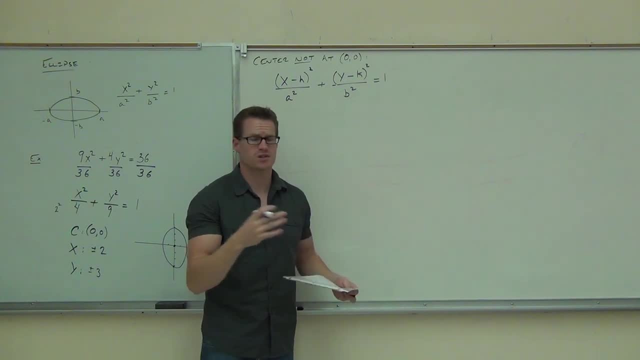 since a circle is a type of ellipse. basically, a circle is just a special ellipse. A circle is a special ellipse where you have the numbers that are the same. You guys notice that that is a circle, right? So a circle is a type of ellipse and an ellipse is not a type of circle. 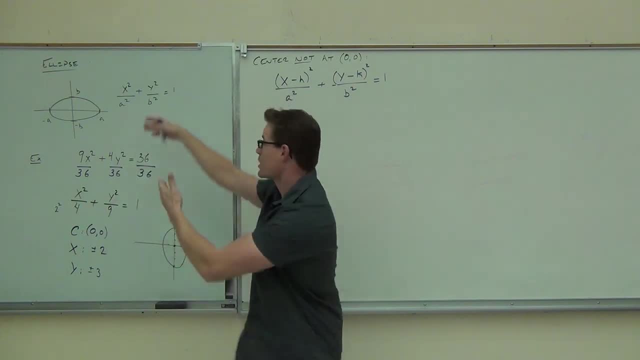 If you divide it by numbers that are different, I don't have a circle anymore. I have an ellipse. 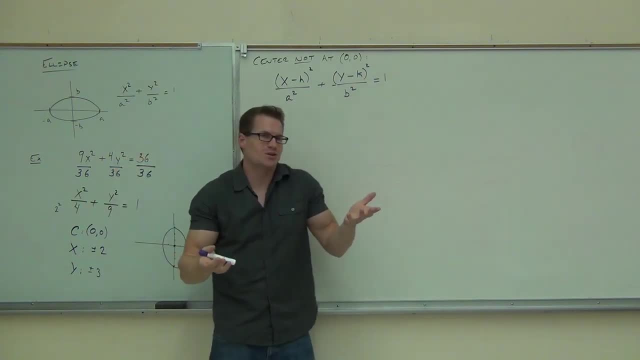 That's what we talked about this whole time, right? If these numbers are the same, we still get a circle. Even like that, it's still a circle. So our ellipses are just spread out circles, of course. 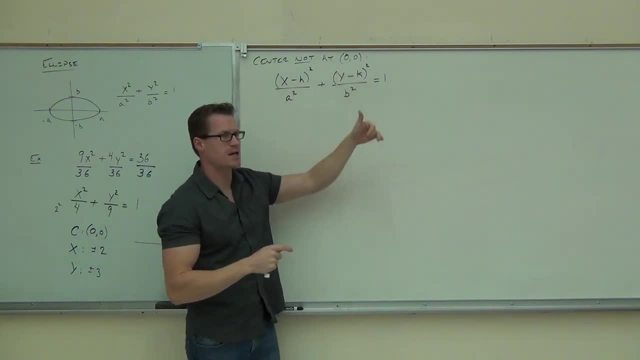 But now that we have this x minus h, y minus k idea, that's the shifting, just like we had with the circles in the last section. You guys seeing the similarity between those two things? All right. 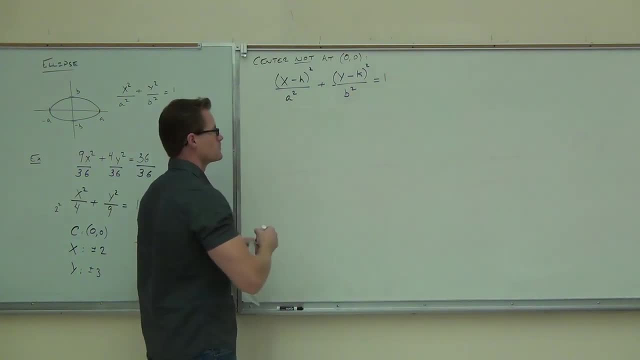 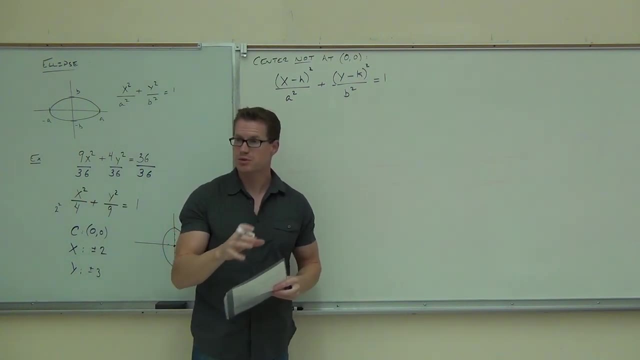 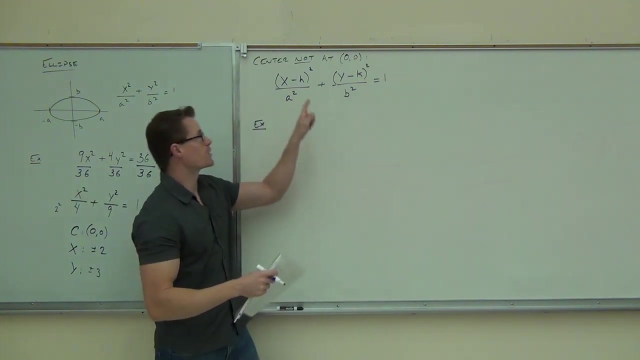 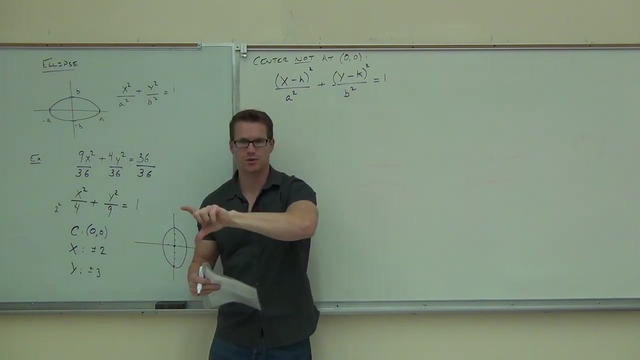 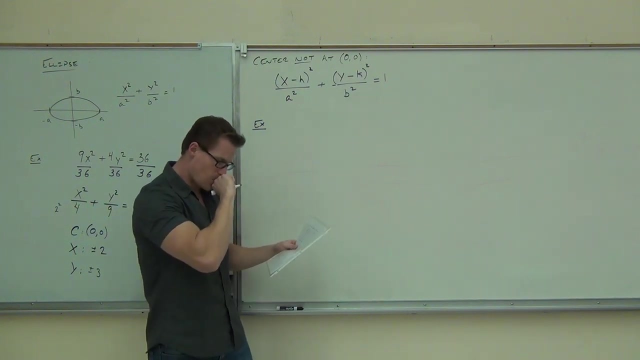 Let's see if we can shift that around. Since this is pretty much very similar to a circle, since a circle is a type of ellipse, basically, a circle is just a special ellipse. A circle is a special ellipse where you have the numbers that are the same. You guys notice that that is a circle, right? So a circle is a type of ellipse. And an ellipse is not a type of circle. A circle is a special type of ellipse, just where you're spread out in the same units in different directions. 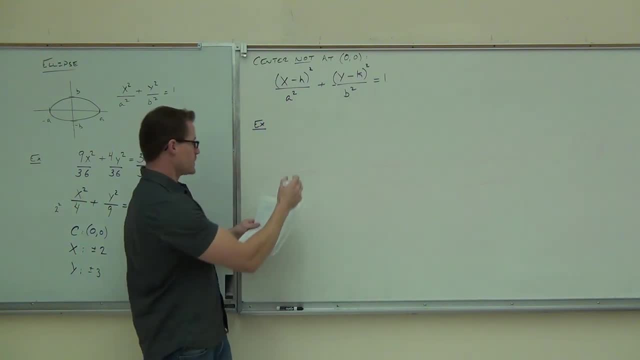 Excuse me. So let's see if we can go ahead and do this here. 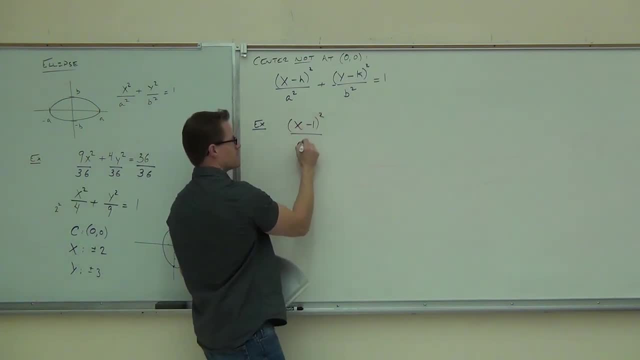 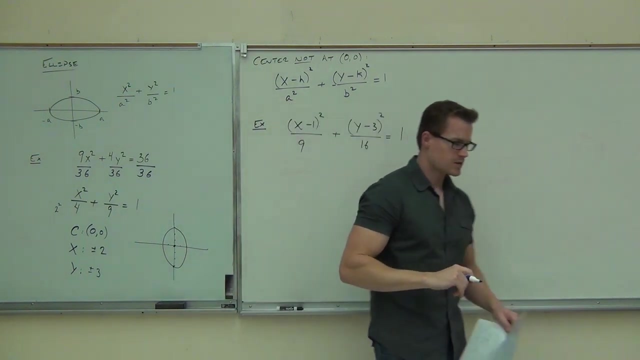 How about x minus 1 squared over 9. So since circles are types of ellipses, what we learned for circles really does apply for ellipses. 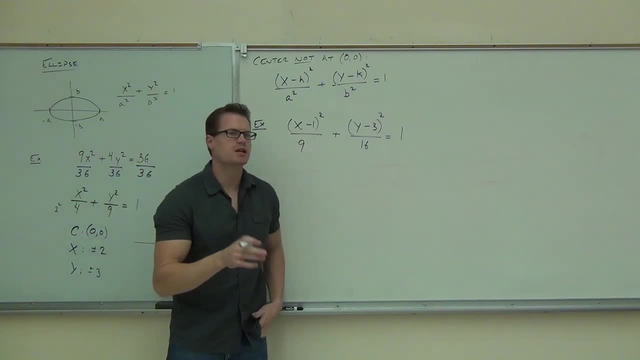 Firstly, again, you need to be able to determine what shape we have. Is it a parabola? No. Man, this looks nothing like a parabola. Parabolas don't have anything with y squared. Is it a circle or an ellipse? Ellipse. 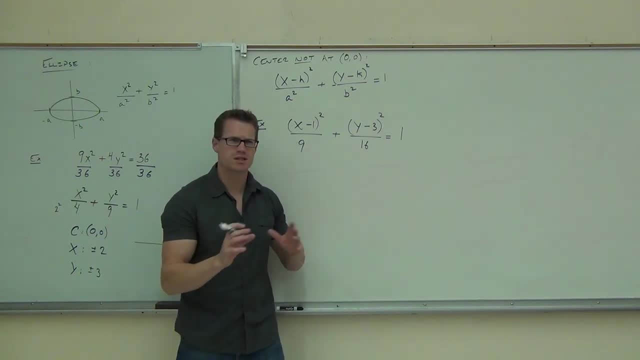 How can you tell the difference, again, between a circle and an ellipse? What's the difference there? It's bigger in one direction. Okay. So which direction is this going to be bigger in? The x direction or the y direction? The y direction. 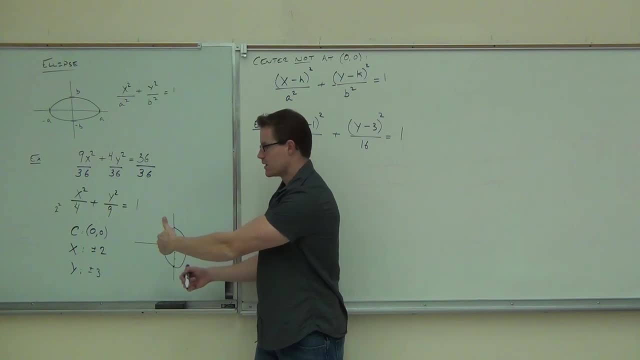 So it's going to look kind of similar to that one, right? Different numbers. We're not going to have 2 and 3 anymore. We'll probably have 3 and 4. We can see that already, hopefully. 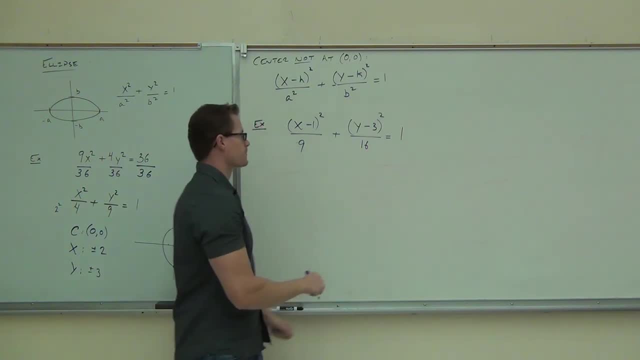 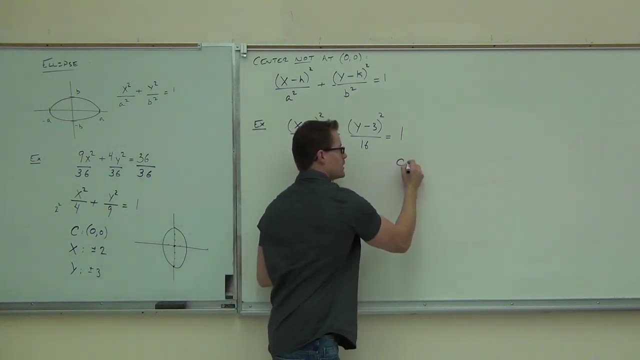 But it's going to stretch out longer along the y axis. Now, let's look at our center. Is our center at 0, 0 still? No. 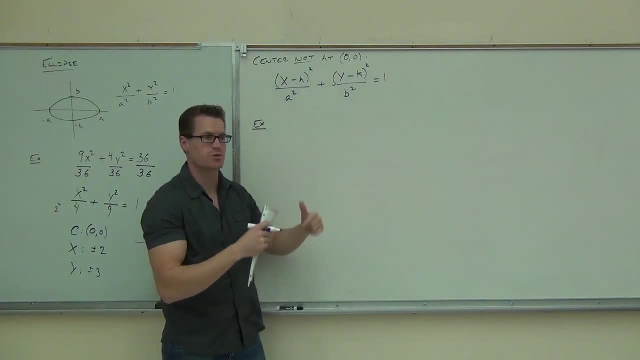 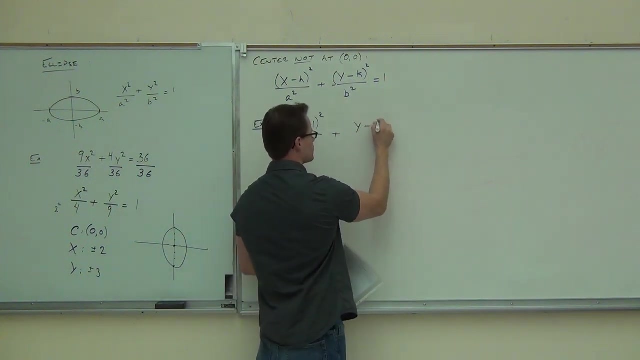 A circle is a special type of ellipse, just where you're spread out in the same units in different directions. Excuse me, So let's see if we can go ahead and do this here. How about x minus 1 squared? So, since circles are types of ellipses, 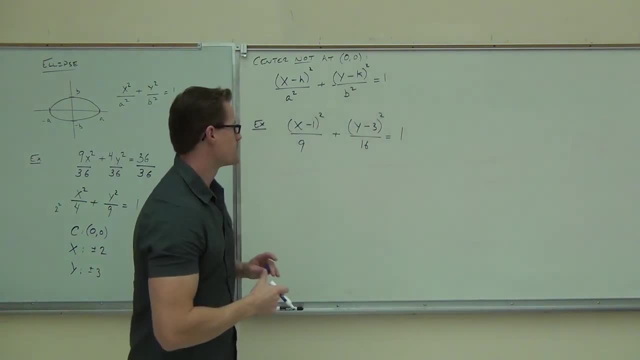 what we learned for circles really does apply for ellipses. First thing we're going to do is we're going to have to do a little bit more analysis. So essentially, again, you need to be able to determine what shape we have. 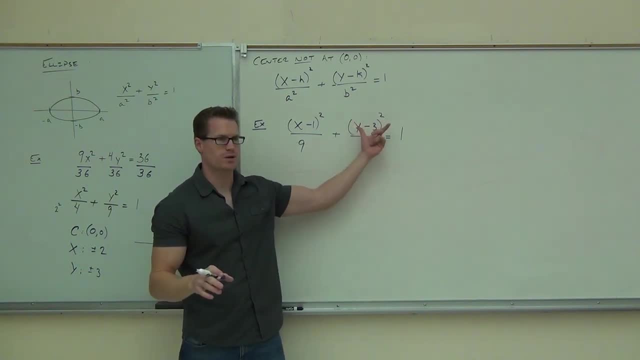 Is it a parabola? No Man, this looks nothing like a parabola. Parabolas don't have anything with y squared. Is it a circle or an ellipse- Ellipse? How can you tell the difference again between a circle and an ellipse? 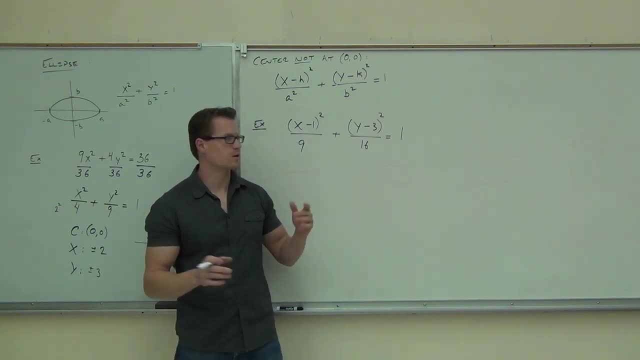 What's the difference there? Bigger in one direction. Okay, So which direction is this going to be bigger in? The x direction or the y direction? Y direction, So it's going to look kind of similar to that one, right? 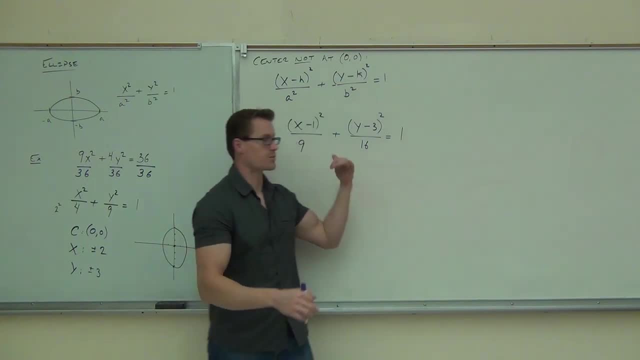 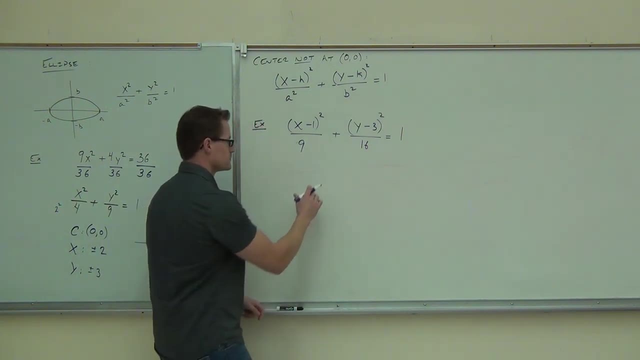 Different numbers. We're not going to have two and three anymore. We'll probably have three and four. We can see that already, hopefully. But it's going to be stretched out longer along the y-axis. Now let's look at our center. 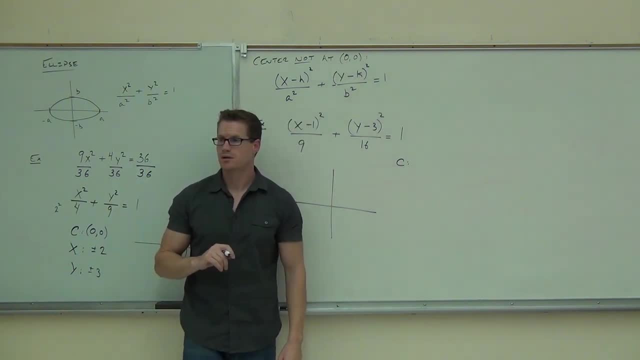 Is our center at 0, 0? still No, What do you think? Is our center at 0, 0? No, Can you tell me where it's shifting? What does this mean? Let's refresh our memories from yesterday. 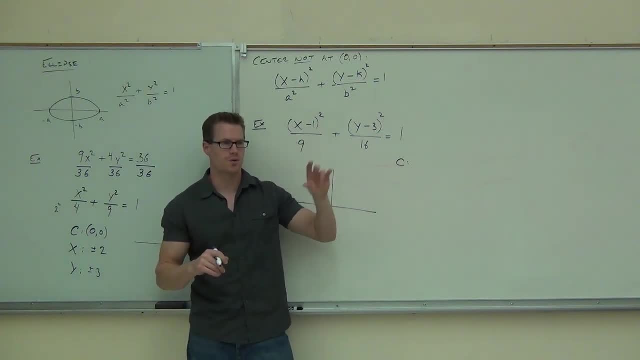 What's that minus 1 mean? Does that mean up down, left or right? Right It means right, Good. It's associated with our x, So that means in an x direction. I'm going to be going either left or right. 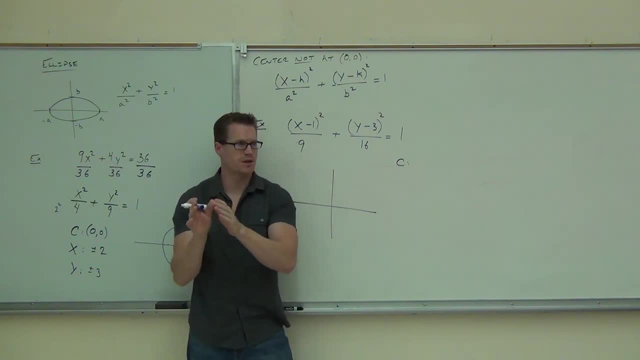 Here, minus means to the right and plus means to the left. It was that opposite idea of how your mind wants to think. right, If you have that minus 1, it's not left 1.. It's right 1.. 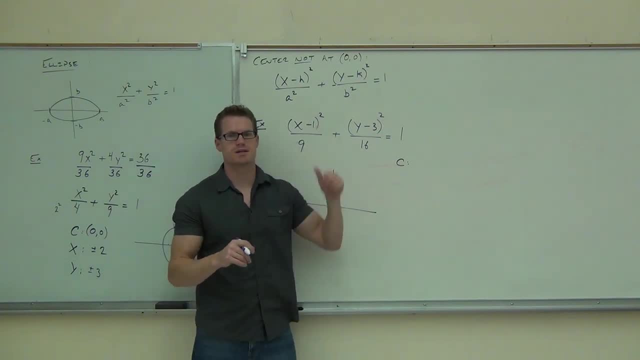 Let's refresh our memories from yesterday. What's that minus 1 mean? Does that mean up, down, left, or right? Right. It means right. Good. 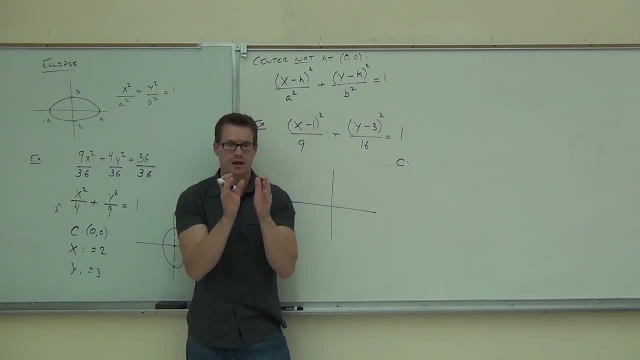 It's associated with our x. So that means in an x direction, I'm going to be going either left or right. Here, minus means to the right and plus means to the left. It was that opposite idea of how your mind wants to think, right? If you have that minus 1, it's not left 1. It's right 1. So this means I'm going to shift it to the right 1 spot. 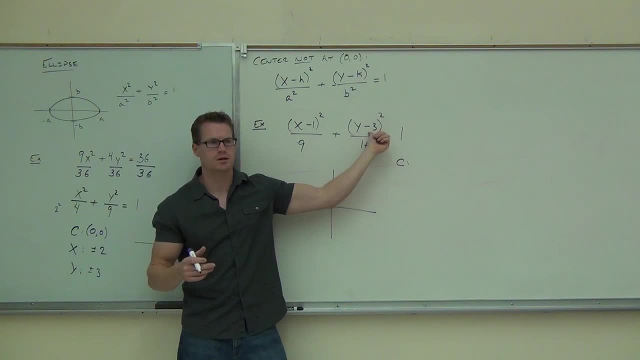 Also, it means am I going to go up or down here? What do you think? Up 1. I'm going to go up 3. Yeah. 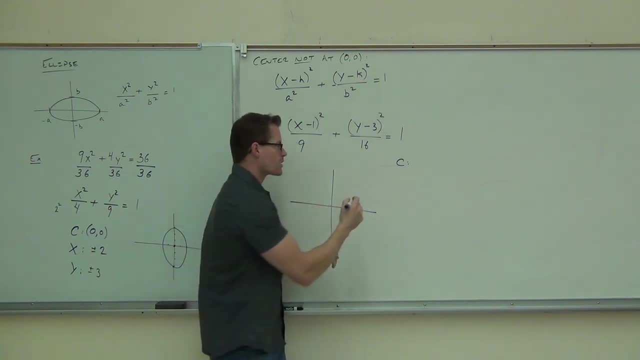 In parentheses, any time you see graphing in parentheses, it's the opposite of what you want to say. So our center here, that means 1. That means 3. Our center's at 1, 3. 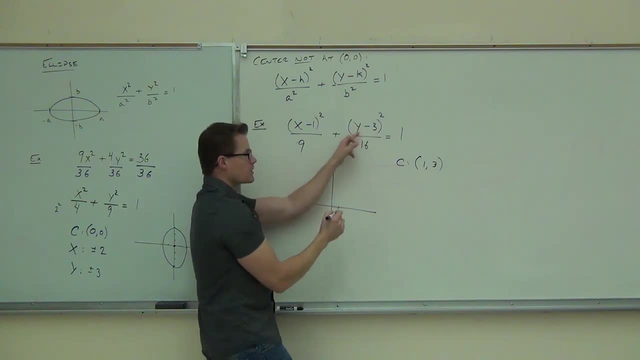 And if we look at that shifting, it says go to the right 1, go up 3, put a spot, put a point. 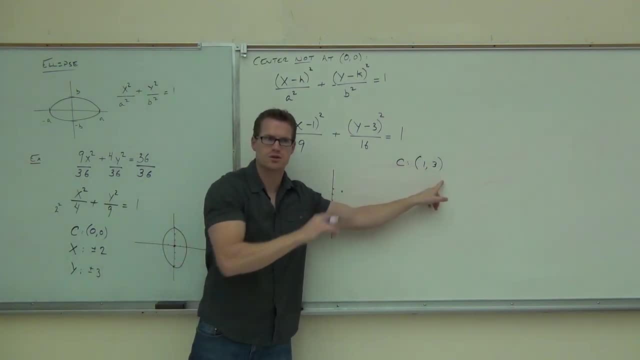 Hey, that's exactly what we found out according to the formula this was going to be, 1, 3. Now, the question is, can you use this idea to graph the rest of your ellipse from these numbers? 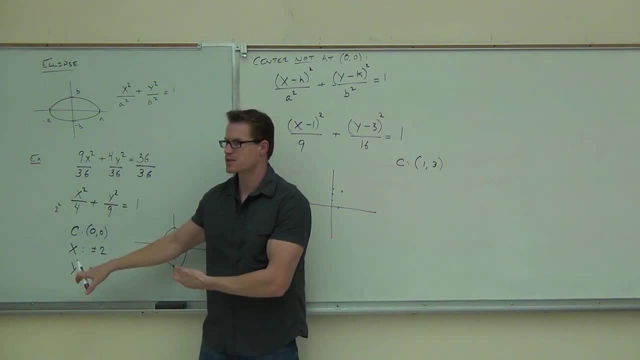 Now, of course, the reason why I got away from the words x-intersection, y-intercept, and y-intercept is because if you think about this as x-intercept, y-intercept, well, that means you're going from the origin. Are we going from the origin here? No. 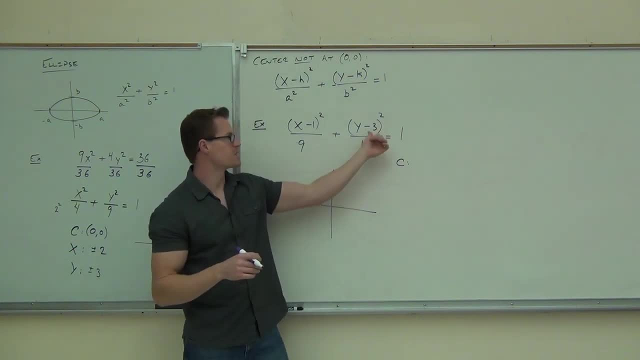 So this means I'm going to shift it to the right 1 spot. Also, it means: am I going to go up or down here? What do you think? Up 1.. I'm going to go up 3.. Yeah, In parentheses, any time you see graphing in parentheses, it's the opposite of what you want to say. it is. 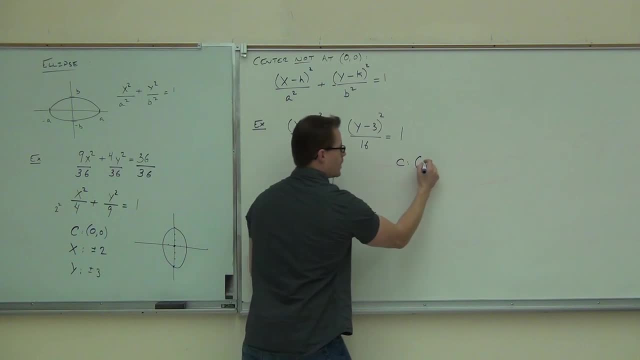 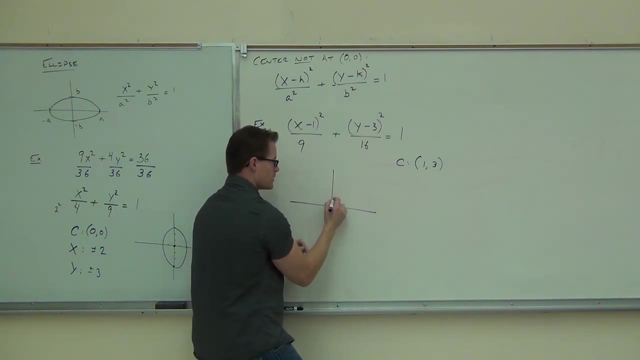 So our center here That means 1.. That means 3.. Our center's at 1,, 3.. And if we look at that shifting, it says: go to the right 1,, go up 3,, put a spot, put a point. 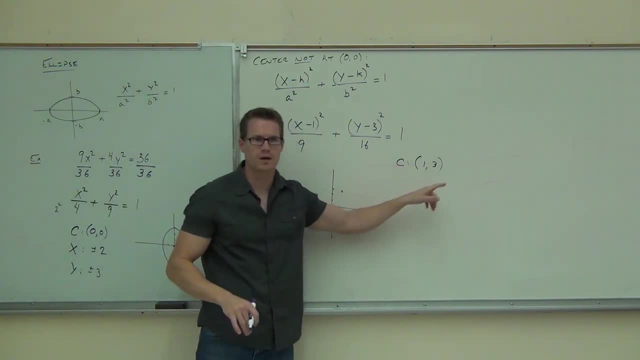 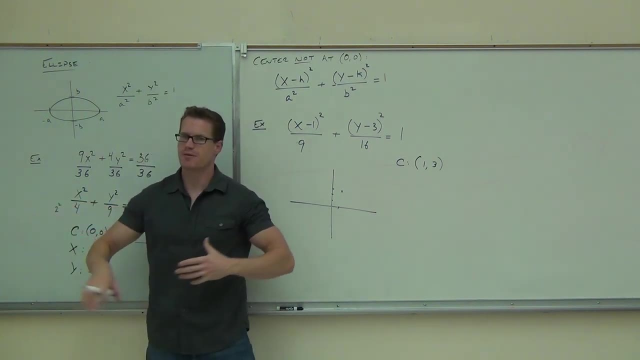 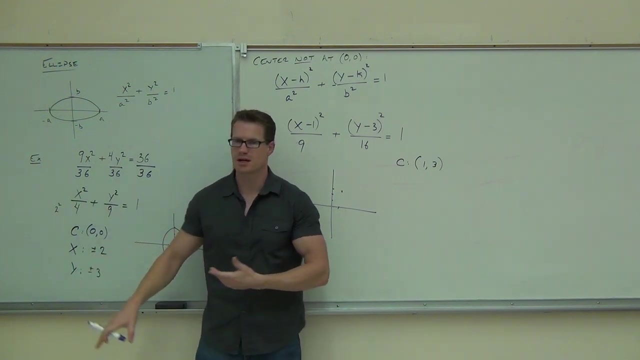 Hey, that's exactly what we found out. according to the formula, this was going to be 1, 3.. Now the question is: can you use this idea to graph the rest of your ellipse from these numbers? Now, of course, the reason why I got away from the words x-intercept and y-intercept is because 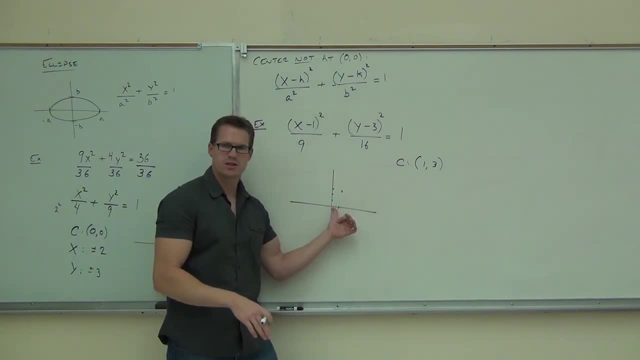 if you think about this as x-intercept, y-intercept, well, that means you're going from the origin. Are we going from the origin here? No, No, we're going from that point now. We're going from our center, just like we did with our circle. 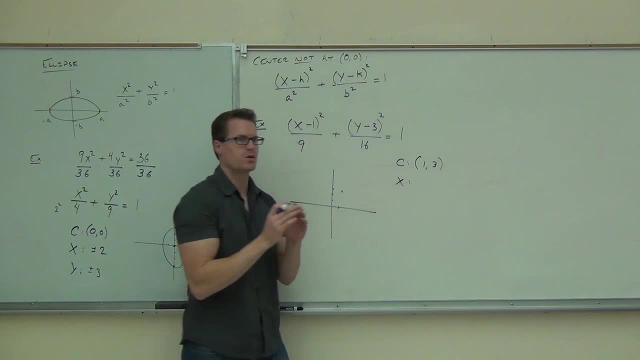 So can you tell me, along the x-direction, how far am I going? left and right? Tell me that 1 right, No, not 1 right. Along the x-direction from that center, how far am I going? 3.. 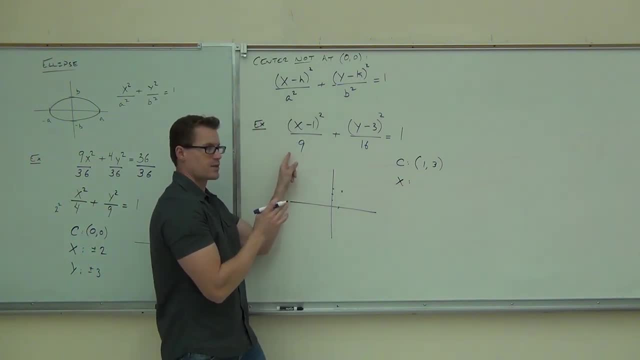 Where are you getting the number 3?? 3 squared, 3 squared. Okay. so right there, that tells us: take the square root of that. We're going plus, We're going minus 3 from wherever our center is. 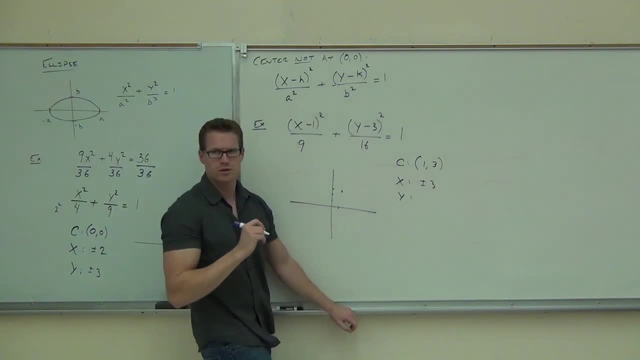 How about along the y-direction folks? How much? 4.. Yeah, Okay, quick show of hands. How many people feel okay finding the center of this thing? Good, Yes, no over here. Yes, Okay, good, How about this x along the x-direction? 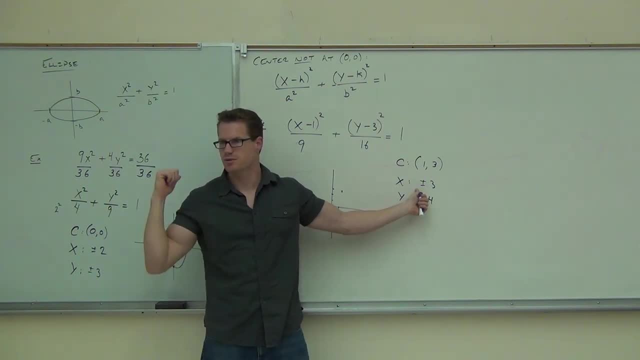 Are you okay finding that plus and minus 3?? Again, it's very, very similar to our ideas, with the ellipse not centered, or centered at 0, 0. And then the plus or minus 4, that's coming from our 16.. 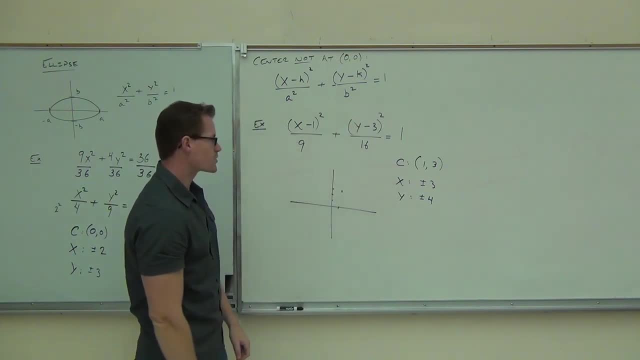 We take a square root of that. Of course we're going in both directions there. So from our center we're going to go not from the origin, but from the center, right 3, left 3, up 4, down 4.. No, we're going from that point now. 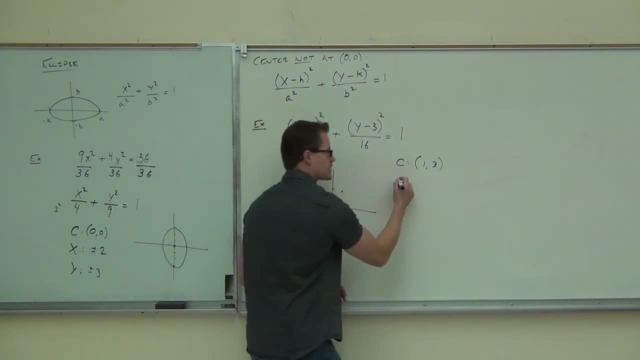 We're going from our center, just like we did with our circle. So can you tell me, along the x-direction, how far am I going left and right? Tell me that. 1 right. No, not 1 right. 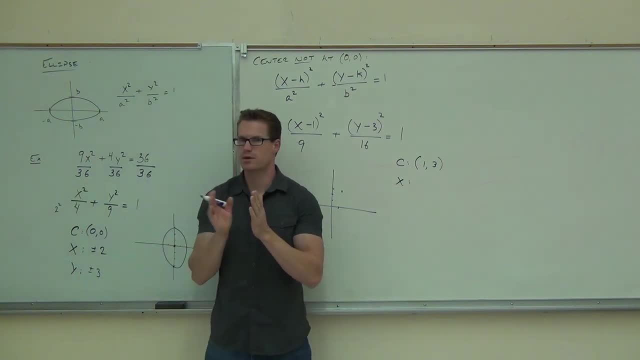 Along the x-direction, from that center, how far am I going? 3. Where are you getting the number 3? From 3 squared to 9. 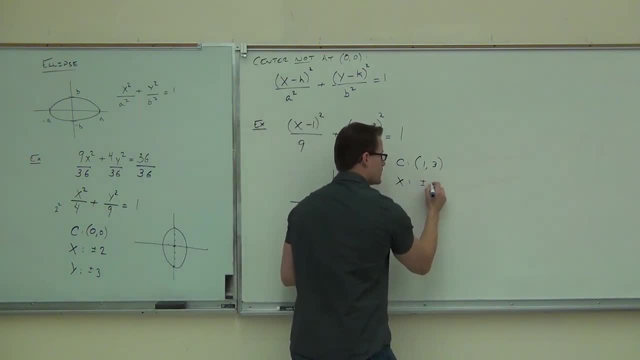 Okay. That tells us, take the square root of that. We're going plus and minus 3 from wherever our center is. How about along the y-direction, folks? How much? 4. Yeah. 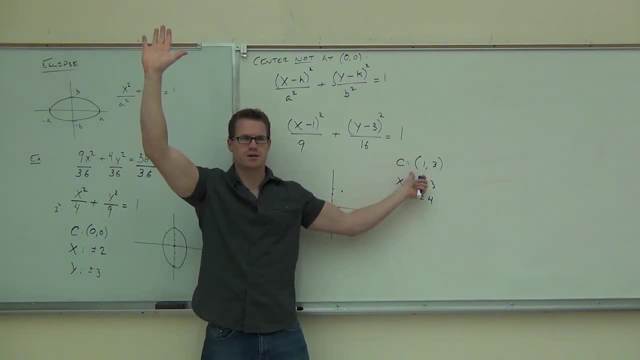 Okay, quick show of hands. How many people feel okay finding the center of this thing? Good. 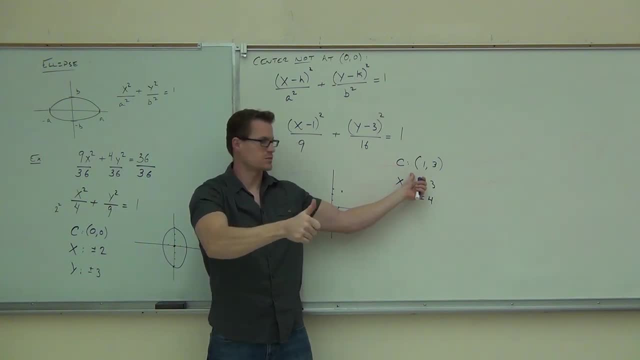 Yes, no over here? Yes? Okay, good. 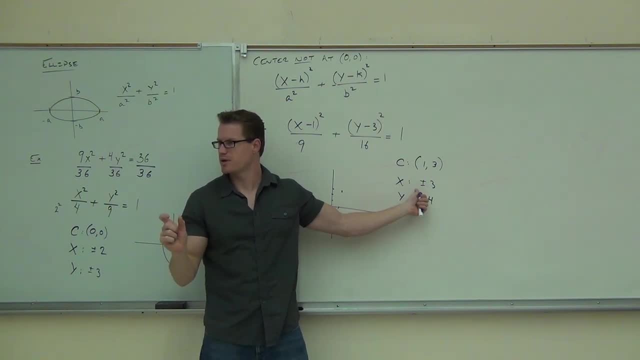 How about this x, along the x-direction? Are you okay finding that plus and minus 3? Again, it's very, very similar to our ideas. 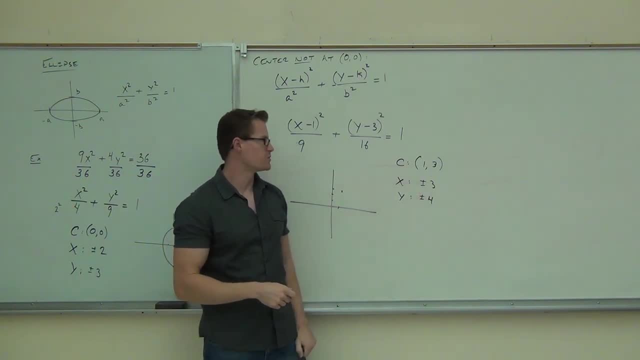 This is the center of the ellipse not centered at, or centered at 0, 0. And then the plus or minus 4, that's coming from our 16. We take a square root of that. 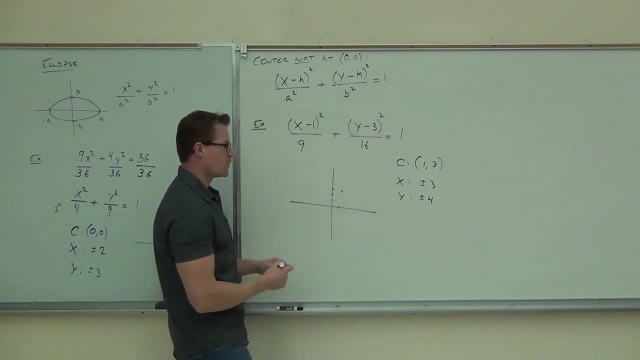 Of course, we're going in both directions there. So, from our center, we're going to go, not from the origin, but from the center, right 3, left 3, up 4, down 4, just like a circle that's not centered at the origin. That's kind of how we do that. 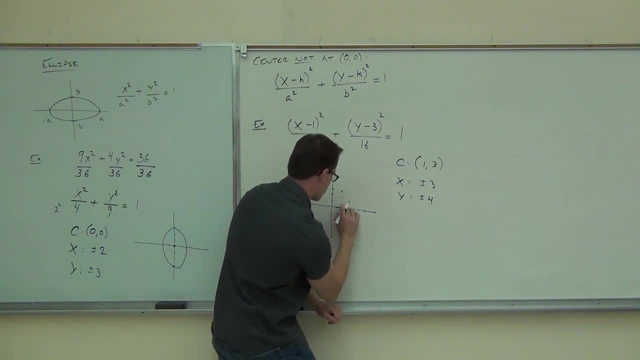 I think my points are a little off, aren't they? 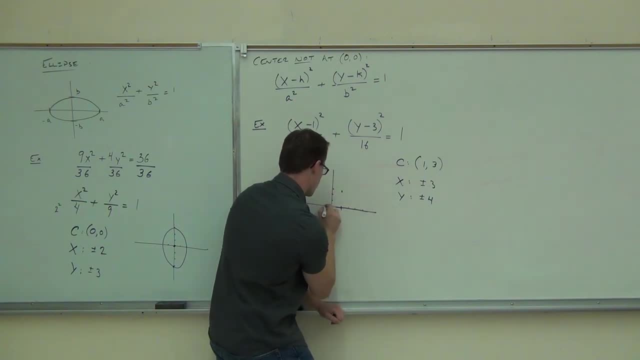 Okay, so, from not the origin, but our center, we're going to go 1, 2, 3 to the right, put a point there. We'll go 1, 2, 3 to the left, put a point there. We'll go up 4, and we'll go down 4, all based around our center. 1, 2, 3, 4. 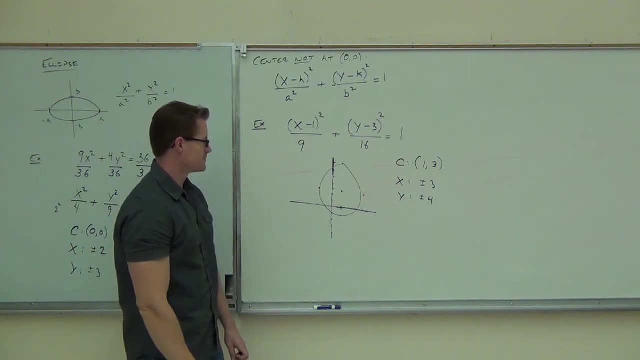 That's the worst ellipse I've ever done in my life. It looks like an A. Here's your A. It looks like a circle. 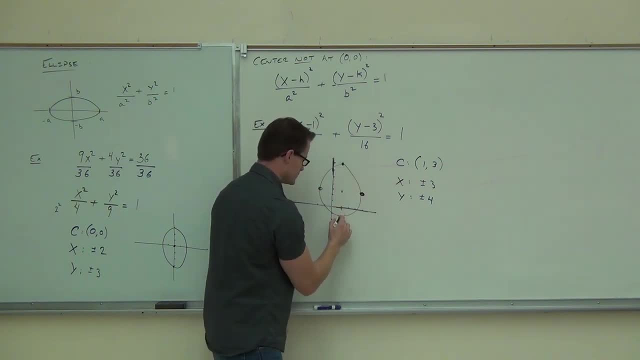 Well, I'm just making the points bigger, and cheat a little bit. It looks like a little water. It's because my graph is sucky. Sorry, my bad. Oh, it's the graph. 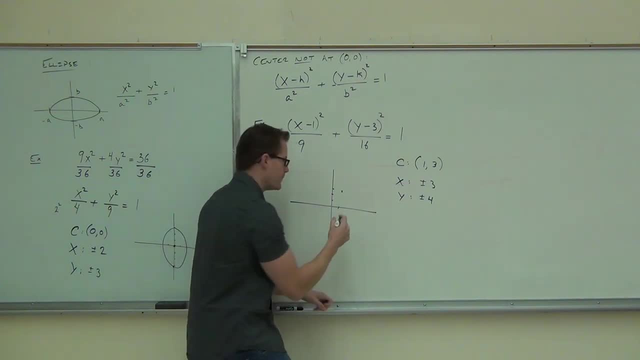 Just like a circle that's not centered at the origin. that's kind of how we do that. I think my points are a little off, aren't they? Okay, so, from not the origin but our center, we're going to go 1,, 2, 3 to the right, put a point there. 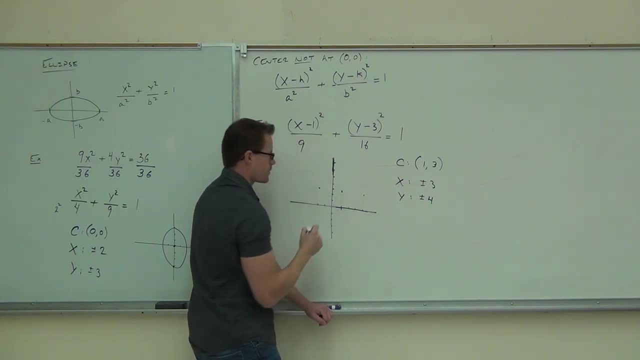 We'll go 1,, 2,, 3 to the left, put a point there, We'll go up 4, and we'll go down 4.. We're all based around our center: 1,, 2,, 3,, 4.. 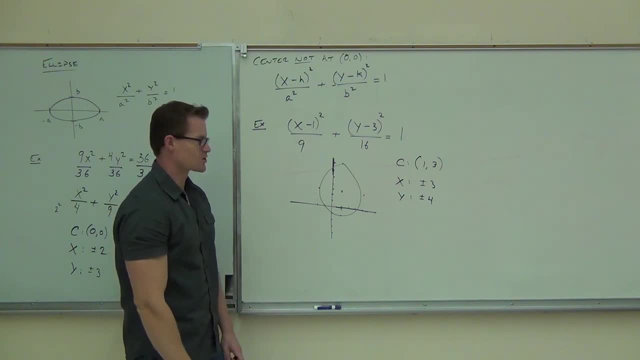 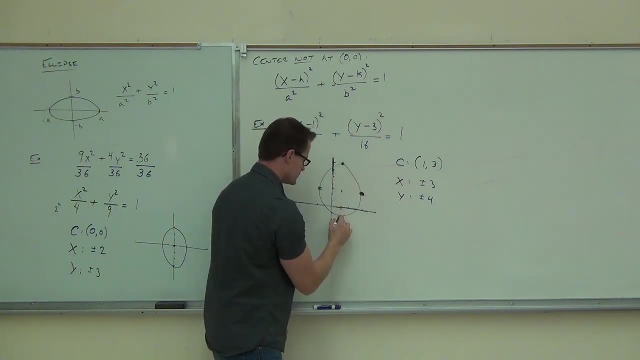 That's the worst ellipse I've ever done in my life. Looks like an A. Here's your A. That looks like a circle. I'll just make the points bigger and cheat a little bit. Looks like a little water. It's because my graph is sucky. 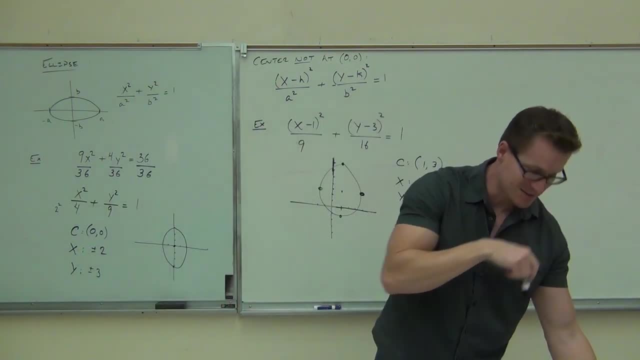 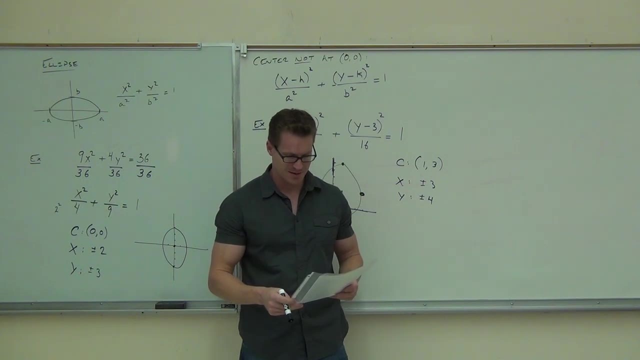 Sorry My bad. Oh, it's the graph. Yeah, it's the graph. Oh, is it me Too bad? I drank today. Man, my goodness, Shouldn't have had that bottle of vodka on the way to work. 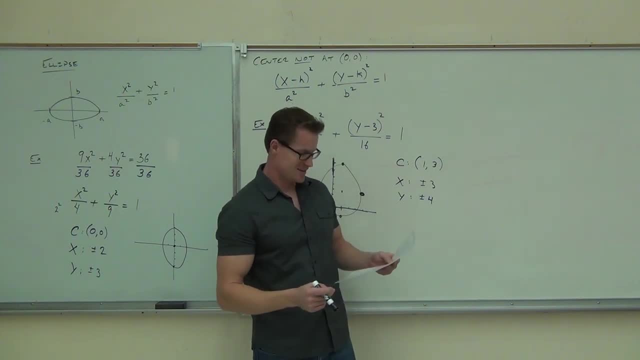 Driving the car going tonight. No, I'm just kidding. Yeah, Anyway, I want you to try one of your own. Let's go ahead and do this one. Make sure you are able to find the center, Make sure you're able to find the X and the Y direction for your ellipses. 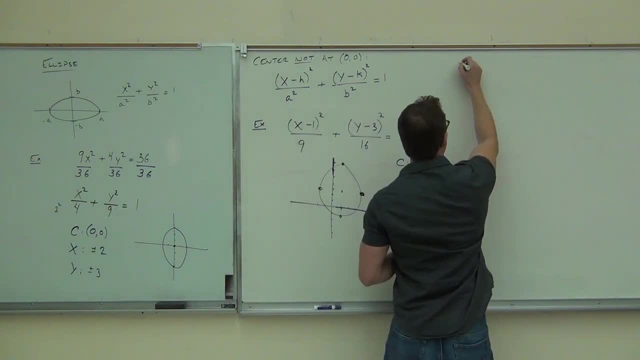 Be able to determine that it is an ellipse and graph it incorrectly. We'll see if it works out. I'll get some help. Okay, I like the idea. I'm not sure I can do anything about that, But I'll just go ahead and try it. 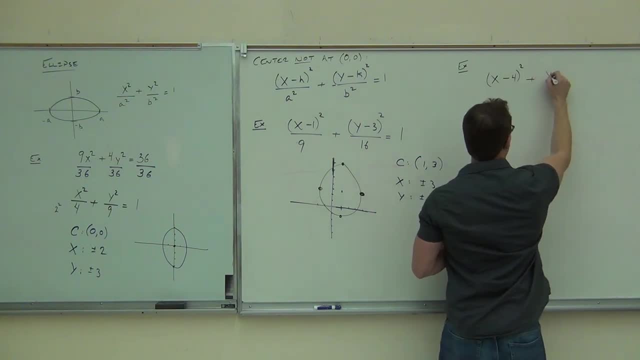 Okay, There we go, There you go. Yes, Now it should work All right. So you keep the X and the Y direction and you're done. What's the other one? That's the straight line, That's the X and the Y direction. 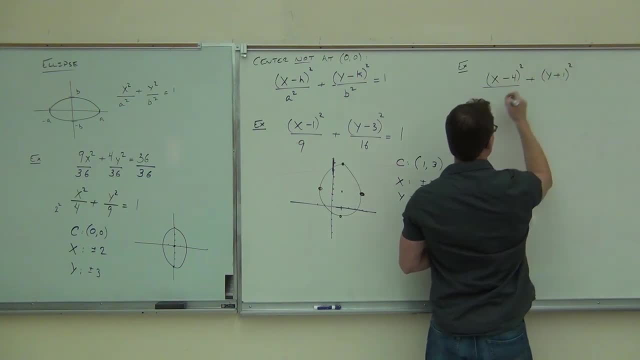 And you're done. And that's the straight line, And that's the one you're doing, And you're done. This is the correct distance of the curve. You're done. That's the perfect distance. That's the perfect distance of the curve. 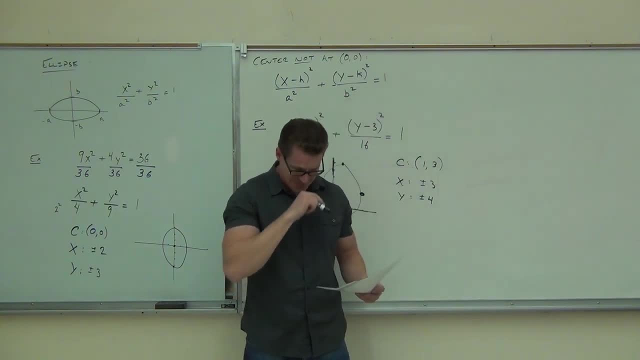 Yeah, it's the graph. It's not, oh, is it me? 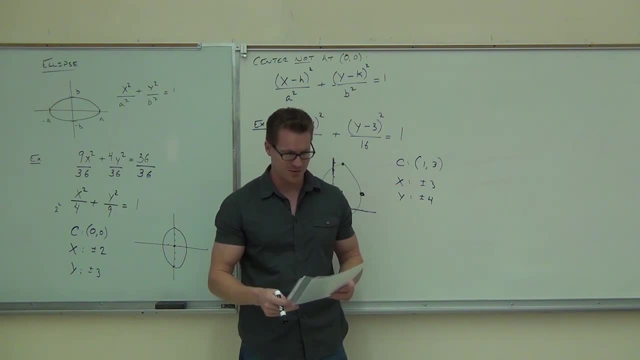 Too bad I drank today. Man, my goodness, shouldn't have had that bottle of vodka on the way to work. Driving the car going tonight. No, I'm just kidding. 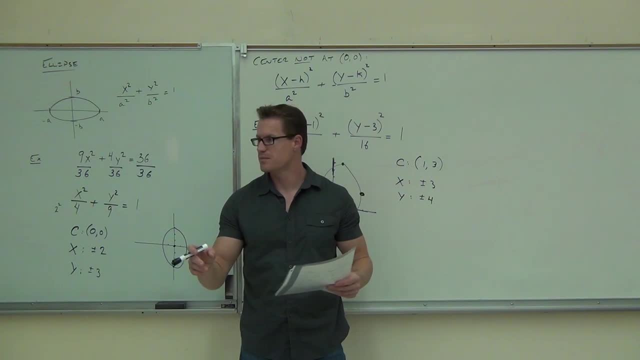 Anyway, I want you to try one of your own. Let's go ahead and do this one. Make sure you are able to find the center. 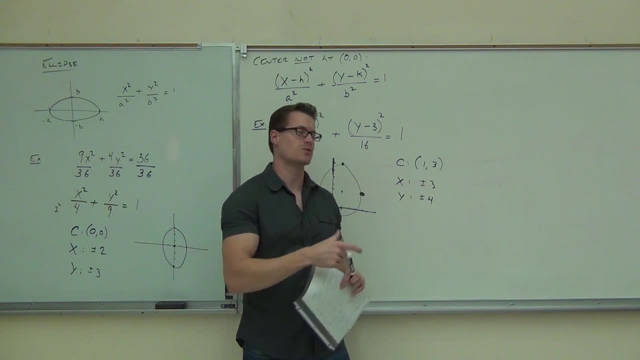 Make sure you're able to find the X and the Y direction for your ellipses. Be able to determine that it is an ellipse and graph it incorrectly. 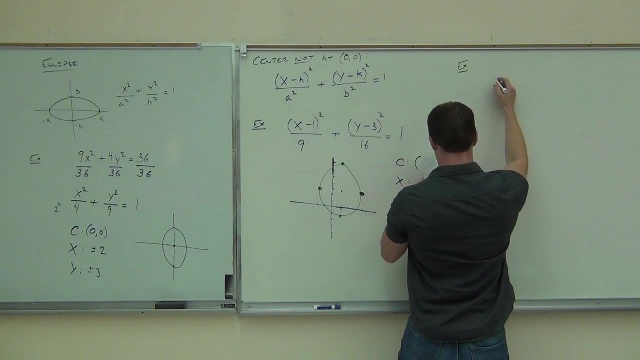 Well, I'm not sure about that. Actually, it's just one of those, like, individual actions. 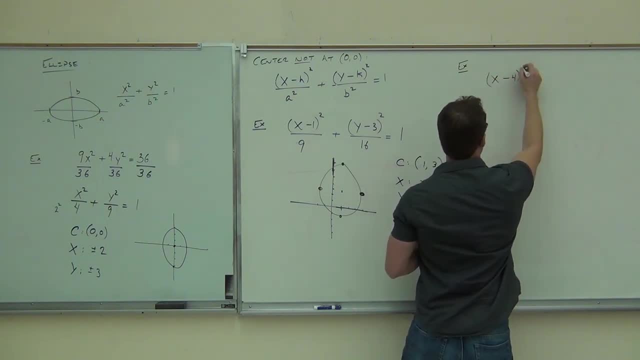 But so long as it's a thing, careful, careful, careful, careful, careful, careful. It's not going to work for you. Yeah, well, it's not going to work for me. No, it's not going to work for me. Well, give me what you have. I'll give you what you have. Really, you have it, but I'm going to keep going. Wait. I'm trying to get back into it. 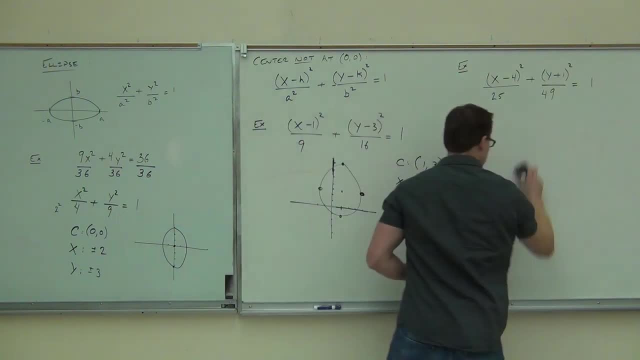 Look, I'm out of my mind. You don't have to be. 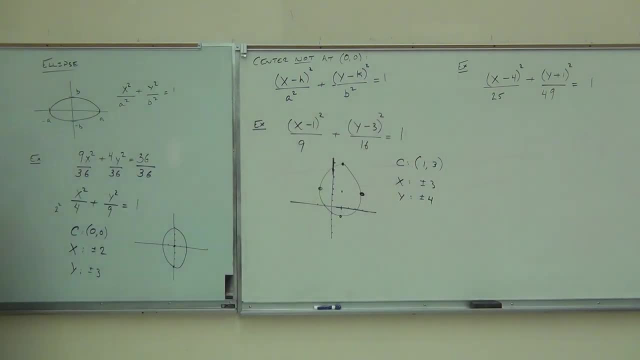 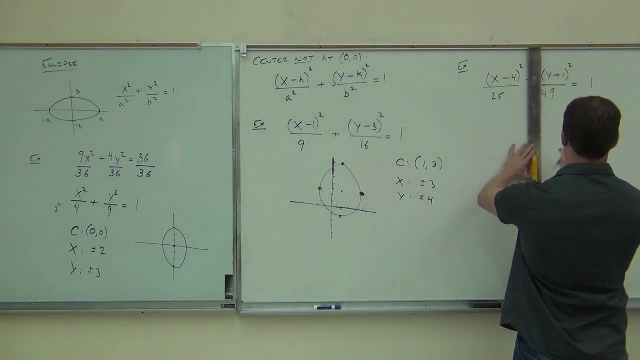 You're going to make it work. Don't bag up my grass, I still have grades to give, I'm the grader. 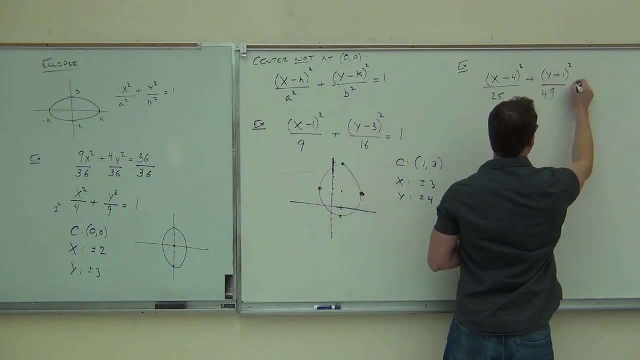 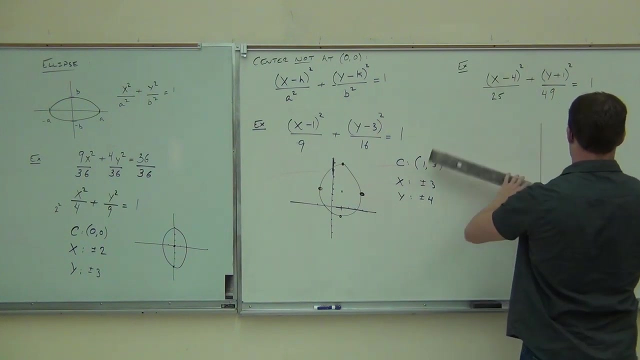 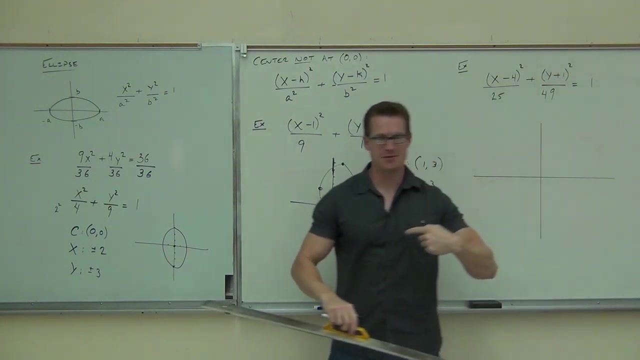 That's the perfect distance of the curve. Okay, Now you're done, I'll fix this thing right now. That's right. I'm not messing around today. Don't bag up my grass. I still have grades to give. I'm the grader. 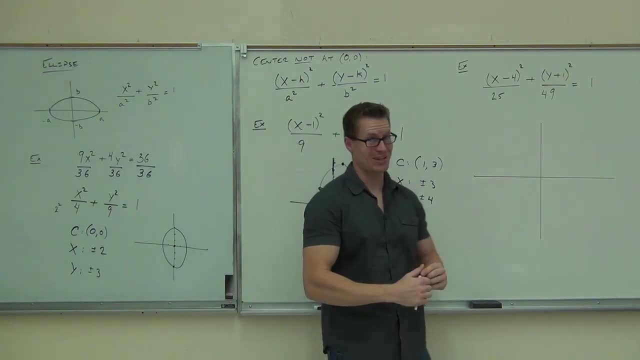 You can't be unfair. Oh, yes, I can be unfair. Yes, I literally can. You're recording this. Yes, You can delete it. I can tell you right now I can be unfair. No, I probably can't. 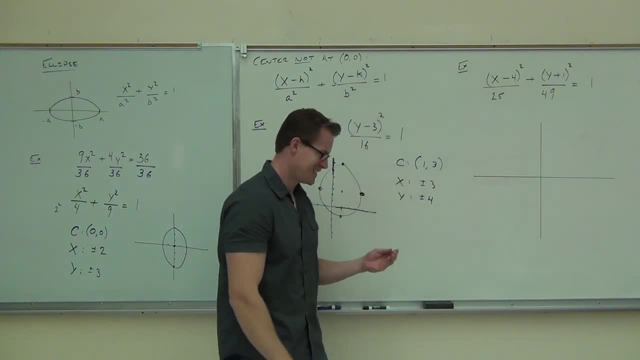 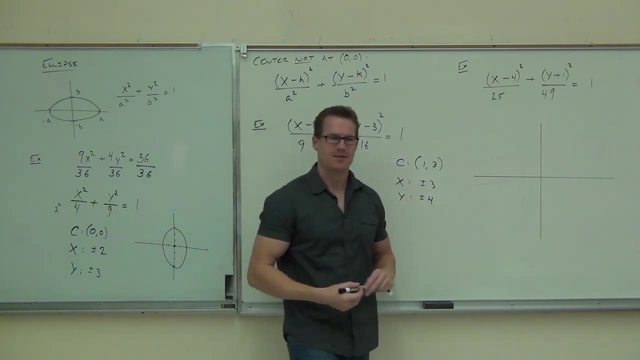 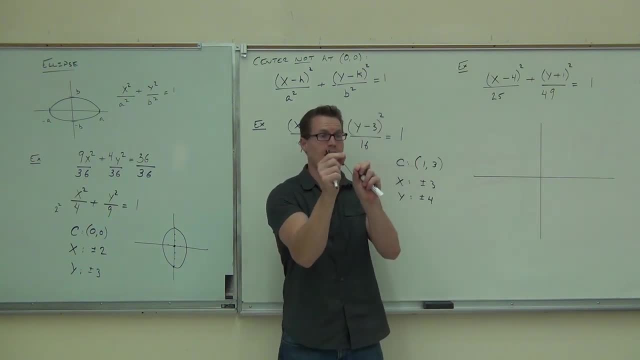 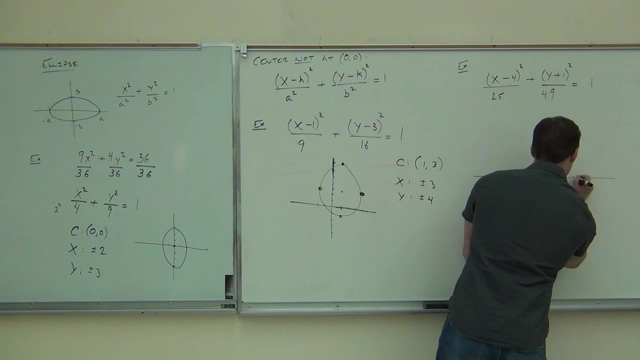 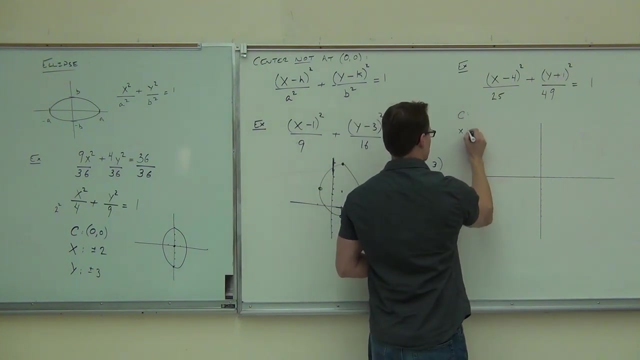 Go ahead and finish up your graphs here. I do want to get graphs. by the way, graph paper will really help you, because you're able to count on graph paper, those little dots, Huh. Okay, ladies and gentlemen, why don't you tell me where is someone on the right-hand? 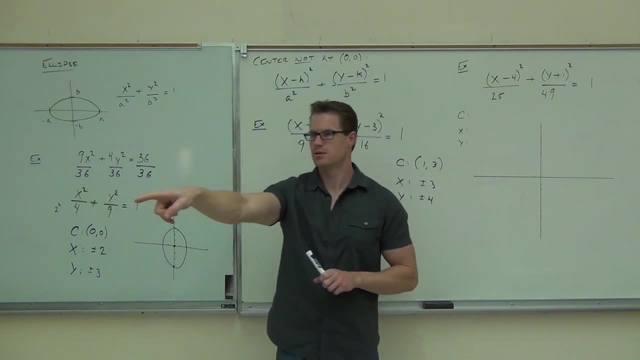 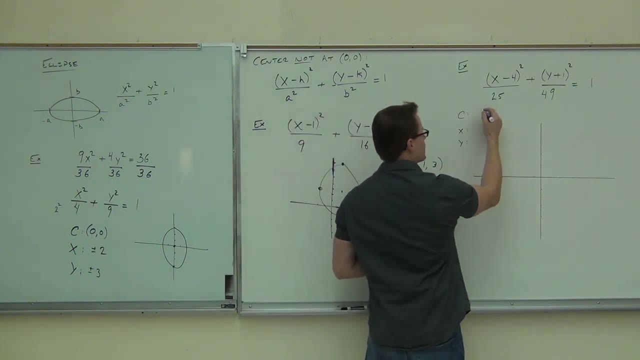 side of the room. Where is our center at, please? Center Four negative one. Four negative one. How we got that? Minus means to the right, four, plus means down one. So we have right here four comma negative one. raise your hand if you got four negative. 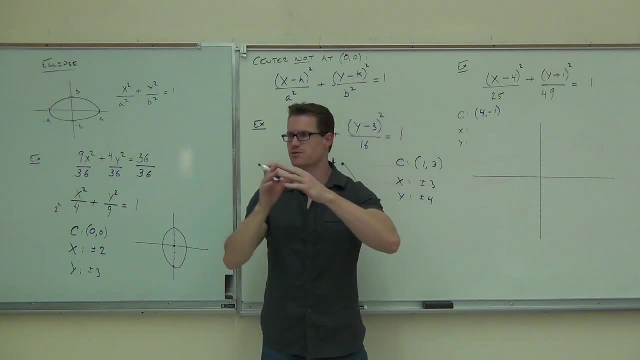 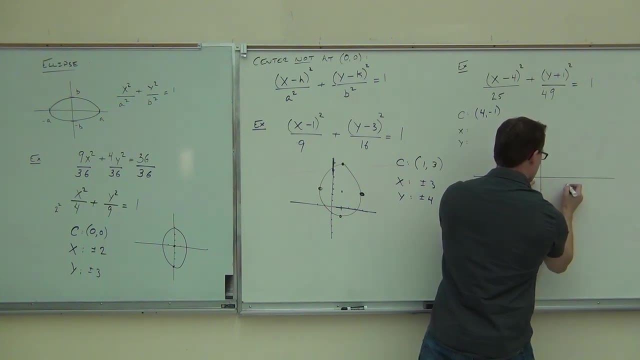 one. Very good, We plot that on our graph first, and then we use the distance spread along x and the distance spread along y to draw our ellipse. So four, one, one, two, three, four down negative one. How much are we going to go to the right and left? You can't be unfair. 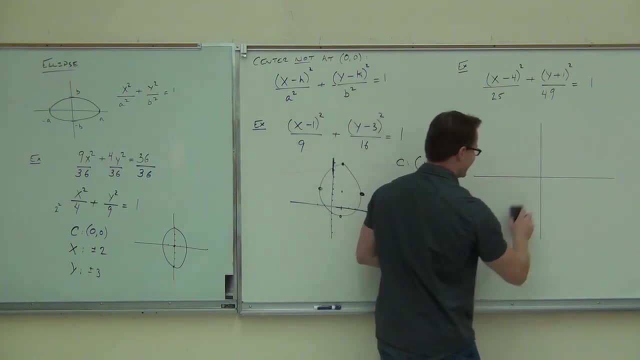 Oh, yes I can be unfair. Yes, I literally can. You're recording this. 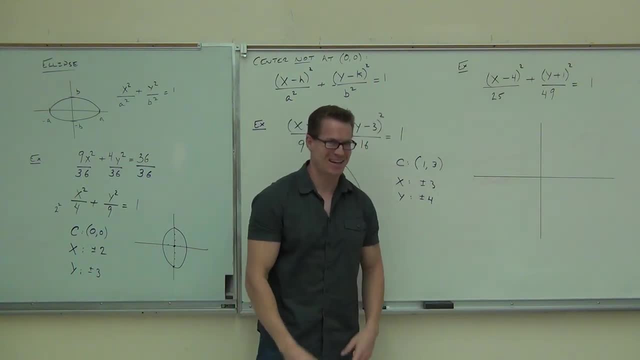 Yes. You can delete it. 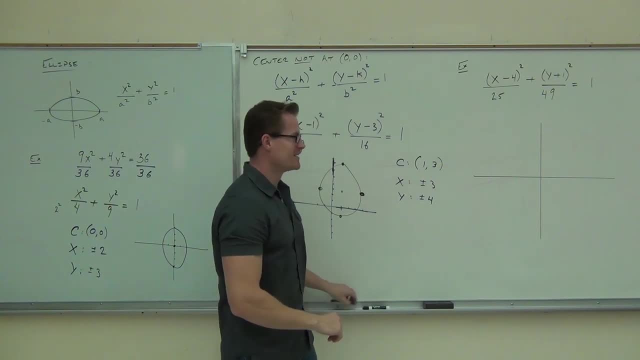 I can tell you right now, I can be unfair. No, I probably won't be unfair. Go ahead and finish up your graphs here. I do want good graphs. 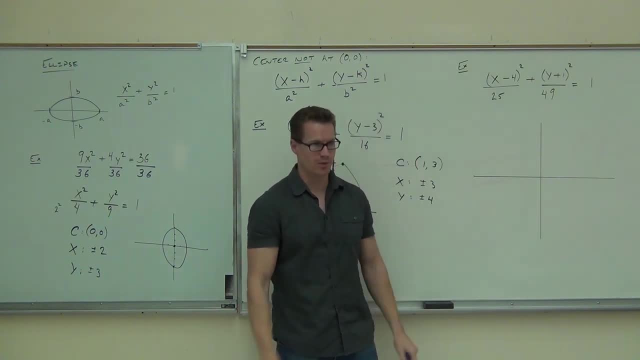 By the way, graph paper will really help you because you're able to count on graph paper, those little dots. And graphs can be great. Thank you. 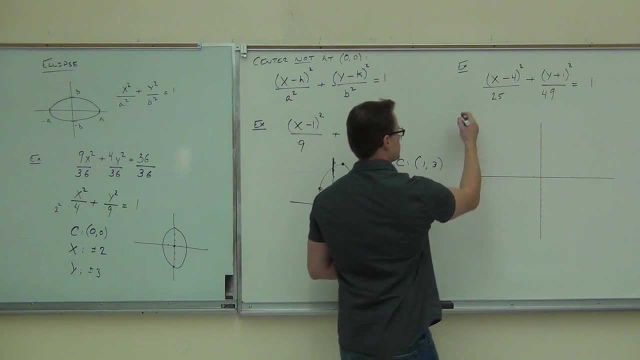 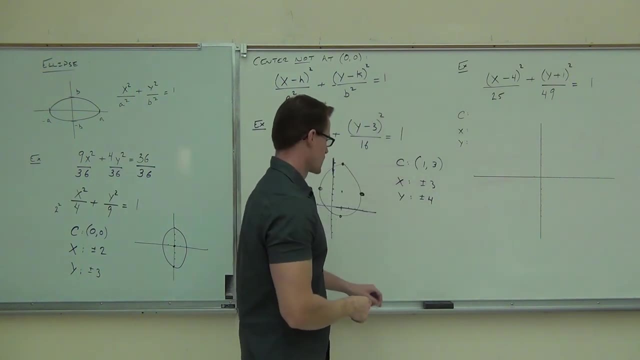 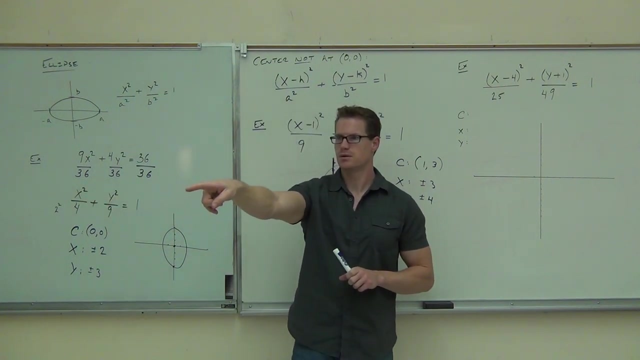 Okay, ladies and gentlemen, why don't you tell me, where is someone on the right-hand side of the room? Where is our center at, please? Center? Four, negative one. Four, negative one. 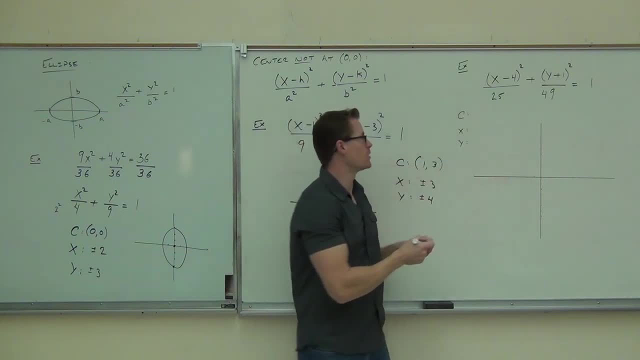 How we got that? Minus means to the right four, plus means down one. 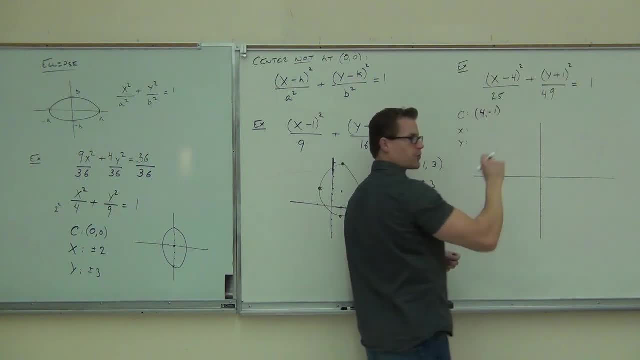 So we have right here four, comma, negative one, raise your hand if you got four, negative one. 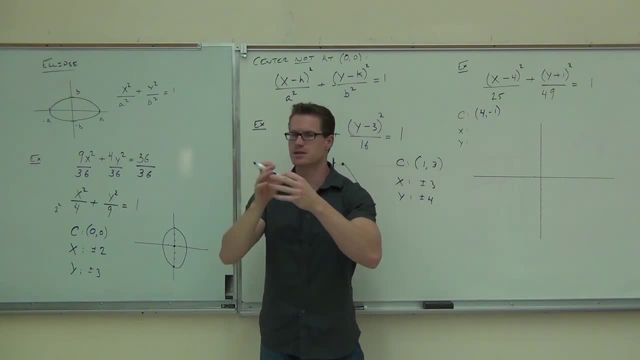 We got that on our graph first, and then we used the distance spread along x and the distance spread along y to draw our ellipse. 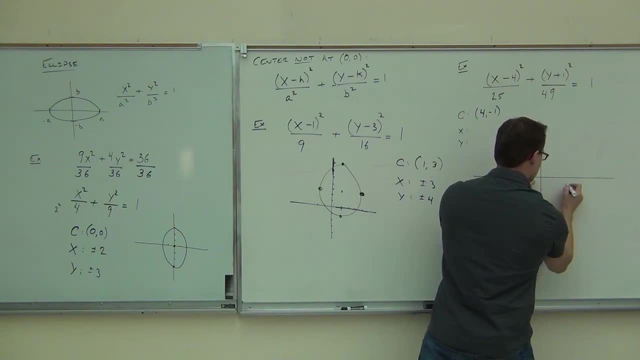 So four, one, one, two, three, four, down negative one. How much are we going to go to the right and left? 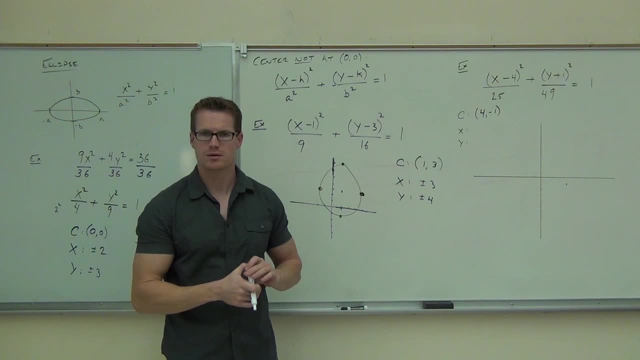 Is it 25, five, seven, or 49? How much? Twenty-five. 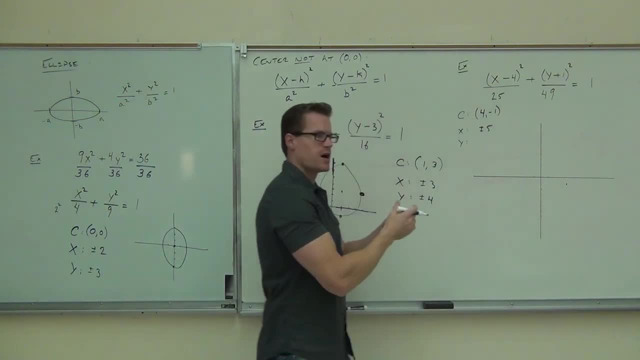 Sure. Plus or minus five in either direction here. 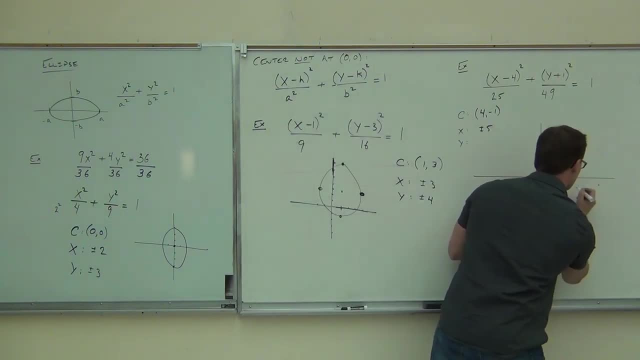 One, two, three, four, five. Twenty-five. 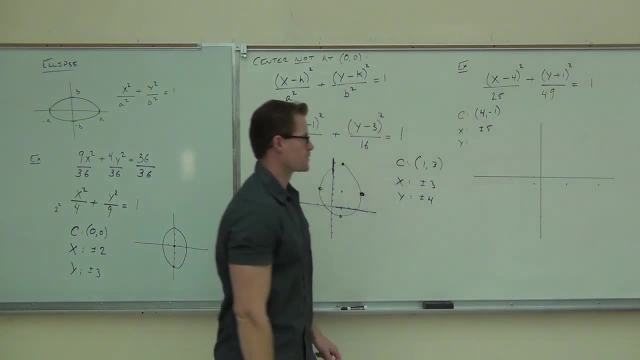 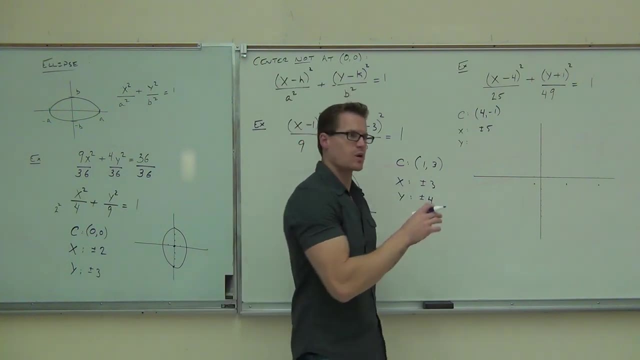 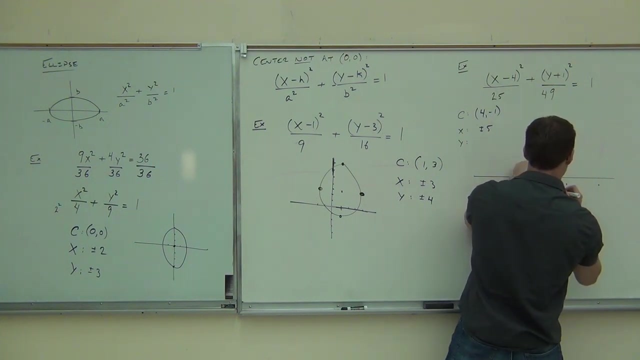 So that's along our x direction, associated with x, that's how we find that number. And along the y, we should get seven out of that. We're taking the square root of those numbers and the bottom of our fraction, we get seven, 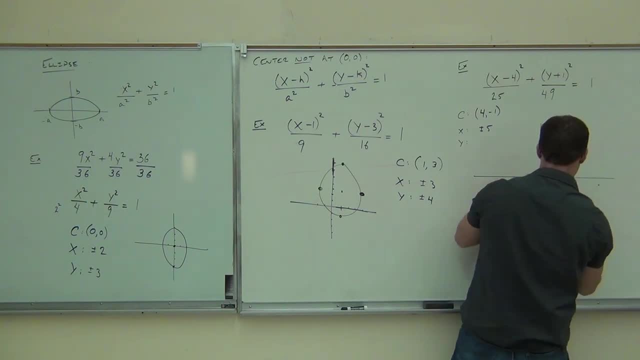 one, two, three, four. All right. 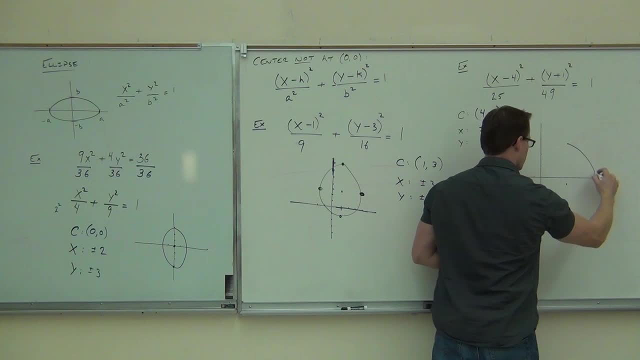 All right. Let's see if we can find the center of any circle or ellipse. Better. Not much better, but a little bit better. 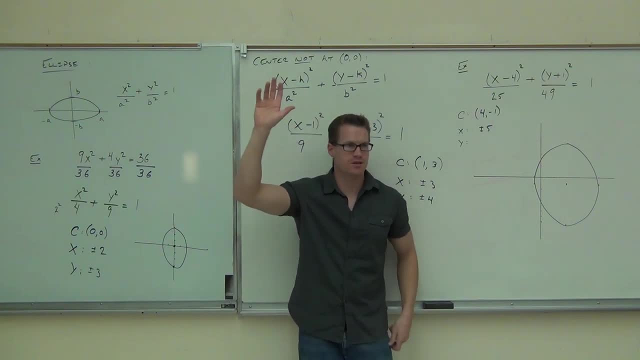 Would you raise your hand if you feel okay with these ellipses? Do you understand the concept of the difference between circles and ellipses? All right. 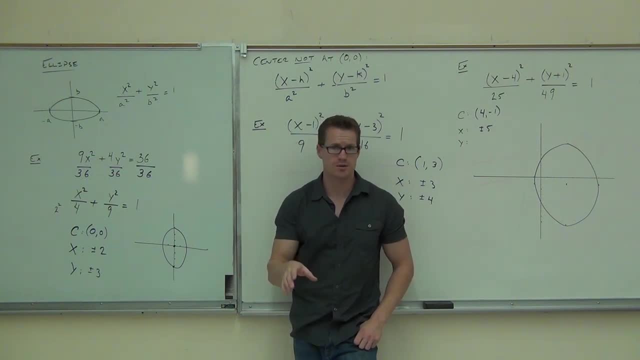 Do you understand how to find the center of any circle or ellipse? Good. 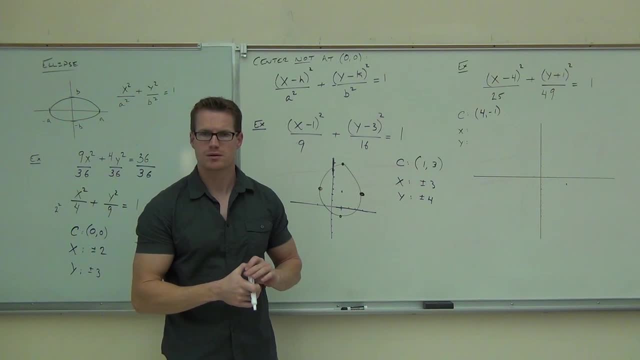 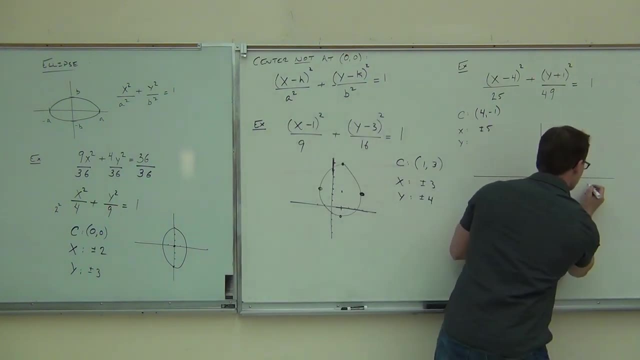 Is it 25, five, six, seven, eight, Five, seven or 49? How much Five Sure? Plus or minus five in either direction here: one, two, three, four, five. So that's along our x direction. 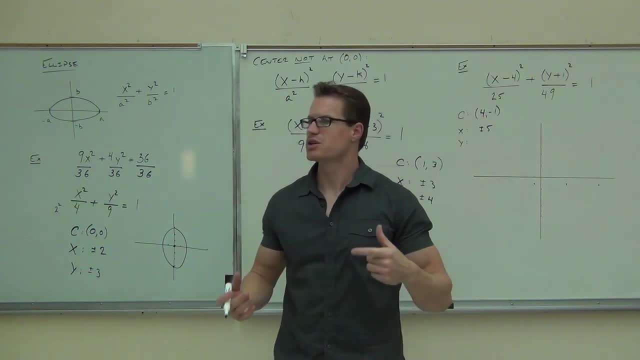 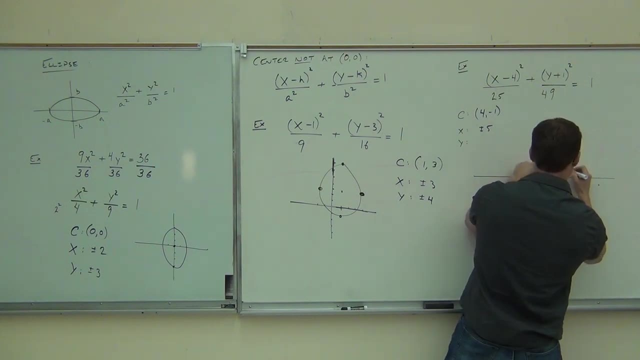 So with x- that's how we find that number- And along the y we should get seven. out of that We're taking the square root of those numbers and the bottom of our fraction, we get seven. one, two, One, two, three, four, five, right? 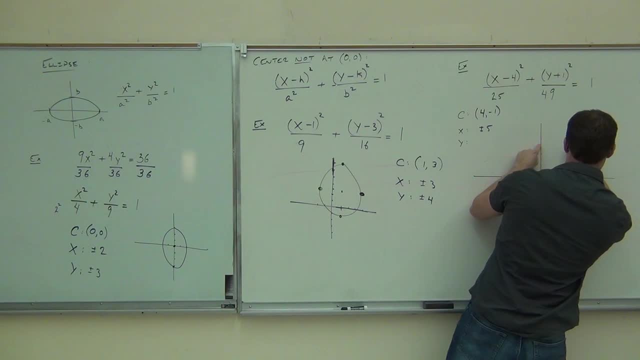 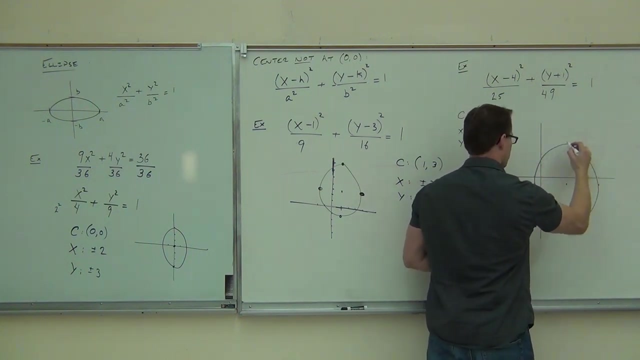 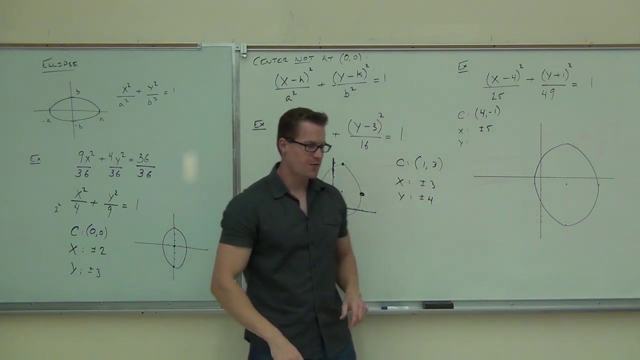 But with the right one, one, two, three, four, five, All right, And we just make that same Answer Better. Not much better, but a little, a little bit better. Would you raise your hand if you feel okay with these ellipses? 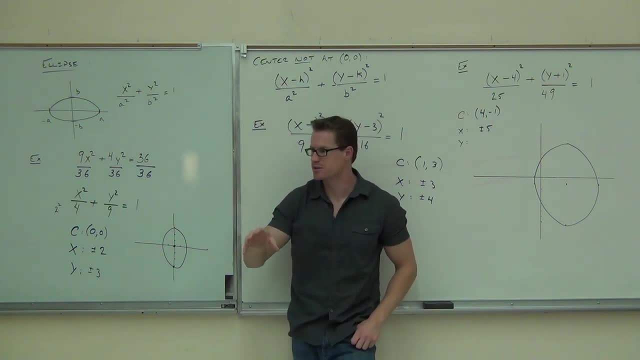 Do you understand that? the concept of the difference between circles and ellipses? Yes, Okay, Alright. Do you understand how to find the center of any circle or ellipse? Good, And now you can find the x-direction and the y-direction, as far as spread goes, and draw that figure. There's one more. 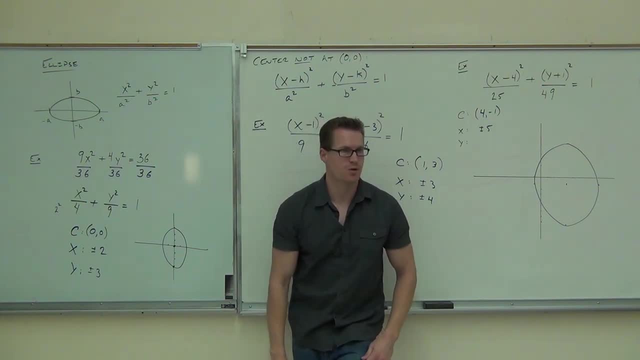 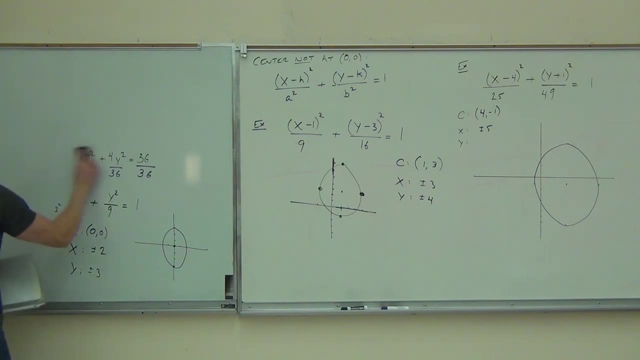 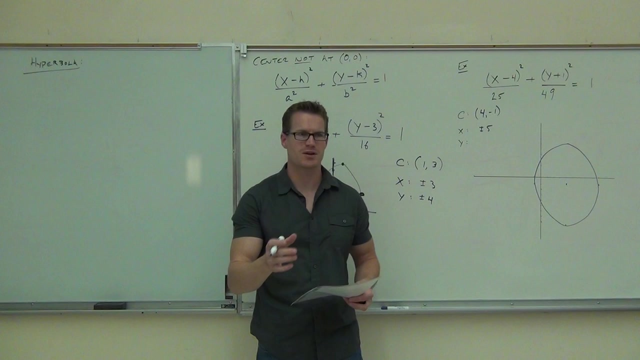 one more thing we need to talk about. We're going to talk about hyperbolas. Say hyperbola with me: Hyperbola, Not hyperbole. We're not talking about exaggeration here, But a hyperbola is a mathematical figure. It's not a circle or an ellipse. 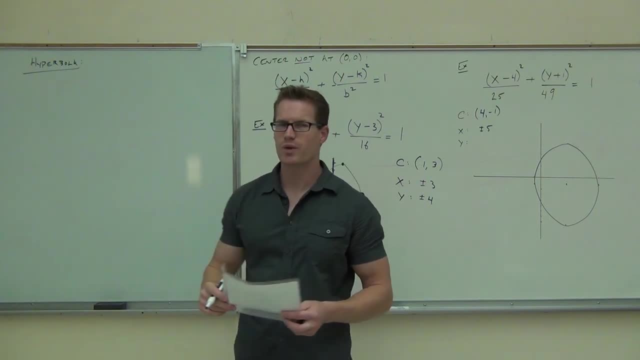 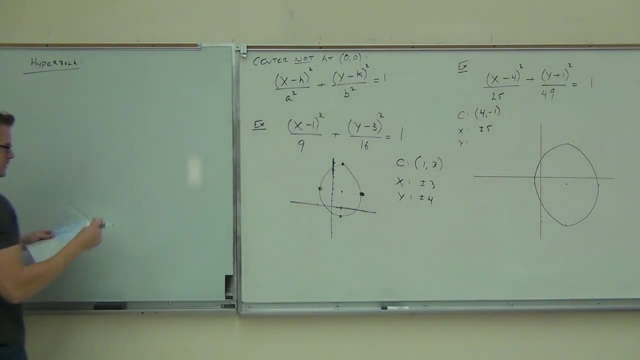 It doesn't look even close to those things. It's kind of weird. It's like if you took an ellipse and separated it and blew it up. It goes like forever. It's crazy looking. It's kind of neat. Here's how a hyperbola looks. There's actually two cases. We'll talk about both cases. 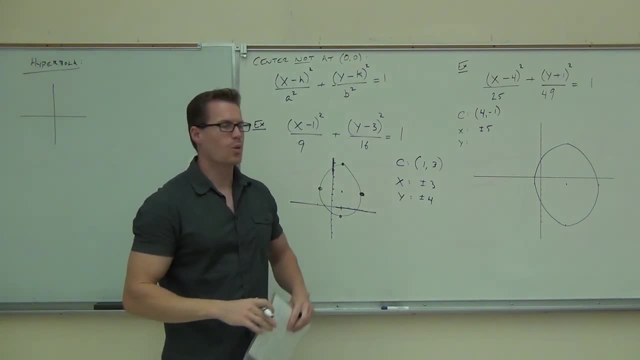 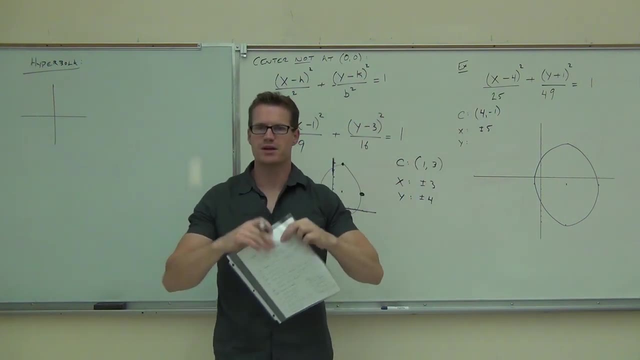 Formula 4 and ellipse in a circle was x squared plus y squared And either, whether it was over a number or not, you had this figure. It was kind of a roundish figure. You had circles that had the same numbers and ellipses that had different numbers. 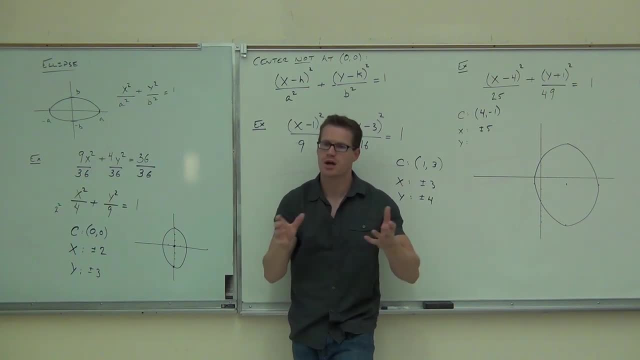 And now you can find the x direction and the y direction as far as the spread goes and draw that figure. There's one more. One more. 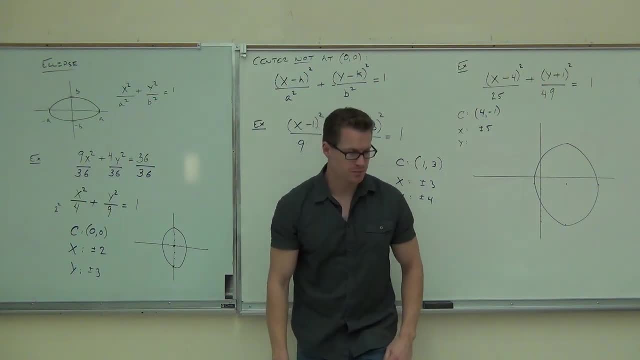 One more thing we need to talk about. We're going to talk about hyperbolas. 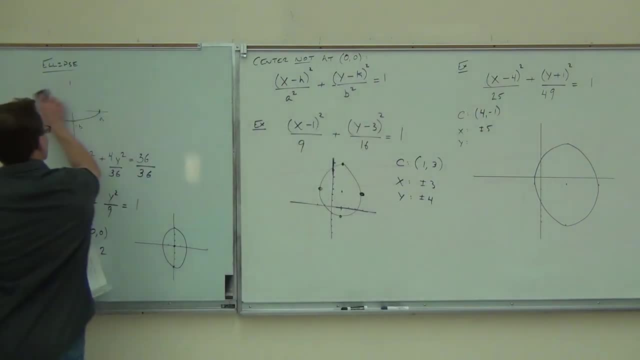 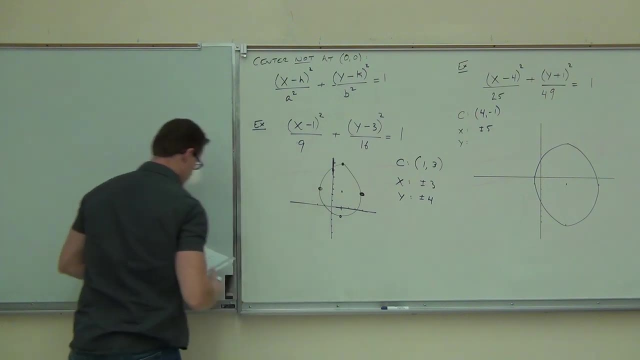 Say hyperbola with me. Hyperbola. Not hyperbole. All right. 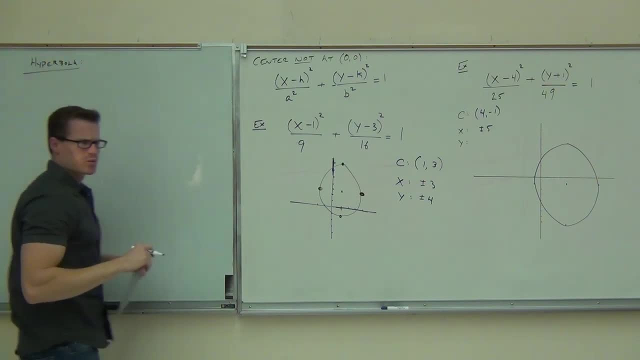 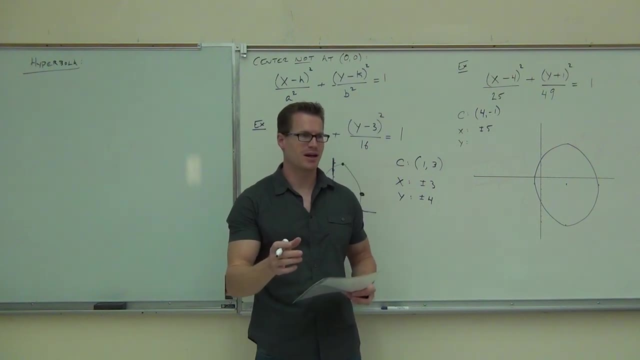 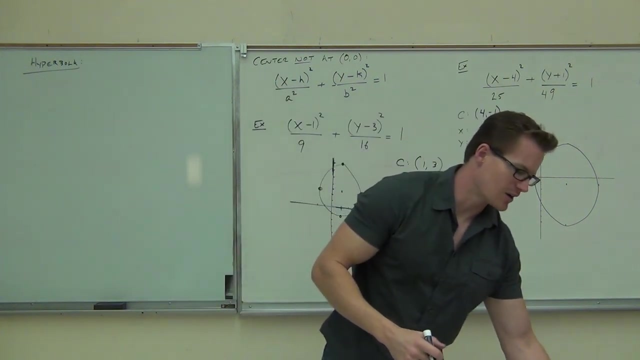 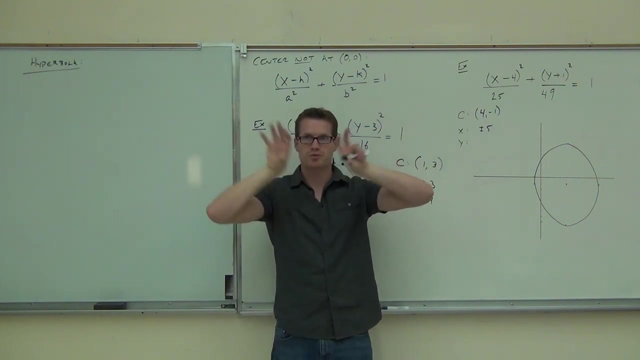 We're not talking about exaggeration here. A hyperbola is a mathematical figure. It's not a circle or an ellipse. It doesn't look even close to those things. It's kind of weird. It's like if you took an ellipse and separated it and blew it up. And it goes like forever. It's crazy looking. It's kind of neat. 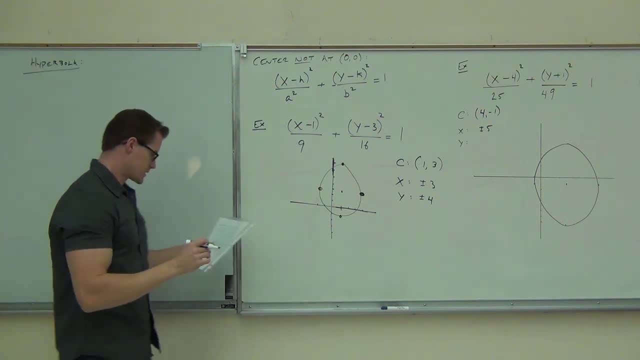 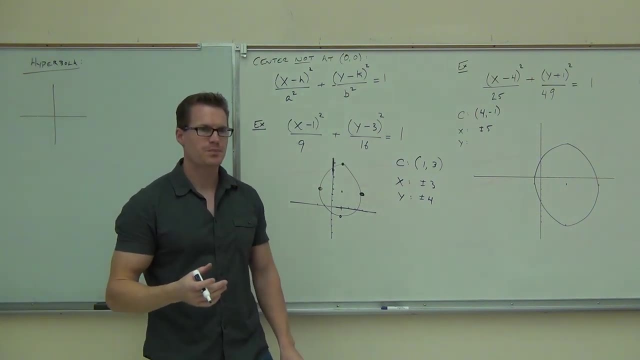 Here's how a hyperbola looks. There's actually two cases. We'll talk about both cases. Formula 4, an ellipse, and a circle was x squared plus y squared. And x squared plus y squared. 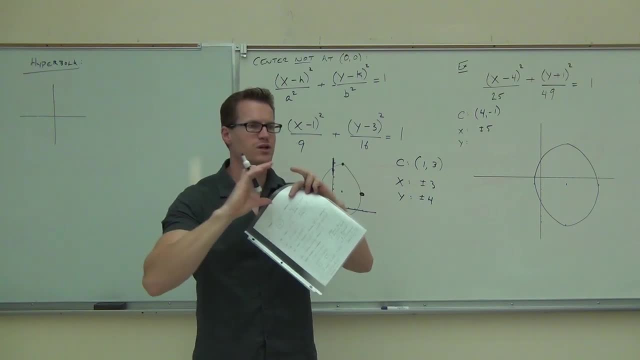 And either whether it was over a number or not, you had this figure. It was kind of a roundish figure, right? You had circles that had the same numbers and ellipses that had different numbers. 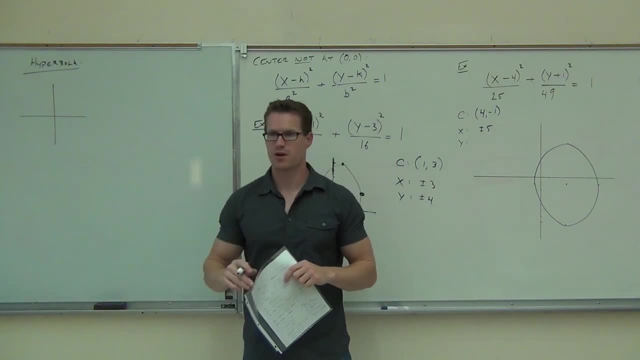 But the key here was that they both had pluses. You follow me on that? They both had those pluses. That plus you can think of. Let me focus up here. 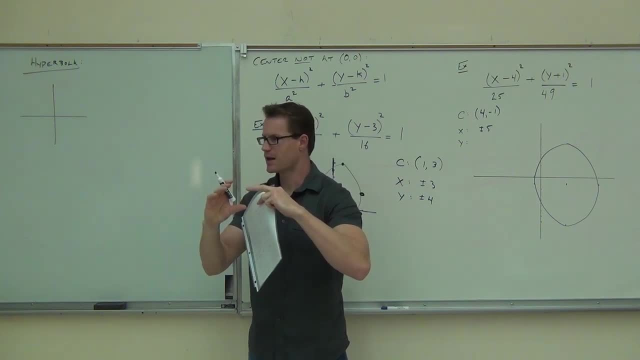 The pluses kind of joined. Your circle together, if you want to think about it like that. It says you're all one connected unit. 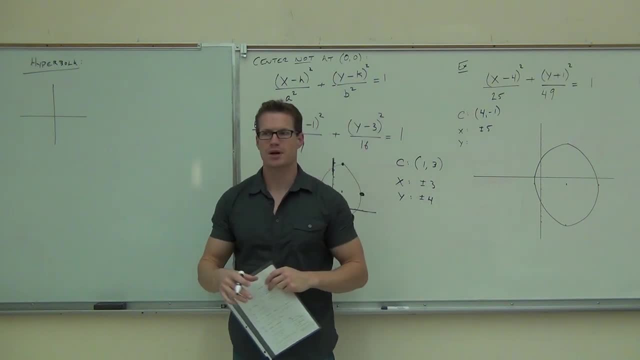 What we're going to have with a hyperbola is not a plus in the middle, but we're going to have a minus. So hyperbola is the only difference between an ellipse and a hyperbola is this. 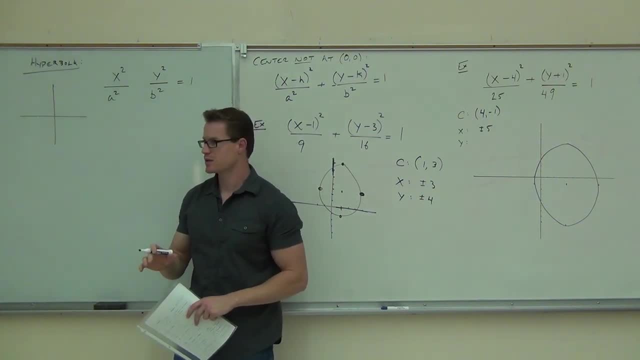 Right now that looks very, very, very similar to an ellipse, doesn't it? That would be an ellipse. That is a hyperbola. 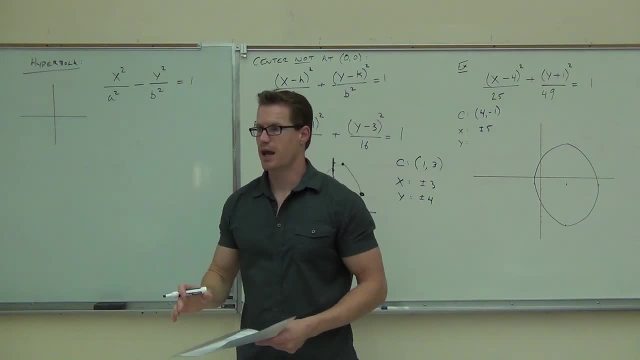 So what's the difference between circles and ellipses and hyperbolas? Circles have the same numbers. Okay, circles have the same numbers. Ellipses don't. But what I mean is you're going to categorize things as circles, ellipses, or hyperbolas. 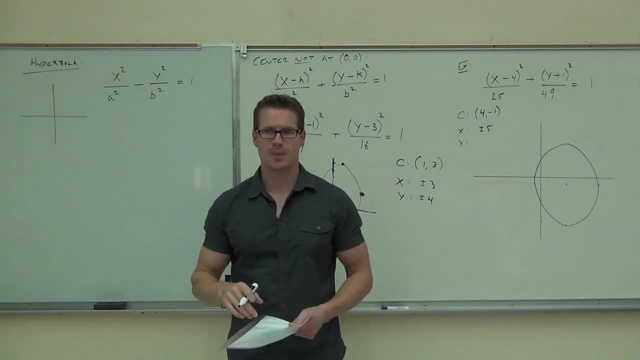 What's the difference between circles, ellipses, and hyperbolas? The minus. The minus. That's it. 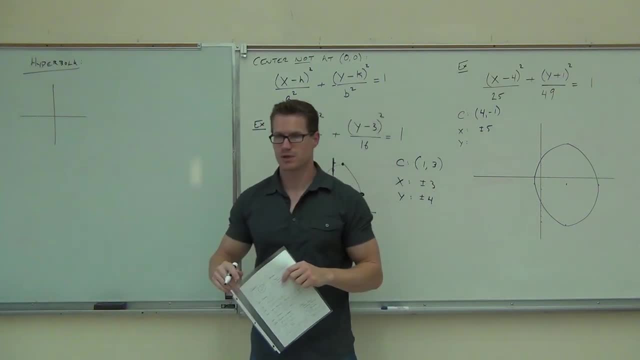 But the key here was that they both had pluses. You follow me on that. They both had those pluses, That plus. you can think of The pluses kind of join your circle together, if you want to think about it like that. It says you're all one connected. 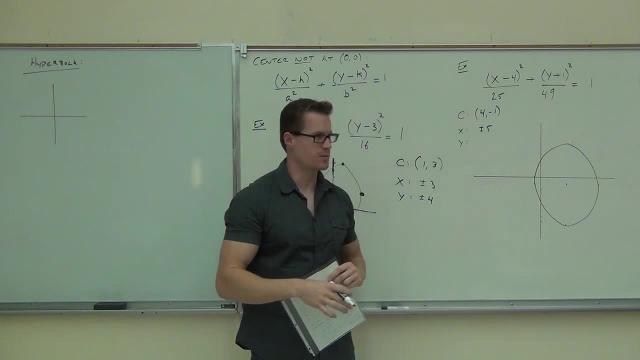 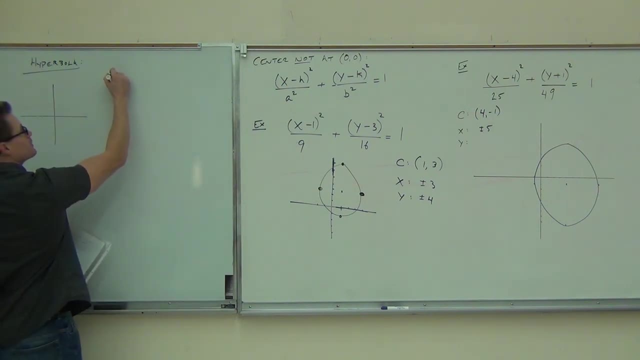 unit. What we're going to have with a hyperbola is not a plus in the middle, but we're going to have a minus, So hyperbola is. the only difference between an ellipse and a hyperbola is this: Right now, that looks very, very, very similar to. 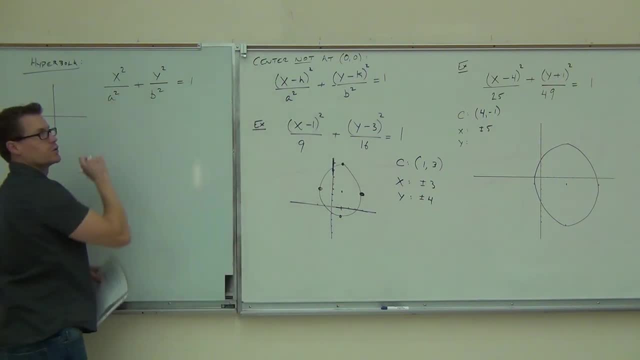 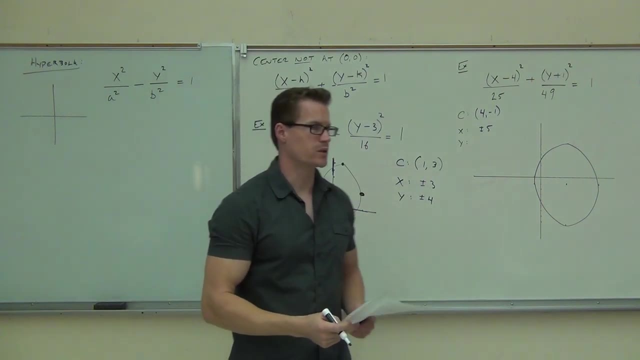 an ellipse, doesn't it? That would be an ellipse, That is a hyperbola. So what's the difference between circles and ellipses and hyperbolas? Circles have the same numbers, ellipses don't. But what I mean is you're going to categorize things as circles, ellipses or hyperbolas. 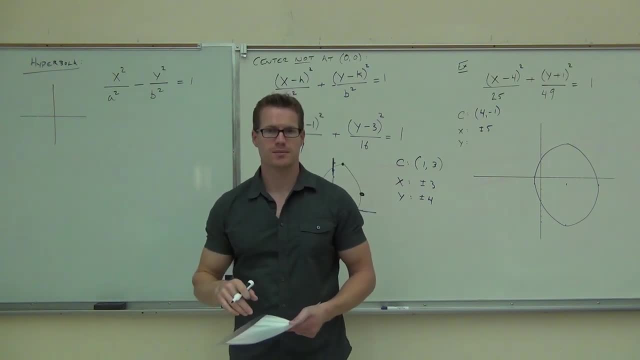 What's the difference between circles, ellipses and hyperbolas? The minus, That's it. The circles and ellipses have that plus The hyperbolas don't. Now, you don't even know what they look like, but hopefully right now you can. 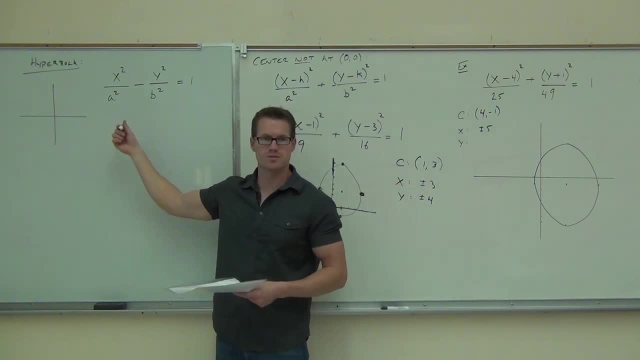 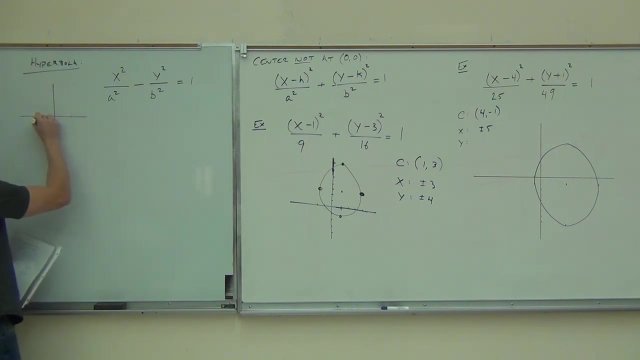 identify the difference formulaically between circles and ellipses and hyperbolas? Can you do that? If it's got a minus, it's a hyperbola. Now, how does this look? It's like that Or Like that About, like that. 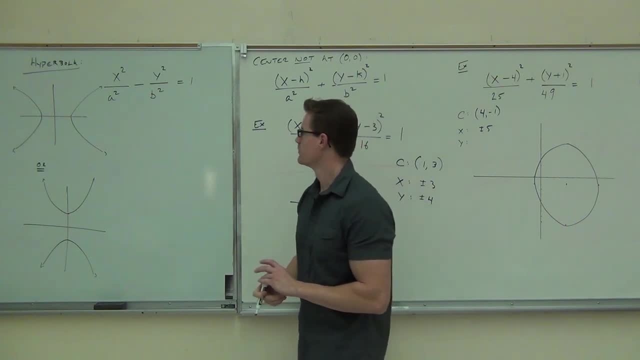 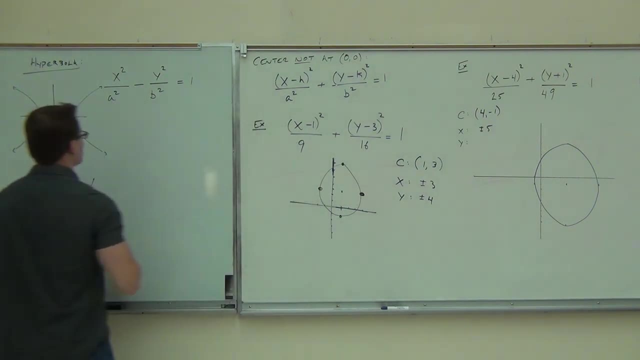 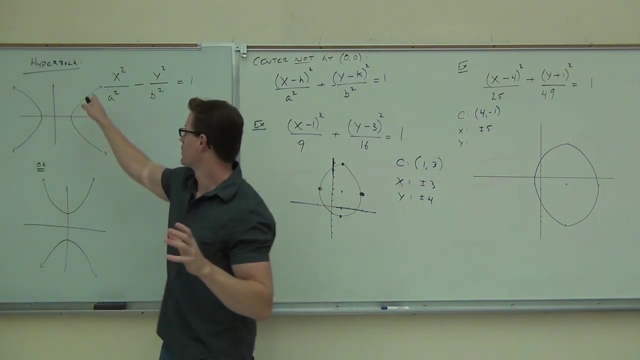 What's the difference? Well, if we have x squared minus y squared, what's coming first, X or y? In our formula, what comes first The x? That means we're going to be spreading out along the x direction. So if you 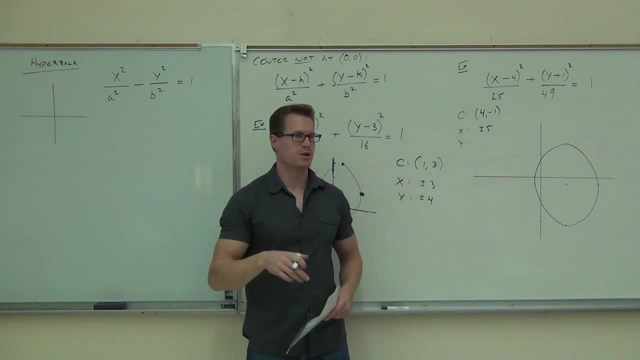 The circles and ellipses have that plus. The hyperbolas don't. 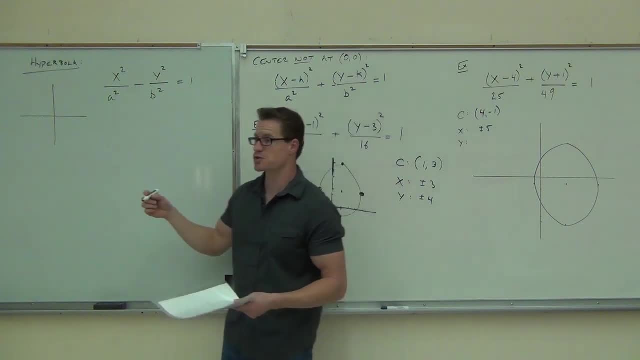 Now, you don't even know what they look like. But hopefully right now you can identify them. Identify the difference formulaically between circles and ellipses and hyperbolas. 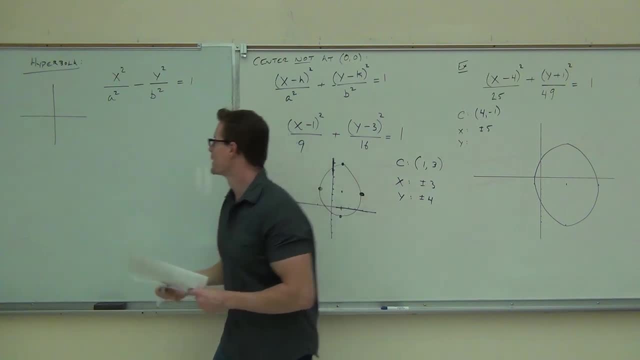 Can you do that? If it's got a minus, it's a hyperbola. Now, how hyperbolas look. 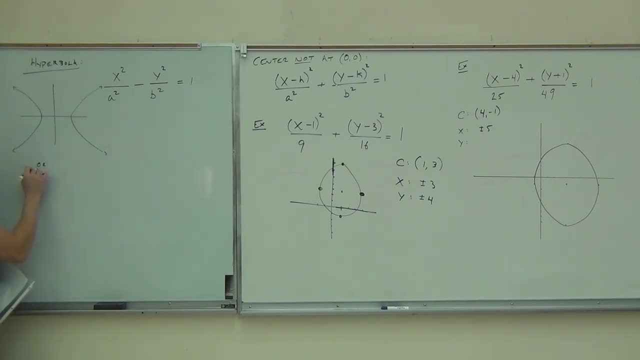 It's like that. Or. Like that. About like that. 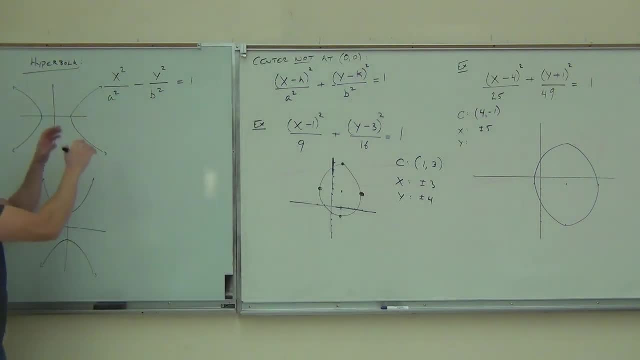 What's the difference? Well, if we have x squared minus y squared, what's coming first, x or y? In our formula, what comes first? The x. 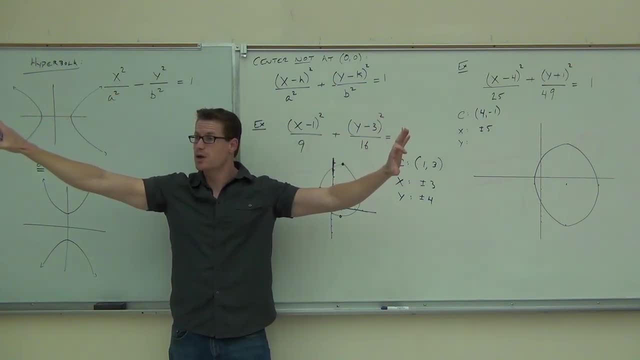 That means we're going to be spreading out along the x direction. So if you start with x, you're going to be going in the x direction. Is that clear for you? What do you think this one's going to start with? Y. It's going to be y. 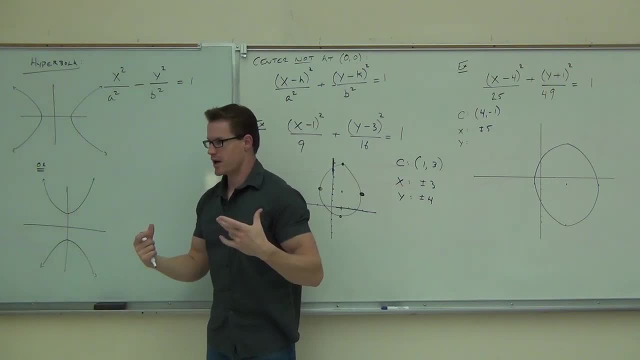 So if I switch those around, notice how addition's commutative, right? Subtraction's not. If I switch around these, it really doesn't make a difference because whatever comes first, you're adding it. Who cares? Like 5 plus 7, same as 7 plus 5. 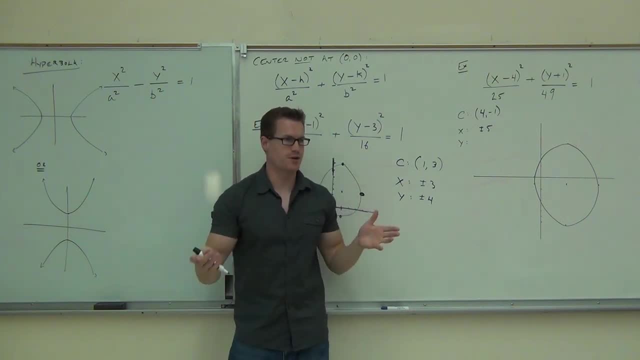 But subtraction, if I switch those around, I should have a completely different figure, and that's exactly what I get. 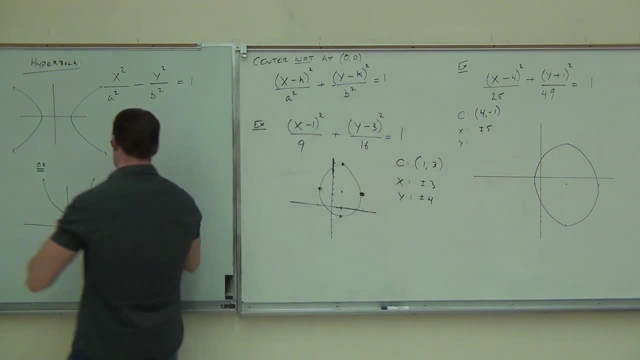 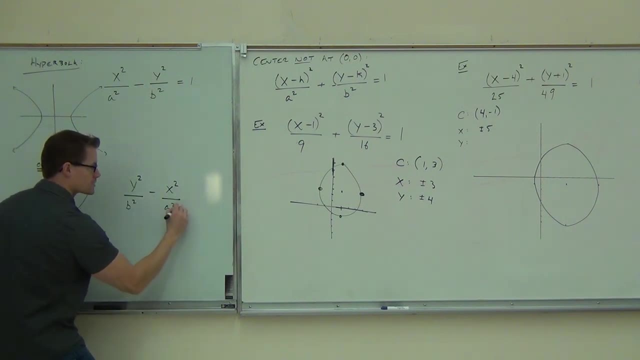 So x squared minus y squared, x direction. If I do y squared minus x squared, notice how the b goes along and the a goes along with those x and y respectively. 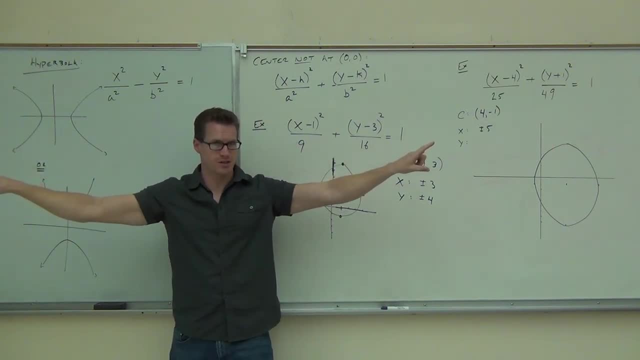 start with x. you're going to be going in the x direction. Is that clear for you? What do you think? this one is going to start with Y, So, if I switch those around, notice how addition is commutative, right. 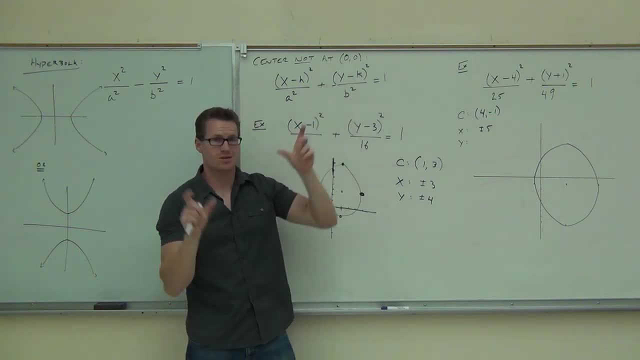 Subtraction is not. If I switch around these, it really doesn't make a difference, Because whatever comes first, you're adding it. Who cares Like 5 plus 7 is the same as 7 plus 5.. But subtraction. 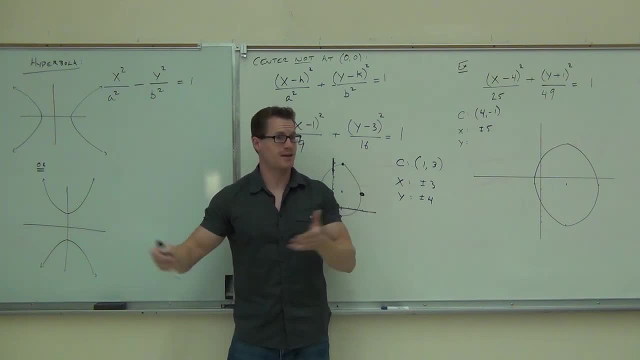 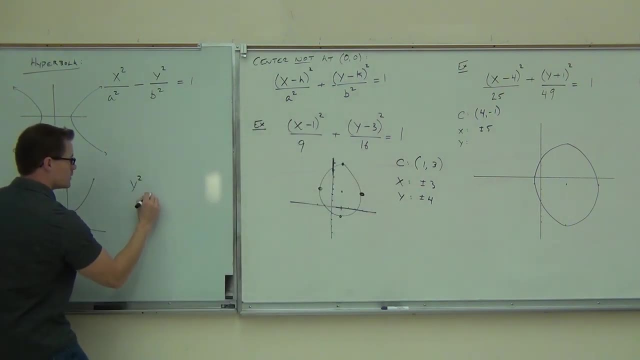 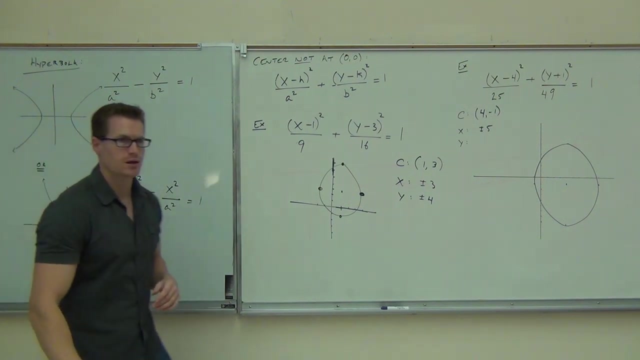 if I switch those around, I should have a completely different figure, and that's exactly what I get. So x squared minus y squared, x direction. If I do y squared minus x squared, notice how the b goes along and the a goes along with those x and y's respectively. I'm now going 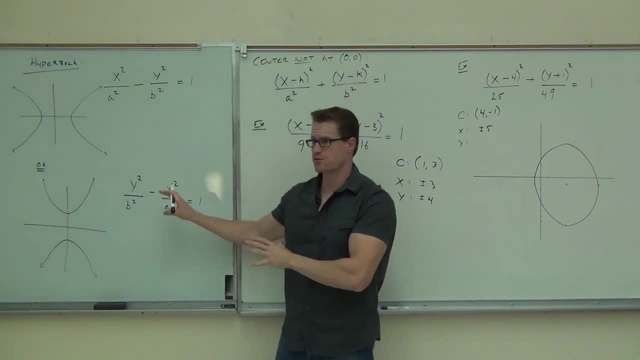 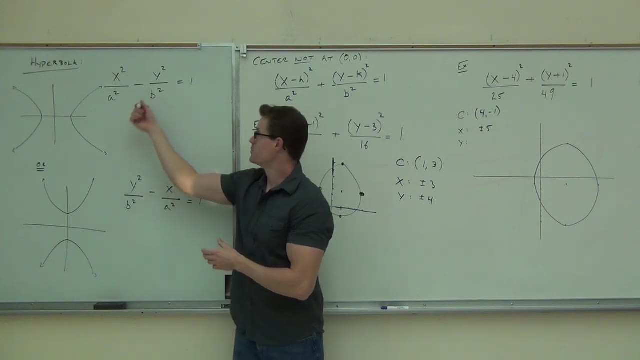 to get spread out in the y direction. Do you guys see the difference and can understand these formulas, Are you sure? So x comes first this way, Y comes first this way, The b's and the a's: they go along with the x and the y's. Now, what do those b's and those a's stand for? Well, 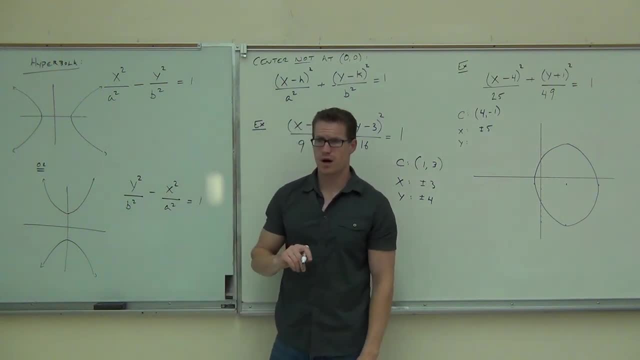 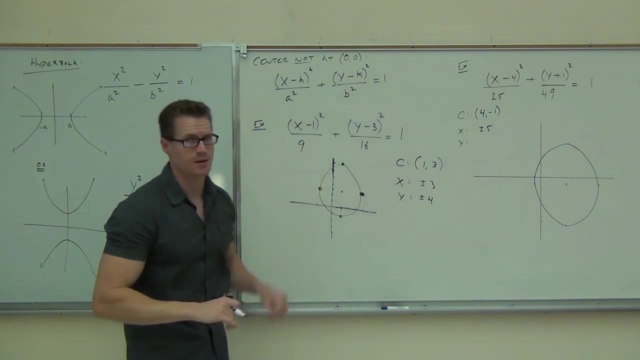 this is kind of cool. What letter is a associated with the x or the y? That means that this, right here, just like an ellipse, just like it, it's going to give you the negative a and the a. It's going to tell you where those things cross the x-axis, just like this did, By the way. where's? 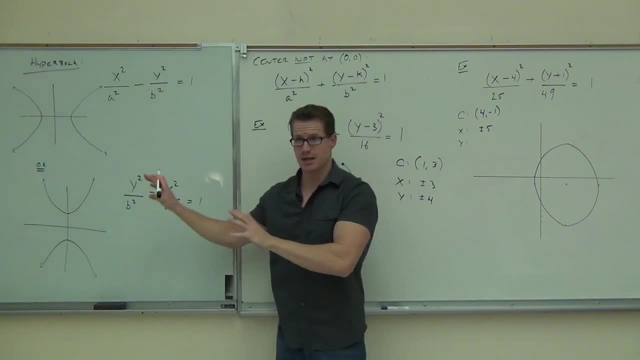 I'm now going to get spread out in the y direction. Do you guys see the difference and can understand these formulas? Are you sure? So x comes first this way. 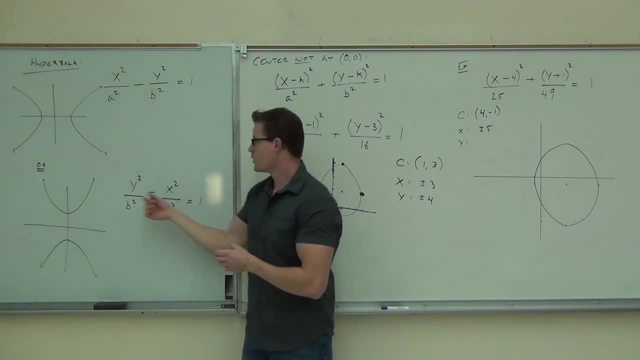 Y comes first this way. The b's and the a's, they go along with the x and the y's. Now what do those b's and those a's stand for? Well, this is kind of cool. What letter is a associated with, the x or the y? X. 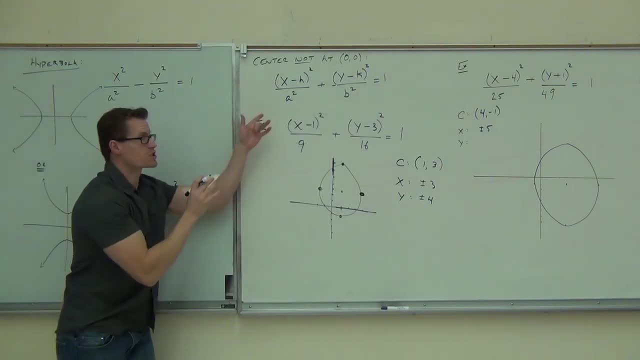 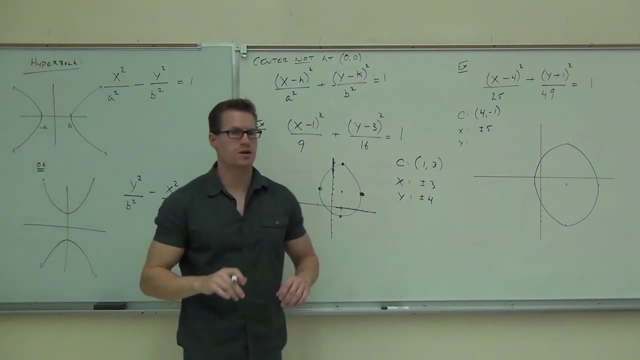 That means that this right here, just like an ellipse, just like it, it's going to give you the negative a and the a. It's going to tell you where those things cross the x axis just like this did. 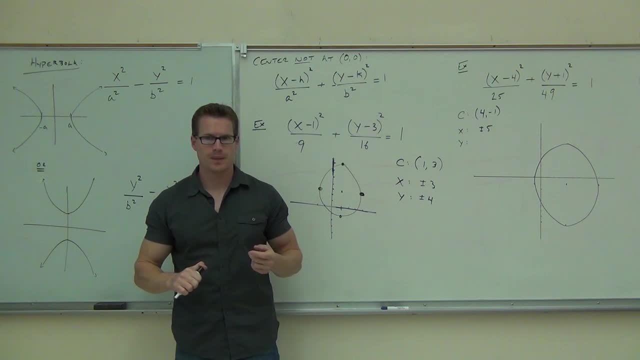 By the way, where? Where's the center for this hyperbola? Zero, zero, zero. Yeah, and that's what we're really going to deal with in this class is centered to zero, zero. Could you do it, switch, shifting it around? Of course. It works just like the ellipses and the circles. You can shift those just like you normally would. We're going to probably stick to centered at zero, zero, okay? Centered at zero, zero. 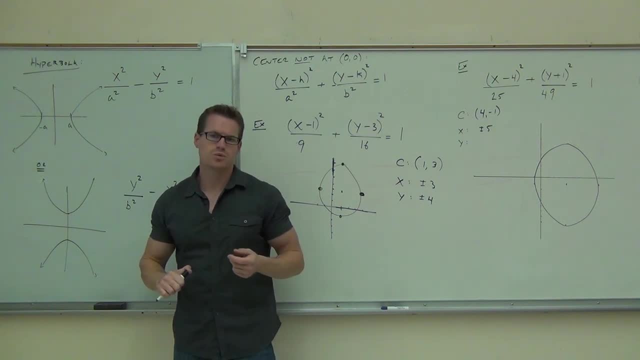 the center for this hyperbola- Yeah, and that's what we're really going to deal with in this class- is centered to 0, 0.. Could you do it shifting it around? Of course It works just like the ellipses in the circle. 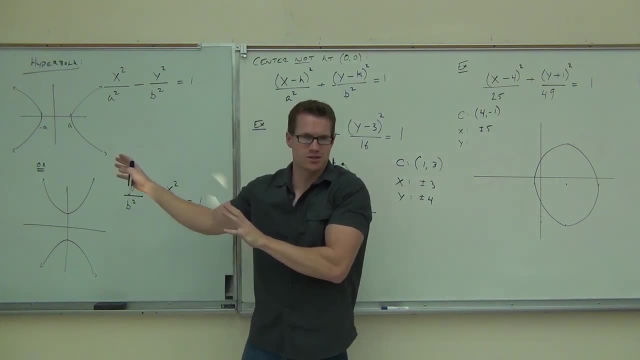 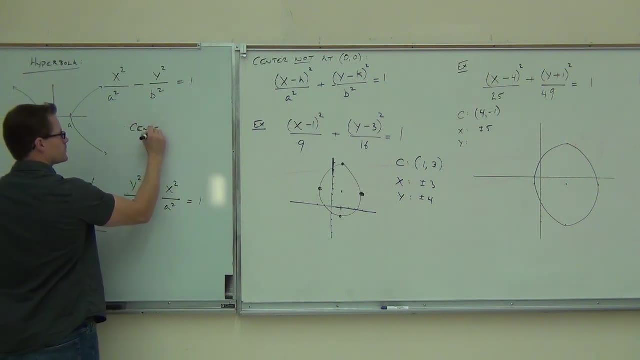 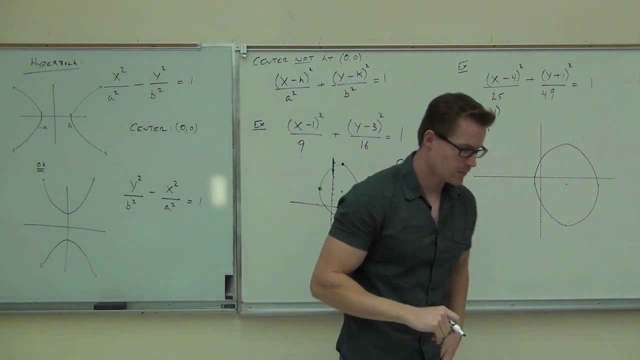 You can shift those just like you normally would. We're going to probably stick to centered at 0, 0,. okay, Centered at 0, 0.. The x-intercepts are given by plus or minus a for this one. 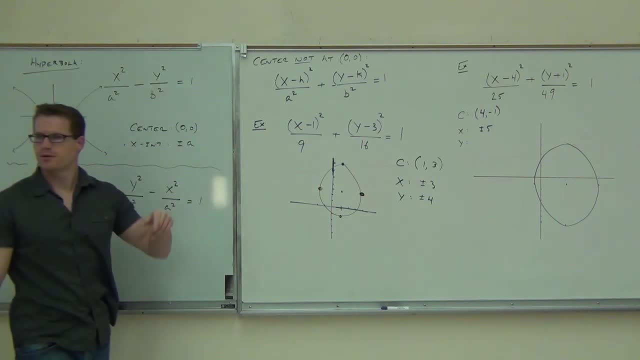 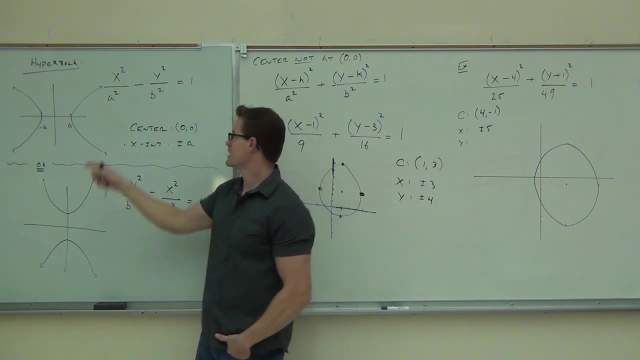 Are there any y-intercepts in this graph? No, Are there any y-intercepts in this graph? That's interesting, isn't it? That's interesting. It says x squared comes first, and if you're splitting on x-direction, there will be x-intercepts, but there's not going to be any y-intercepts. 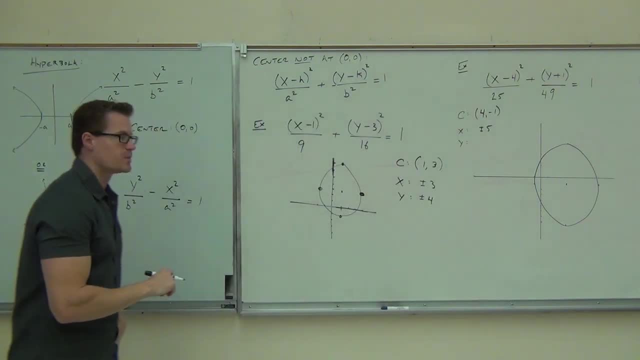 The x is going to be centered at zero, zero. The x-intercepts are given by plus or minus a for this one. 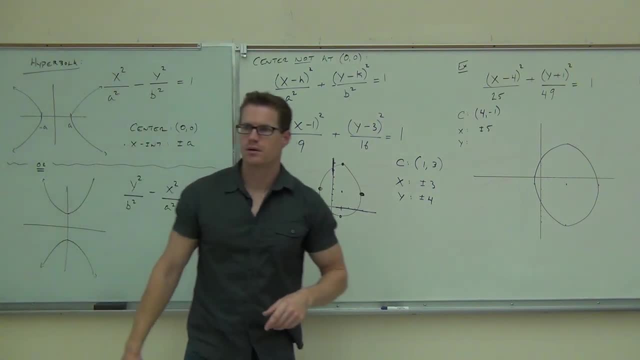 Are there any y-intercepts in this graph? No. Are there any y-intercepts in this graph? 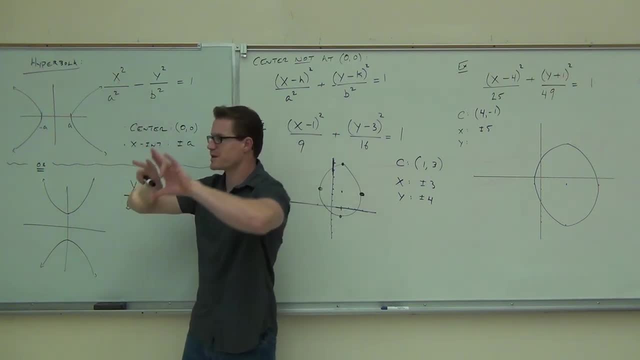 That's interesting, isn't it? That's interesting. It says x squared comes first, you're splitting on x direction, there will be x-intercepts, but there's not going to be any y-intercepts. 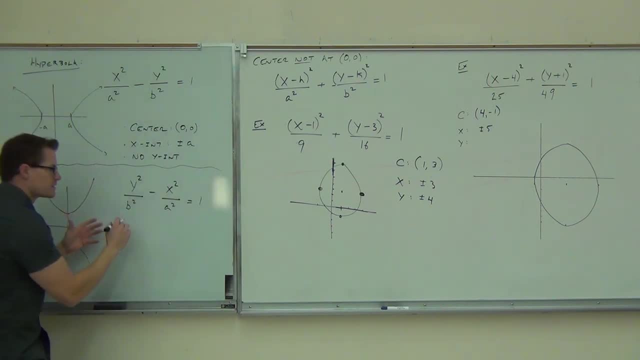 Weird. Now, this has the same center, of course, we're centered around zero, zero. 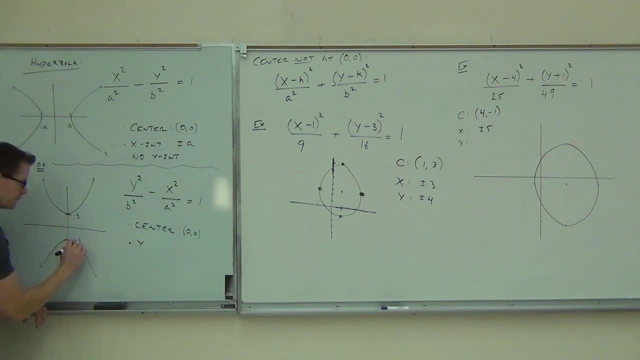 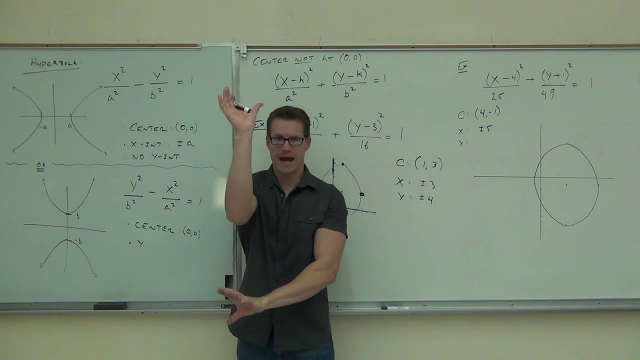 And our y-intercepts are going to be given by b and negative b, again, very, very much like an ellipse. You look under that y, since we know it's spreading along the y-axis, you're going to have some y-intercepts, but there's no x-intercepts. 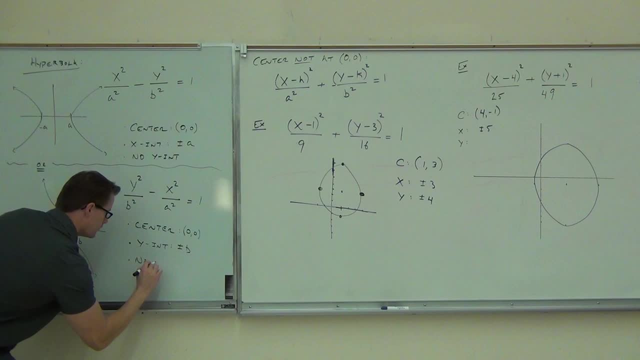 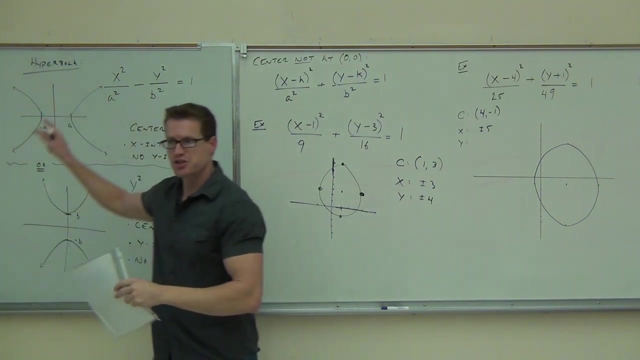 So, we've got our two cases, we have x coming first, x-direction, y coming first, y-direction. In our x-direction, we're going to have x-intercepts, but not y. In our y-direction, we'll have y-intercepts, but not x. Those numbers are similar. Still found exactly the same way that you do your index. 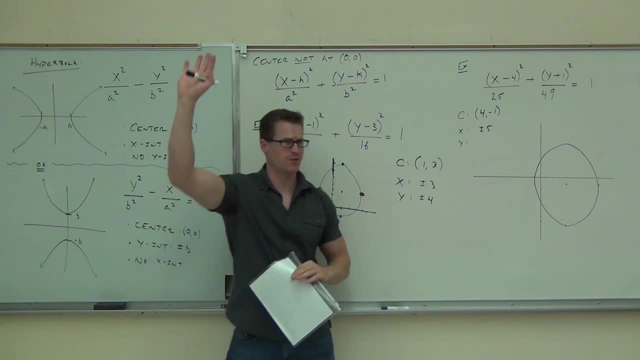 So, we'll give you spread along the x and spread along your y, respectively. Raise your hand if you feel okay with our hyperbola so far. Let's try maybe two examples. 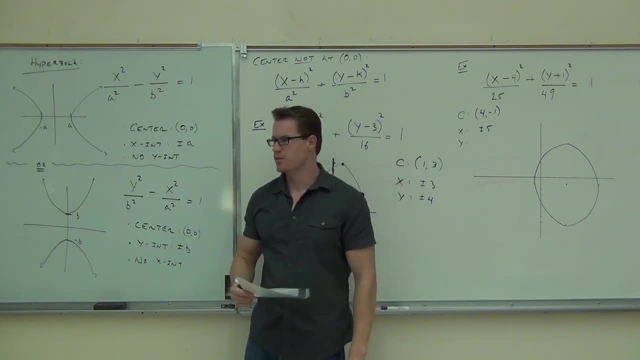 I'll recap everything in a nice little chart for you, and then we'll be done with our section here. 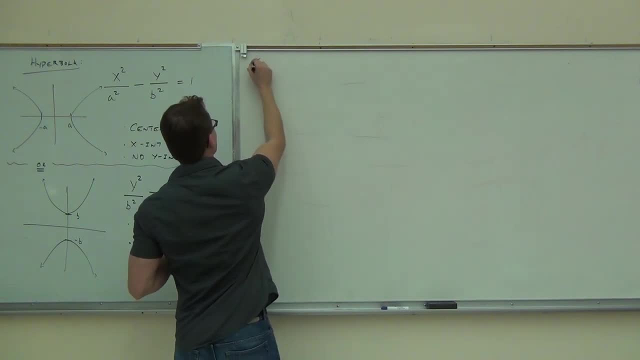 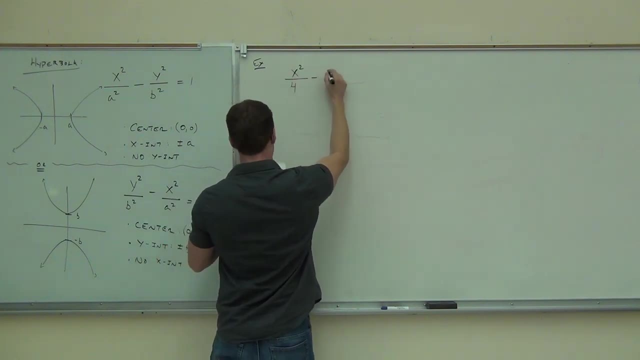 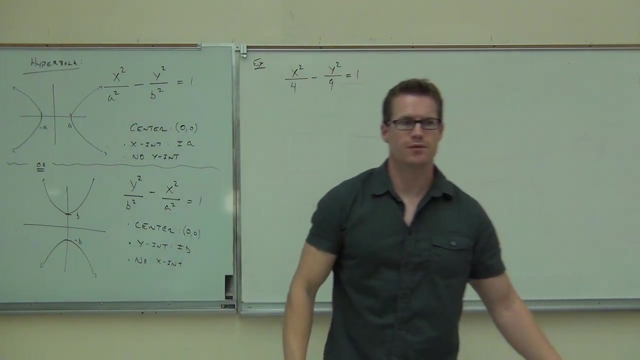 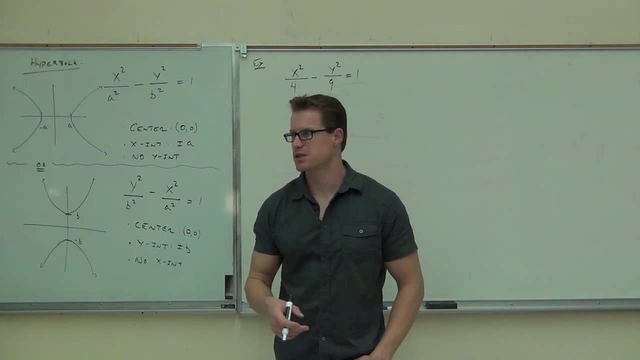 Okay, now the first thing you need to do, of course, is figure out whether you have parabola, circle, ellipse, hyperbola. Those are the four figures we've got. Those are our conic sections. So, is it a parabola? 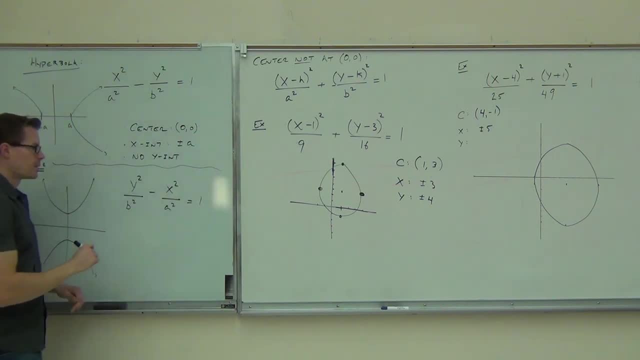 Weird. Now this has the same center. Of course. we're centered around 0, 0.. It's going to shift. That's the same thing we're going to sound. So we're going to want to strike that y-intercept once again and move over towards here where we're not going to be. 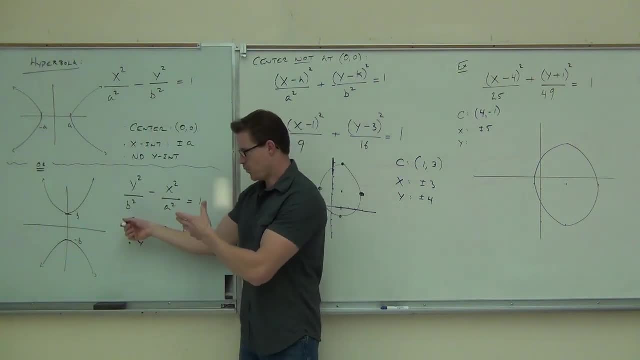 getting the y-intercept just yet This is coming from x. How come there's nothing I could see, as you can see here, an x-intercept, but none. Morally we were assuming that. all right, and then to the white. 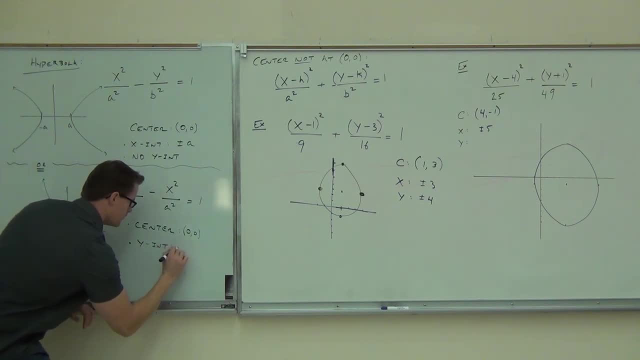 Nobody was in between. That's not true at all and our y-intercepts are going to be given by b and negative b, Again, very, very much like an ellipse. You look under that y, since we know it's spreading out along the y-axis. 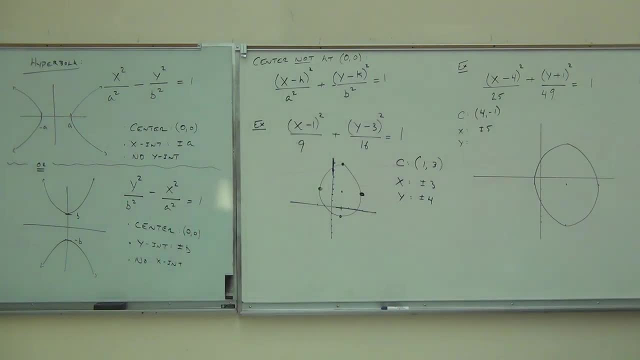 You're going to have some y-intercepts. There's no x-intercepts. Okay, Thank you very much. Thanks, mall всего leo. So we've got our two cases. we have X coming first X direction, Y coming first Y direction. 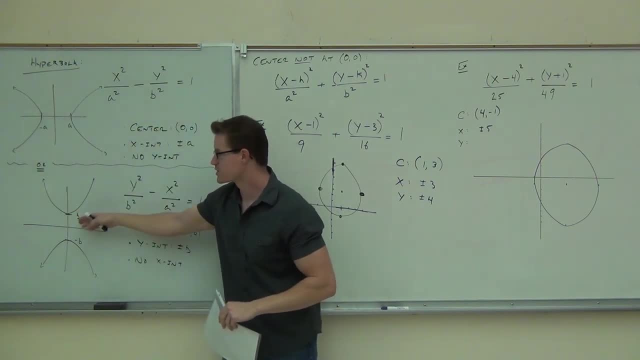 In our X direction, we're going to have X intercepts but not Y. In our Y direction, we'll have Y intercepts but not X. Those numbers are still found, exactly the same way that you do your index. So we'll give you spread along the X and spread along your Y respectively. 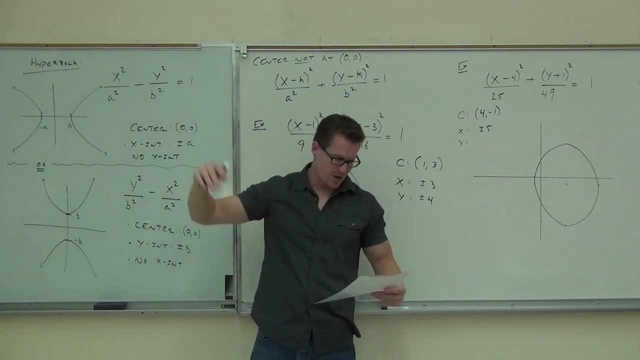 Raise your hand if you're okay with our hyperbola. so far, Let's try maybe two examples. I'll recap everything in a nice little chart for you and then we'll be done with our section here. 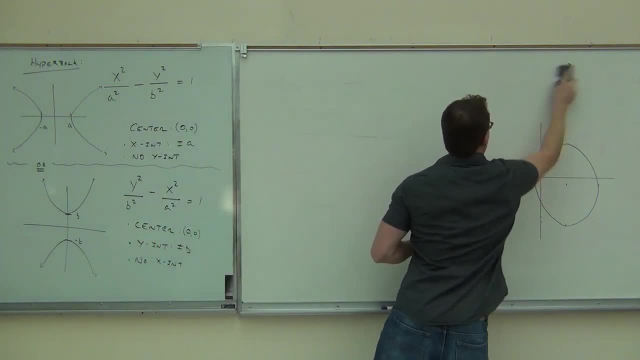 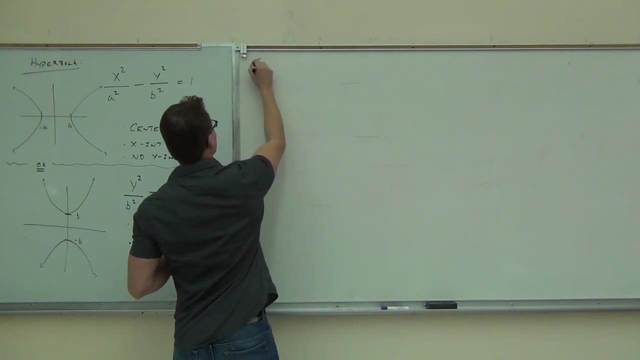 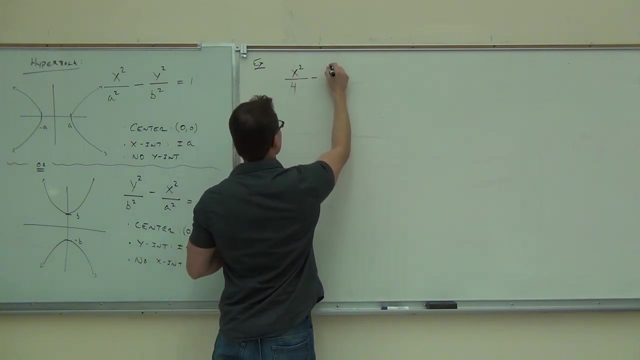 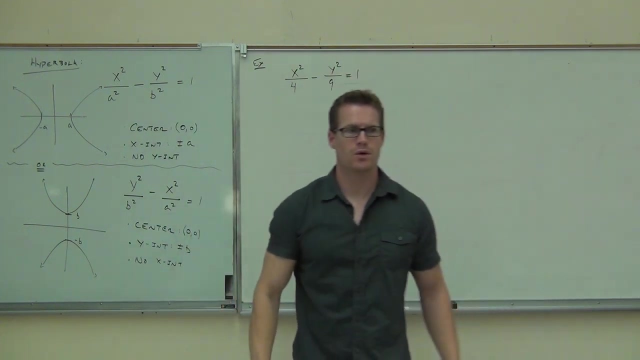 For 10% interest. mer breaker- dark energy guidance. Now, the first thing you need to do, of course, is figure. 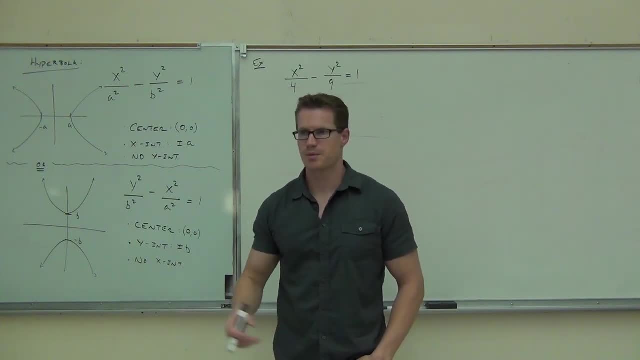 out whether you have parabola, circle, ellipse, hyperbola. Those are the four figures we've got. Those are our conic sections. So is it a parabola? That's a silly question, right? Doesn't look anything like a parabola. 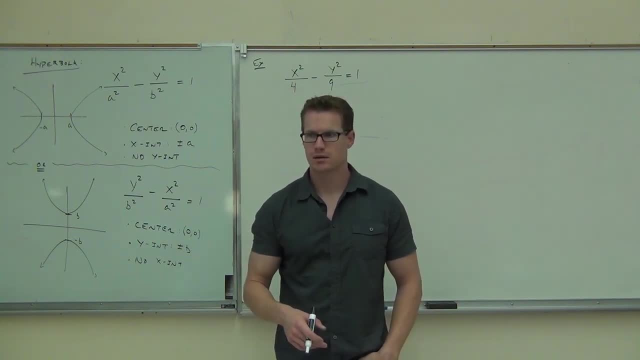 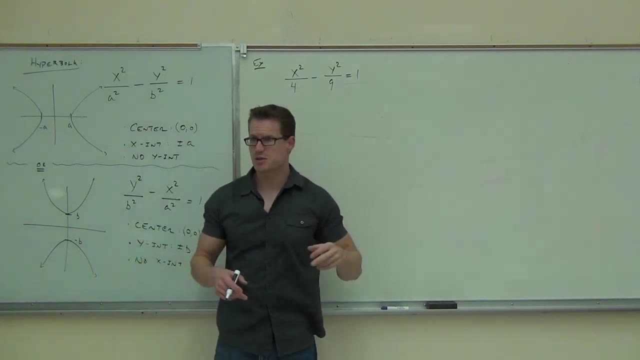 Is it a circle? No, Why not? Two reasons: firstly, number's different right. Secondly, circles have pluses. Is it an ellipse? No, No, No, It has the different numbers. It looks very much like an ellipse. That's a silly question, right? It doesn't look anything like a parabola. Is it a circle? Why not? 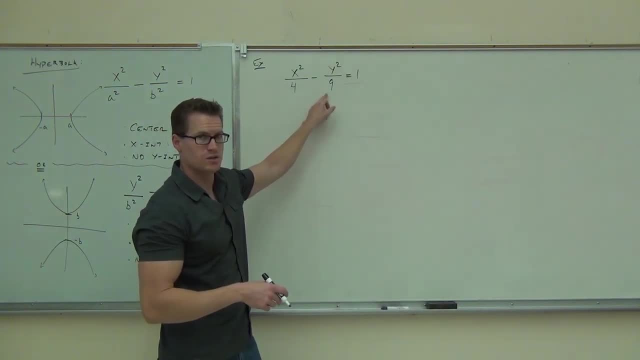 Two reasons. Firstly, numbers are different, right? Secondly, circles have pluses. Is it an ellipse? No. 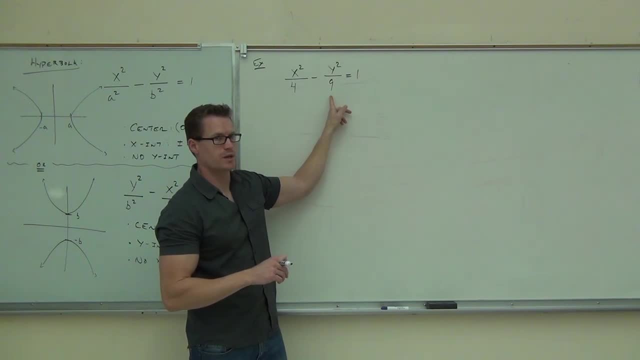 No, it has the different numbers. It looks very much like an ellipse, but what do ellipses have right here? Pluses. 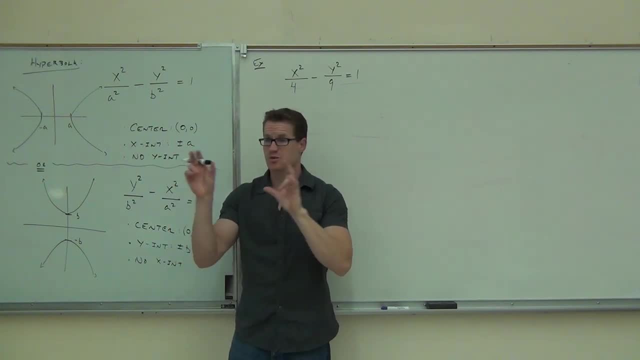 So, this is definitely a hyperbola. If you see a minus and you see the x squared, y squared minus, you've got a hyperbola, no matter what. 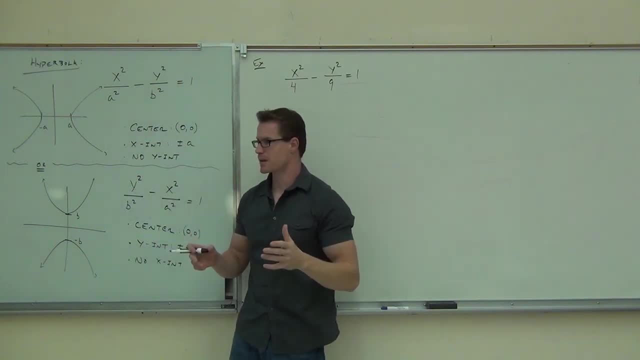 Even if the numbers are the same and you have the minus, you'd have a hyperbola, and that would work. Now, all we've got to be able to do is figure out what the x-intercepts are. All we've got to be able to do is determine whether we're horizontally spreading along the x-direction or vertically spreading along the y-direction hyperbola, 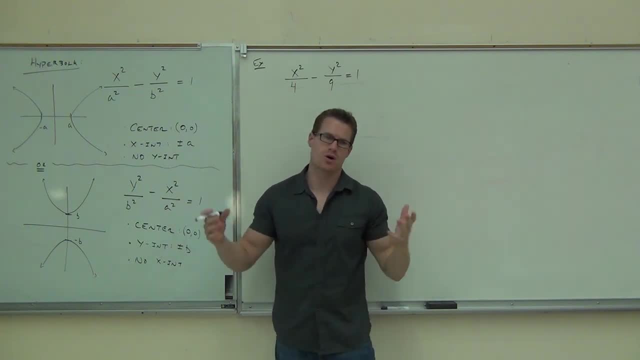 put our little marks, our intercepts, to what we have, and then draw our graph. What are we, in this case, are we spreading out x-direction or are we spreading out y-direction? x-direction. Why? Because the x-intercepts are the first. 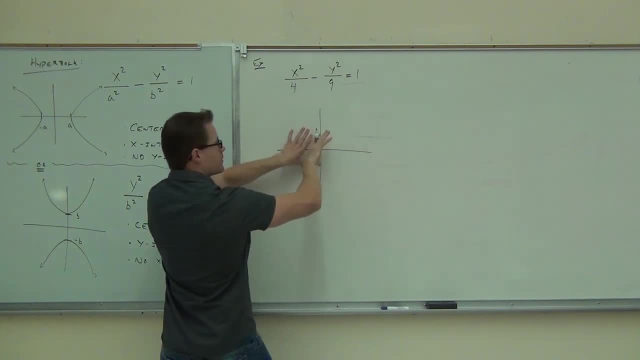 Okay, so what we know is that we should have this looking graph, the Dumbo look, the big ears. They kind of look like ears, right? Well, to me, I have a pretty good imagination, so to me, they look like ears. 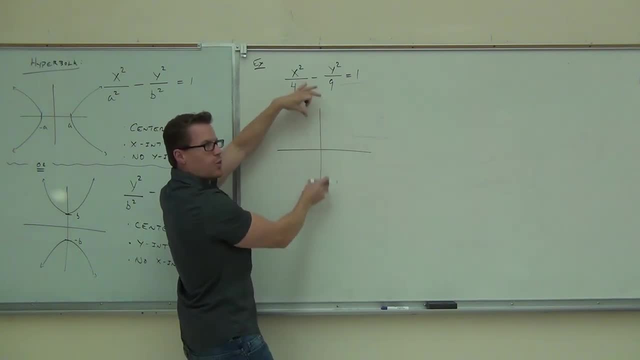 So, if we know we're spreading out this way, are we going to have any y-intercepts? No. Are we going to have x-intercepts? Yes. Yes. How do you find your x-intercepts? Square root of y-four. 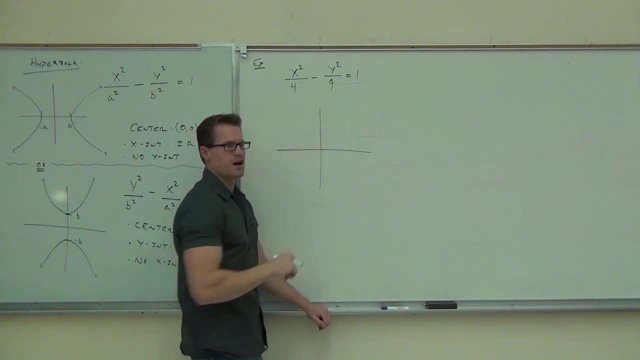 Square root of y-four. Why are we looking at the nine? Because there's no y-intercepts. 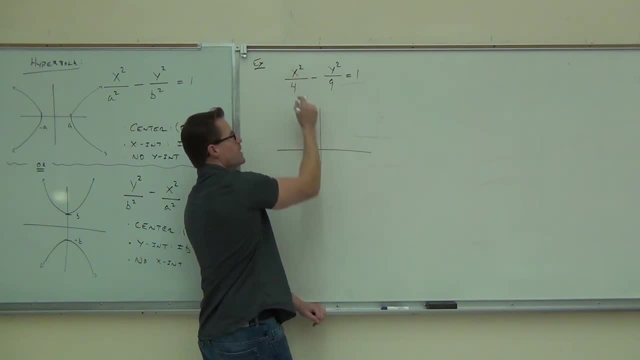 Yeah, there's no y-intercepts. We just have x. We know that whatever comes first, that's giving us our intercepts. Are we two, four, or sixteen? What do you think? Zero, two, zero. 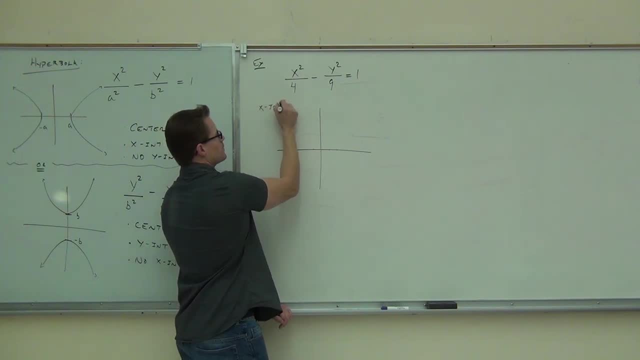 We're at two. Okay, so the x-intercept, plus or minus two. 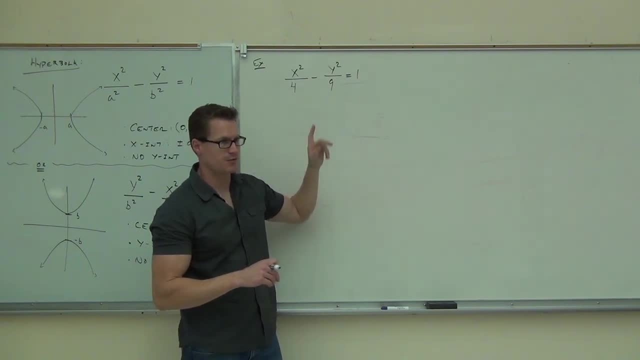 But what do ellipses have right here? Pluses. So this is definitely a hyperbola. If you see a minus and you see the x squared, y squared, minus, you've got a hyperbola, no matter what. Even if the numbers are the same and you have the minus, you'd have a hyperbola and that. 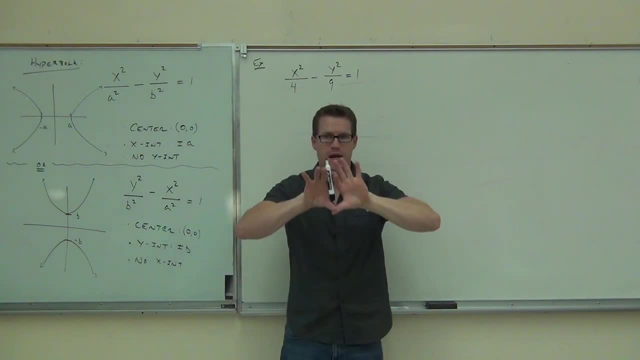 would work. Now, all we've got to be able to do is determine whether we're horizontally spreading along the x direction or vertically spreading along the y direction. hyperbola. put our little marks, our intercepts, to what we have, and then draw our graph. 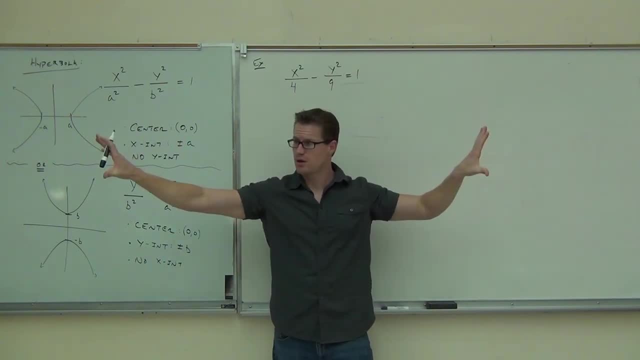 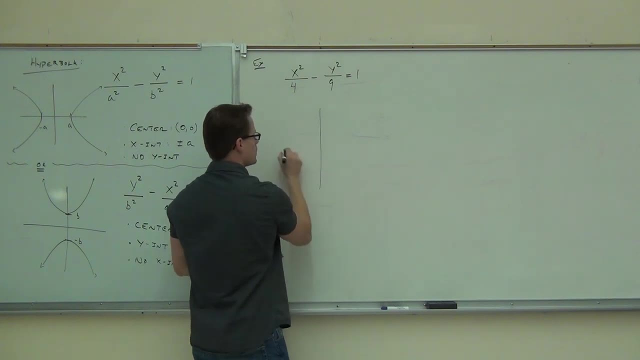 What are we in this case? are we spreading out x direction or are we spreading out y direction, x direction? Why? Because x is the first. Okay, So what we know is that we should have this looking graph: the dumbo, look the big ears. 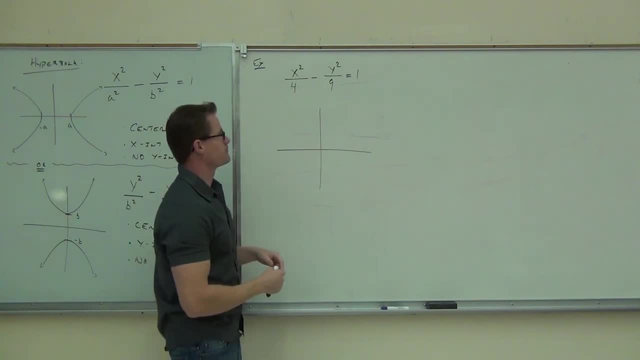 They kind of look like ears. right, I have a pretty good imagination, So to me they look like ears. So let's see. So if we know we're spreading out this way, are we going to have any y intercepts? 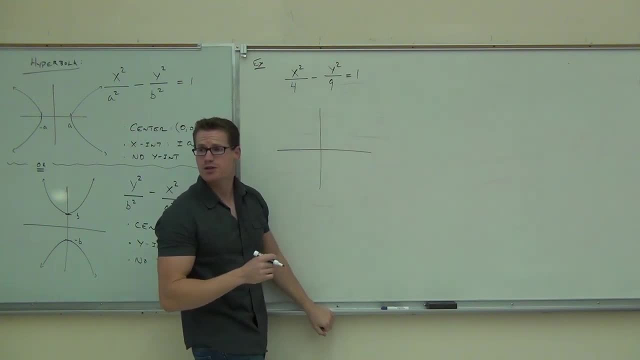 No, Are we going to have x intercepts? Yes, Yes. How would you find your x intercepts? Square root of y, Square root of y-four. Why are we looking at the 9?? Because there's no y intercepts. 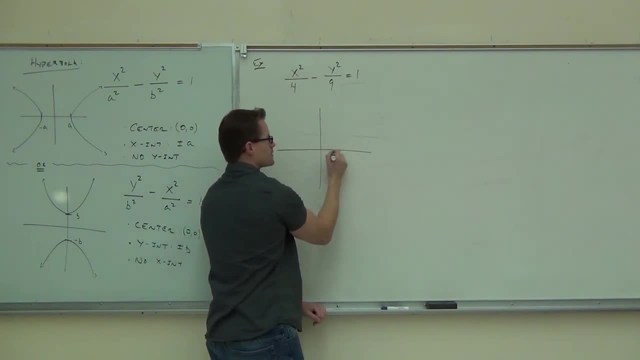 There's no y intercepts, We just have x. We know that whatever comes first, that's giving us our intercepts. Are we 2,, 4 or 16? What do you think? think We're at 2.. Okay, so the x-intercept plus or minus 2.. We're going to be centered. 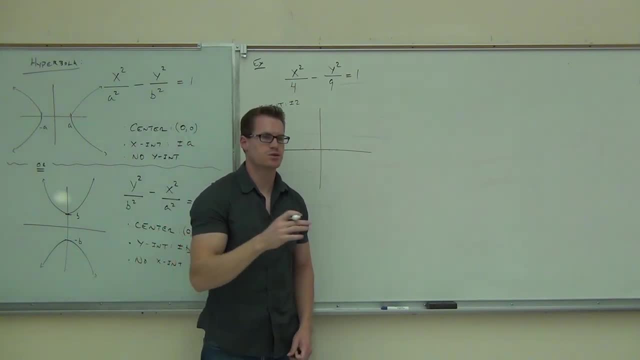 at 0, 0.. Of course, if you weren't centered at 0, 0, you could still do that right. It'd be just like doing that whole ellipse thing that we just covered. So here we're, centered at 0, 0.. We have 2 and negative 2 making our markers for the x-intercept, and we can go. 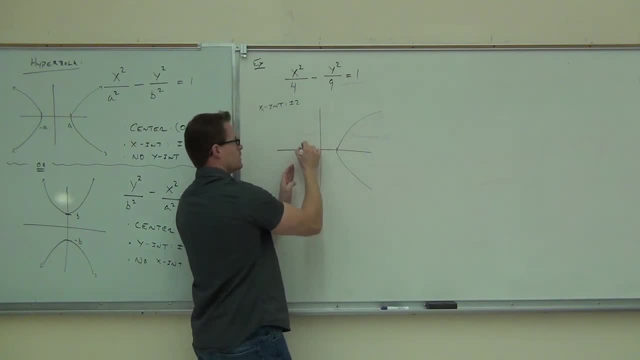 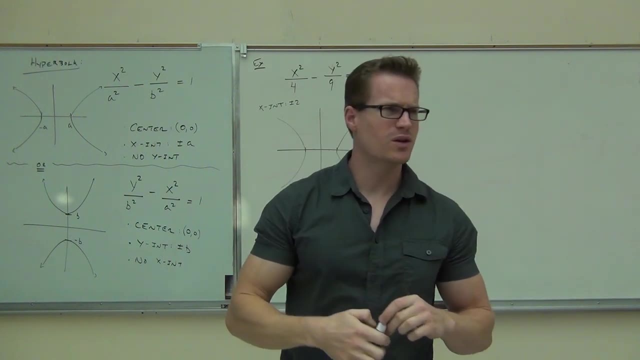 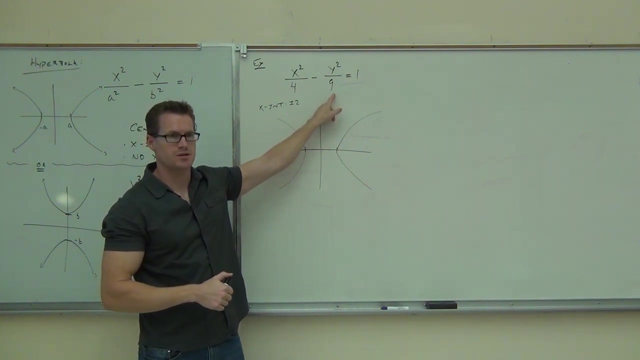 ahead and draw our hyperbola this way and that way. Raise your hand if you feel okay with that graph. Now, have you been wondering what this number does? Do you want to see what it does? Sure, Here's what this number does, According to an ellipse that would: 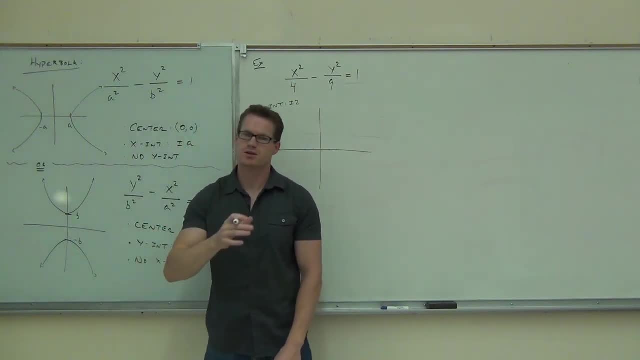 We're going to be centered at zero, zero. Of course, if you weren't centered at zero, zero, you could still do that, right? 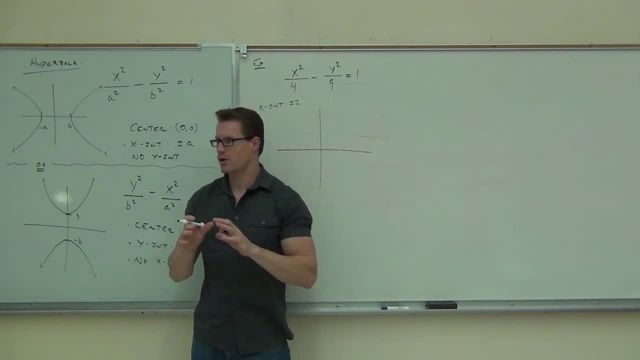 It'd be just like doing that whole ellipse thing that we just covered. So, here we're centered at zero, zero. We have... 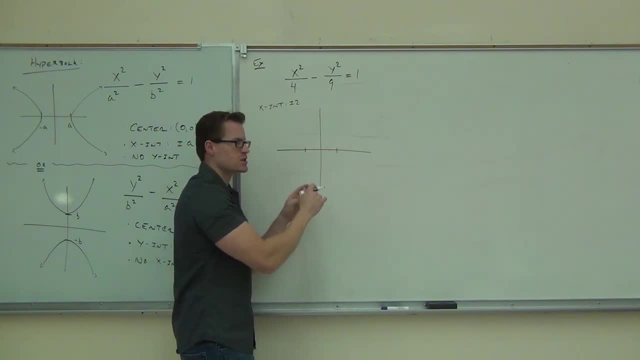 Two and negative two making our markers for the x-intercept, and we can go ahead and draw our hyperbola this way and that way. Raise your hand if you feel okay with that graph. 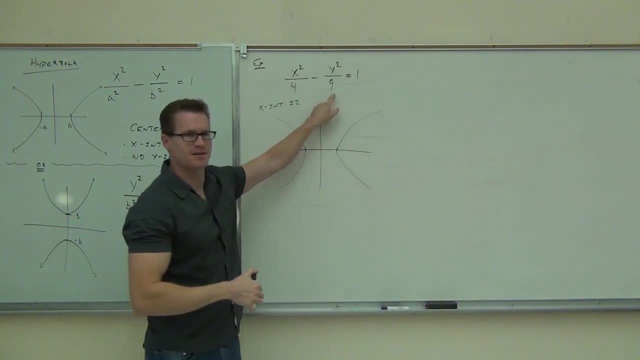 Now, have you been wondering what this number does? Yeah. Do you want to see what it does? Sure. 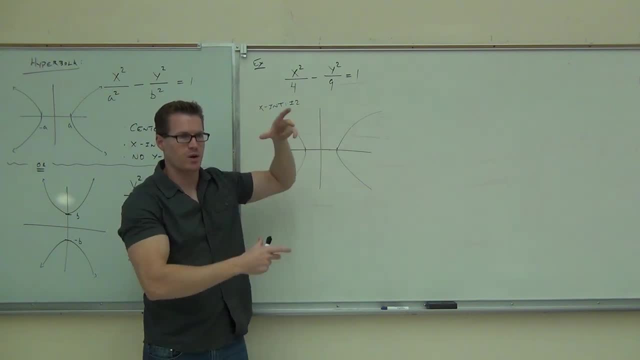 Here's what this number does. According to an ellipse, that would give us y-intercepts, right? Or the spread along the y. Now, of course, we don't have y-intercepts. 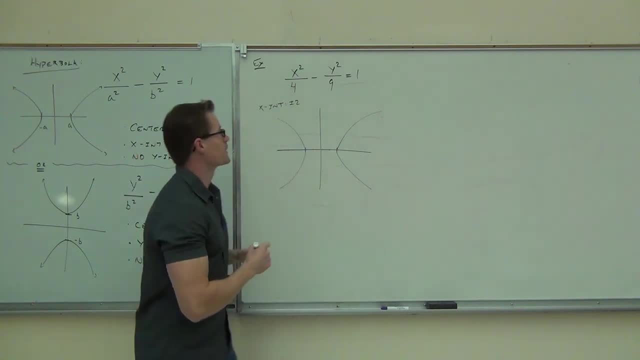 Here's what that number does. Here's what b does in this case. 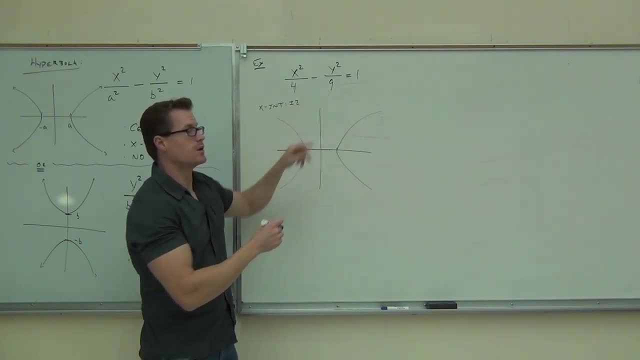 What number would we be looking for if those were y-intercepts? What would we have? 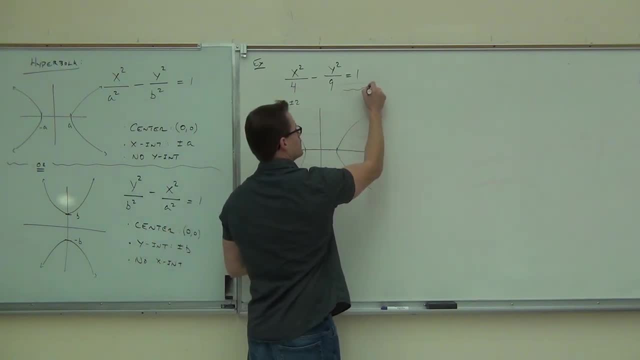 So the y-intercepts would be plus or minus three. So we would have, let's see, one, two, three, one, two, three. Do you agree that if this were an ellipse, it would cross at two, negative two, three, negative three? Mm-hmm. Okay. Here's what this does for hyperbola. 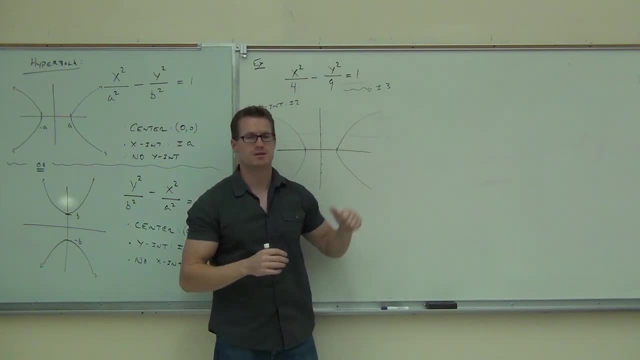 That still makes a difference here, but this is what it does. What you'd do with those numbers, see, this figure is exactly right. Right now, this looks like a parabola, and this looks like a parabola, doesn't it? 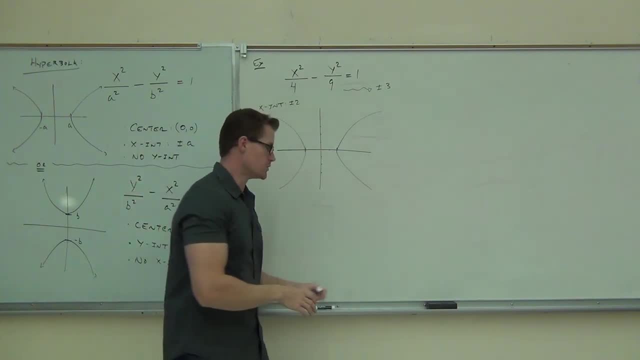 This looks like two, these aren't parabolas. Here's what these actually do. 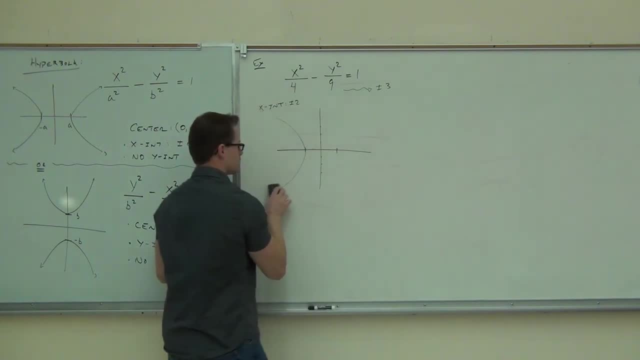 What I want you to do is erase this. What you do with your a's and your b's, you actually use those numbers. Right? 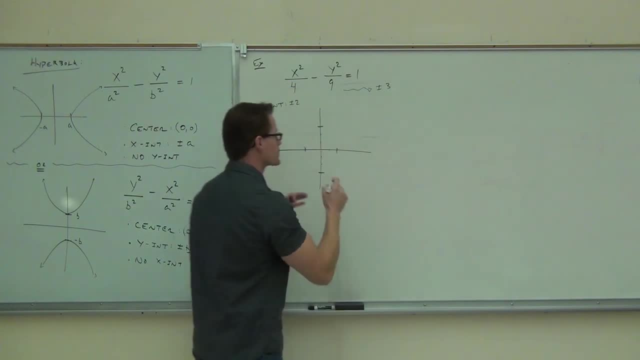 to make a box. So make a nice rectangular box around those. Here's how you do it. Okay, so let's recap. Can you find your x-intercepts? Sure. Can you find your y-intercepts, even though you don't really have y-intercepts? Now what's kind of nice about this, this gives you the shape of your hyperbola inherently with this box. What you're going to do, first you're going to say, are you okay with your box? What you're going to do now, make a diagonal line that goes through these corners, make a diagonal line that goes through those corners. 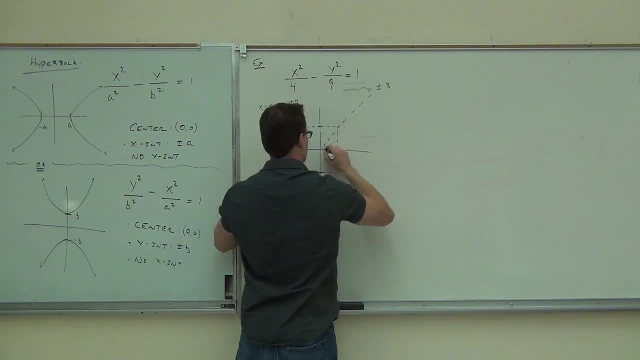 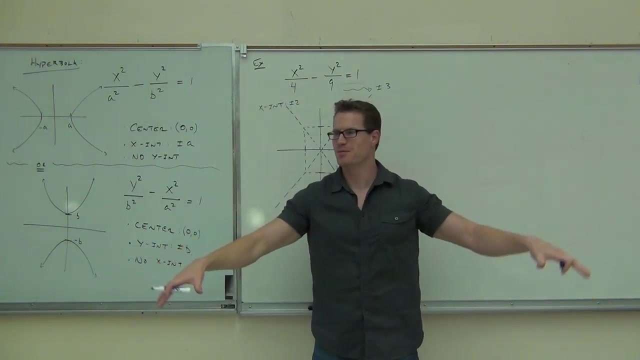 Oh, it looks kind of cool, right? Like something out of Star Wars, like a TIE fighter. No, that would be an X-Wing fighter. Oh my gosh, I made a faux fur coat. 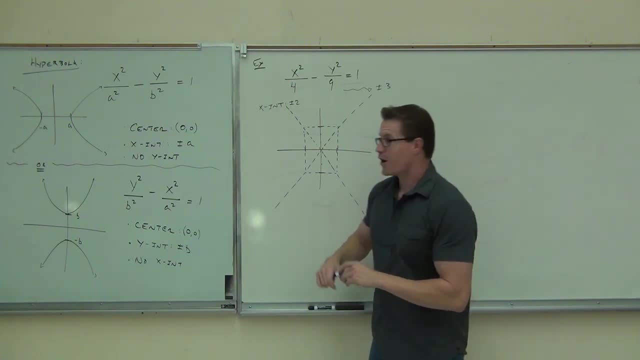 Oh, according to Star Wars lore, that's horrible. Are you all right getting your diagonal crosshairs 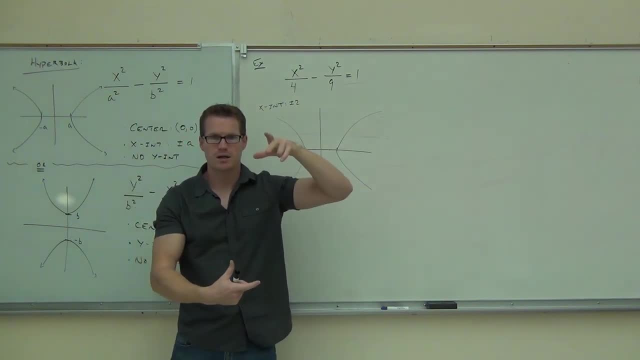 give us y-intercepts right, Or the spread along the y. Now, of course, we don't have y-intercepts. Here's what that number does. Here's what b does. in this case, What number 1? What would we be looking for if those were y-intercepts? What would we have? So the y-intercepts? 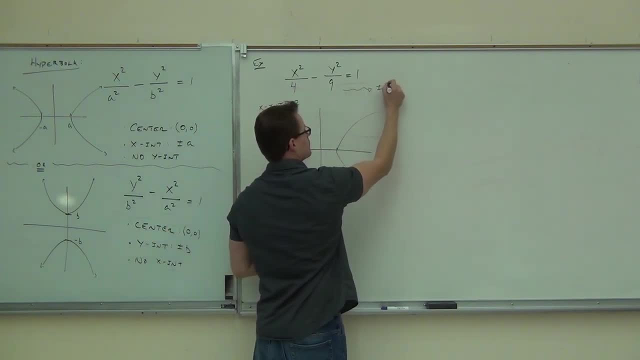 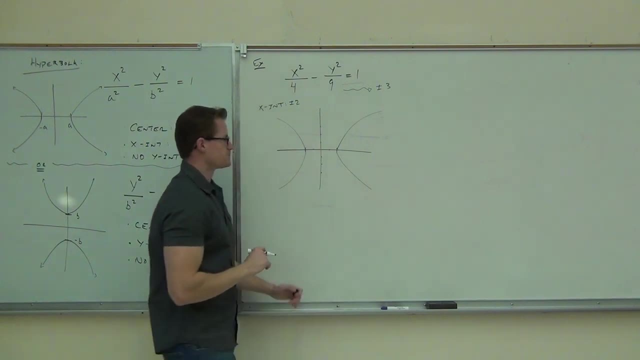 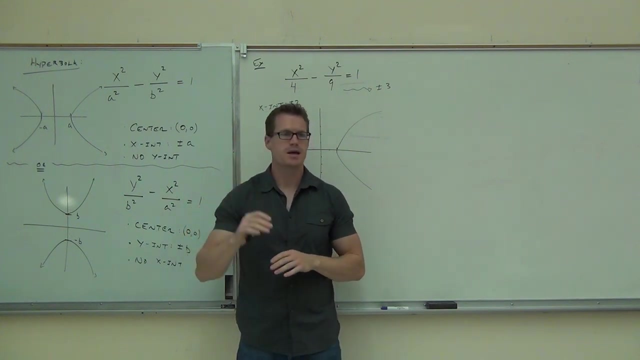 would be plus or minus 3.. So we would have, let's see: 1, 2, 3, 1, 2, 3.. Do you agree that if this were an ellipse, it would cross at 2, negative 2, 3, negative 3? Here's what. 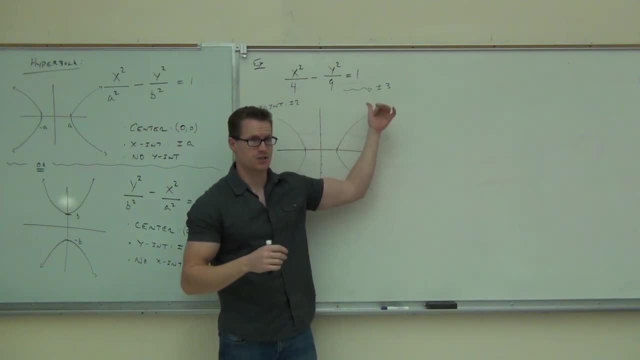 this does for hyperbola. That still makes a difference here, but this is what it does. What you do with this number is you're going to have a number that's going to be born 5.. There's 3 over there, here's 2, to make a big number. What goes? 8, minus 3,. 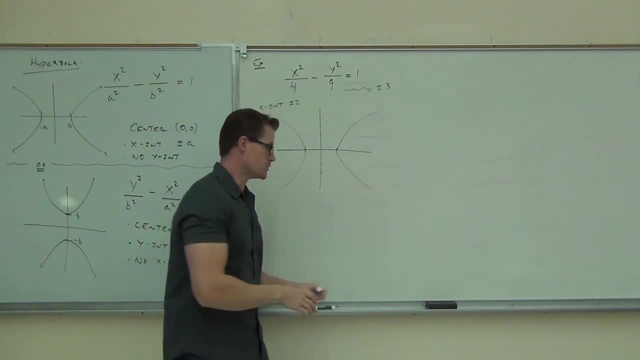 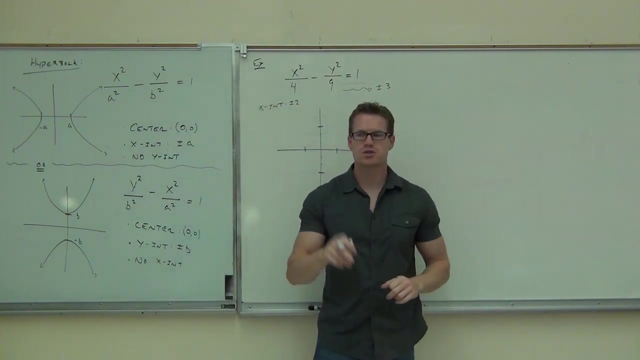 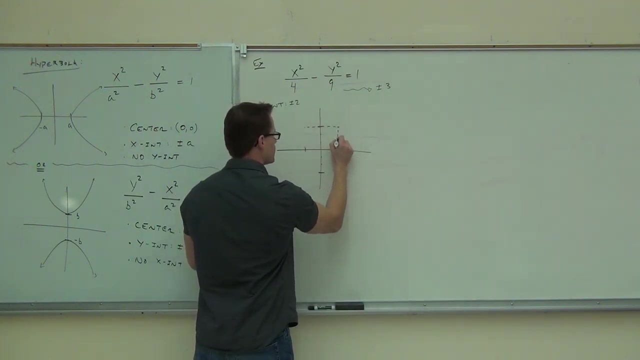 I don't know in1,, so it's at 2.. So if this were an ellipse, it would be 10, and I all agree that that's a big number, And so this will also be equal to that number. Okay, so let's recap. 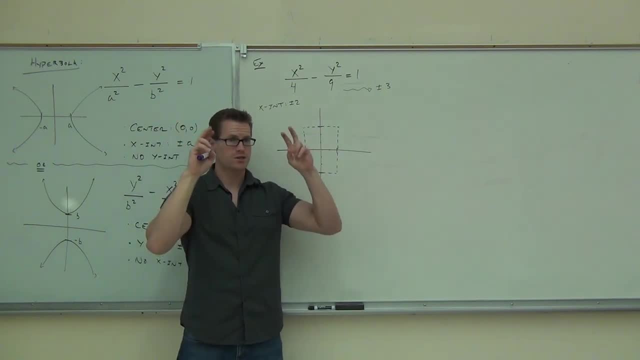 Can you find your x-intercepts? Sure, Can you find your y-intercepts, even though you don't really have y-intercepts. Now, what's kind of nice about this? this gives you the shape of your hyperbola, inherently with this box. 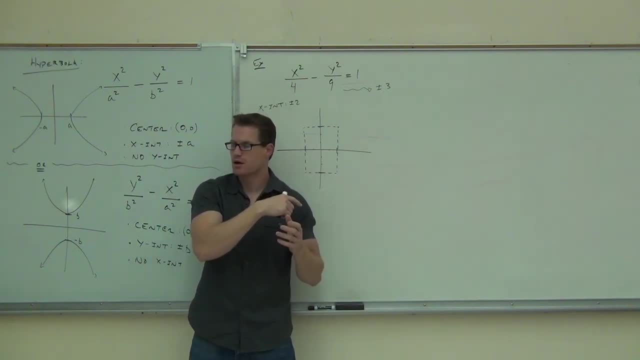 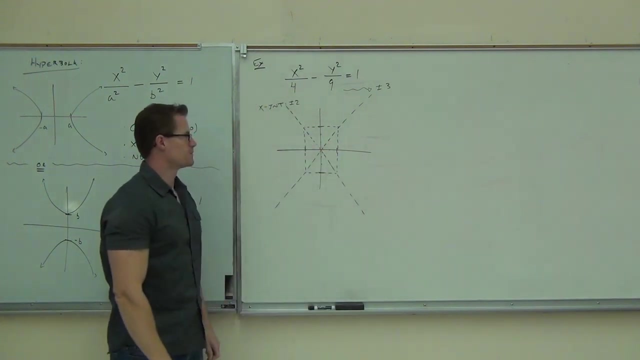 What you're going to do first of all. are you okay with your box? What you're going to do now? make a diagonal line that goes through these corners. Make a diagonal line that goes through those corners. Oh, it looks kind of cool, right. 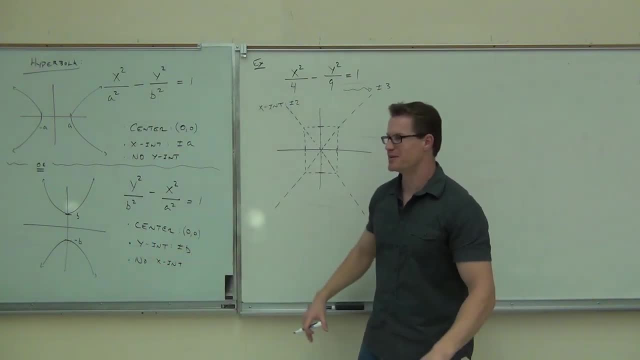 Like something out of Star Wars, like a TIE fighter. No, that would be X-Wing fighter. Oh my gosh, I made a faux pas. according to Star Wars lore, That's horrible. Are you all right getting your diagonal crosshairs across your graph? 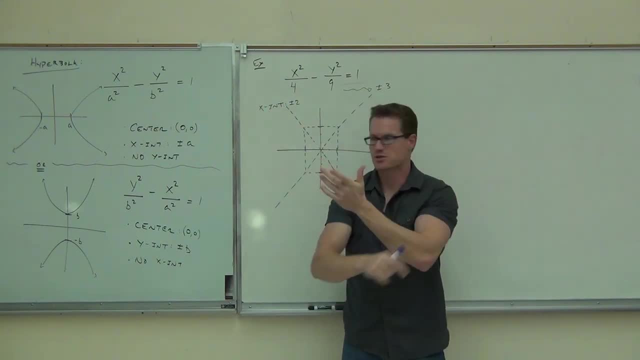 across your graph? Yeah? This is how, so according to this, yeah, you'd still have a B and a 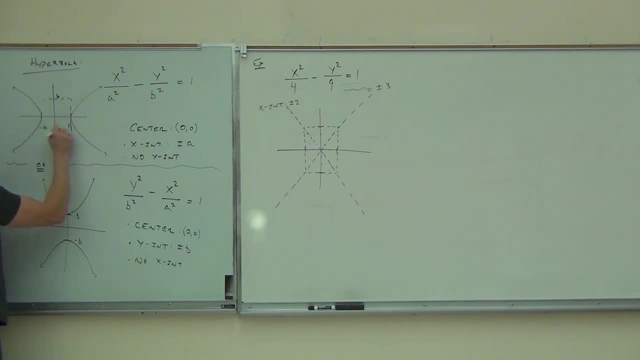 negative B. But what that does, makes it a box for you. It makes up diagonal lines. Here's how you use that to your advantage. 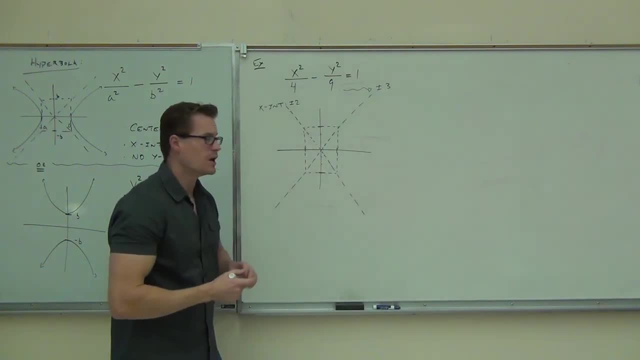 You see, this right here tells you the shape of your hyperbola. Now, you already know it's 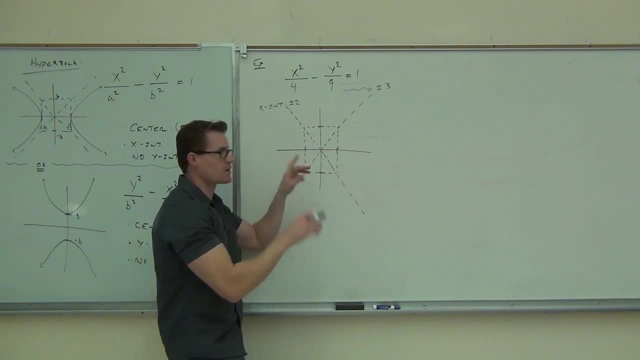 going to be here. You already drew that graph, right? I just erased it. You already know it's going to be here, it's going to be here, and it's going to go this way. You follow? 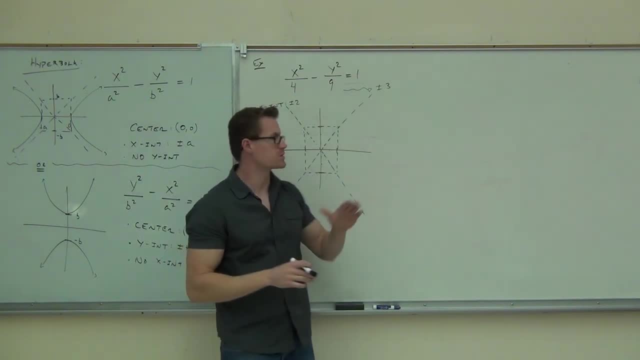 These lines give you what are called asymptotes. Hyperbolas are asymptotic to those lines that 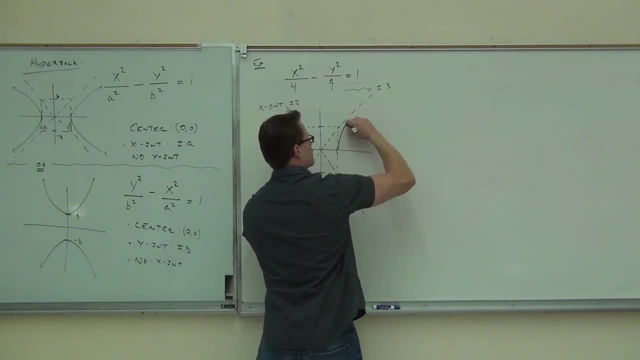 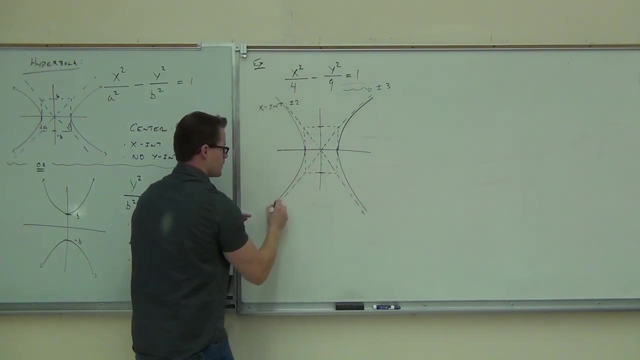 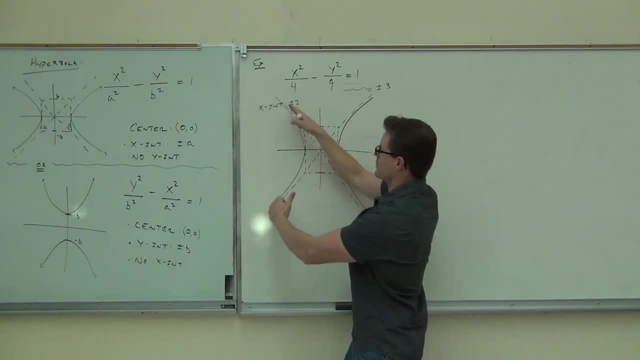 it's not a parabola. It's going out forever, like that, and like that. It's getting closer and closer to those diagonal lines. Is it ever going to touch them? No. But it follows 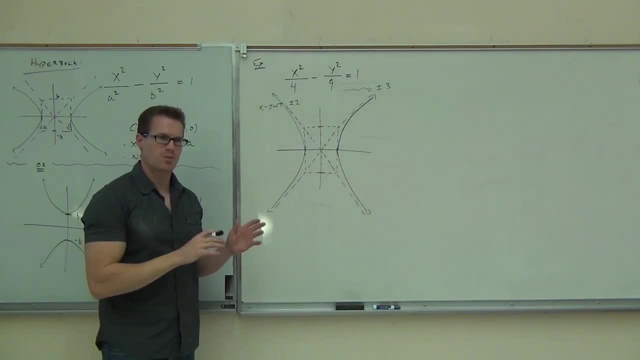 them. Do you guys now see the shape of your hyperbola? You can see a lot better with that box thing, can't you? It's not a parabola. It's not the same thing. Otherwise, we'd have 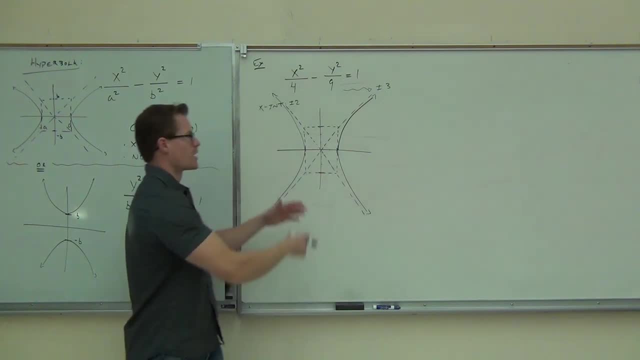 called these parabolas and say, oh, they're just two of them. That's not the same thing. 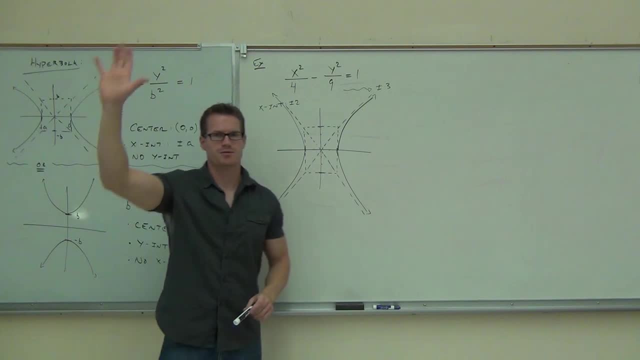 They're hyperbolas. They're weird shapes. Kind of nice. How many of you understand the idea of hyperbolas? All right, good. Tell you what, why don't you try one of your own. We'll do one together, then I'll do that recap, give you your test review, and be done. 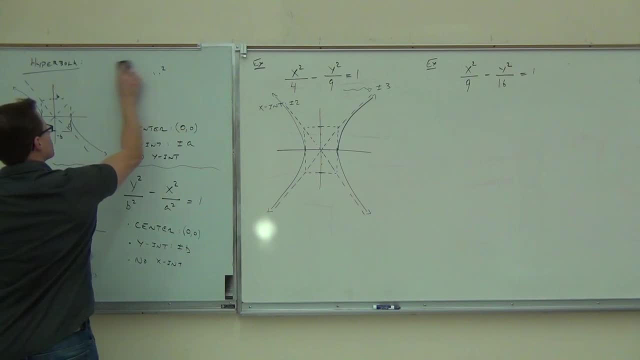 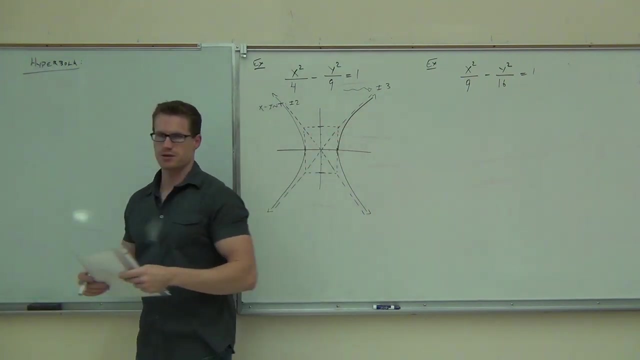 Are you feeling like a rock star, and you understand this one? Why don't you try the next one I put on the board, too. We're going to do that just after that. I'm going to go quickly through it, too. . . . 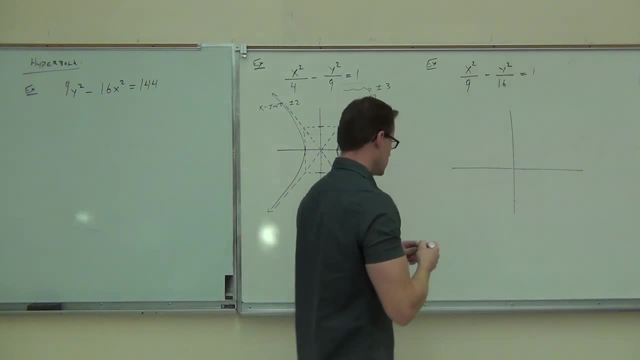 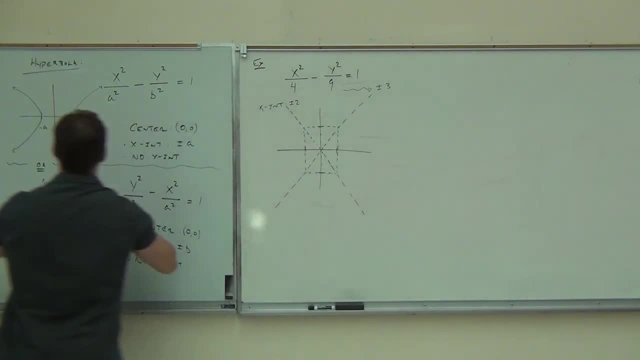 Yeah, This is how. so according to this, yeah, you'd still have a B and a negative B, But what that does? it makes it a box for you and makes up diagonal lines. Here's how you use that to your advantage. 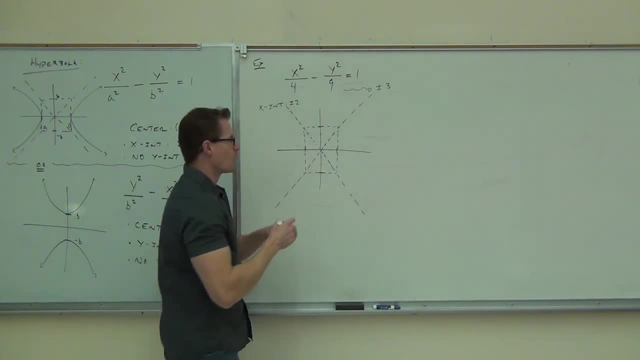 You see this right here tells you the shape of your hyperbola. Now, you already know it's going to be here. you already drew that graph right. I just erased it. You already know it's going to be here. It's going to be here. 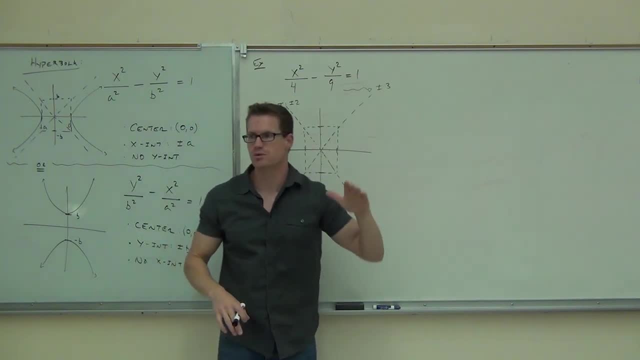 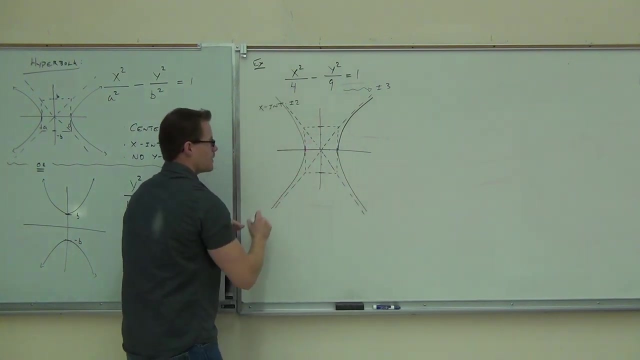 It's going to go this way. You follow These lines, give you what are called asymptotes. Hyperbolas are asymptotic to those lines that you drew through your box. So you go like this and you follow that, and you follow that. 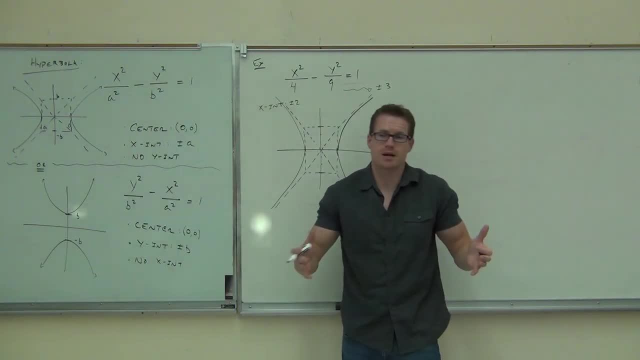 That's actually how the hyperbola looks. It's not a parabola. It's going out forever like that and like that. It's getting closer and closer to those diagonal lines. Is it ever going to touch them? No, But it follows them. 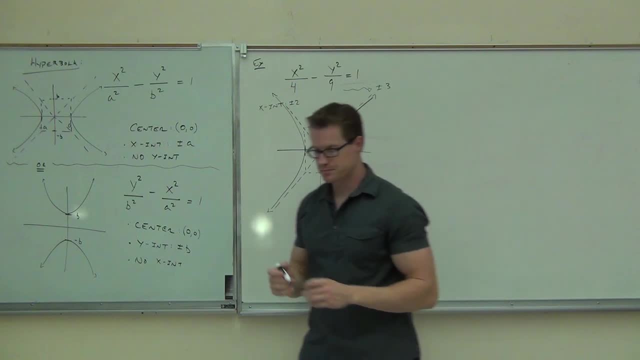 Do you guys now see the shape of your hyperbola? You can see a lot better with that box thing, can't you? It's not a parabola, It's not the same thing. Otherwise we'd have called these parabolas and say, oh, there's just two of them. 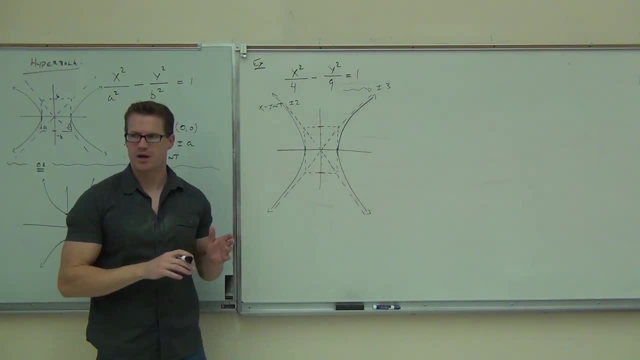 That's not the same thing. They're hyperbolas. They're weird shapes, Kind of nice. How many people understand the idea of hyperbolas? Not that good. All right, Let's see. Let's see, Let's see. 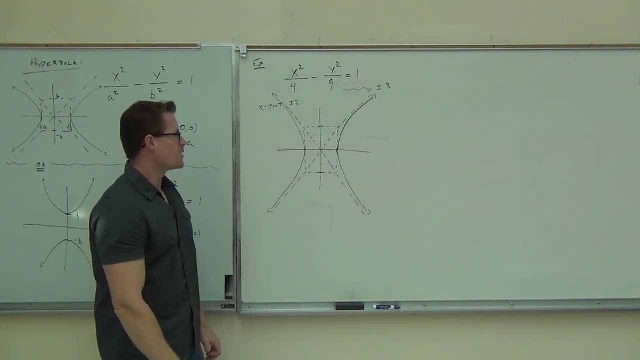 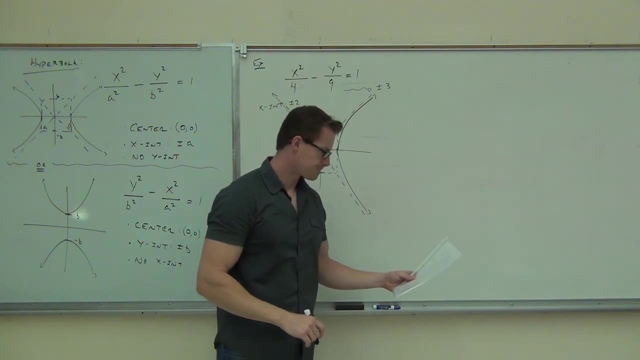 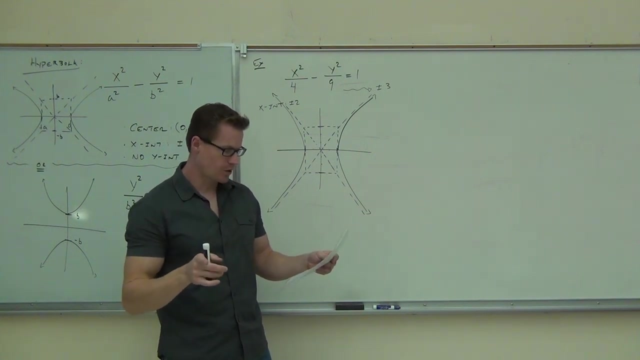 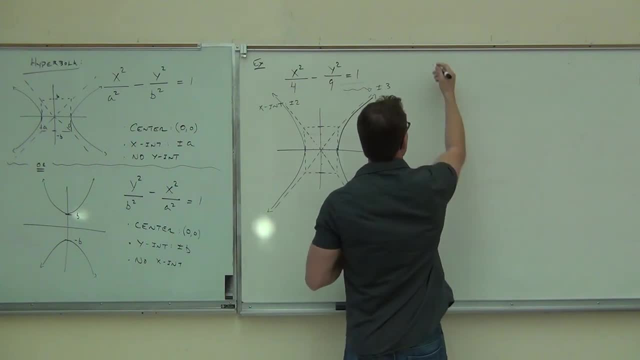 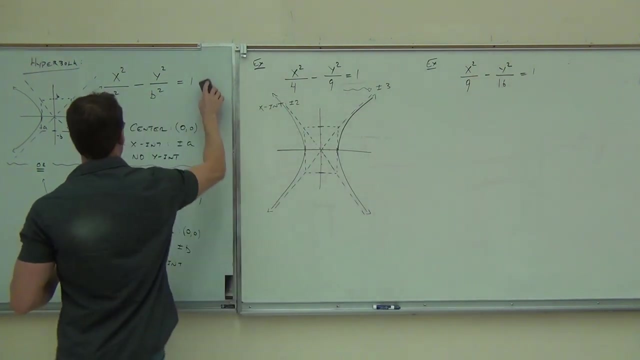 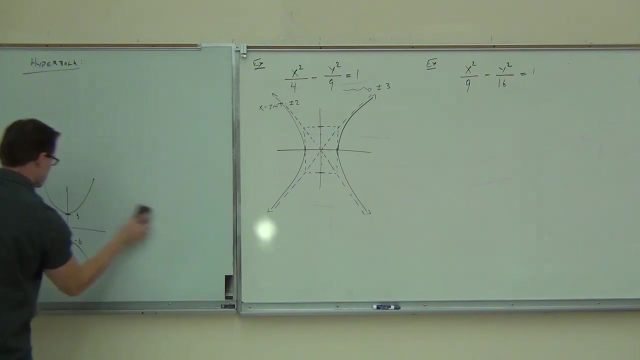 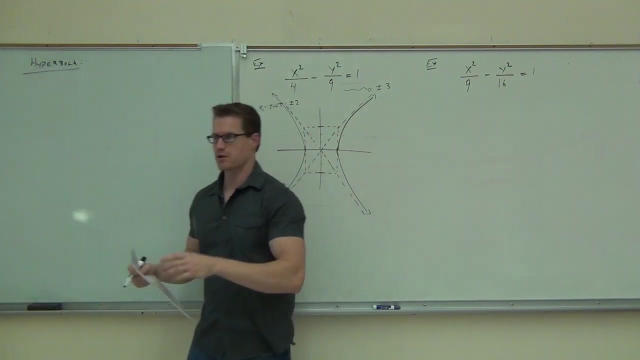 We'll do one together. then I'll do that recap, give your test review. Are you feeling like a rock star? and you understand this one? Why don't you try the next one? we put on the board too? We're going to do that just after that and we'll quickly through it too. 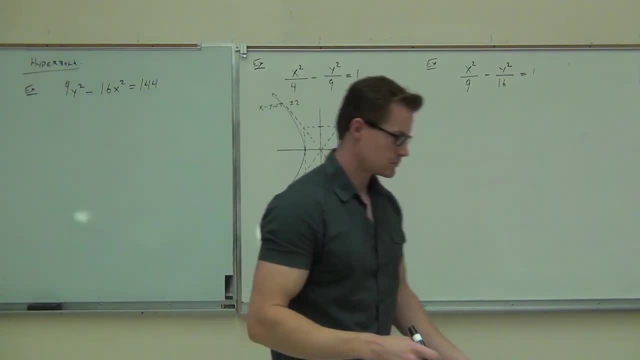 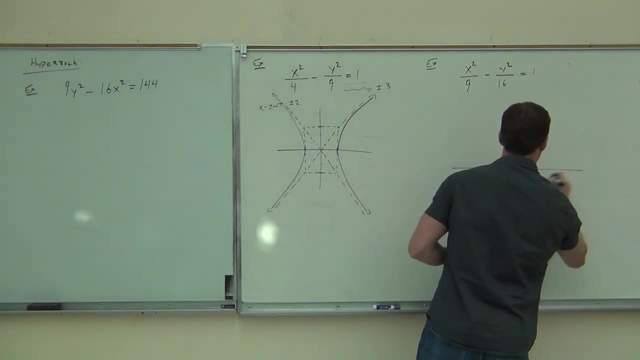 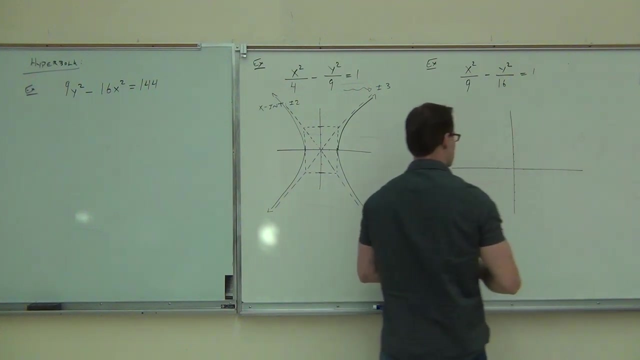 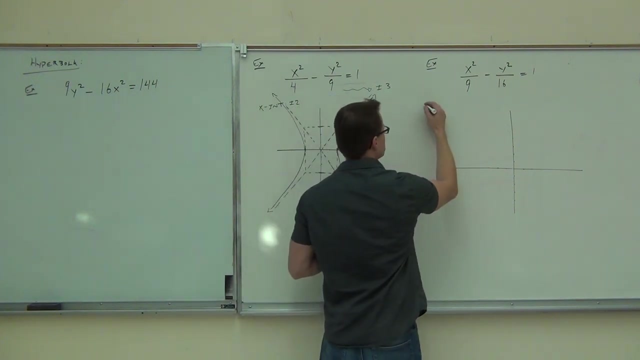 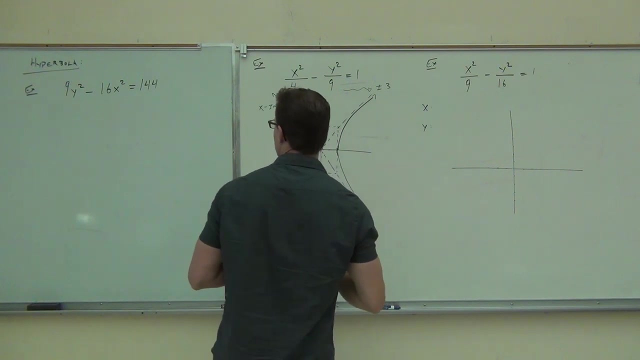 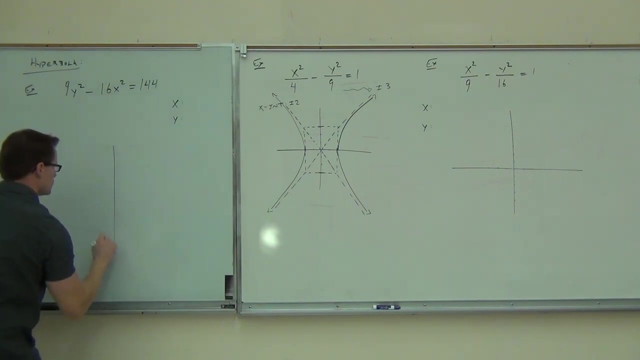 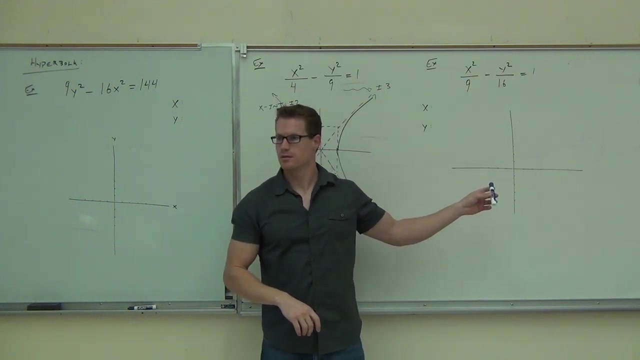 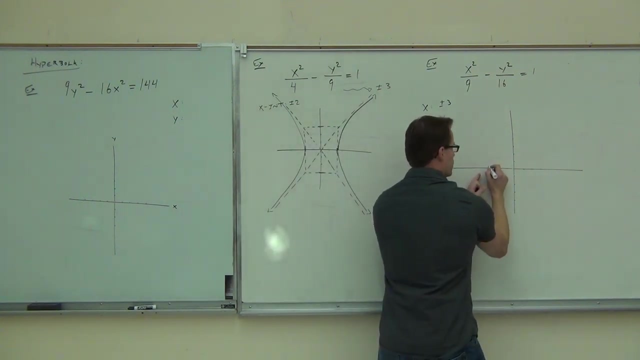 So we're going to make a box around. plus or minus x equals 3 and plus or minus 4 along our y. 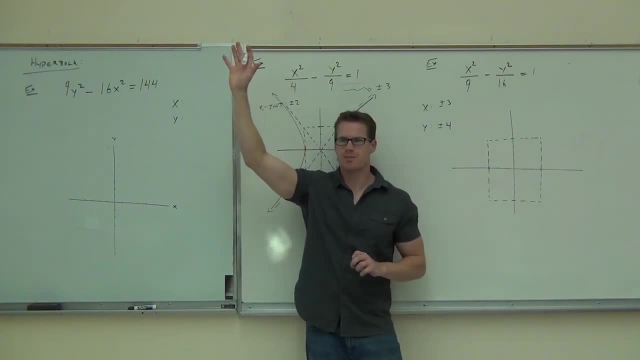 Would you raise your hand if you made it that far? You get that box and everything, All right. what do you do with that box? How does that help us Cross areas? that's right. Make the x through the corners of our box. 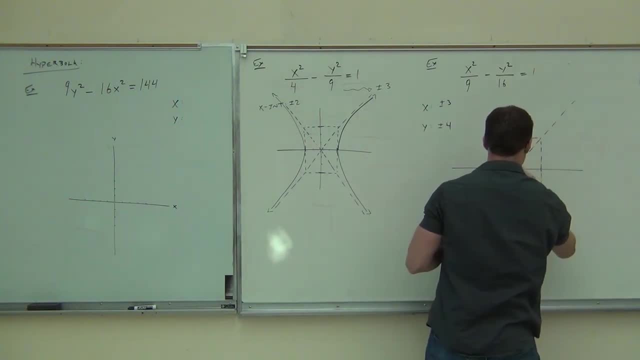 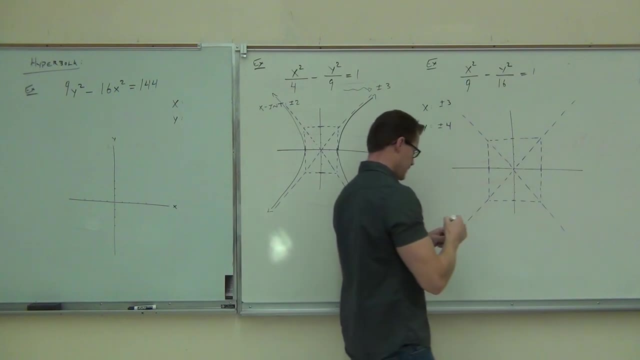 Now can you see that, whether y or x comes first, you're going to have some sort of a box, right, It's going to give you the same exact box. What changes is? which direction are you going? Are you going the y direction or the x direction? 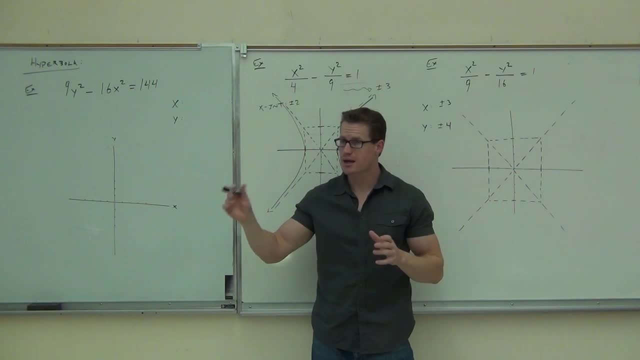 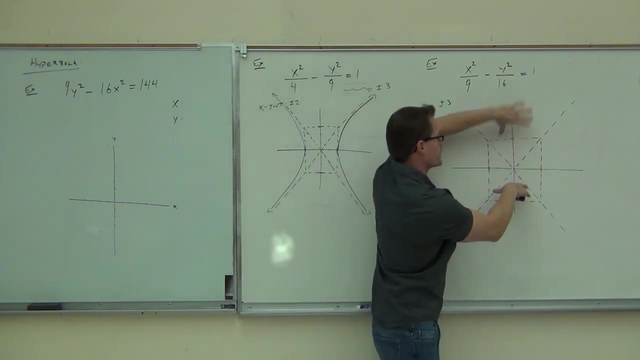 That's why we had to know which letter. Which letter comes first, our x or our y. If our x comes first, we're this way. If our y had come first, you'd have the same exact box. only if you're going this way, 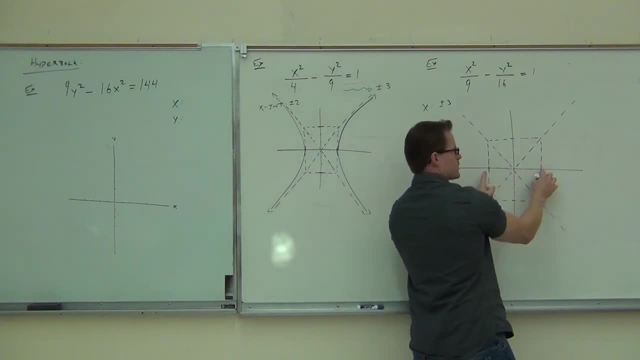 Do you guys see that on your graph? So here, sure, we're intersecting here and here because x came first. That means x intercepts and no y intercepts and we're going to be asymptotic. That means we're going to get really close to those diagonal lines. 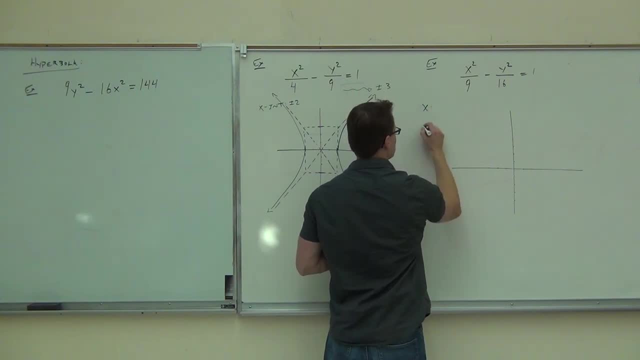 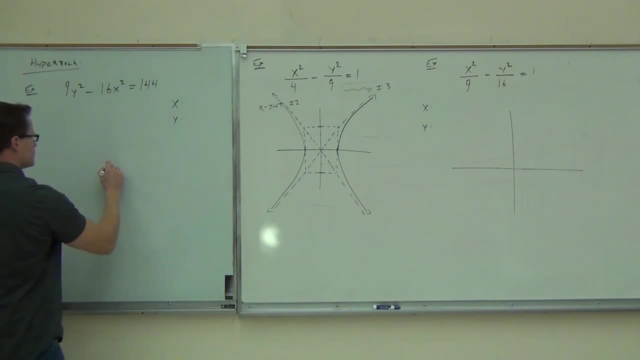 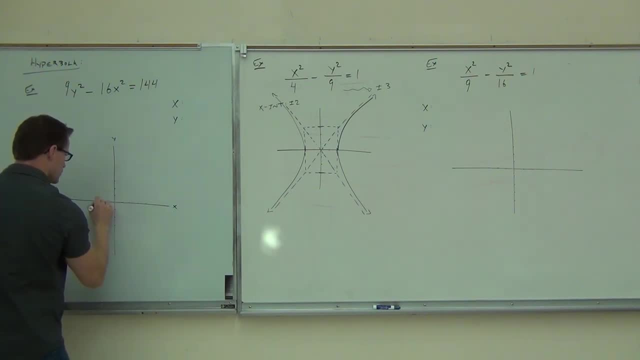 Are we able to do that one? 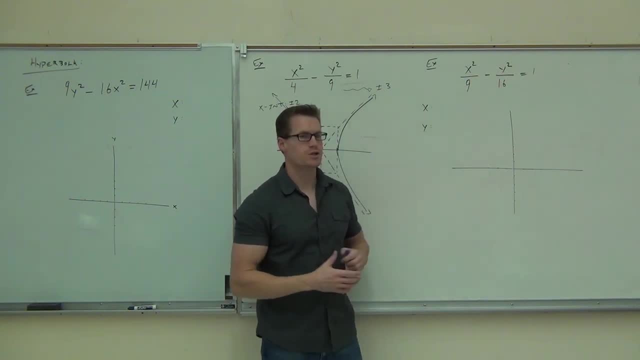 Let's take a look at it. Firstly, identify what shape it is. Can you tell that it is, in fact, a hyperbola? 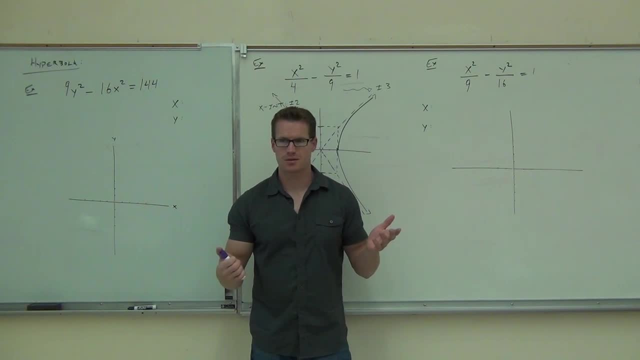 What gives it away? Minus. That's kind of nice, right? 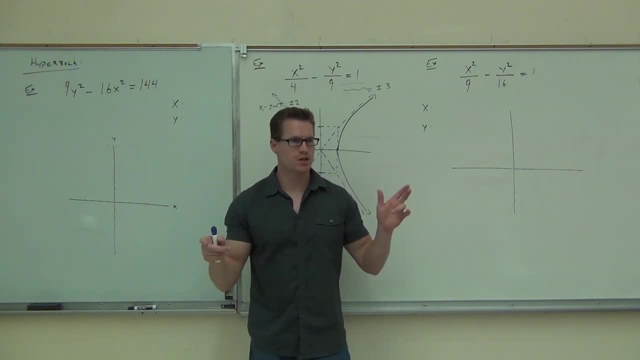 Minus, you get x squared, y squared with a minus between them. Which direction is it going? X direction or y direction? X direction. So very similar to this one over here. 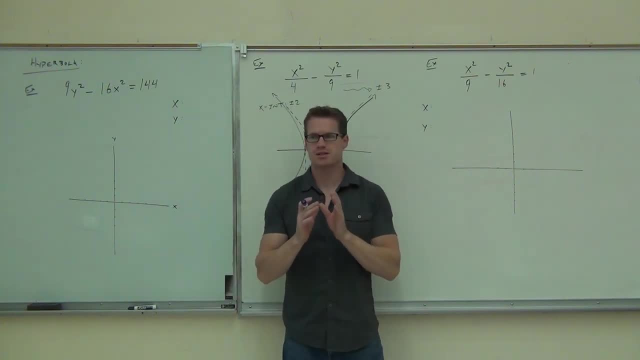 Make your box up. What is your x intercepts here? 3 plus minus. Good, okay. So plus minus 3. 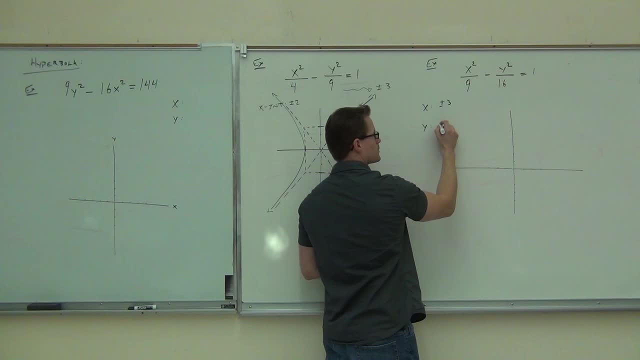 And here for our y's? 4. So we're going to make a box around plus or minus x equals 3, and plus or minus 4 along our y. 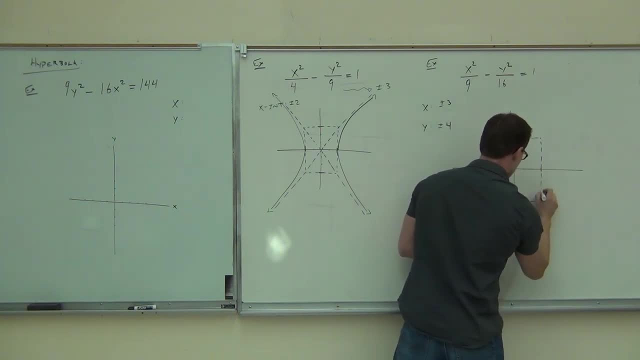 Well, it's amazing how you made it that far. You get that box and everything. All right, what do you do with that box? How does it help us? Cross the error. Cross the errors, that's right. Make the x through the corners of our box. Jesus, what was he doing? He waszzle, he waszzle, and he wash Fall exposed. All right, what else was he manicuring? 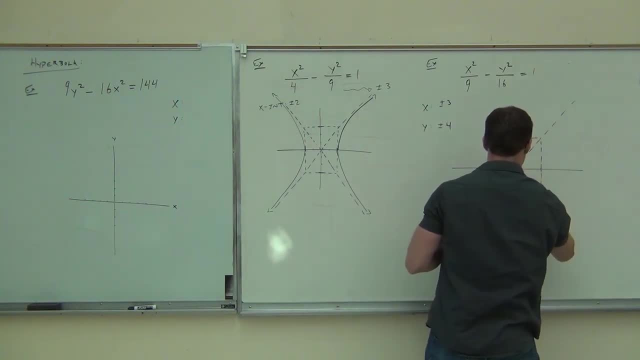 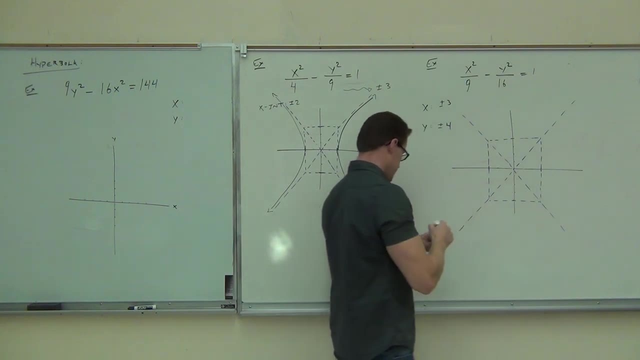 MUSIC That's it. 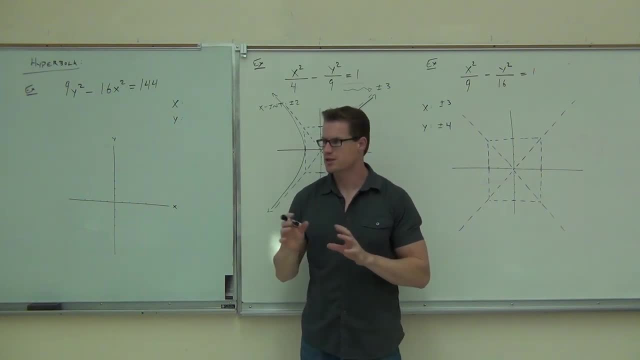 Now, can you see that whether y or x comes first, you're going to have some sort of a box, right? It's going to give you the same exact box. What changes is which direction are you going. Are you going the y direction or the x direction? That's why we had to know which letter comes first, our x or our y. If our x comes first, we're this way. 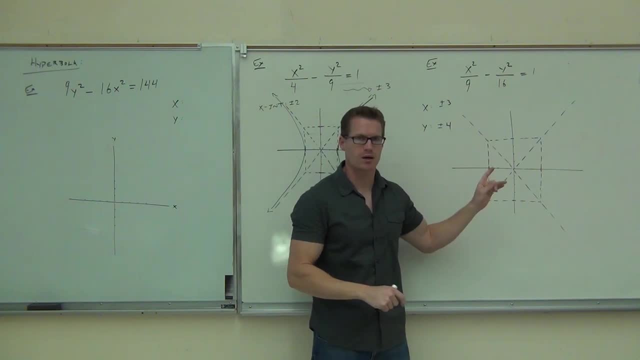 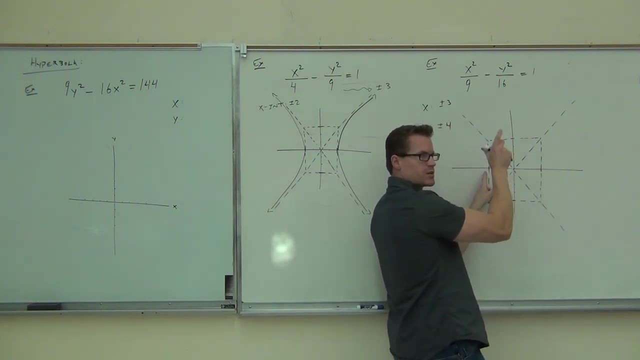 If our y had come first, you'd have the same exact box, only if you're going this way. Do you guys see that on your graph? So here, sure, we're intersecting here and here because x came first. That means x intercepts, no y intercepts, and we're going to be asymptotic. That means we're going to get really close to those diagonal lines. Ooh, that was a good one. Not bad. Do you have that graph on your paper? Uh-huh. 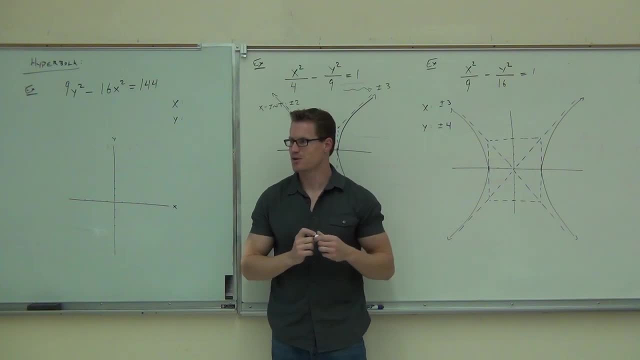 Okay. Kind of neat looking? It'll draw these pretty fantastically. It shapes pretty easily, right? Not a whole lot of work. 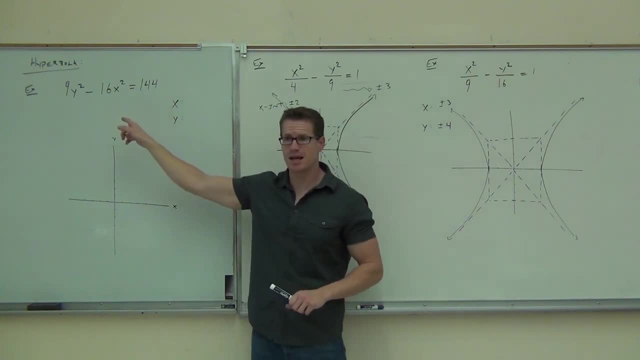 Now, let's try that one. Firstly, can you identify what shape it is? Is it a parabola? No. That's a silly question. Is it a circle? No. Hyperbolic? Circle? No. It is. Hyperbolic. Sure. What gives it away again? Line sign. 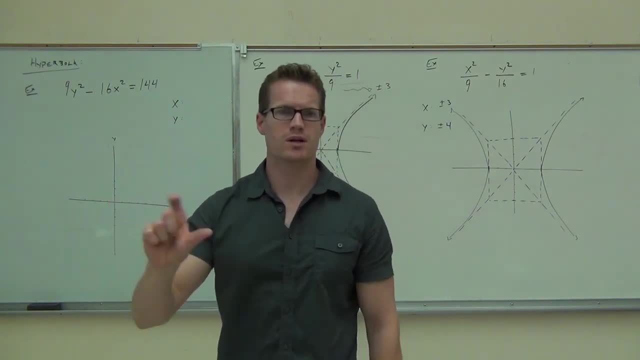 Line sign. Yeah, we talked about that. Now, what do you have to do to get that in the form that you want it to be in? Divide that by 144. Let's do that. So if I divide everything by 144. 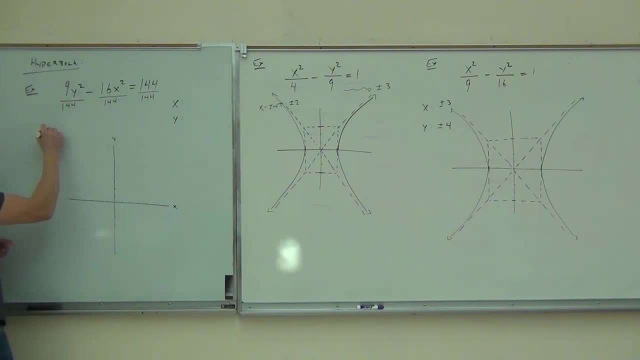 We're going to get Y squared over 16 minus X squared over 9 equals 1. Okay. 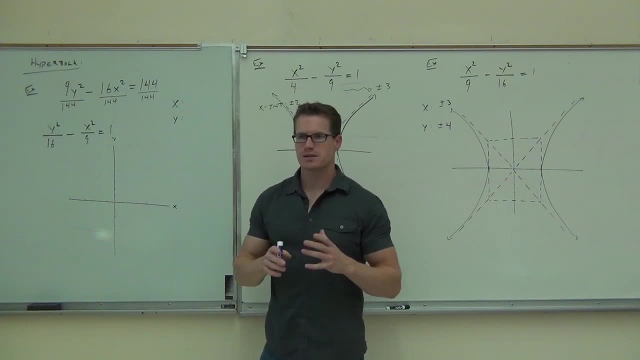 Okay. Can you tell me what are my X intercepts here as far as the box goes? What are my X intercepts? Wait. Why not 16? Because 16 came first. 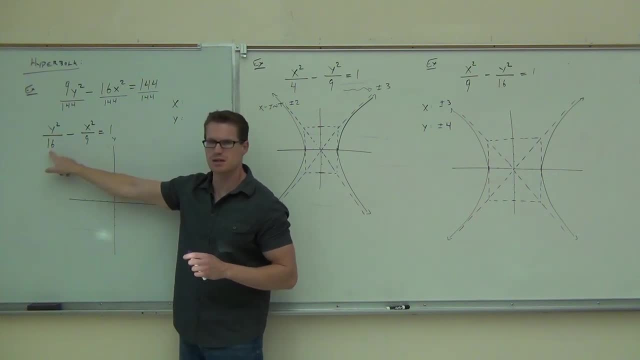 Why 9 and not 16? Why does that give me my X intercepts here in this case? 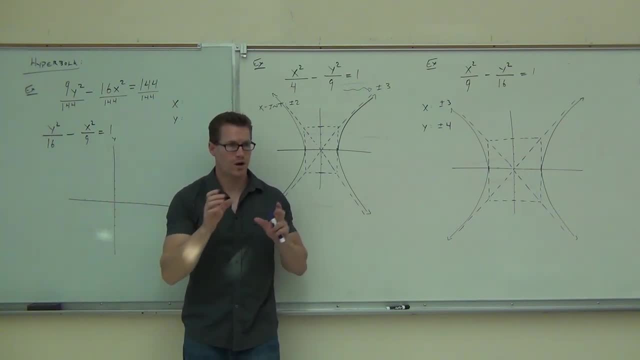 Okay. So no matter where the X is, where that X is tells you how far you spread your box out along the X axis. Does that make sense? 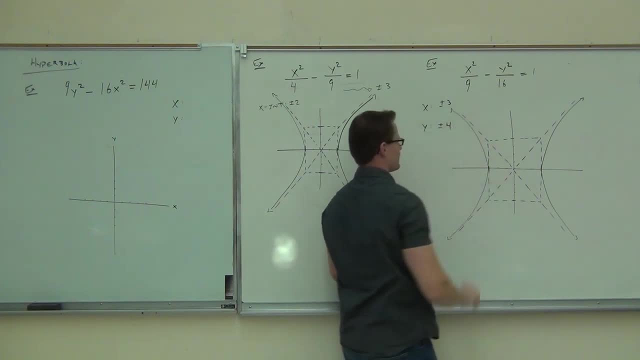 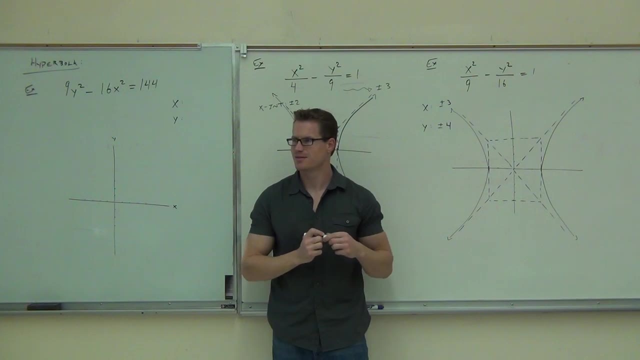 Ooh, that was a good one, Not bad. Do you have that graph on your paper? Uh-huh, Okay, Kind of neat looking. It'll draw these pretty fantastically. shapes pretty easily, right? Not a whole lot of work. 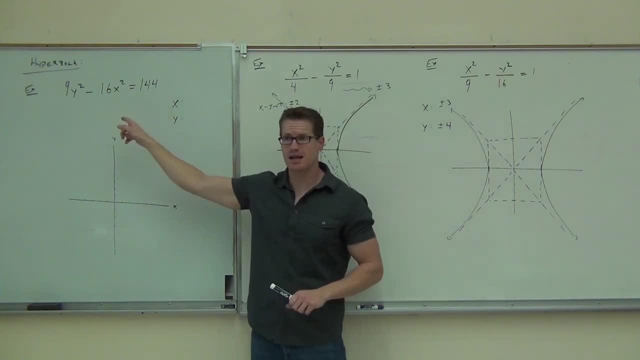 Now, let's try that one. Firstly, can you identify what shape it is? Is it a parabola? No, That's a silly question. Is it a circle? No, Hyperbola Circle. No, It is. 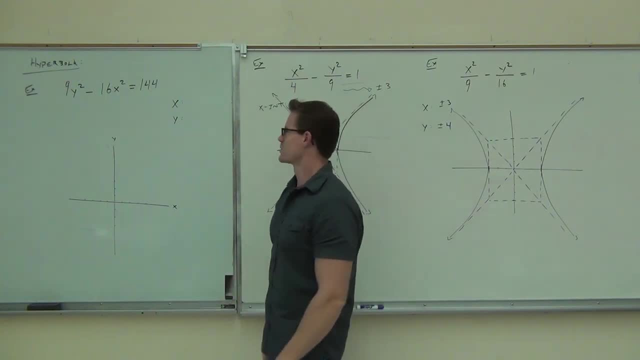 Hyperbola Sure. What gives it away again? Minus sign, Minus sign. Yeah, we were going to talk about that. Now what do you have to do to get that in the form that you want it to be in? 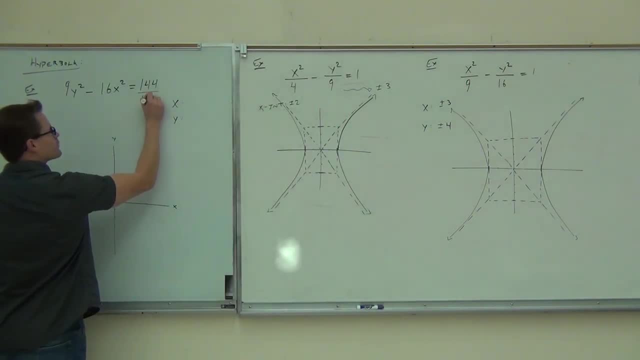 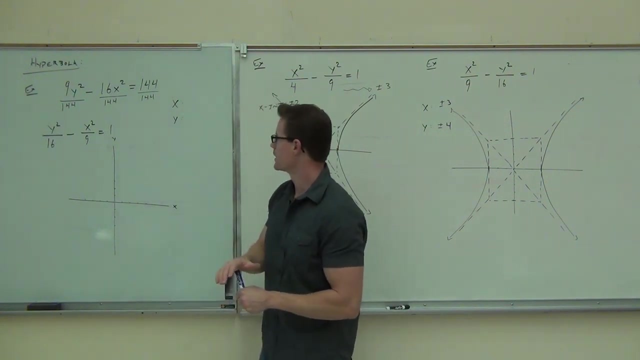 Divide that by 144.. Let's do that. So if I divide everything by 144, we're going to get y squared over 16.. Very good, Minus x squared over 9 equals 1.. Okay, Can you tell me what are my x intercepts here? as far as the box goes? 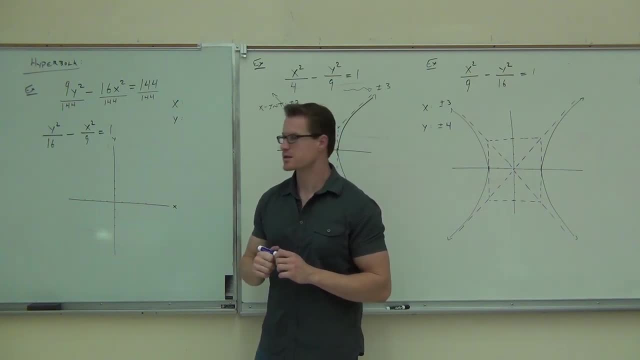 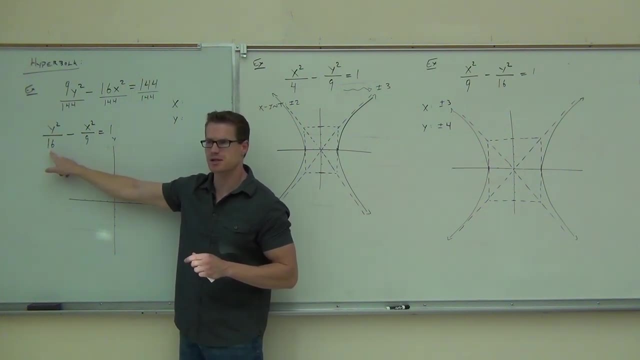 What are my x intercepts Minus 3.. Wait, why not 16?? Because 16 came first. Why 9 and not 16?? Why does that give me my x intercepts here? in this case, Because it's under the x square. 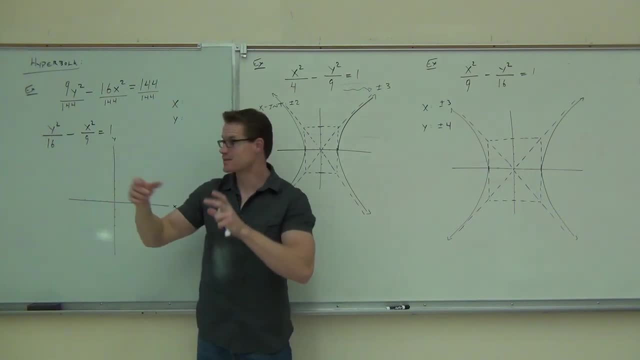 Okay. So, no matter where the x is, where that x is tells you how far you spread your box out along the x axis. Does that make sense? So, even if it's the second one that still tells you, It tells you your distance, x right, in the form of x plus and minus 3.. 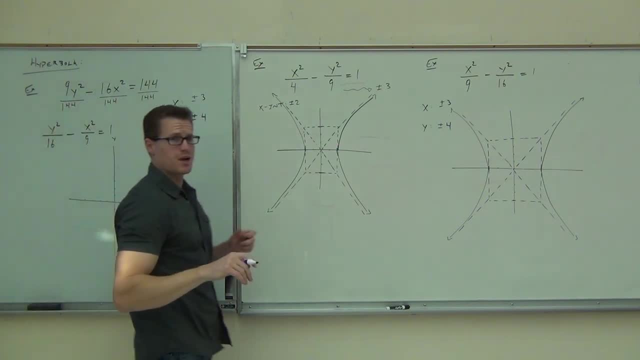 And the y axis says plus and minus 4.. Do you see where the 3 and the 4 are coming from? The 9 is under the x. That means along the x, plus or minus 3. That's the square root of 9.. 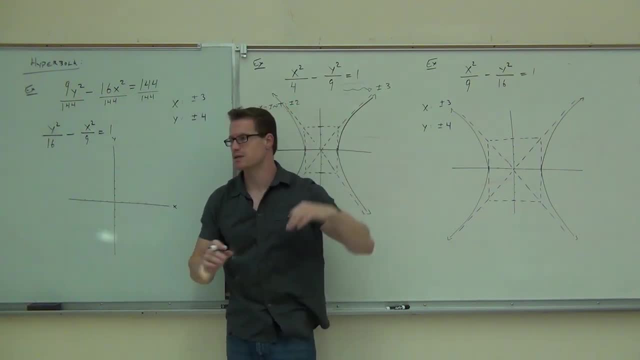 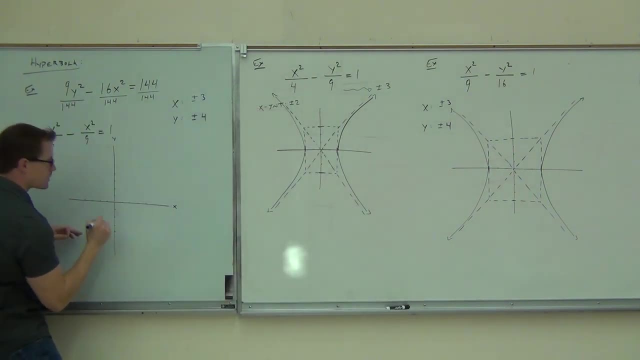 16 is under the y. That means along the y, plus or minus 4.. That's the square root of 16.. So let's go ahead and let's make this box up. We know we're going to be plus or minus. oh, I forgot one. 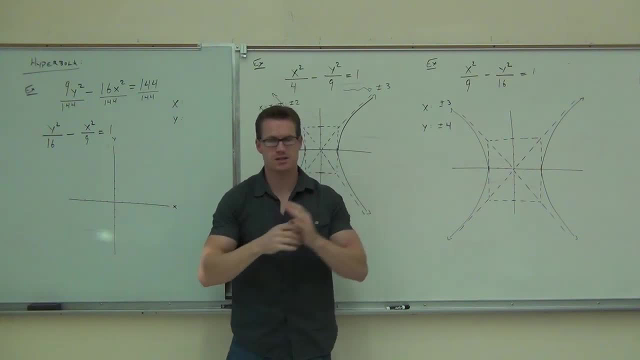 So even if it's the second one, that still tells you your distance X, right in the form of X. Plus and minus 3. 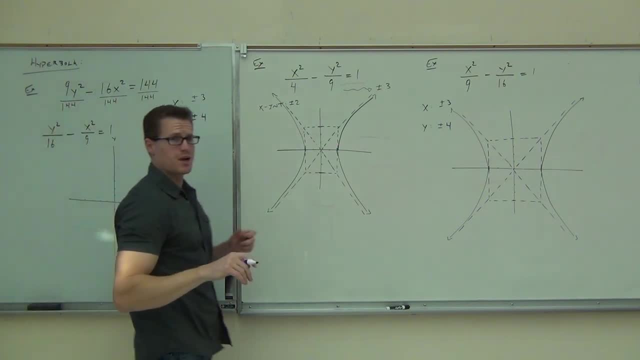 And the Y axis says plus and minus 4. Do you see where the 3 and the 4 are coming from? The 9 is under the X. 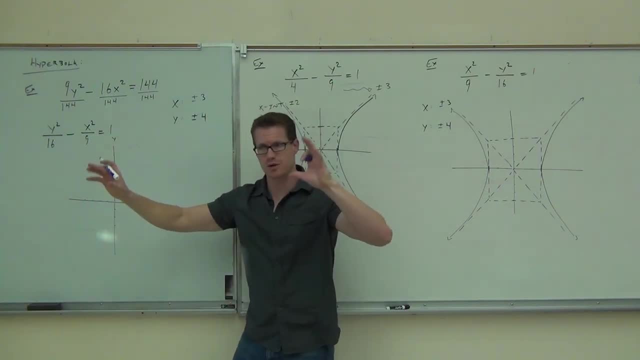 The 9 is under the X. That means along the X plus or minus 3. That's the square root of 9. 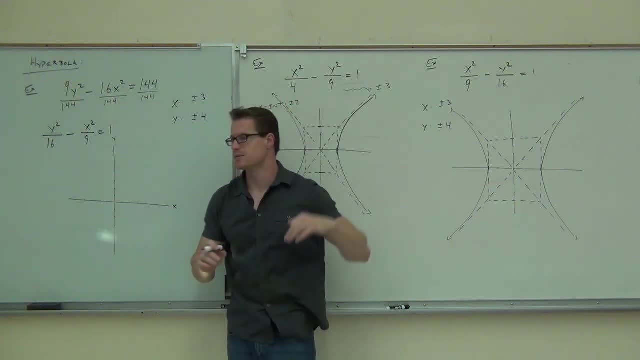 16 is under the Y. That means along the Y plus or minus 4. That's the square root of 16. 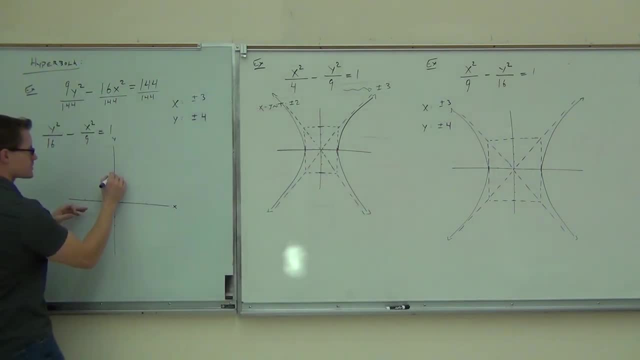 So let's go ahead and let's make this box up. We know we're going to be plus or minus, I forgot one, plus or minus 4 along the Y, plus or minus 3 along the X. Here's 3, 3. Here's 4, 4. 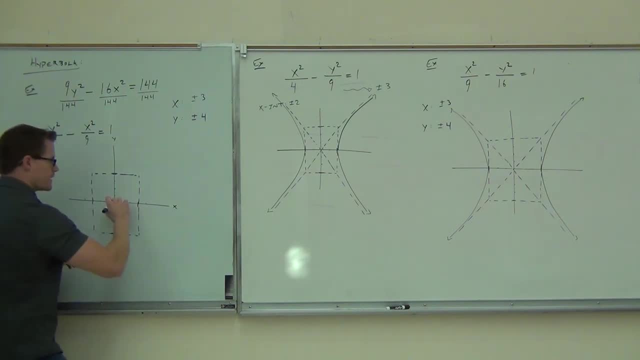 We'll make our diagonal line just like we did before. Notice how the process is not changing. 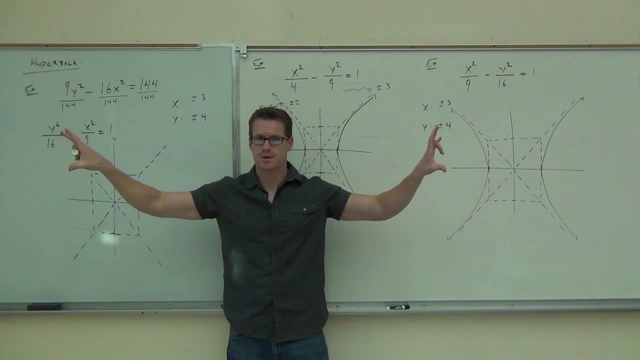 The only thing you've got to determine is where it goes. Is it going this way or this way? Yeah, it's vertical. Why is it vertical? 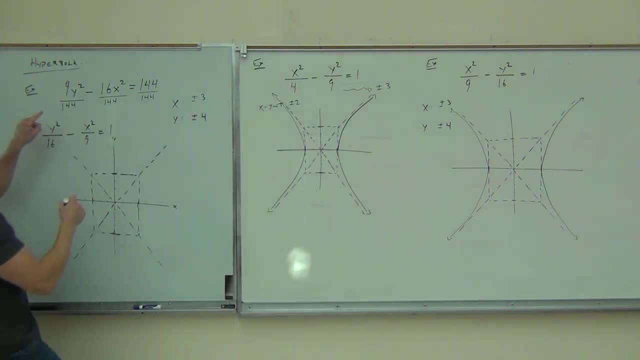 So we'll go ahead and draw that. The Y came first. 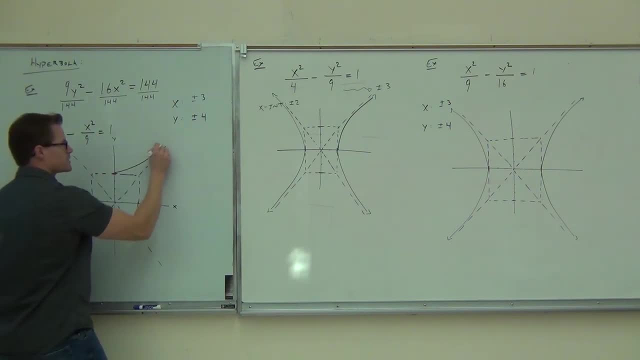 That means we're spread out along the Y axis. We will have Y intercepts but no X intercepts. And that's the only way we can draw that. 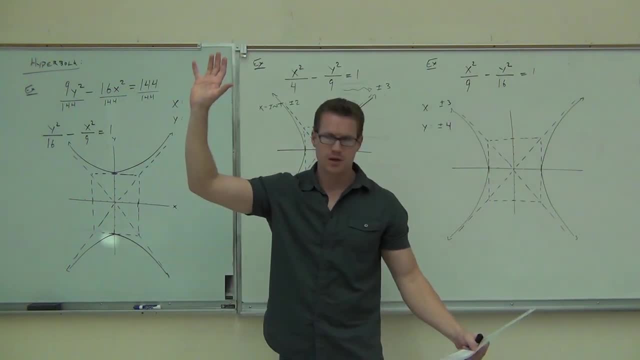 Would you raise your hand if you feel okay with our hyperbolas so far? Okay. 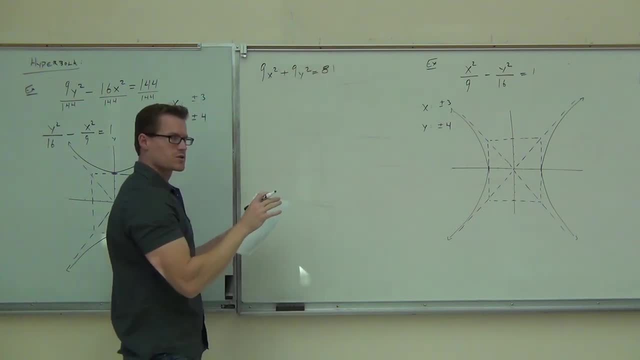 We're not going to do these problems, so don't worry. I just want to make sure you can identify what they are. Okay. 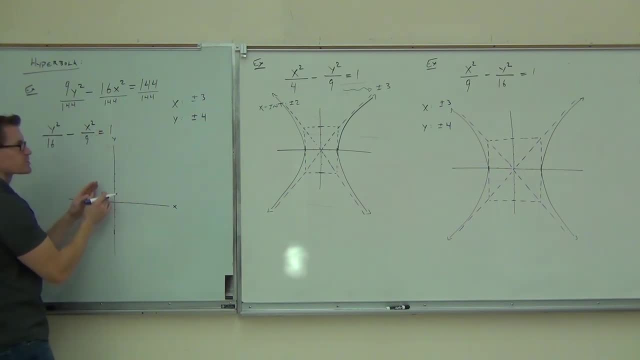 Plus or minus 4.. Let's make this box up. We know we're going to be plus or minus. oh, I forgot one. Plus or minus 4 along the y. plus or minus 3 along the x. Here's 3, 3.. 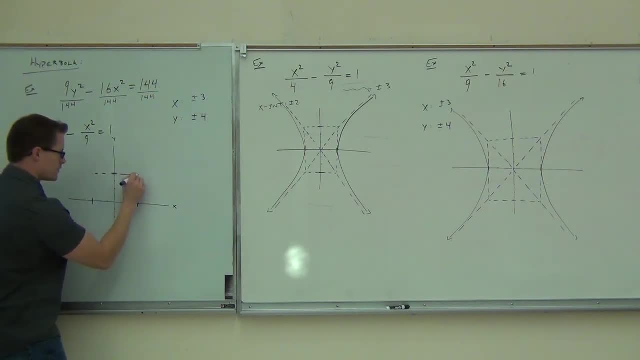 Here's 4, 4.. We'll make our diagonal line, just like we did before. Notice how the process is not changing. The only thing you've got to determine is where it goes. Is it going this way Or this way? 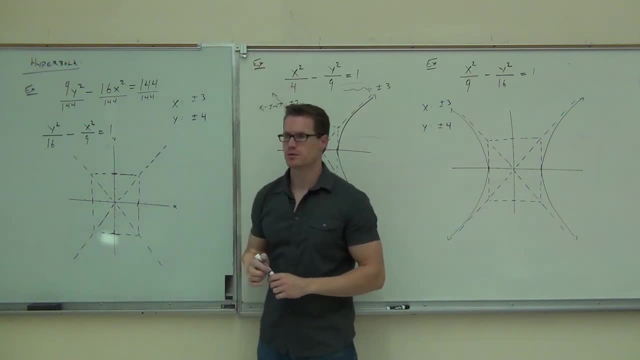 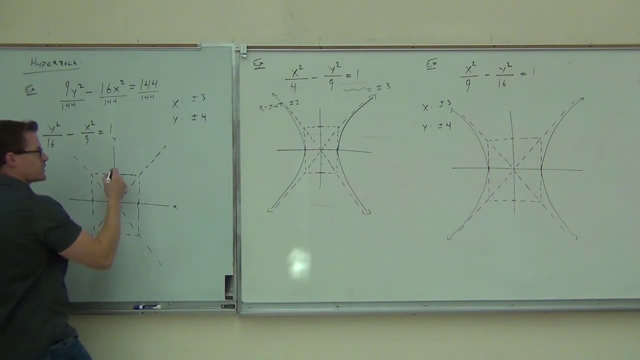 No, Yeah, it's vertical. Why is it vertical? So we'll go ahead and draw that. The y came first. That means we're spread out along the y axis. We will have y intercepts but no x intercepts. 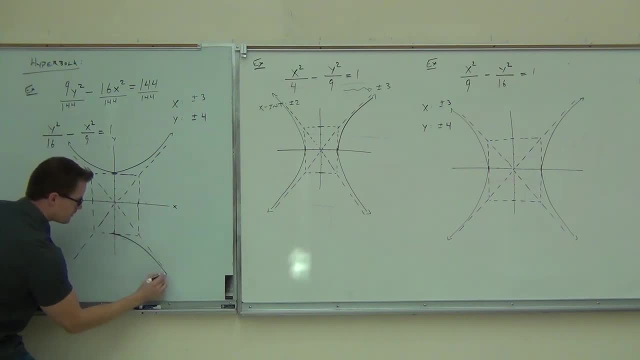 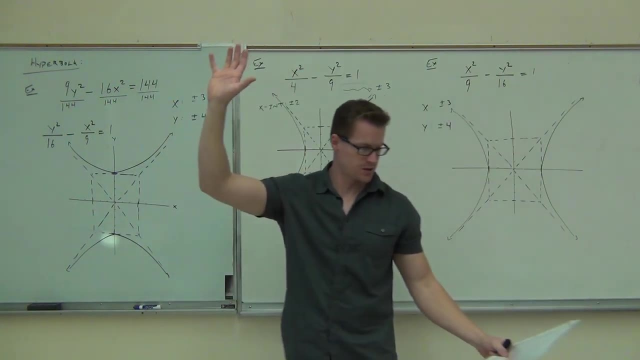 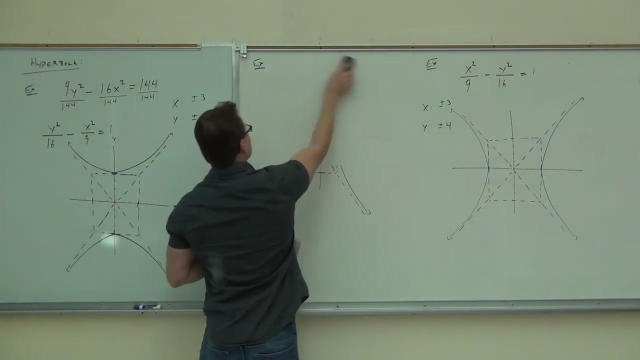 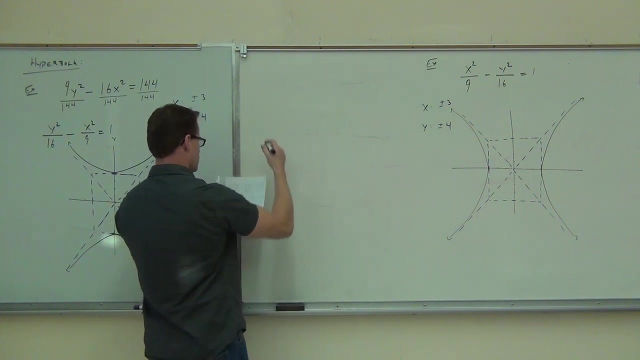 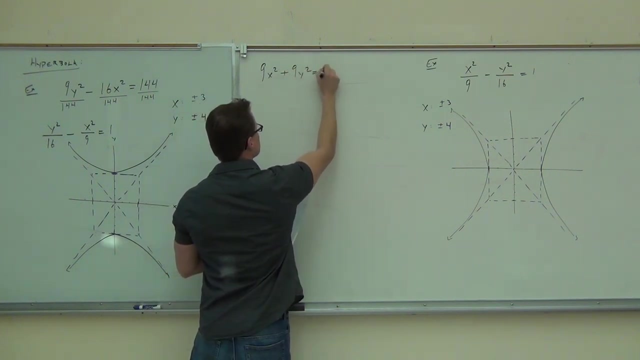 And that's the only way we can draw that. Would you raise your hand if you feel okay with our hyperbolas? so far, Okay, You're doing great. We're not going to do these problems, so don't worry. I just want to make sure you can identify what they are. 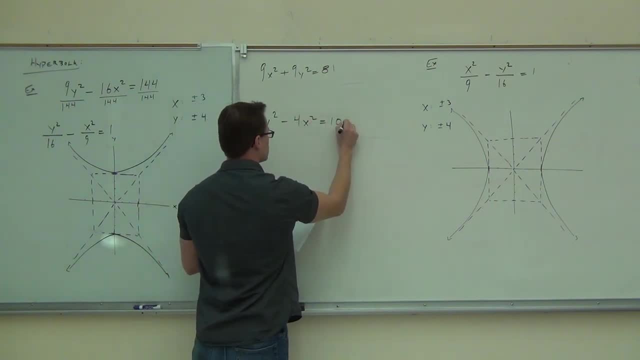 You can do this. We're going to close the top for now. We're not going to do these problems, so don't worry. I just want to make sure you can identify what they are. Dr, Dr. 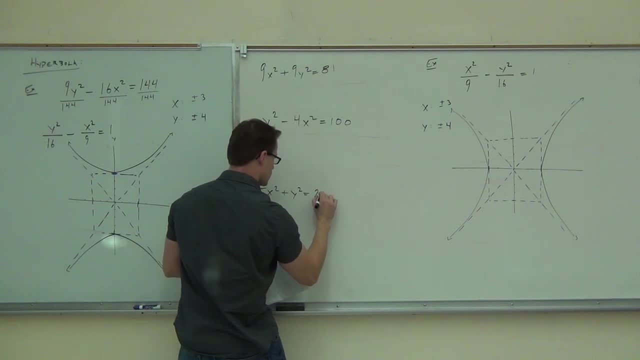 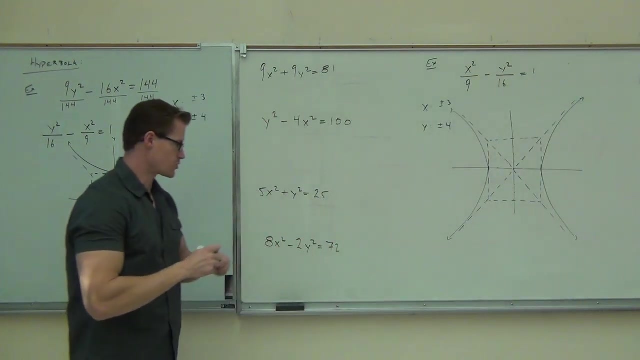 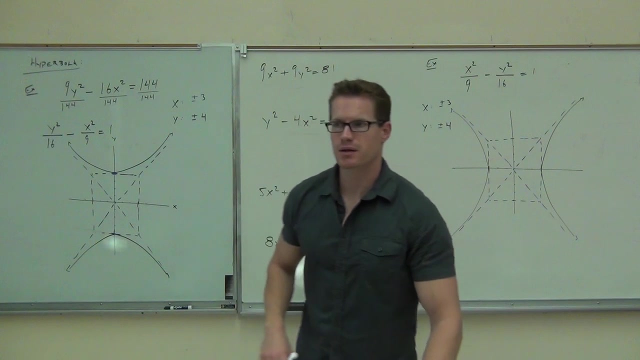 These ones might be good ones for you to try for your review. You should be able to identify what each and every one of these shapes are, So let's go right down the list. Can you identify what that is? 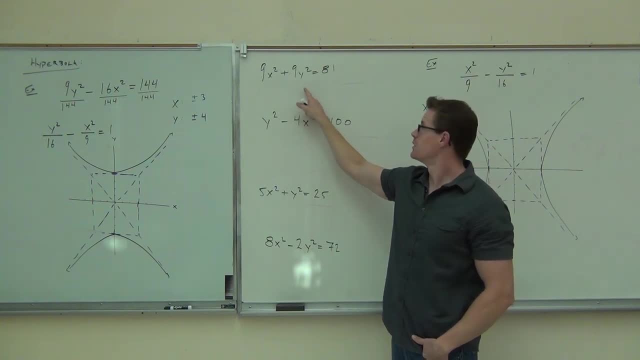 Circle, Circle, Circle. Okay, what's the radius? Three, Three, Three, Very good. Wow, that was impressive. Why not nine? Why aren't we looking here? Well, if you were to divide everything by 81, then take the square root of that. what? 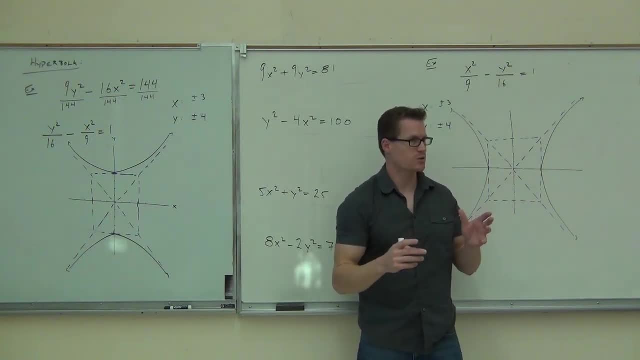 you get. you're going to get three, Not a radius of nine. So the first thing you got to do with circles: either get rid of those numbers or get rid of that number. Okay, either way, that would work for you.